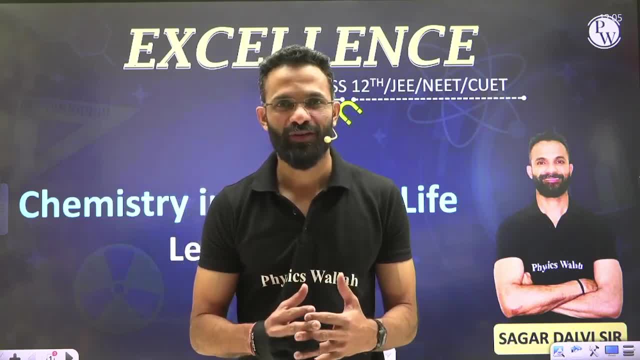 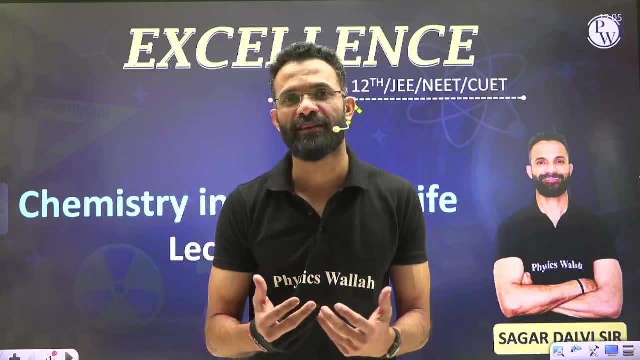 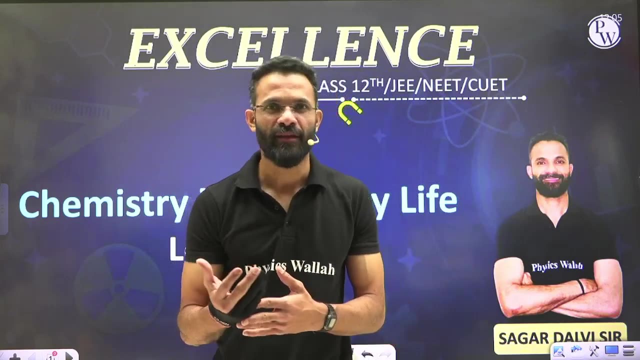 life today we are going to learn about all that. For example, see, when some disturbances in our biological process takes place, then we experience some general illness, some mild or moderate illnesses. For example, we experience minor pain, we experience headache, we experience 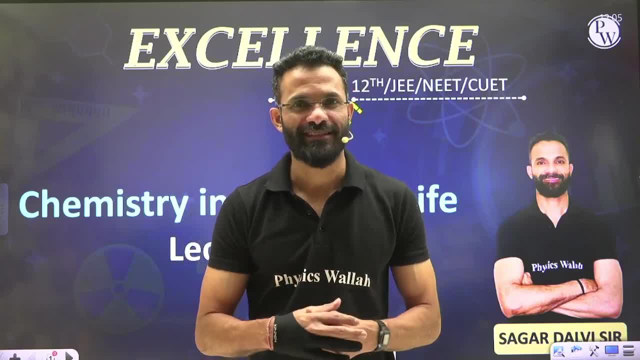 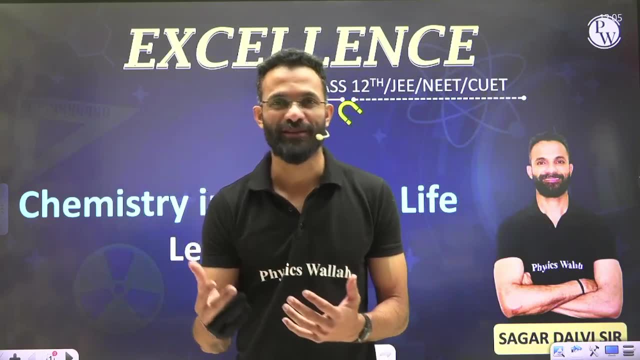 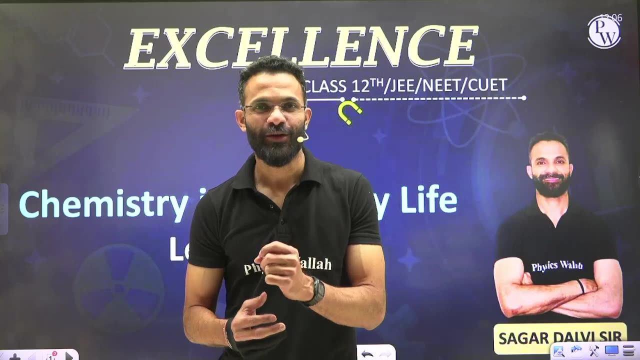 cold fever, all those kind of general illnesses. So when we are experiencing any of these kind of illnesses- not always- we approach the doctor. Sometime we take medicine ourselves, So we need to know that which particular medicine has to be taken when we are experiencing any of these kind. 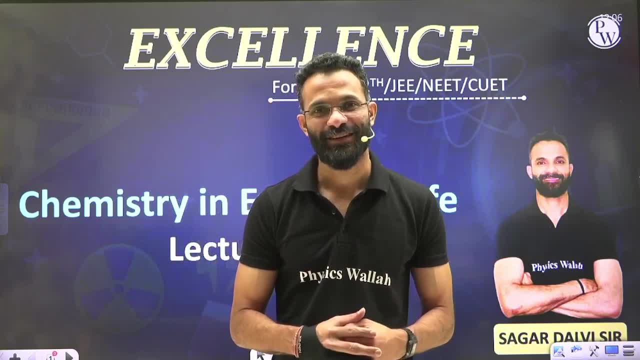 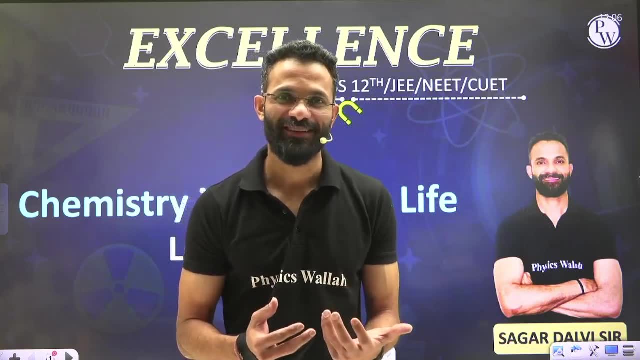 of disturbances in our biological processes. For example, it is very common that when we are experiencing some minor pain in our body, we tend to take paracetamol. So we know that. what is the function of paracetamol, right? everyone So in this. 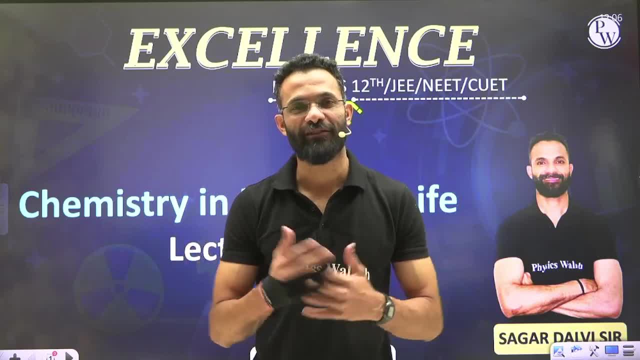 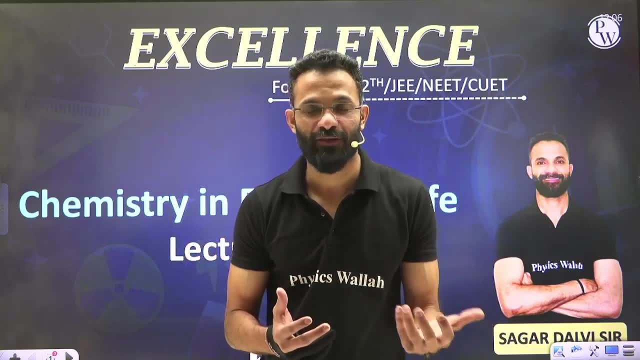 chapter we will be discussing about all those classification of wide varieties of drugs and particular drugs. if we are known by its name, then it belongs to which particular category and what is going to be its pharmacological effect. All this basic information we will be learning in 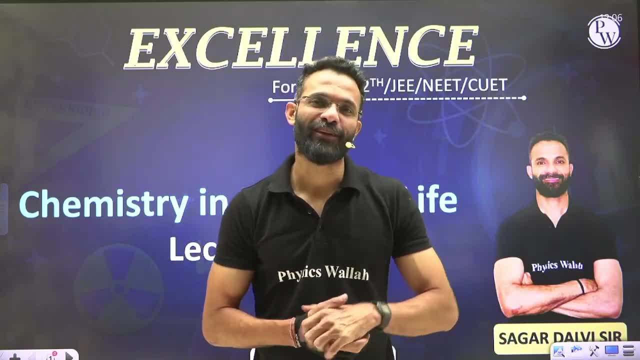 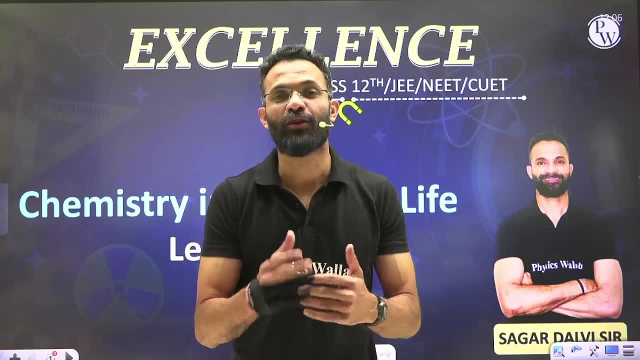 this chapter. Other than that, in our daily life we are going to learn about all those kind of compounds. In our daily life we come across soaps and the detergents. So all those types of soaps and the detergents, chemically, what are those kind of compounds? We are going to learn that today. So everyone, more or less. 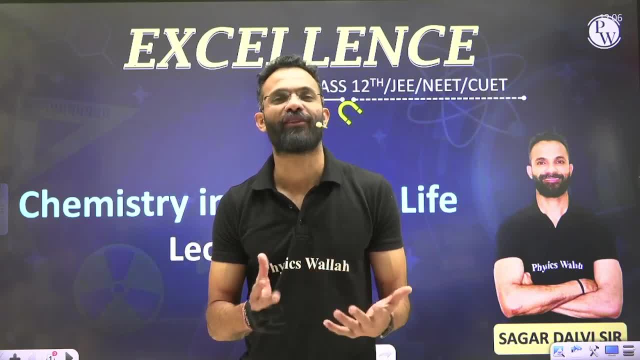 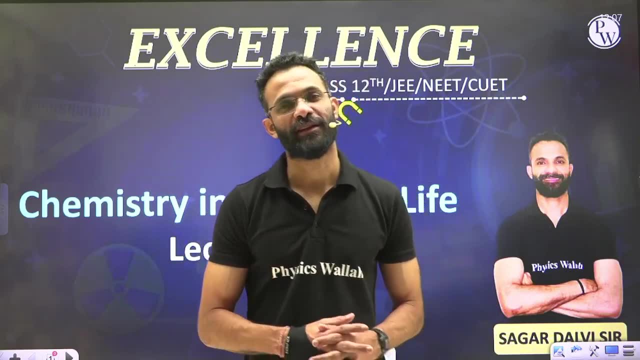 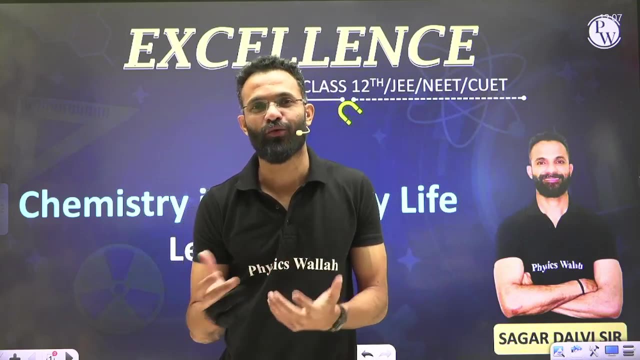 this chapter is going to be an informative chapter. You won't find we writing mechanism like we often do it for other parts of organic chemistry. So, yes, it is going to be an informative chapter. But let me also tell you that if you see all previous questions, you will find at least one or question. 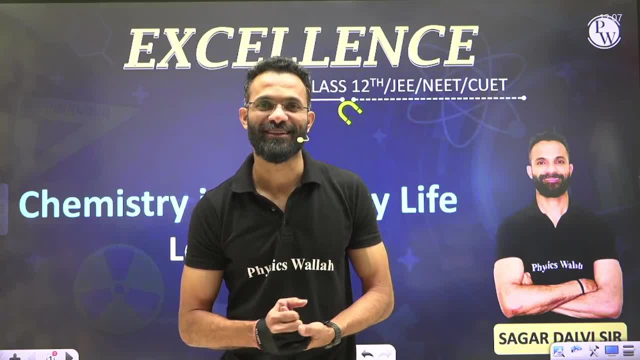 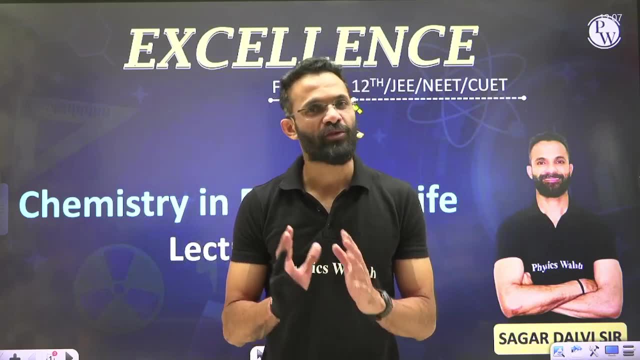 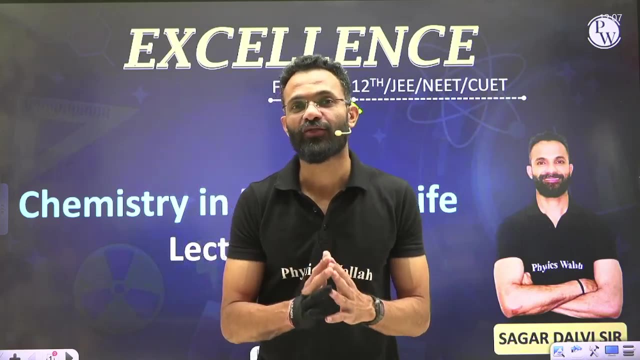 coming up on alternate years, So that's why this is important as well. Well now, as far as examination point of view is concerned, I would say the information is going to be quite easy. The only thing will be, if you're talking about a particular class of a drug, then we will have to remember many 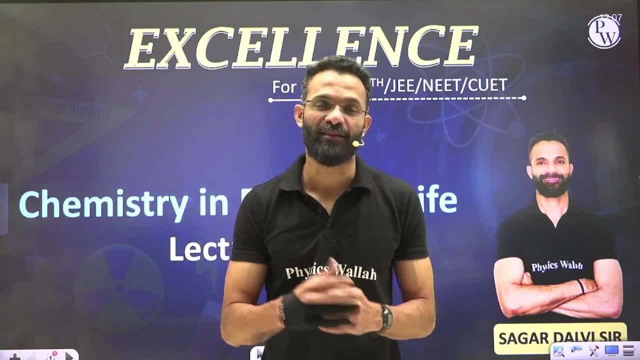 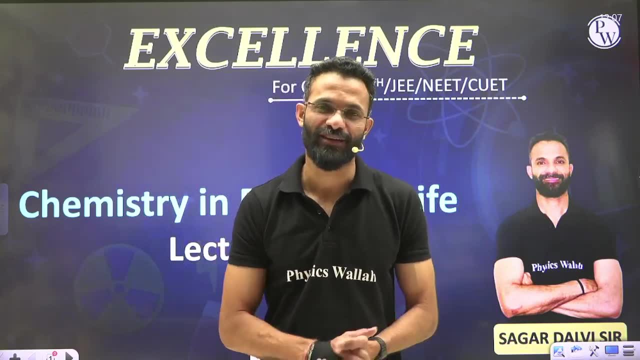 names of that particular category of a drug. So the task for you guys is going to be of remembering the names of a different chemical substances or drugs, what you can call it everyone. So, yes, you will find at times things are getting more informative, but we have no. 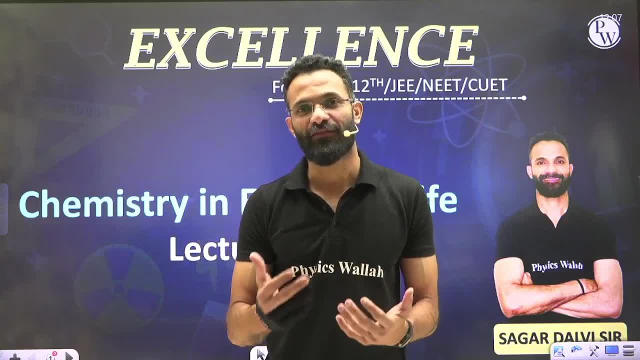 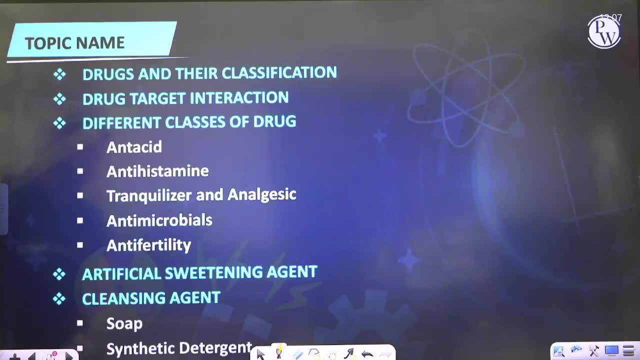 option. It's just that we'll have to make sure that we are practicing enough to remember the names of medicines. So, guys, let's get started with chemistry in everyday life. Let me just brief you first what precisely we are going to learn today. So first we'll get introduced to 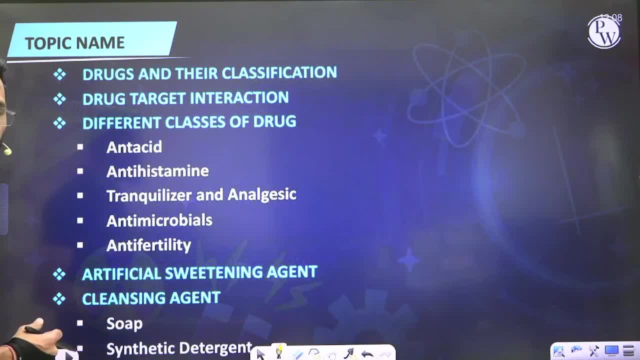 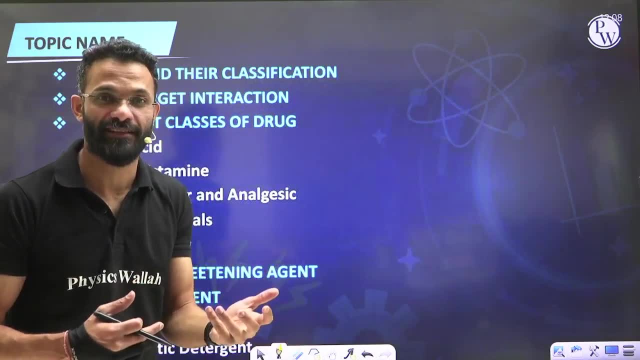 the drugs and the classification of drugs. Then we'll talk about how drugs exactly interact with some macromolecular targets, which we call it the chemical targets. So let's get started, So we'll be learning interaction between the target molecules and drugs And then, like I said, we 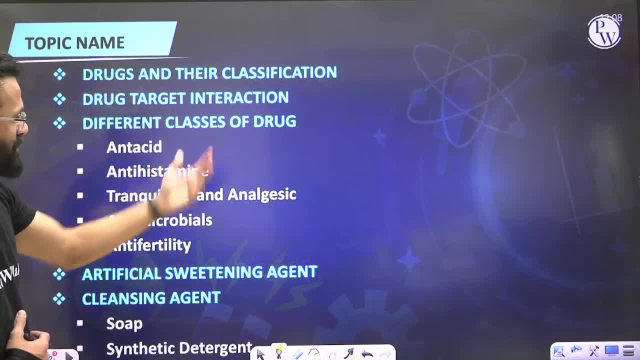 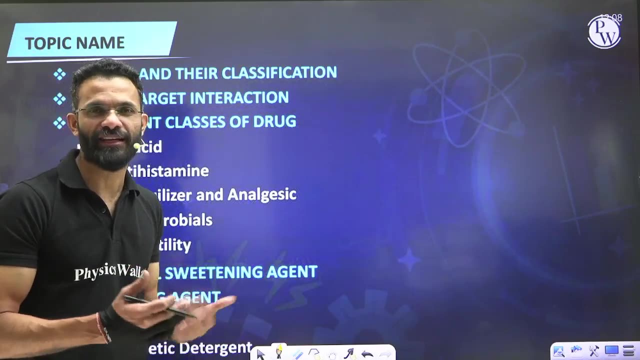 will be learning different classes of drugs and examples of each one of that, which will include what are antacids, what are antihistamines? We'll be talking about tranquilizers. Well, tranquilizers are those drugs which we basically eat or we take it for any kind of disease or 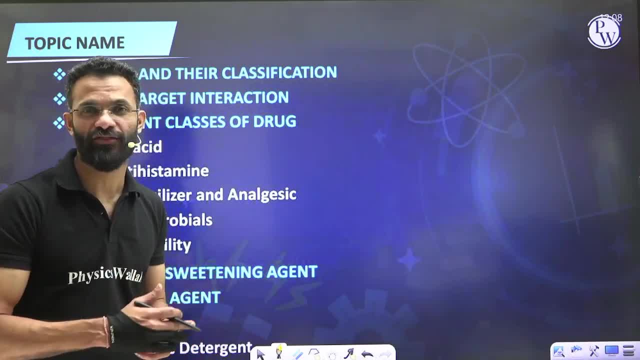 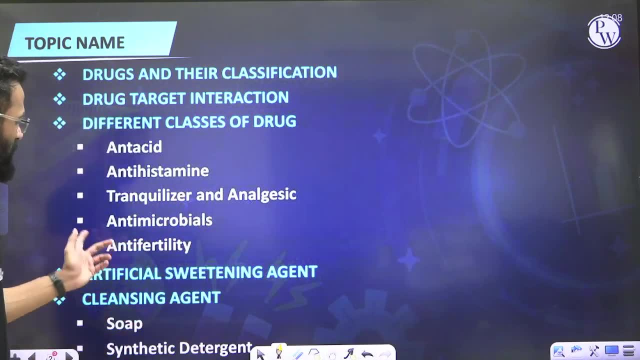 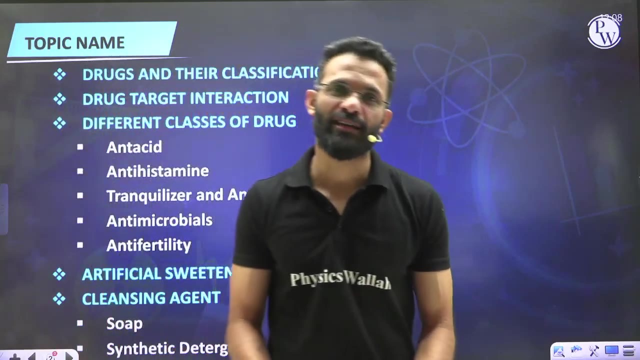 stress, anxiety or any other those kind of mental illnesses. We'll be also learning about analgesic. Of course painkillers belong to this category. Then we'll be talking about antimicrobial- Antimicrobials- basically, they are nothing but antibiotic, antiseptic and disinfectant. So all 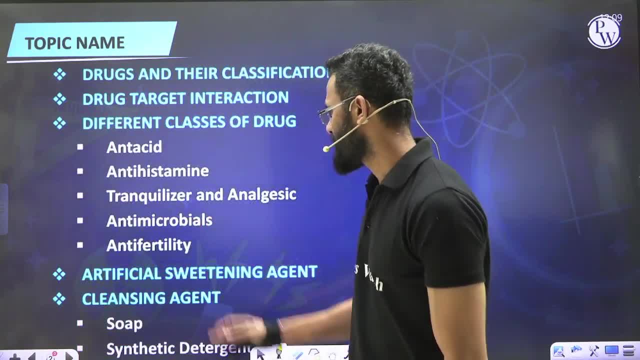 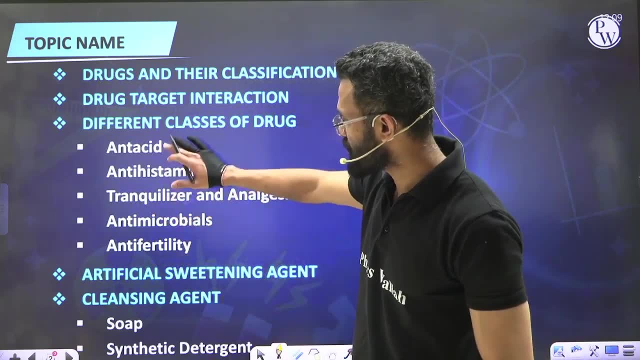 those three categories will be coming under: antimicrobials, And then, eventually, birth control pills is what you call it as anti-fertility drugs. So, guys, these are the different class of drugs that we'll be coming across And, like I said, the only task for you guys would be to 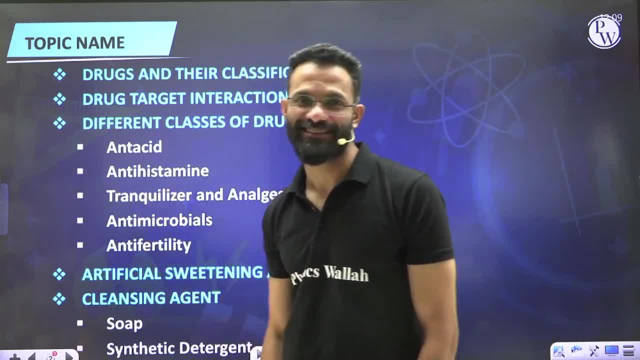 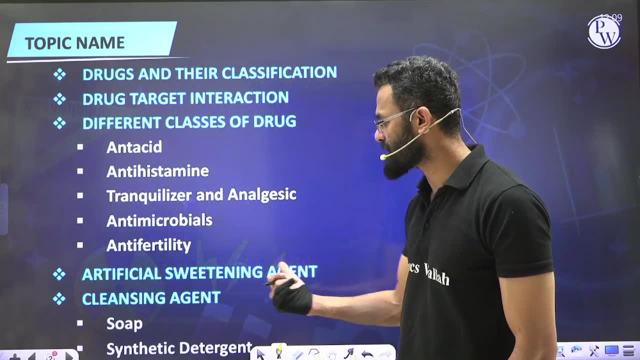 remember the examples of these different classes. Once this is done, we'll be then talking about artificial sweetening agents. So these are basically chemical substances that we use in our food, Followed by we'll be talking about cleansing agent, that is, soap and synthetic. 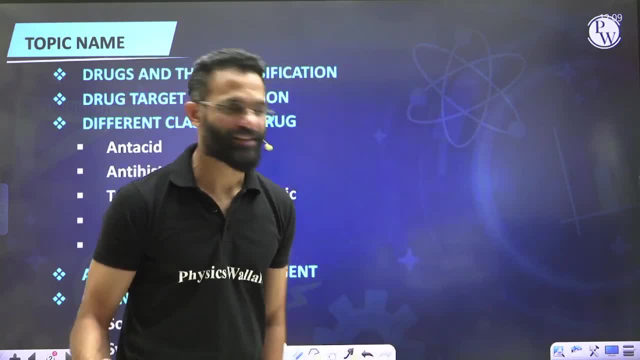 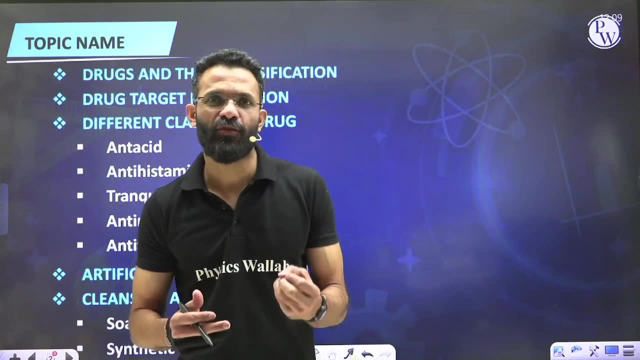 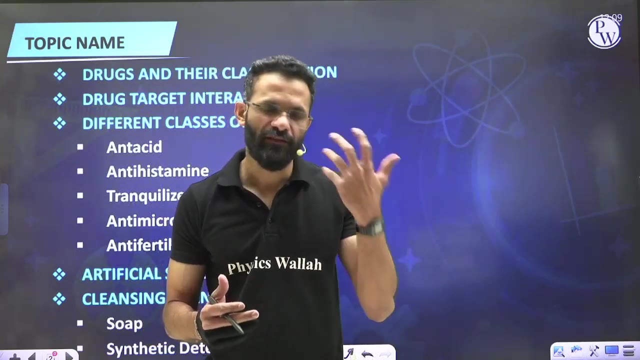 detergents. So, guys, let us get started with the first, that is, what are drugs? Well, let's take example of what we come across in our daily life. Look, suppose, if you are experiencing some pain in some part of our body, or even if you are experiencing, let's say, 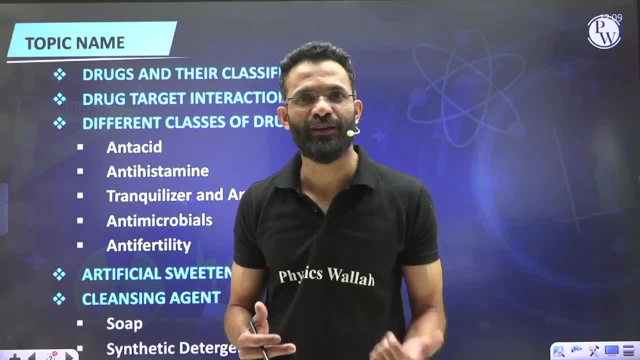 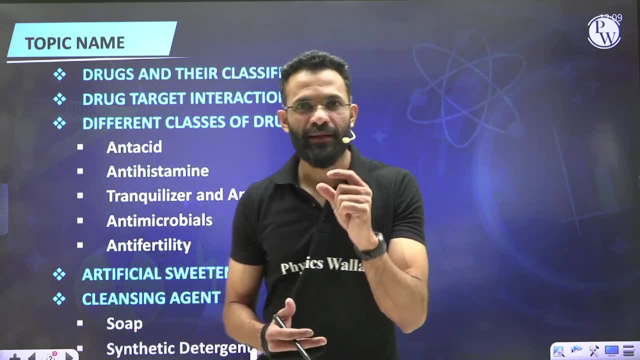 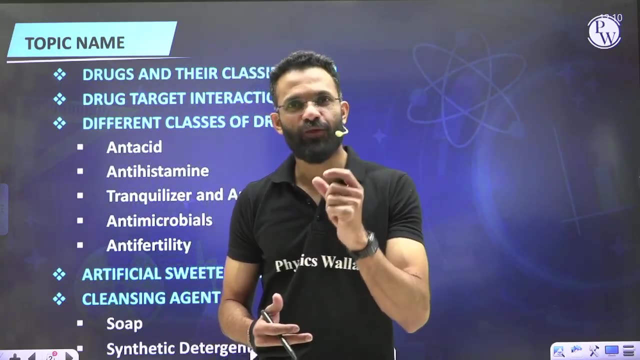 headache. So we take a tablet such as Crocin, a very commonly used tablet, right? If you have ever seen that tablet, then you will see that on that tablet it is anyways. one tablet is going to be how much Like? probably one or two grams, Yes, But if you read what is written on the tablet, 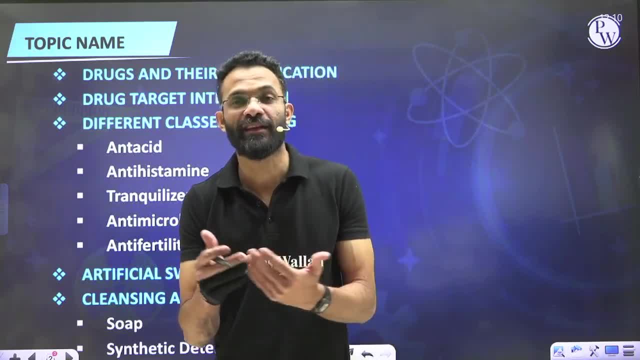 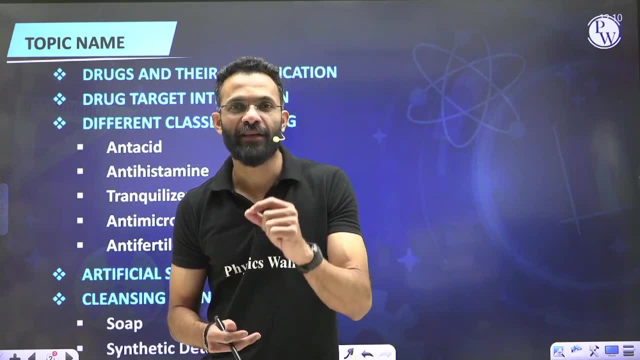 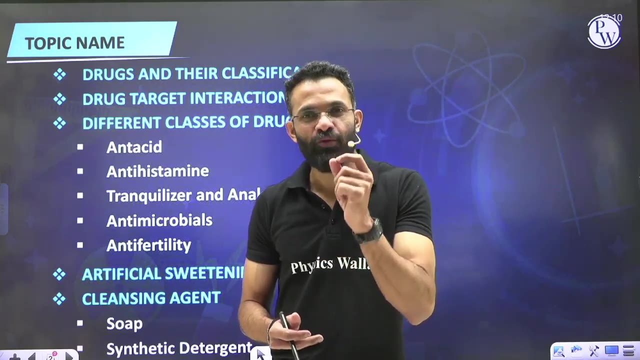 you will see that it is 100 mg, 50 mg, sometimes as low as 20 mg also. So that mg that we see, that is basically an API. API is Active Pharmaceutical Ingredients. So if your tablet is altogether, let's say, of one or two grams, but the active medicine which is going to make 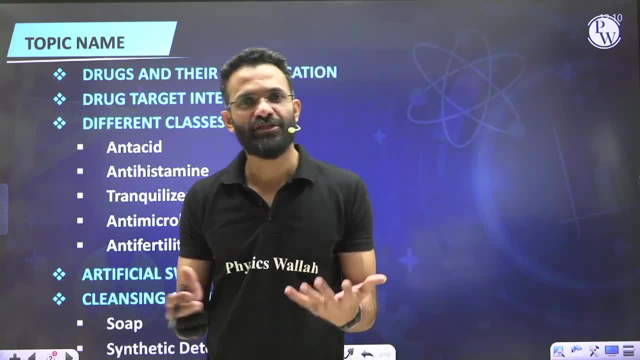 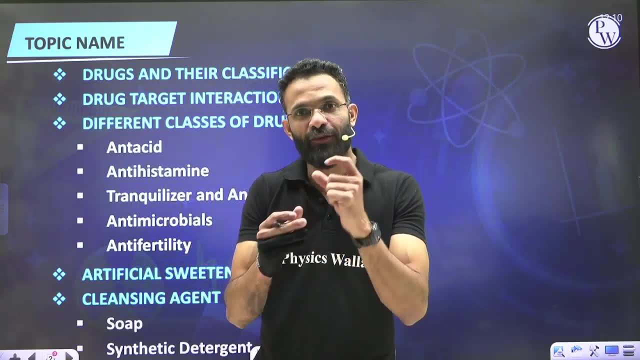 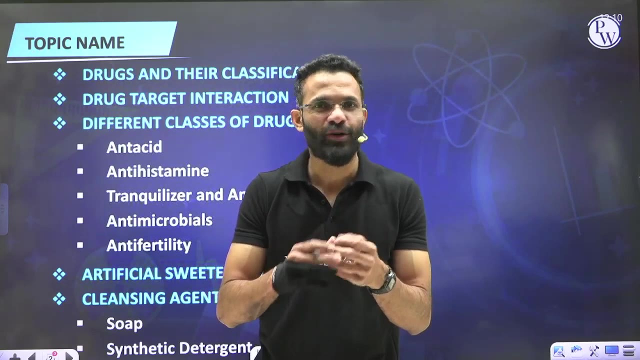 an impact on whatever illness you are experiencing is going to be just probably 50 milligrams. Rest of the thing which is present to make the entire weight loss of a tablet as one or two gram is basically other substances such as fillers or binders or some other. 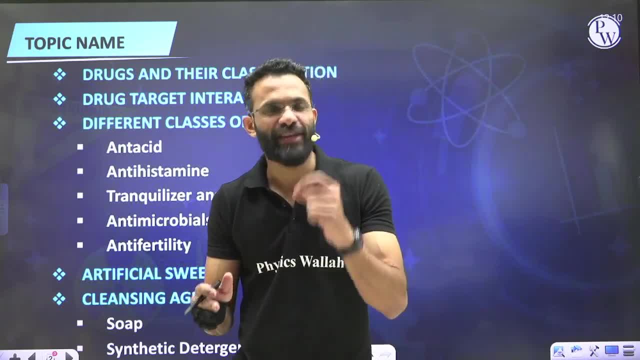 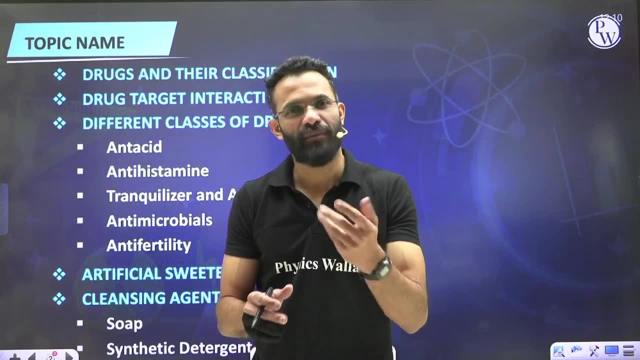 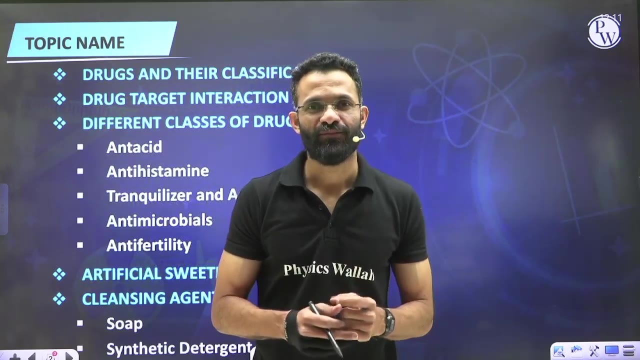 food additives, etc. etc. So the actual medicine which makes an impact or which treats the disease or illness is just about, let's say, 50 mg. So if you see the drugs which we eat- we always take it in a very, very low concentration- You will find these drugs, or the chemical substances, are the 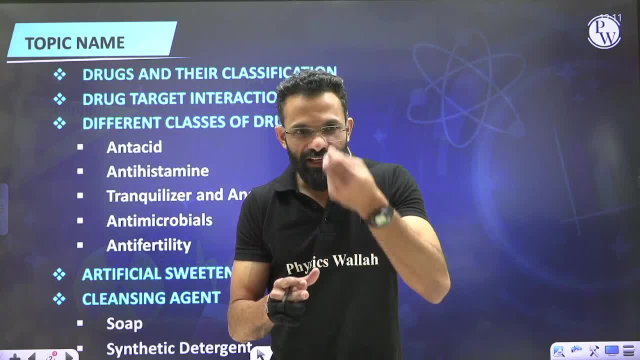 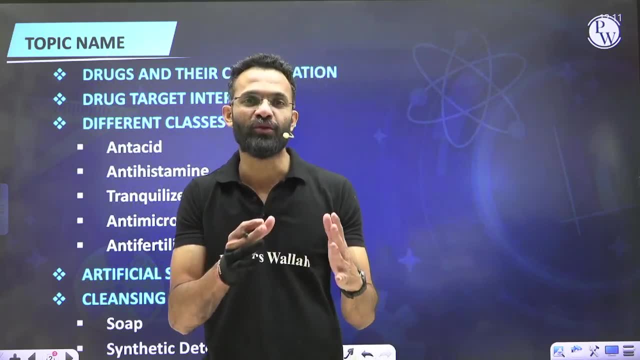 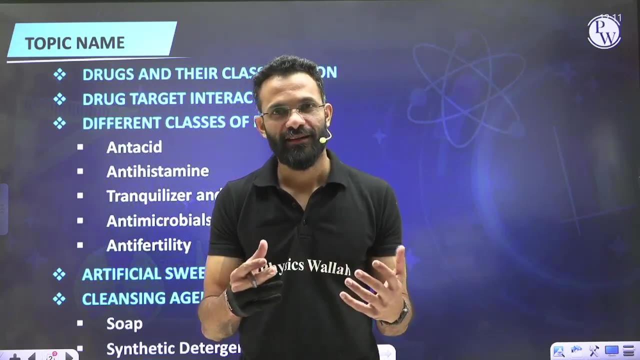 ones which are of low molecular masses. Now, when you eat those substances, these chemical substances interact with some of the macromolecules in our body, such as carbohydrates, proteins, lipids, etc. Now, when these chemical substances, which are of low molecular masses, interact with the target, 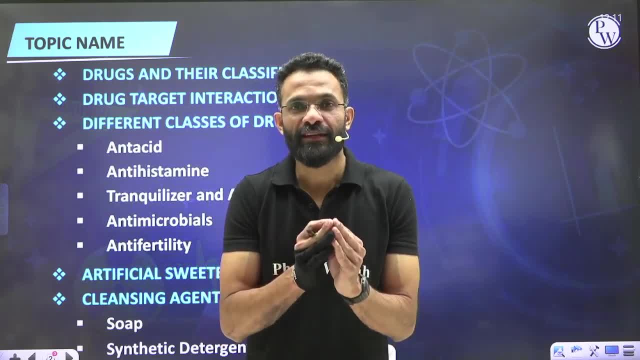 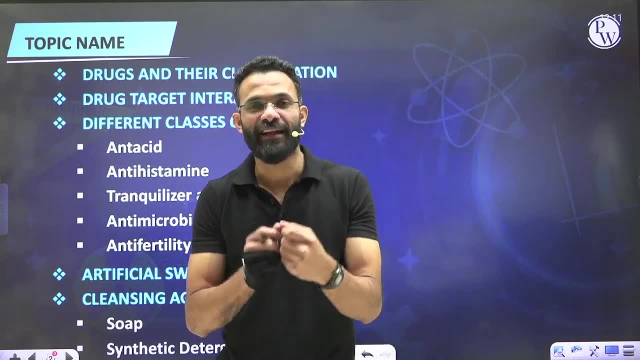 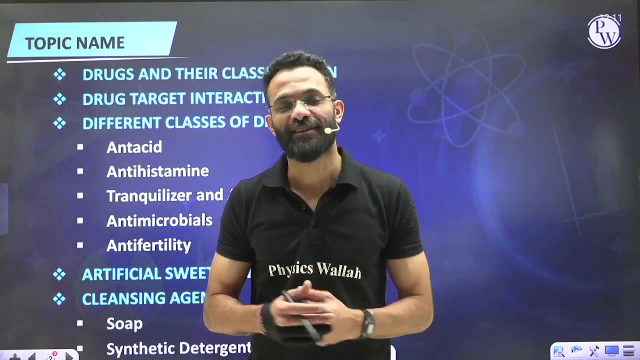 molecules, the macromolecules which I said. this creates some therapeutic response. If the response created or if the response given by the interaction between chemical substance and the macromolecule is therapeutic and comforting to us, then those chemical substances we call it as drugs. 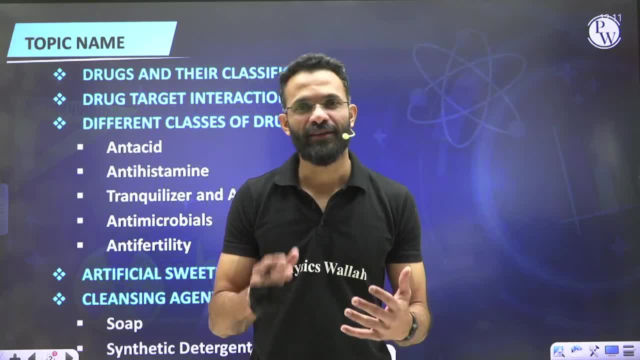 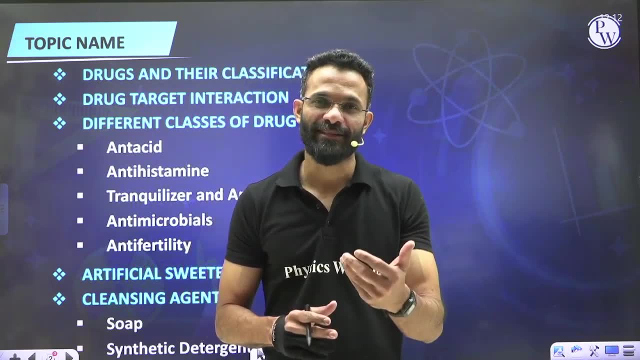 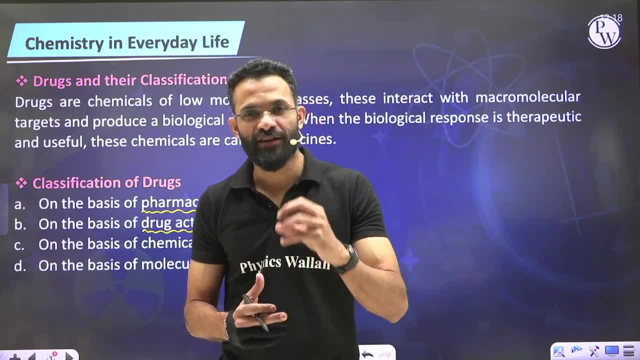 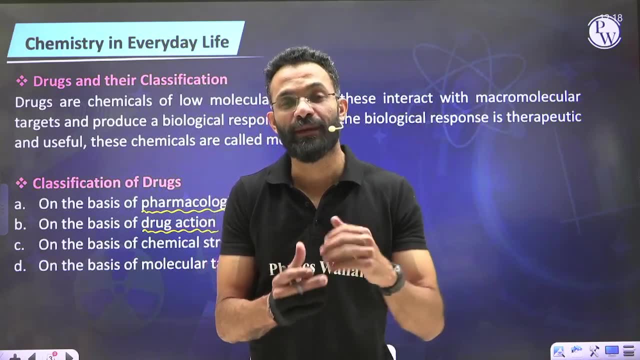 then it is a drug. If that response is therapeutic, comforting, relieving, then it is a drug. If that response is therapeutic, comforting, relieving how exactly these drugs affects the biological process. we need to first understand how, in general, biological processes takes place themselves, and then how drugs are used to repair those processes. 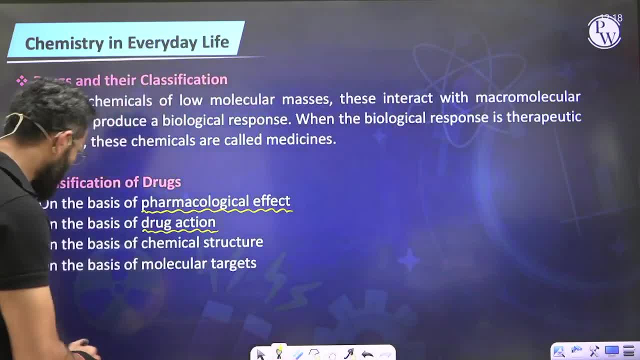 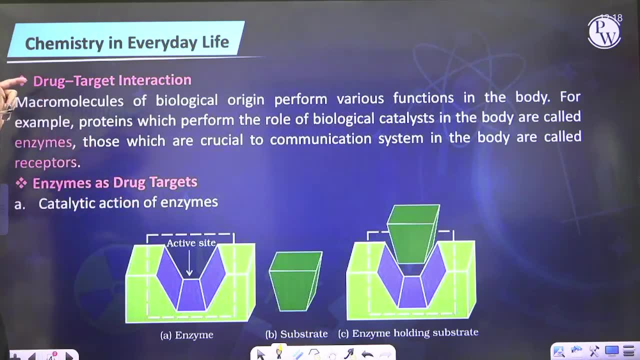 hence it is important for us to first understand that how exactly a particular biological processes takes place. so in order to understand drug target interaction, like i said, drug target interaction, target are those macromolecules. targets are those macromolecules which basically are responsible for some of the biological processes. for example, if i talk about enzyme, so enzymes are basically. 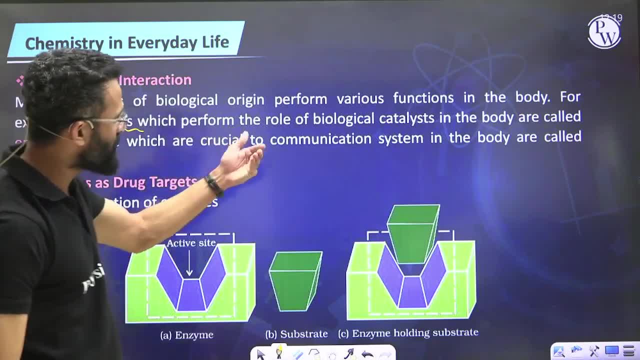 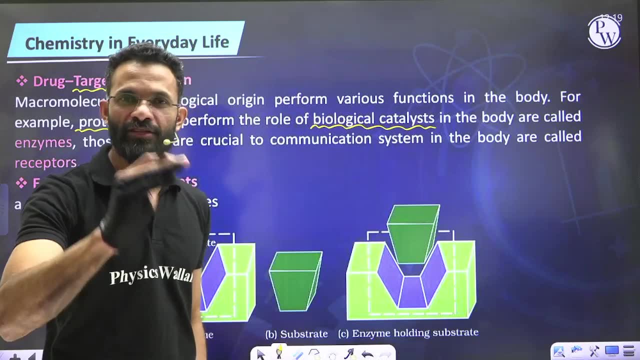 proteins, which performs a function of a biological catalyst in the body. so enzyme is one of the macromolecules of a biological process. so enzyme is one of the macromolecules of a biological target and that enzyme is nothing but protein molecule which performs the role of biological 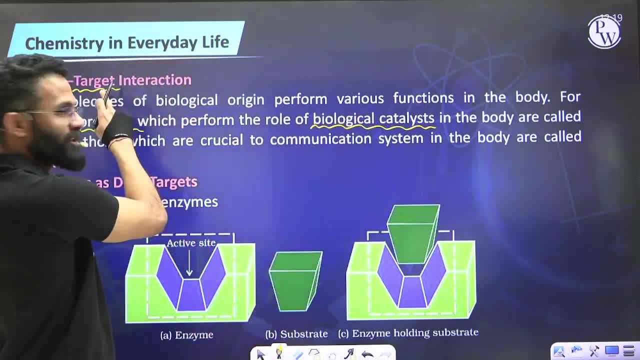 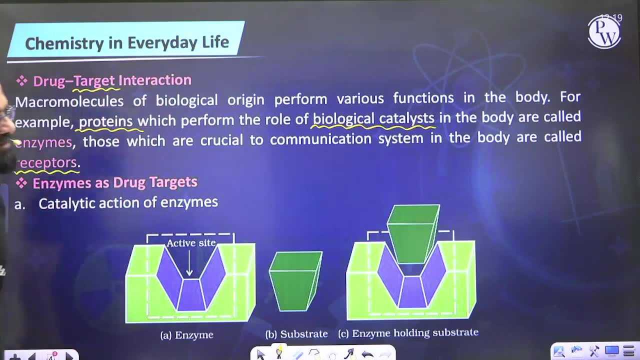 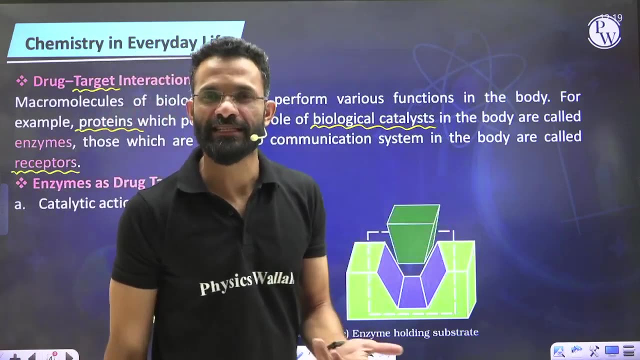 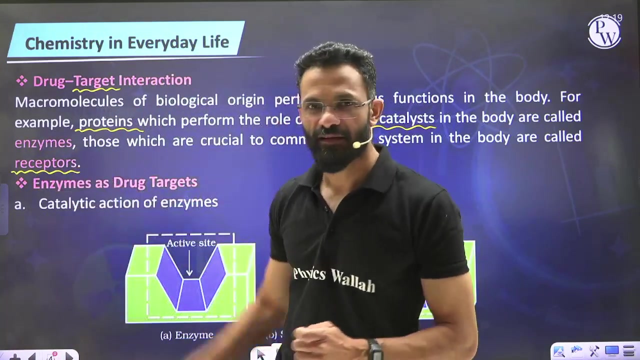 catalyst. so enzyme is one of the target, or a macromolecule similar to that. there is another target which you call it as receptor. so receptors are those protein which are basically important for the body's communication process. so the communication that happens in our body is basically performed by the macromolecules which we call it as receptor. now, when i talk, 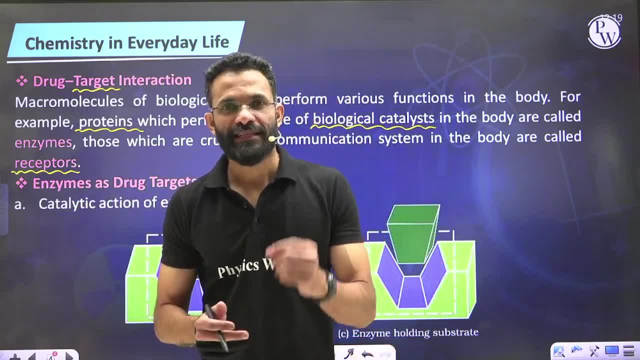 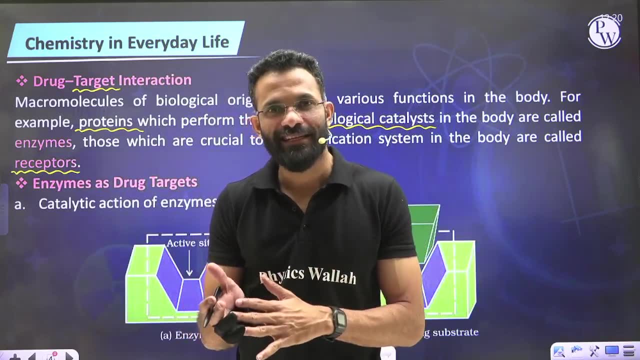 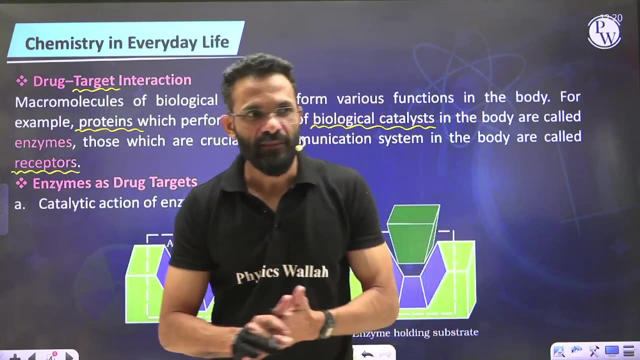 about communication. what does that mean? see the signal in the body from one neuron to other neuron, or maybe from neuron to muscle, is carried by some of the part of body which is what you call it as receptor. for example, let's say: uh, while playing we fell down and we got some wound on our leg. 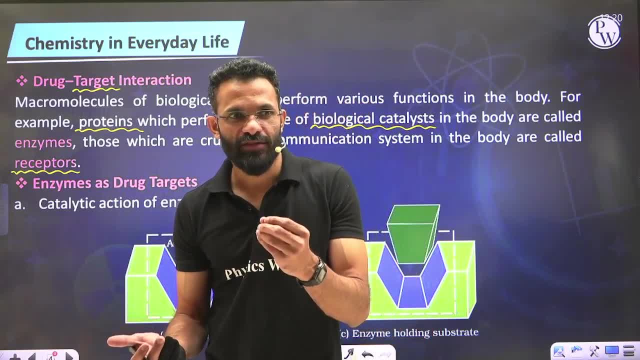 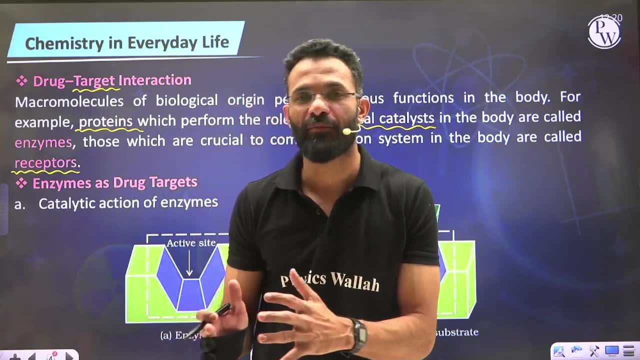 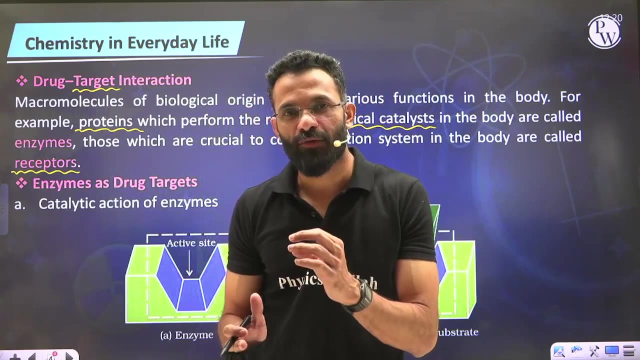 okay in our leg. so that wound is now slowly started causing inflammation and then that inflammation is going to cause pain in that part of our body. but that pain which is caused in the body, or the inflammation which is caused in the body, is to be communicated through some chemical substances. 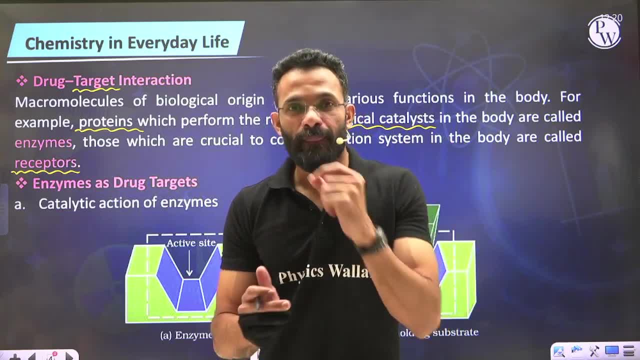 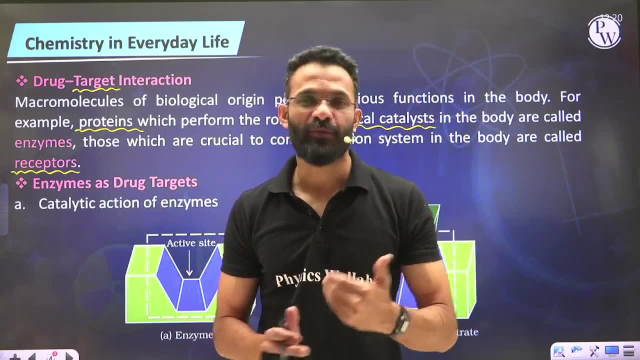 to our brain, so that communication process right from the wound and the signaling to our brain is carried out by the brain, so that wound is now slowly started causing inflammation and then that pain is carried out. that process is basically carried out by the macromolecules, what you call it as. 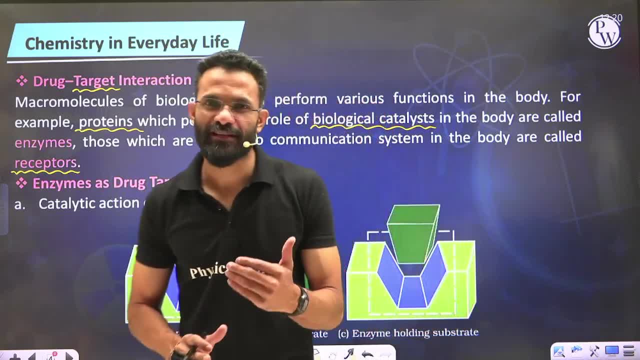 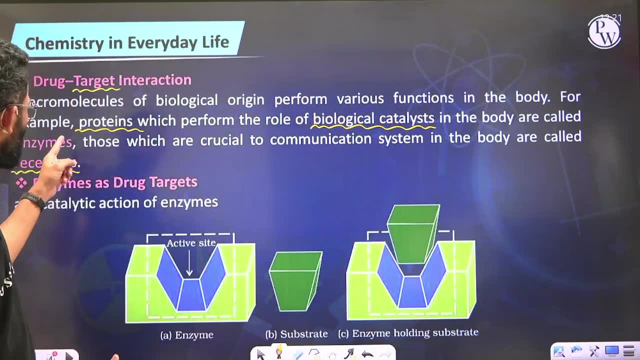 receptor. so basically, today here in our chapter, as far as our syllabus is concerned, we will to discussing about to important macromolecules or molecular targets, what his enzyme and receptor, and then we will see how drugs interact with this enzyme and with receptor. but before we 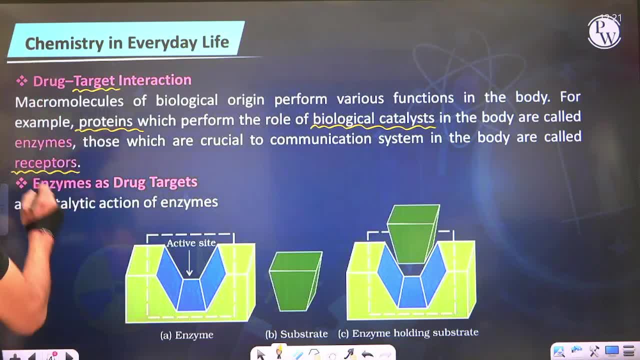 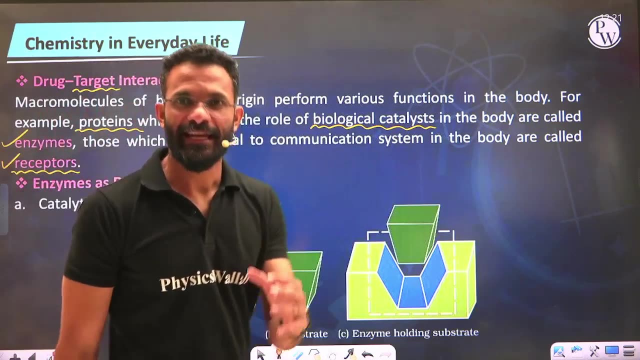 learn the interaction will have to first understand how enzymes and receptor function Themself, and then we'll talk about how drugs interact with them. So let us first talk about Enzyme as a molecular target. So, like we said, Enzyme are basically a protein molecules which are responsible for the catalytic activity. 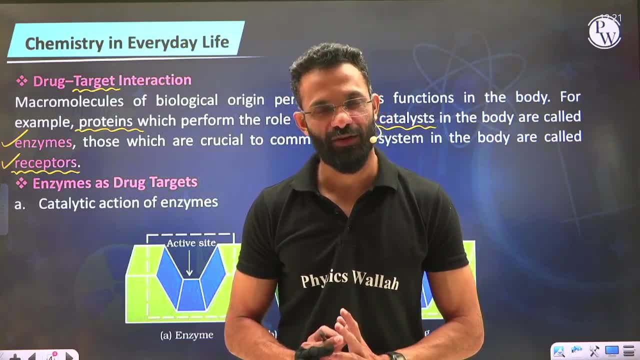 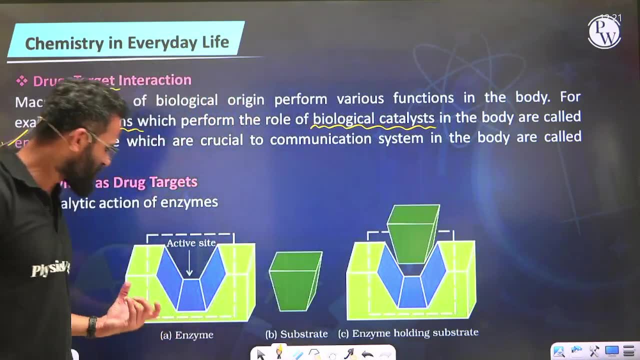 What a particular biological processes. All right, so how exactly this enzyme functions. Let us see that first, everyone. Okay, so let's say, this is a protein molecule which you call it as enzyme. You see, here in that enzyme, There is a particular site which we are calling it as an active site, or there is a cavity which you are calling it as. 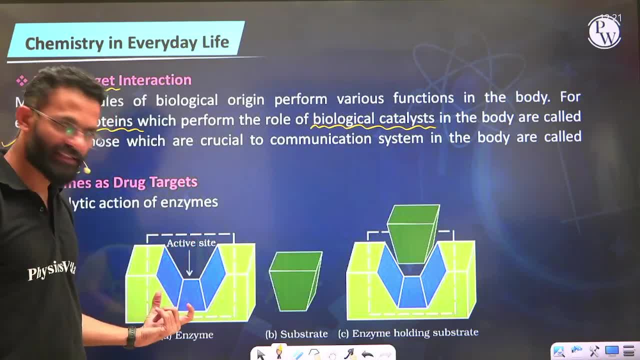 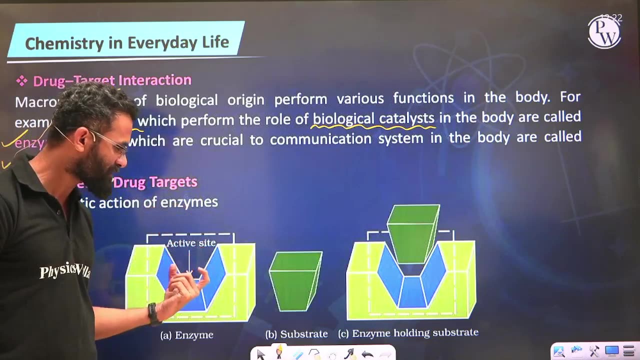 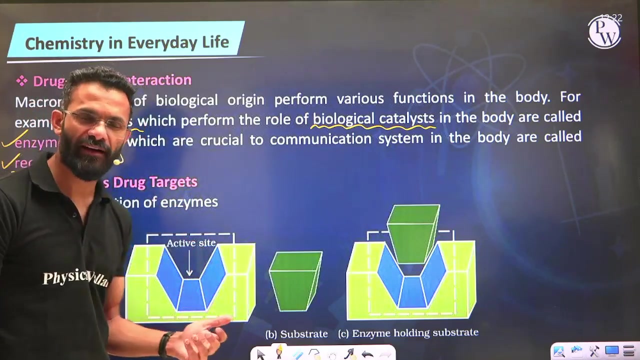 active site. so what this enzyme does is: this enzyme provides this active site for some substrate to come and get accommodated in this particular cavity. Now accommodation of that particular substrate In this active site takes place via several interaction. So the interaction between the substrate and the active site could be via ionic bonding or could be van der Waal forces. 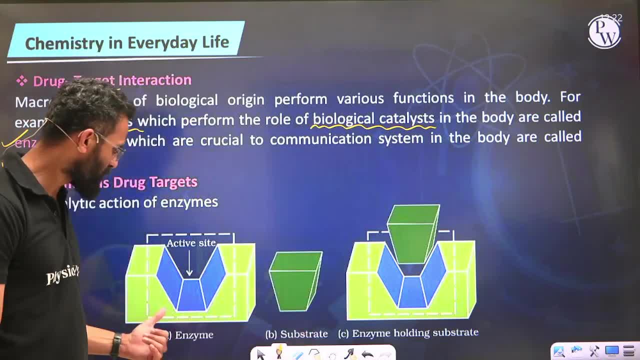 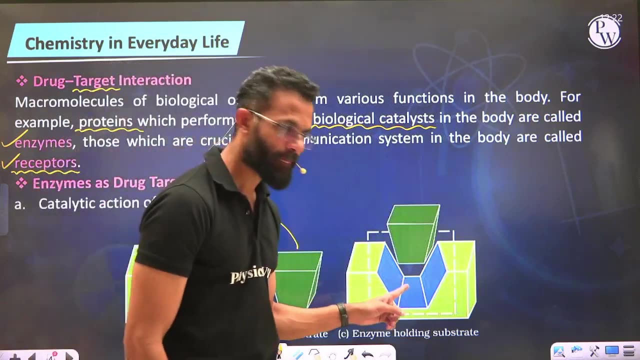 Hydrogen bonding, so on and so forth. So what protein? what this enzyme does? it provides active site for the substrate to get Accommodated in this particular active site. once it gets accommodated, You can see the substrate is being accommodated in the active site, like here, and the interaction that is. 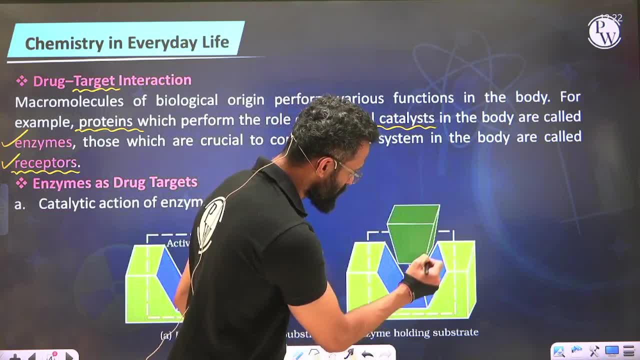 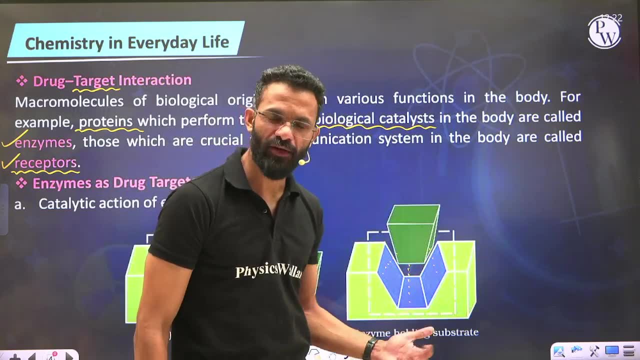 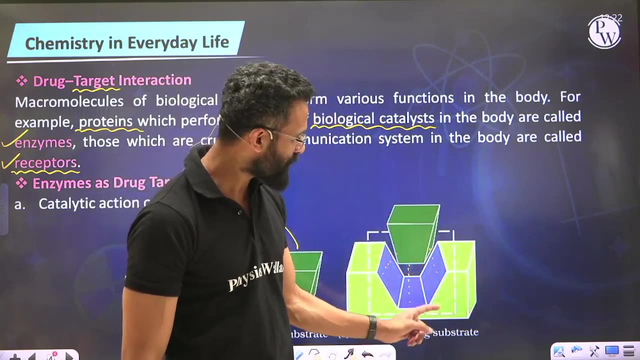 taking place between The substrate and this part of enzyme is why ionic bond or weak van der Waal forces, or could be hydrogen bond, Once it get deposited in this active site. now the second function this enzyme. does this enzyme allow this substrate to react with external 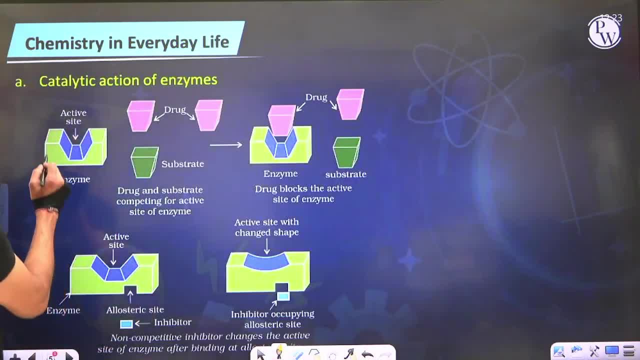 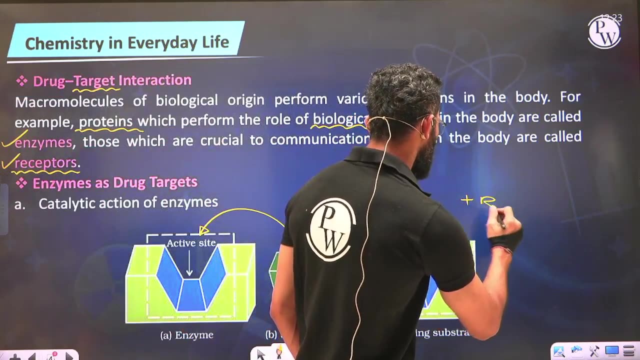 Reaction. let me show you that diagrammatically. So you see enzyme is provided active site. this active site Basically will allow substrate to get deposited here and then the substrate will be brought in contact with some external reagent. So this, After getting accommodated, will interact with some reagent and will produce some biological response. 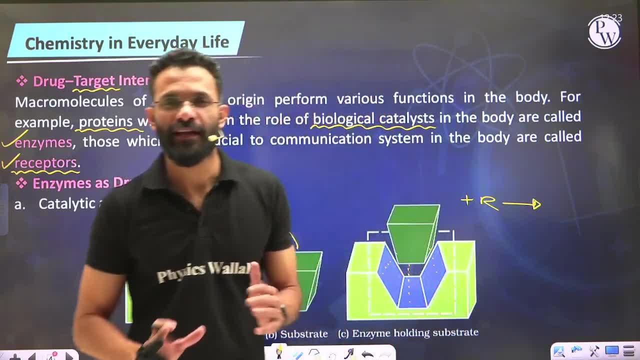 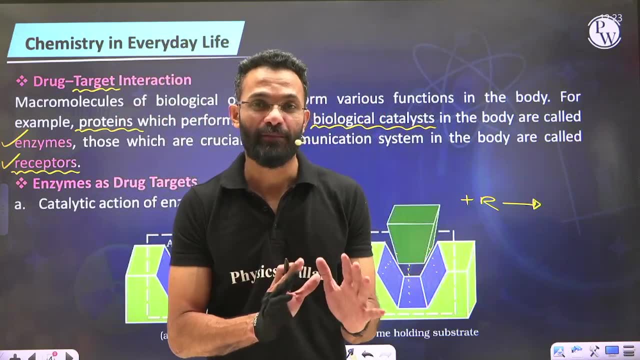 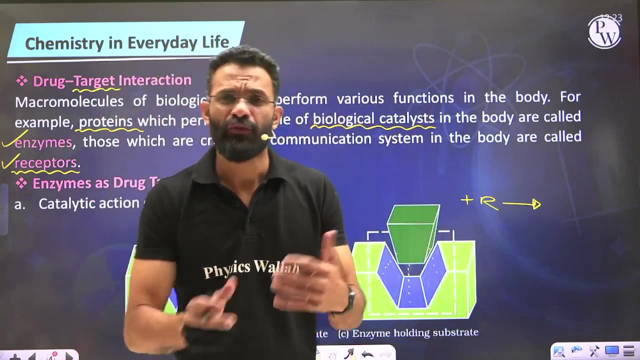 Now let us take one example again. whatever example I'll be telling you, This is just for the sake of understanding the concept. Biologically, it will not be absolutely correct all the time. All right, so let's say, if i'm talking about: uh, we went for a party to a friend's place the other night, okay, 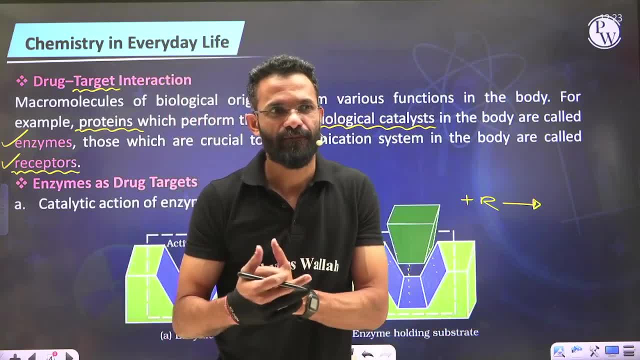 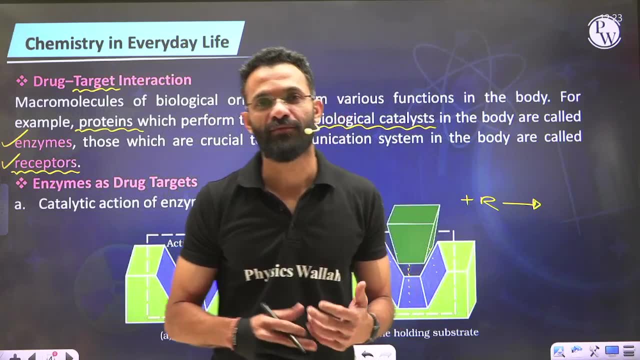 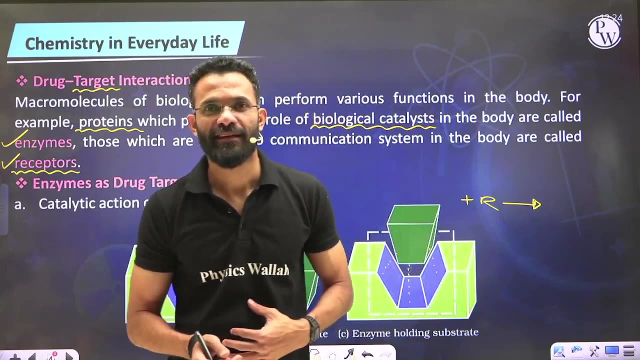 and we ate some food which was probably not good or it was a spoiled food. so, because you ate a spoiled food, it started creating some infection in your body, which you call it, as in general, food infection, all right, so the next morning you started experiencing stomach ache and slowly. 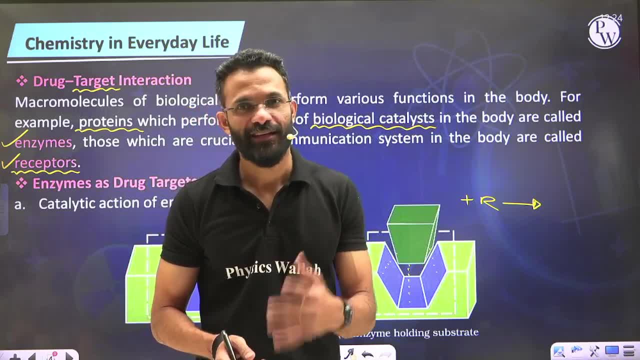 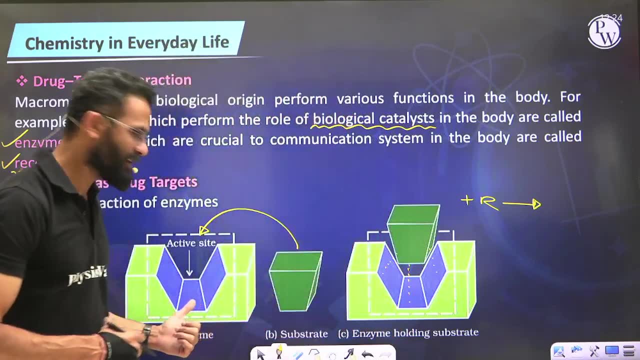 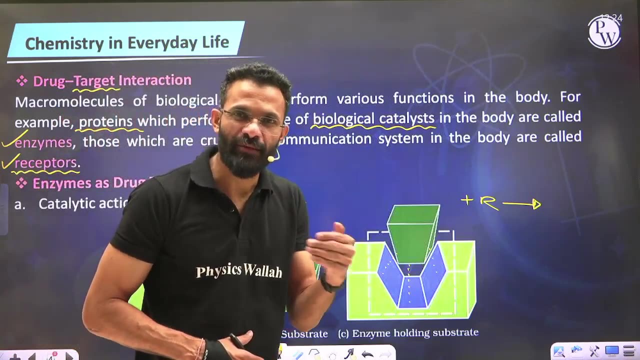 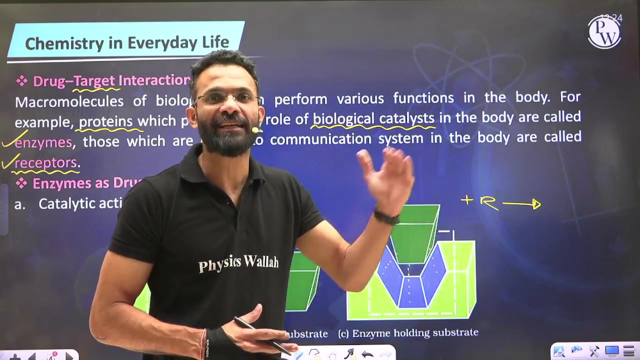 you started getting feeling of vomiting and you realize that the food infection has occurred in your body. so how is this process related to the enzyme and the substrate? interaction is, let's say, the food infection that is causing or that is taking place in your biological system is slowly, slowly enhancing, is slowly, slowly increasing. and how is that? increasing by time? 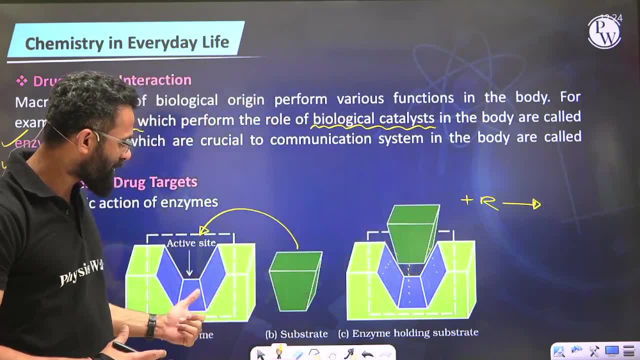 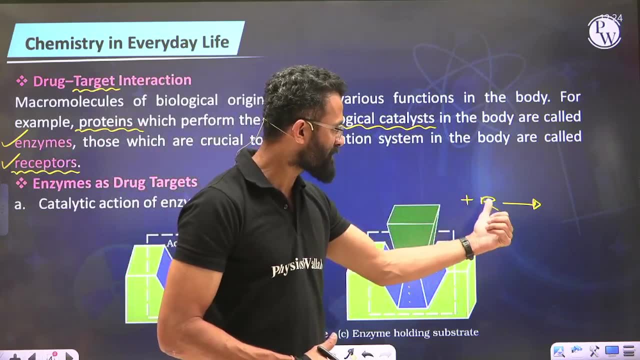 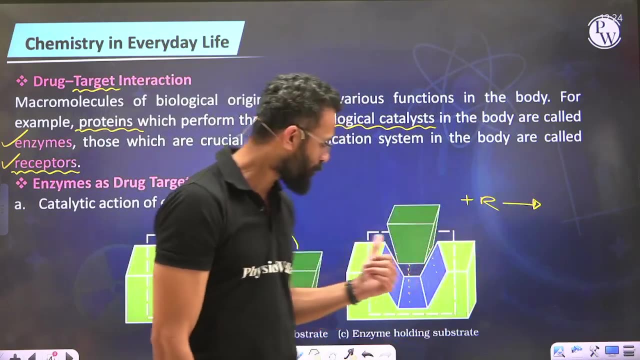 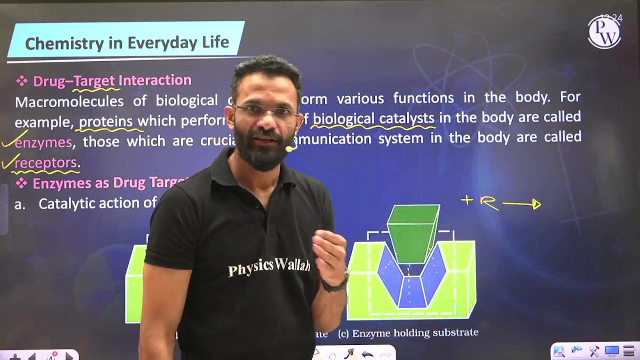 is because this enzyme is allowing some substrate molecule to get deposited and once they get deposited, they are allowing some external reagent to react with it and the reaction rate have been getting increased. so whatever reaction is taking place, its rate have been increased because this enzymes are acting like a biological catalyst. so the food, 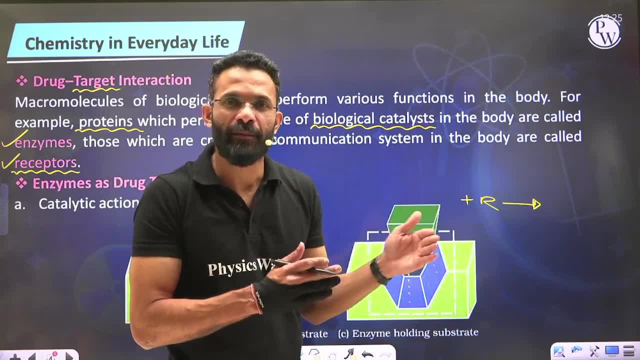 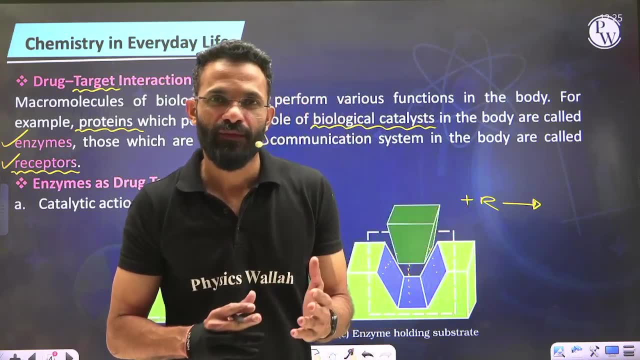 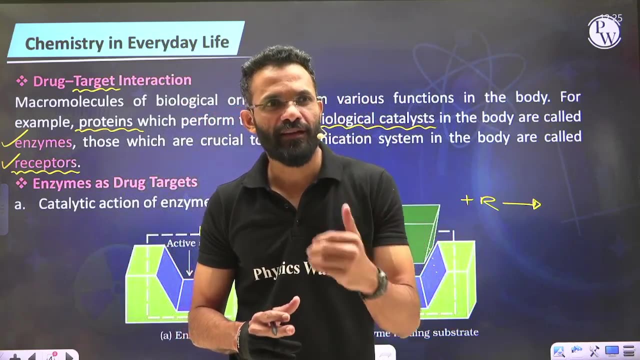 poisoning that we are experiencing is getting aggravated by time because it is being catalyzed by some enzyme present in our system. now what we do once we start experiencing this: we go to the doctor and doctor gives us some medicine, and that medicine probably after eating. maybe in a days time or maybe in few hours, we start feeling. 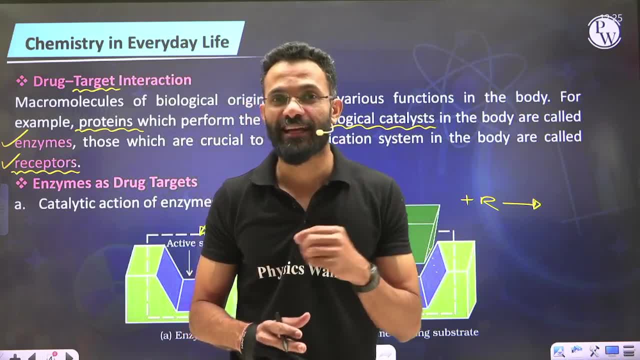 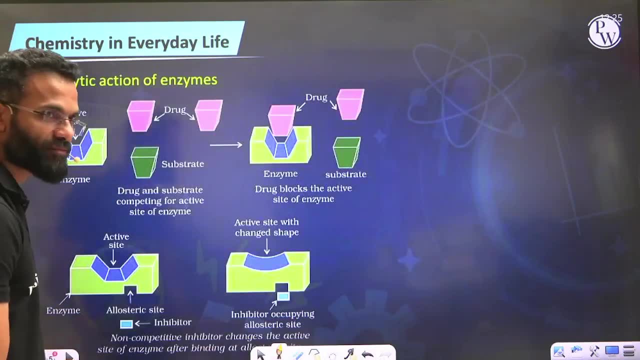 better. so what this medicine is doing is what we have to understand: drug target interaction. so now, see, now we went to a doctor and doctor gave us some medicine. let's say this is the medicine or a drug. now, if you see, the shape and the size of drug is exactly similar to that of substrate. 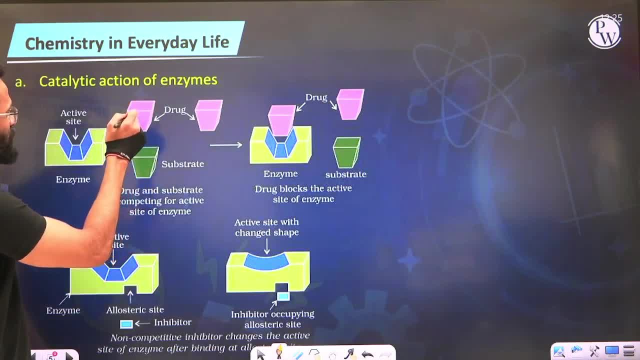 so when you eat the medicine, what this medicine will do? this medicine or the drug will compete with the substrate which was getting deposited in the cavity of enzyme, so this drug itself will get deposited or itself will get accommodated in that active site and will not allow substrate to get. 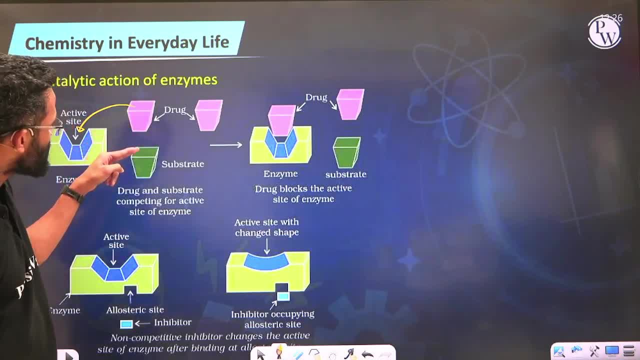 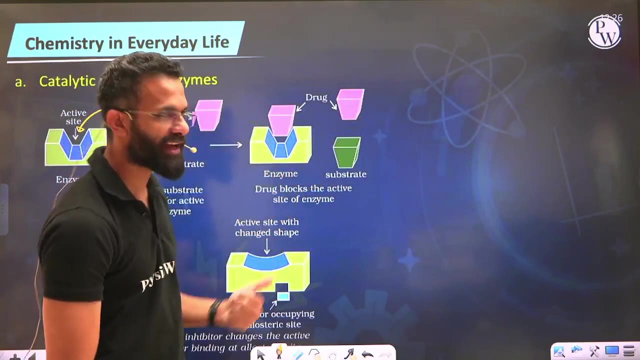 accommodated in this active site. so what this drug has done is this drug has literally competed with the substrate and itself got accommodated in the active site. now, once drug get accommodated in this active site, of course there is no way now substrate can come and get accommodated. so the interaction between the 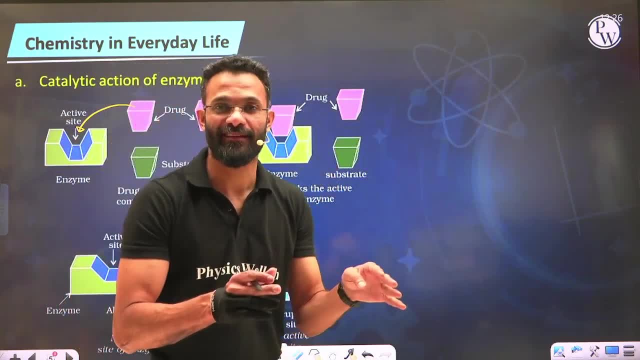 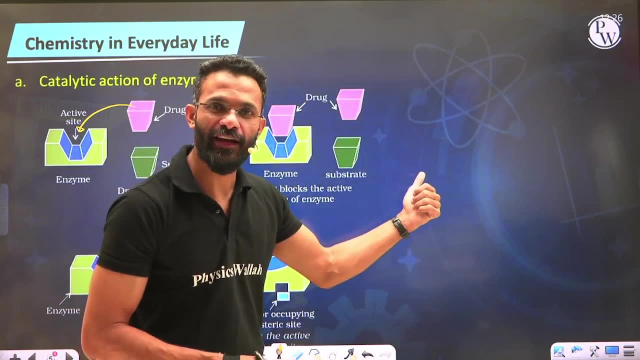 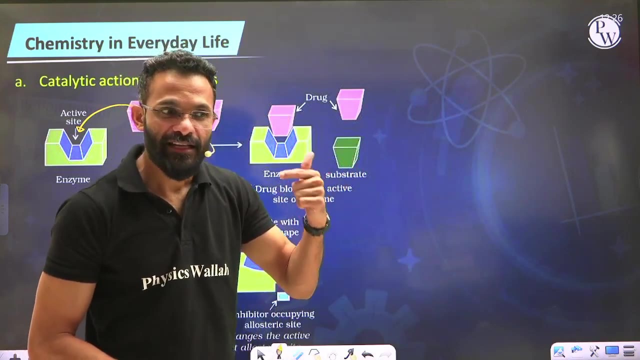 substrate and enzyme have been inhibited have been inhibited. if substrate will no more get accommodated in the enzyme, it cannot further react with the reagent and it's no further reaction will takes place. so the food poisoning that we were experiencing, that reaction rate or that catalysis. 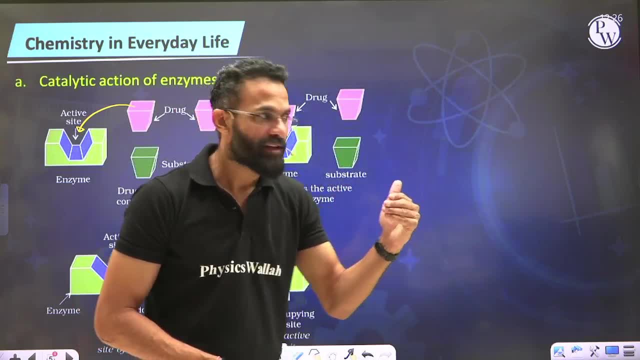 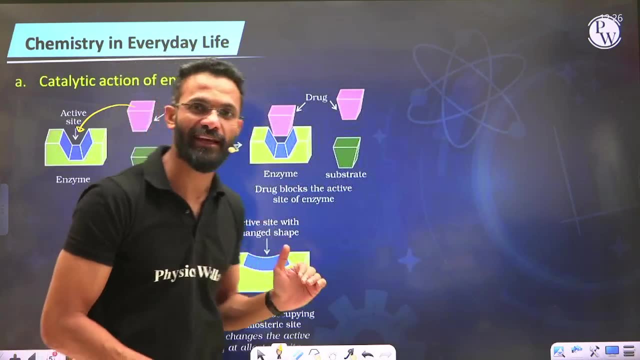 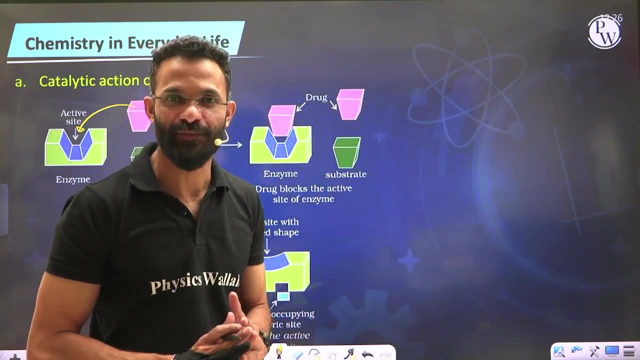 of the reaction have been now prevented. and now, if you eat sufficient concentration of drug, this drug will not let those substrate to get accommodated in the enzyme and hence, slowly, slowly, it will stop that reaction which was causing a food poison in a biological system. so such drugs, which directly compete with the substrate, 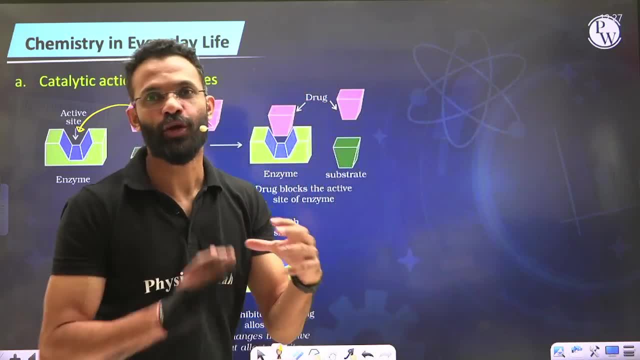 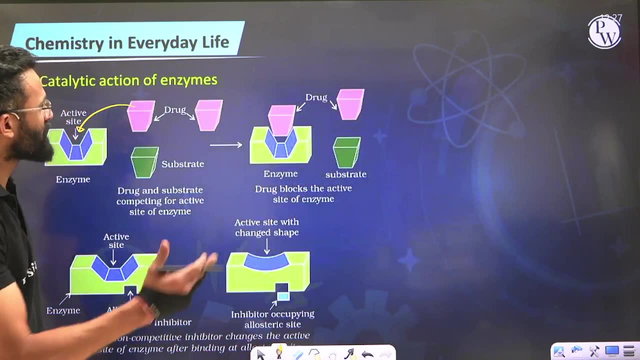 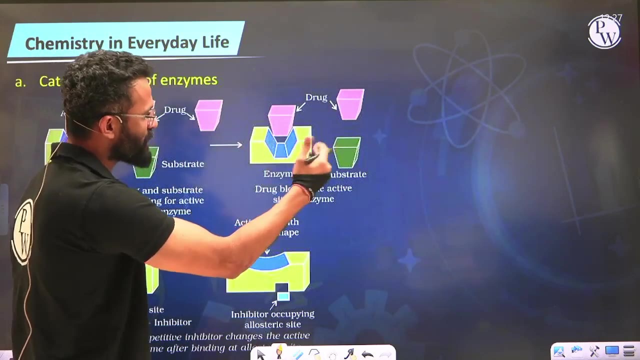 take place. so the food poisoning that we were experiencing that reaction rate or that catalysis, and inhibit the reaction. we call it as competitive inhibitors. what do we call it competitive inhibitors? so one of the type of drug which directly compete with the substrate and inhibit the reaction or catalyze reaction is what you call it as competitive inhibitor. so this is. 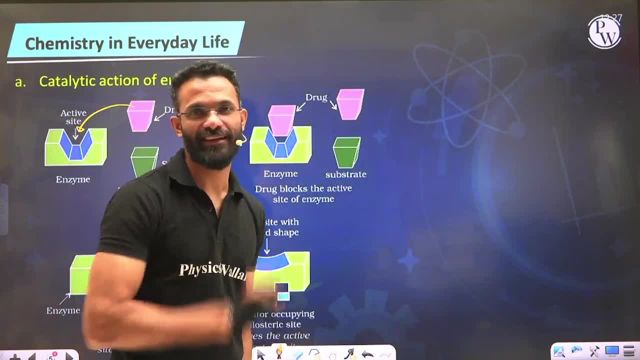 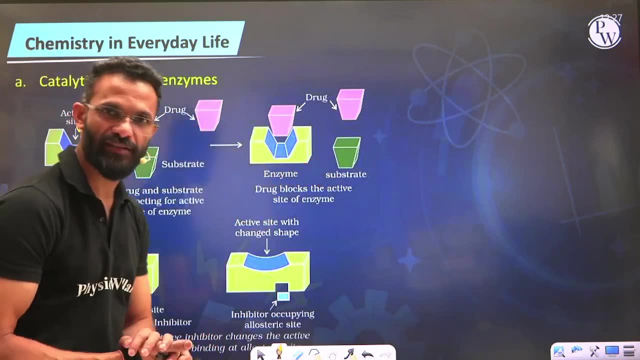 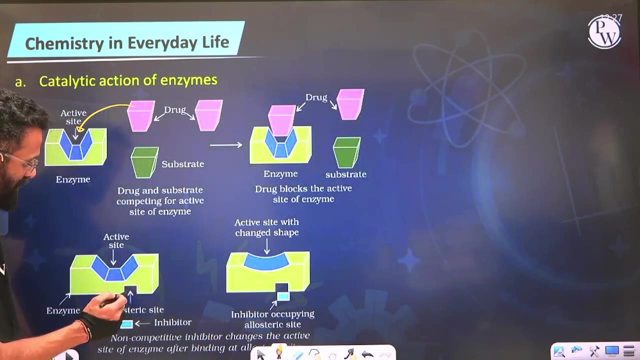 one of the type of interaction of a drug with the enzyme. now see, not always the drug directly compete with the substrate and get a commodited in the active site. sometime those drugs get accommodated in some other part of find them. you see, here let's say there is one more part. 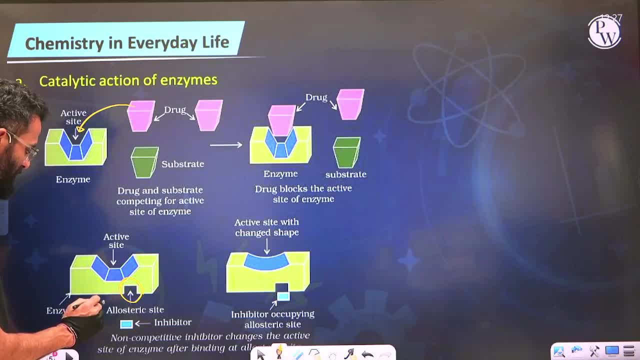 in the enzyme, which we are calling it as allosteric site. this is allosteric side, let's see. so now we ate some drug or a medicine, that medicine got a commodity in this allosteric said not at the active side, but when thisuchi we eat it out. this is all n timeframe and that was the thousand lifetime cycles that was so wht. this is the story lately in our curious your questions. 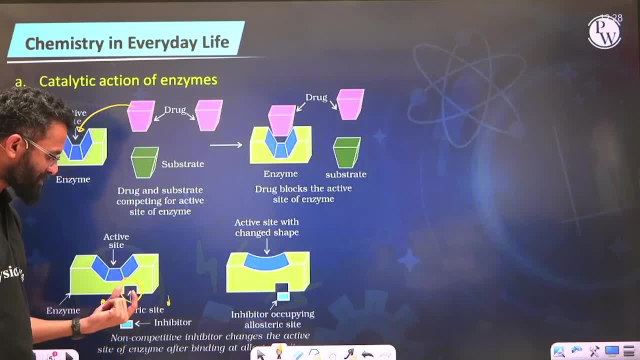 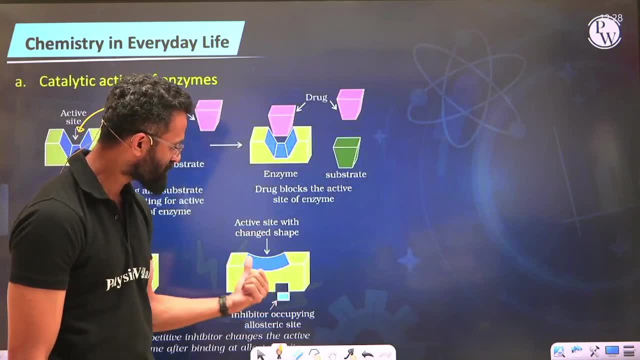 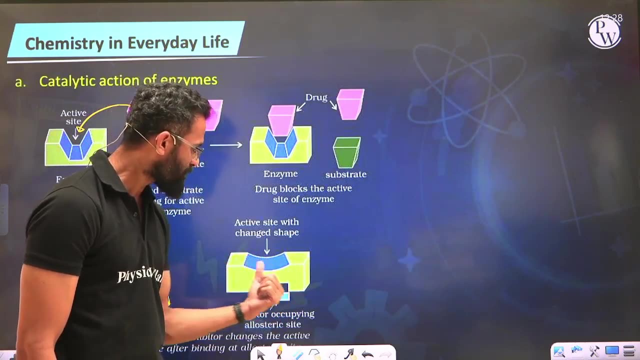 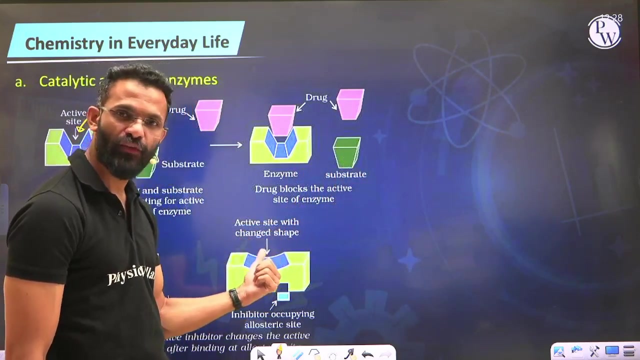 But when this medicine gets attached or gets accommodated in the allosteric site, it changes the shape of active site. You see, the shape of active site has changed because now drug has been accommodated in the allosteric site. If the shape of active site has changed then even if substrate is available, this substrate will not be able to fit into this active site because the shape of active site has changed altogether. 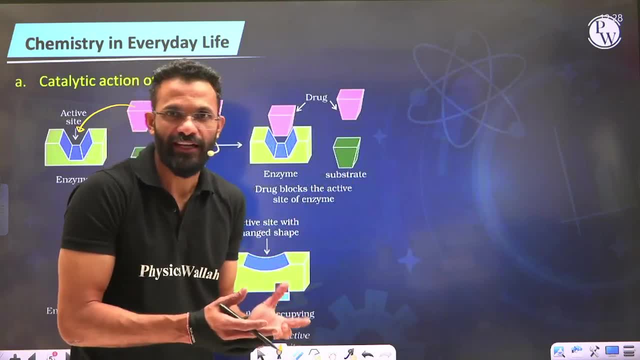 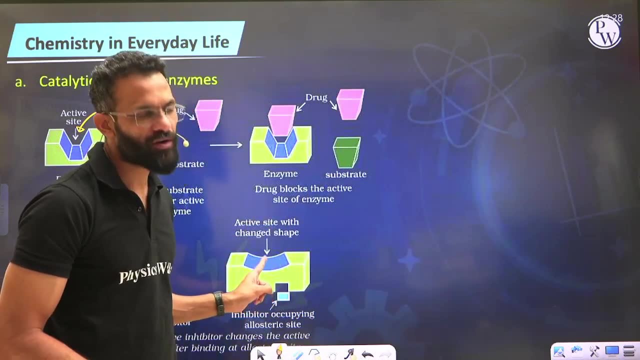 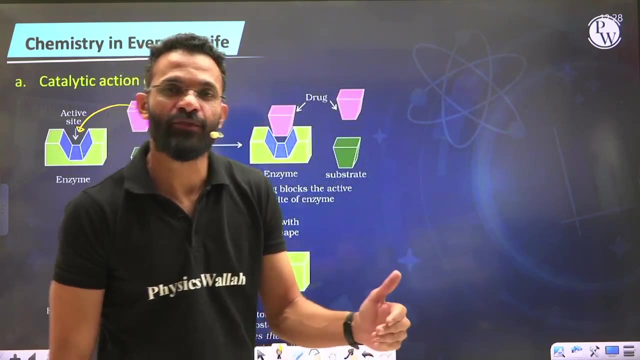 So this cannot fit in here just like lock and key, As a result of which there is no deposition of substrate anymore taking place on the cavity or on the active site of enzyme, So no further catalytic reaction can take place. That's how the catalytic reaction have been inhibited. 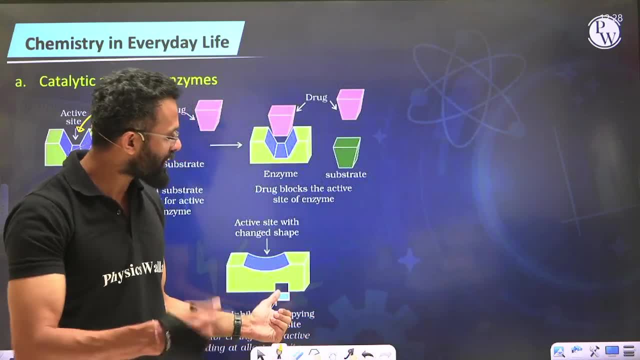 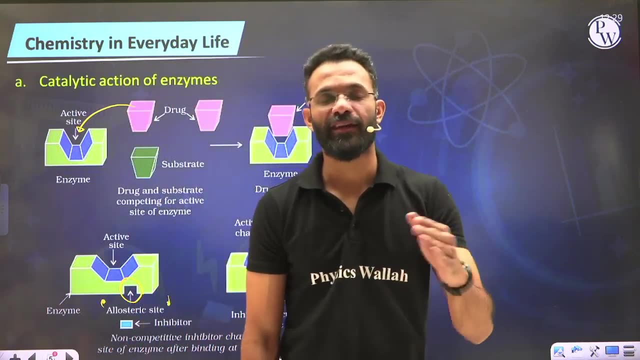 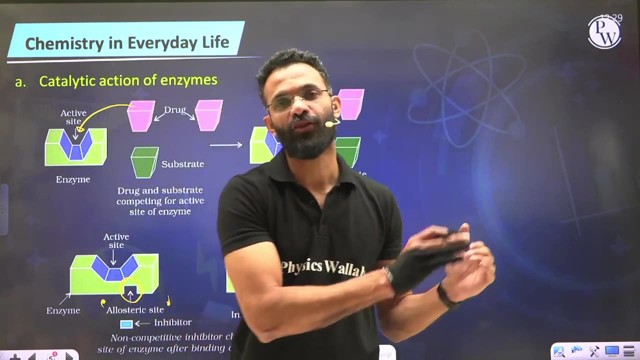 But in this inhibition drug is not directly competing with the substrate. So such kind of drugs, or the medicine, we call it as non-compatible Competitive inhibitors. So, guys, those medicines which prevents the catalytic action of enzymes are of two types. 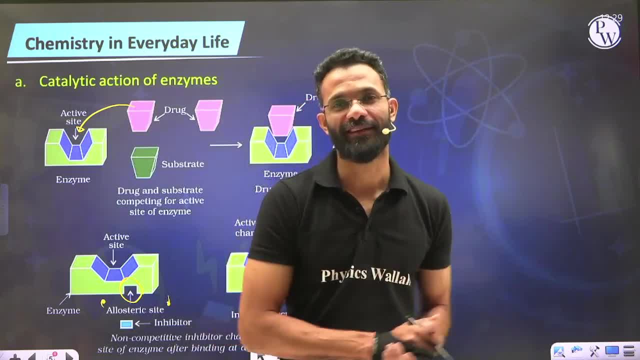 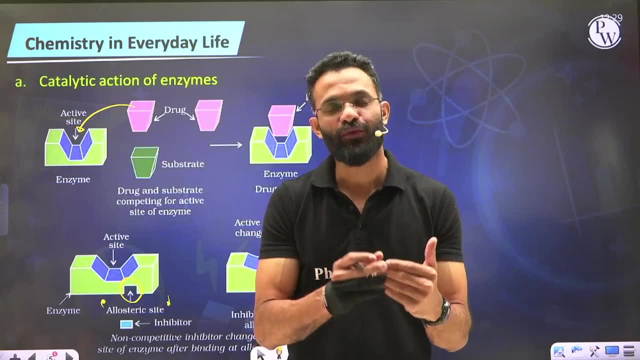 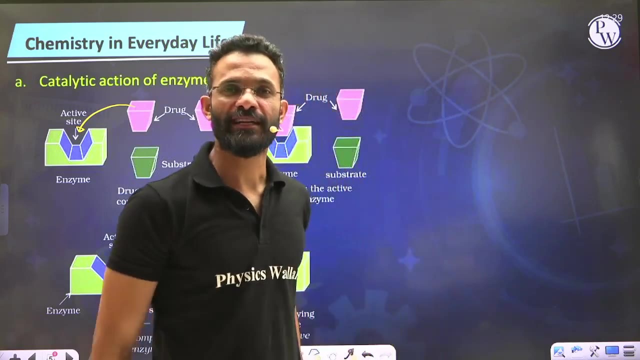 Competitive inhibitors and non-competitive inhibitors. So this was first interaction of medicines or the drugs with the enzyme, which are nothing but macromolecule. We call them as molecular targets, Just like enzyme, Like we said, the second macromolecule which we are going to learn. 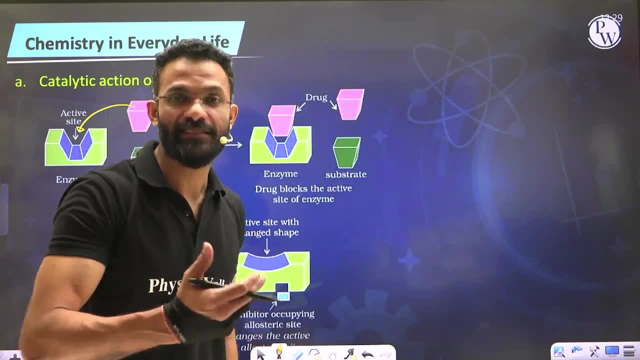 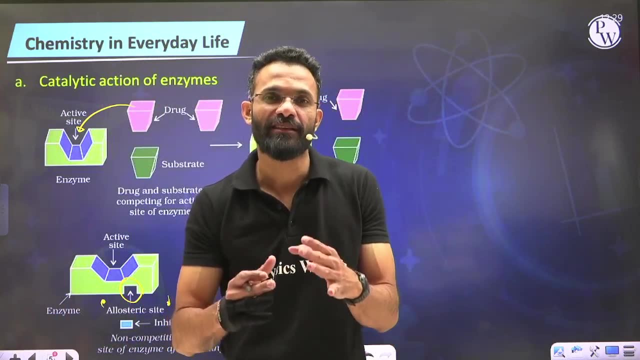 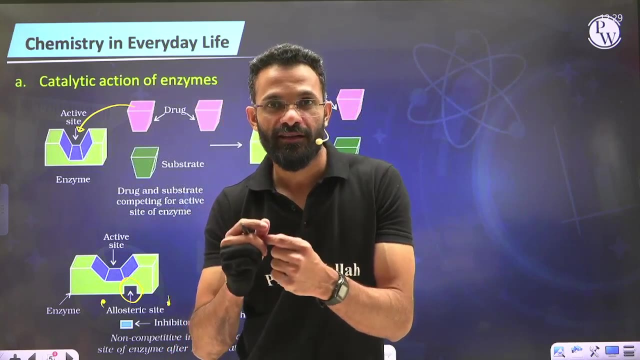 And we are going to learn its interaction with the drug is a receptor. Receptor are again, those protein molecules which are essential for body's communication process. Like I give you an example: If at some part of your body you got hurt, then you start experiencing pain. 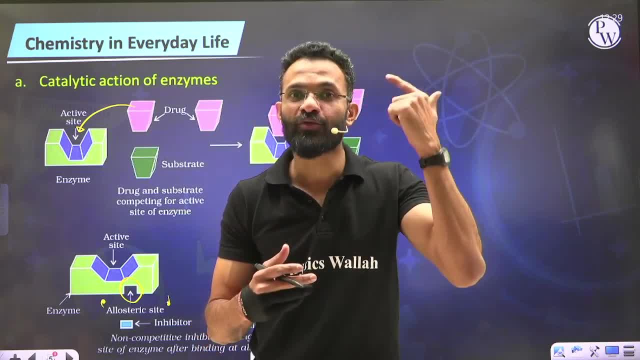 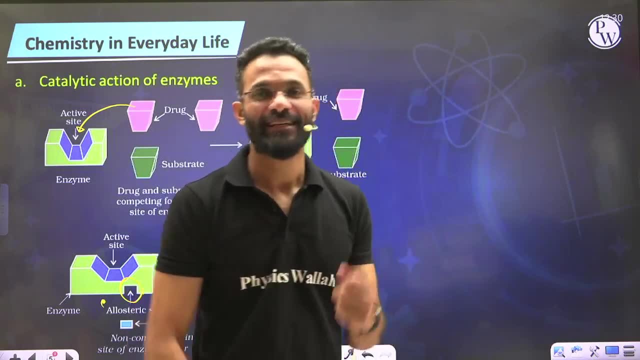 But who tells you that you are experiencing pain? How your brain come to know that you are experiencing pain is through the receptor and its interaction with the chemical substances. So, guys, let's try and understand first the functioning of receptor. Okay, so now what we are talking. 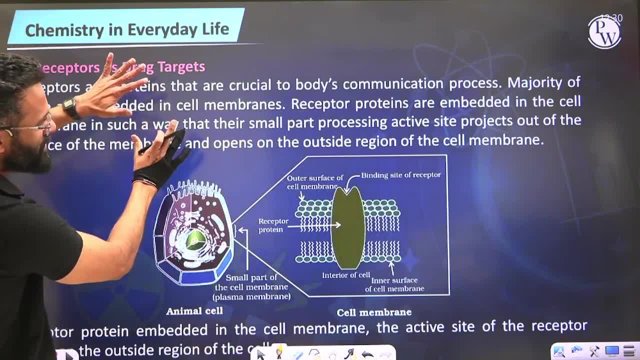 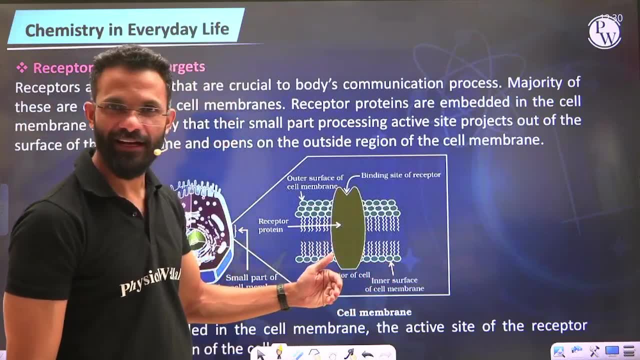 Receptor as a drug target. Let us read this basic information first to understand. You are absolutely not required to remember this diagram, but for understanding how the receptor communicate with the body, it is important for us to see at least the required part of it. 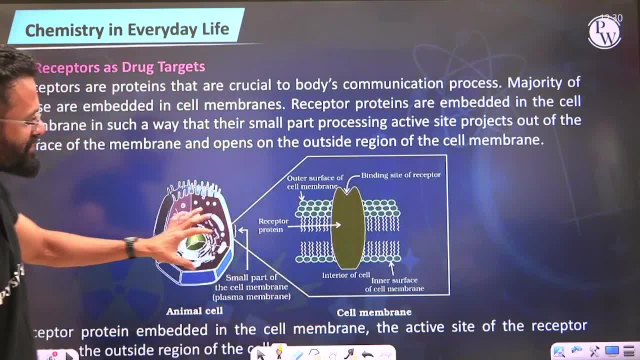 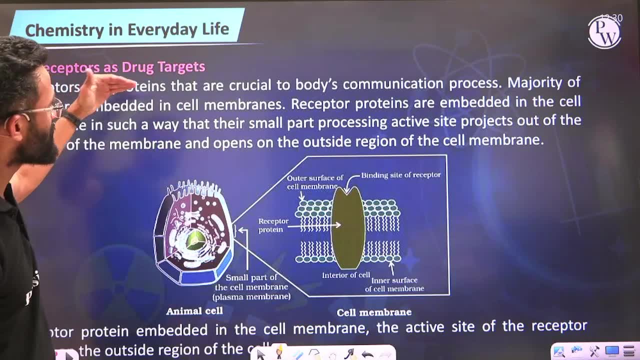 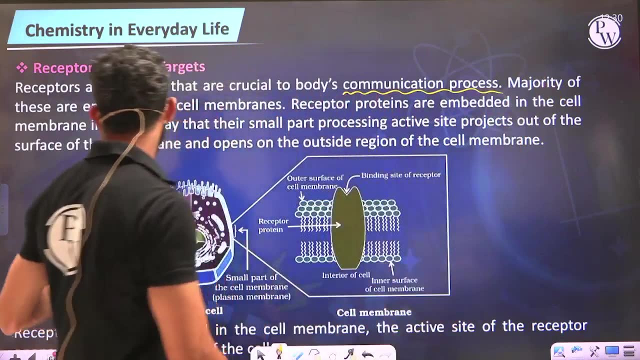 So what is this? This is basically animal cell, and this is the Magnified image of a cell membrane. Let's come here. Receptors are protein that are crucial for body's communication process. Majority of these are embedded in the cell membranes. 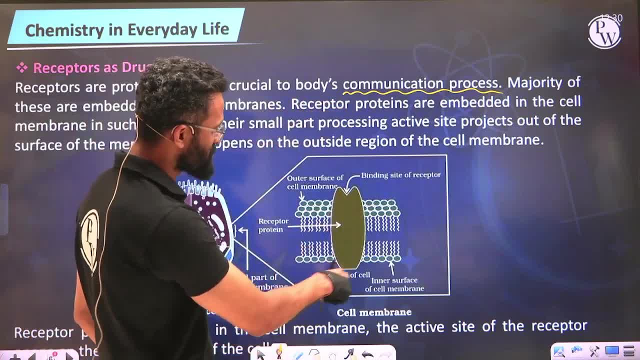 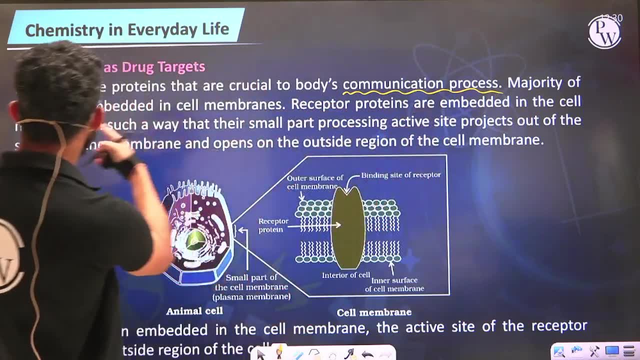 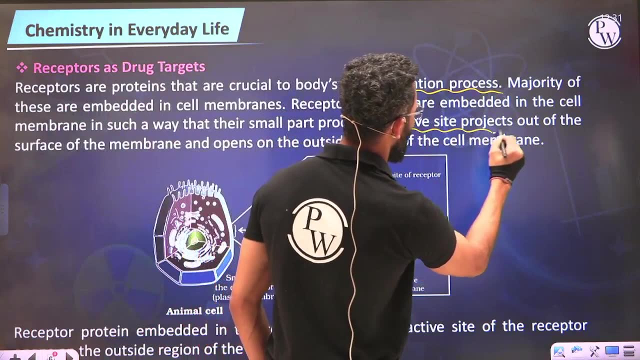 Receptor proteins. you can see now, This is basically your internal cell. So receptor proteins are embedded in the cell membrane in such a way that their small parts possessing active site project out of the cell membrane, Project out of the surface of cell membrane. 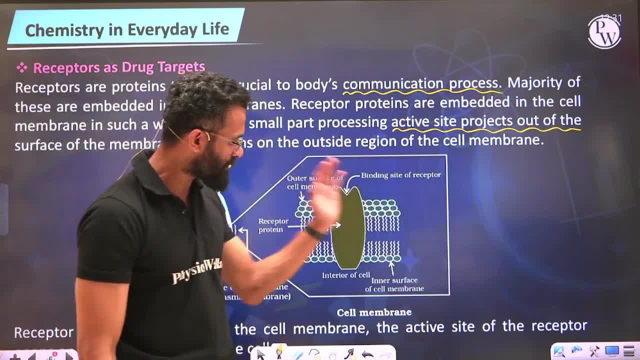 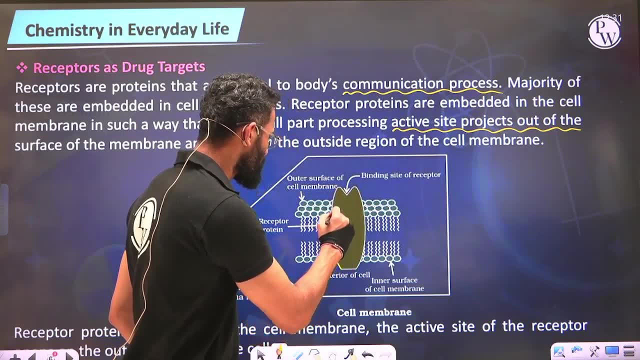 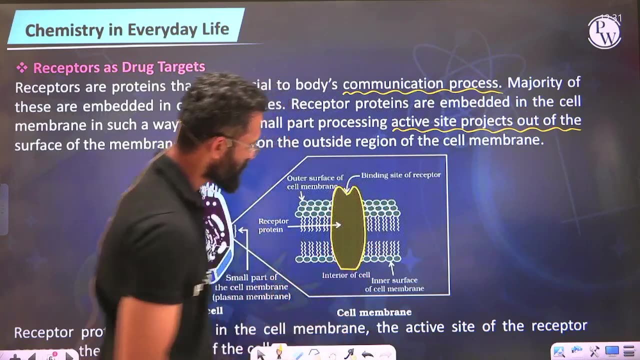 So, guys, in this animal cell, if this is the diagrammatic representation of cell membrane, this shape that you see here, this one Is basically that protein which we're calling it as a receptor. so you will see, Receptor is actually embedded in the cell membrane. but 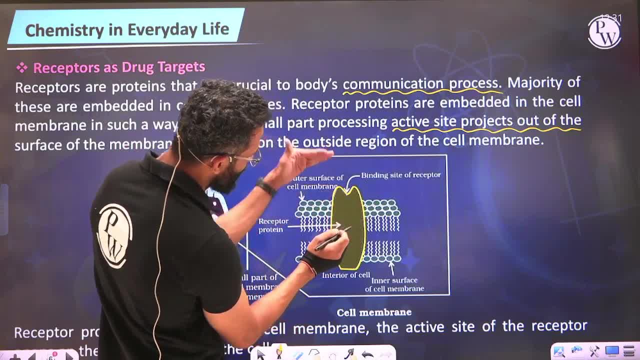 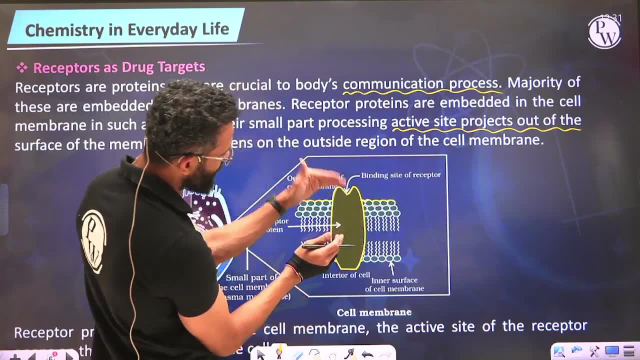 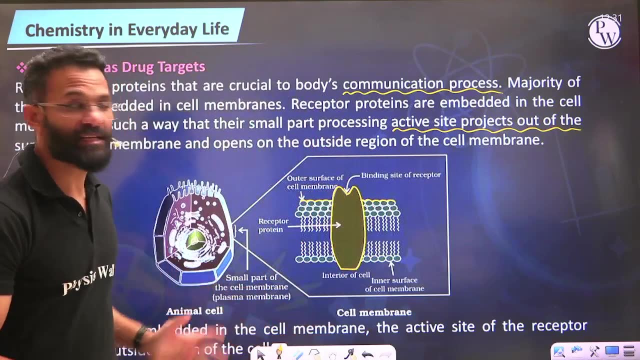 Some part- part we are talking about, this part is projecting outside the cell membrane. you see, so this part is projecting outside the cell membrane and this is what we call it as active site. okay, now what happens basically is in our body. there are some chemical substances which 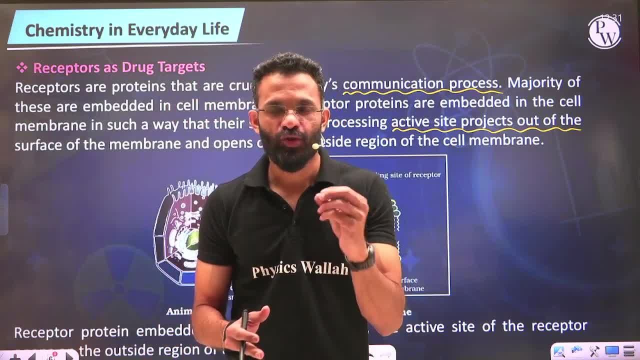 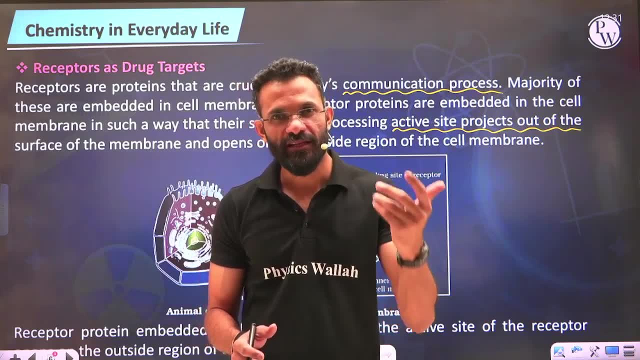 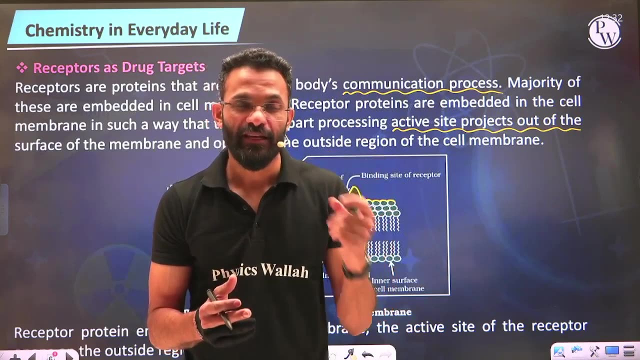 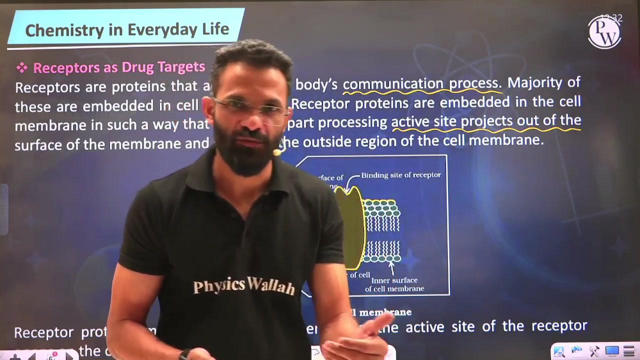 are secreted by the body itself and those chemical substances are responsible for communicating between two neurons or from neuron to muscle. those chemical substances which communicates in our body or sends a signal to our brain is what you call it as chemical messenger. but how does this chemical messenger actually passes the signal to our body to understand that? 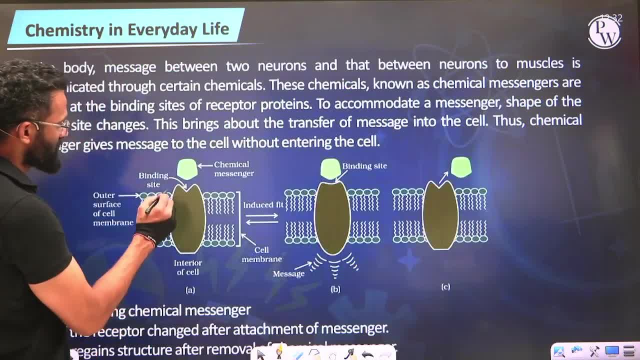 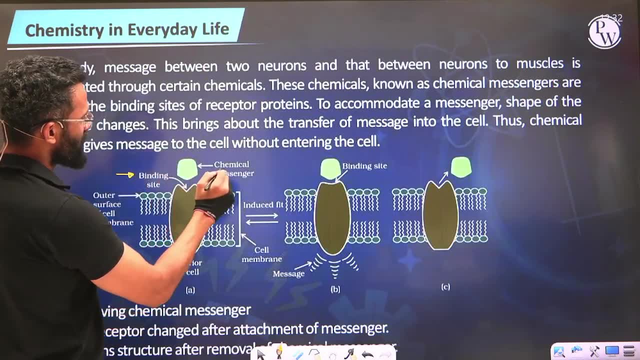 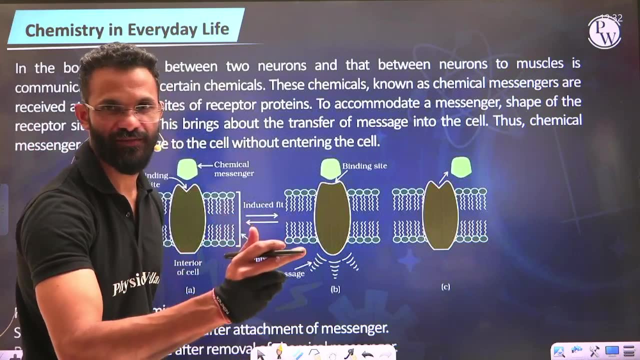 let's see the next diagrammatic representation. so this is the active site, this active side, or you can also call it as binding side. this is what you call it as chemical messenger. the chemical substances which is responsible for transferring the message is what you call it as. 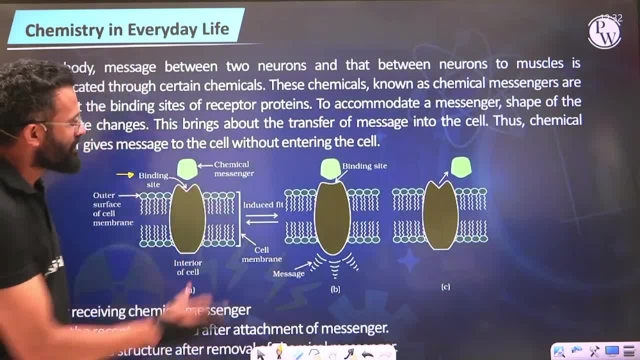 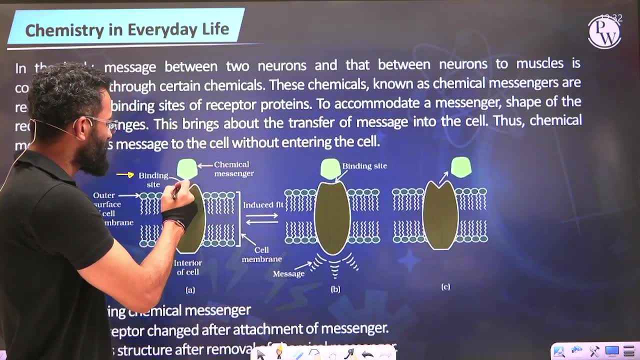 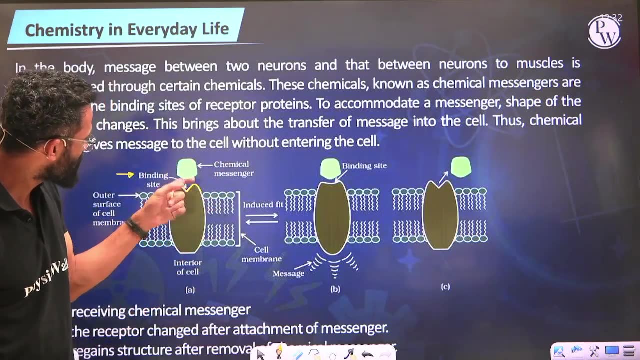 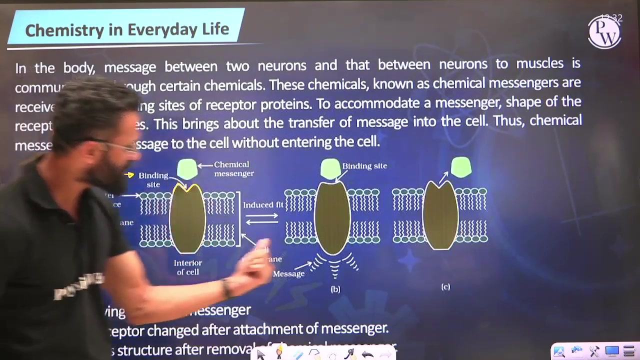 chemical messenger. so see what has happened. a chemical messenger or a chemical substance which is secreted in the body itself get attached to the active site of receptor when itself get attached to the active site of receptor. in order to accommodate this chemical messenger, the receptor initial state of the cell has been changing its shape. now the 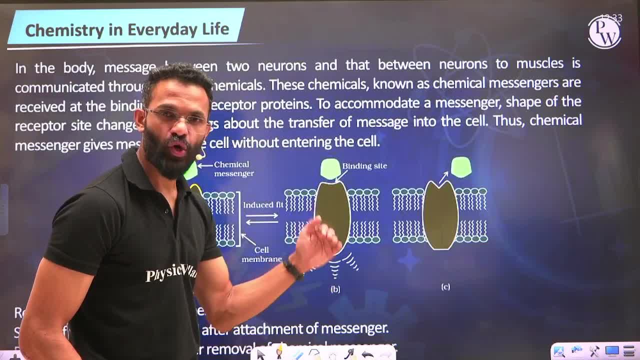 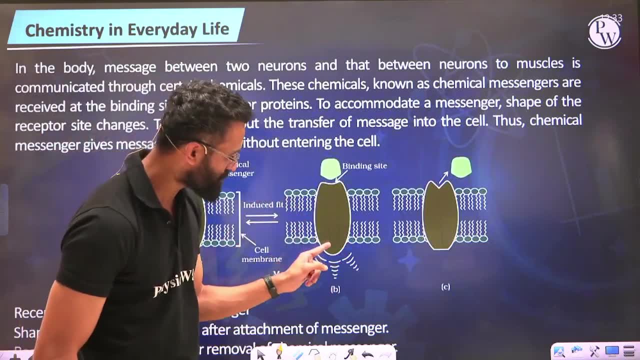 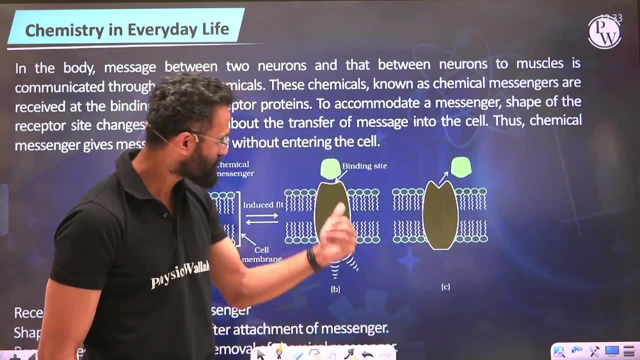 chemical messenger itself has been turned on again to the active site of the chemical messenger. this cell changes its shape. you see that not cell, this receptor is changing its shape. so in order to accommodate the chemical messenger, the receptor protein is changing its shape. so change in the shape of the receptor protein. 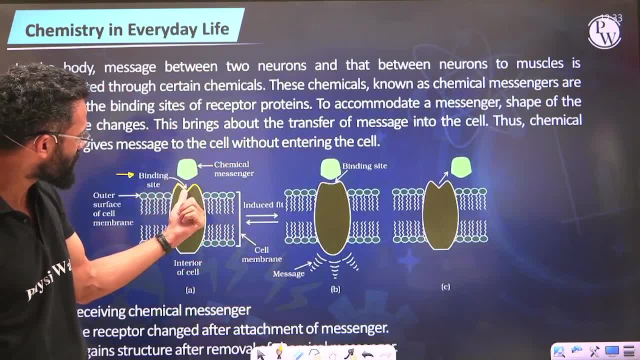 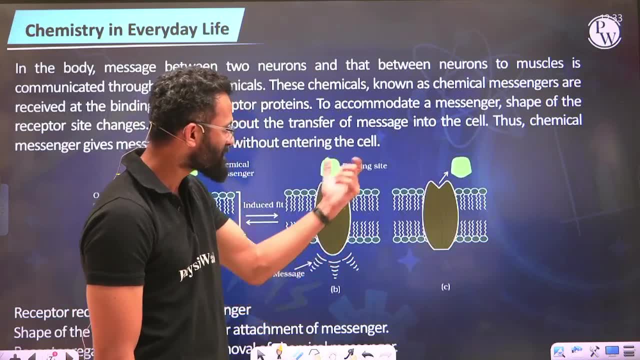 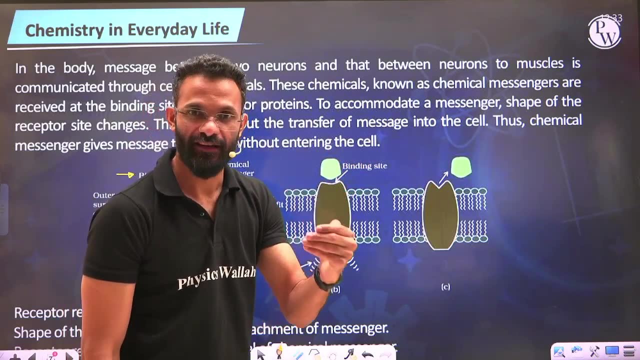 got attached to the active site of the receptor protein and it has changed its shape. so the change in the shape itself is the signal given to the cell that some chemical messenger has conveyed some message to the body. so a message is conveyed to the cell without actually interacting with the cell, see the 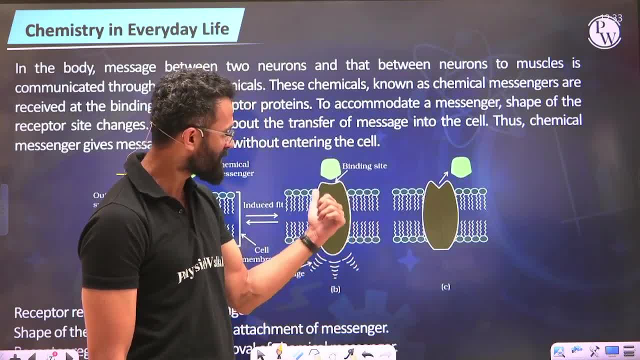 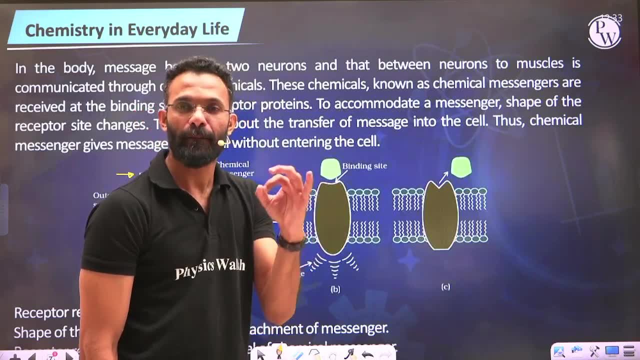 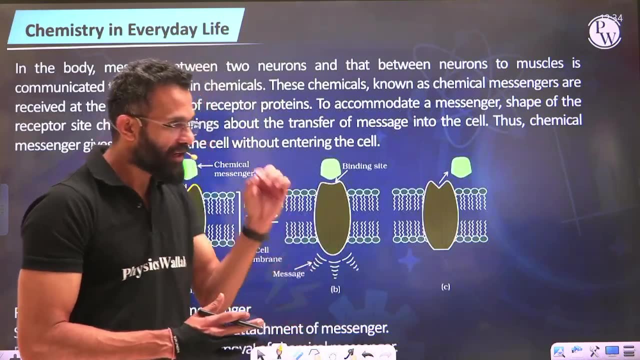 chemical messenger has not interacted with the cell. it has just interacted with the receptor protein. but change in the shape of receptor protein itself is an indication that some message has been conveyed. so you will find there are several such receptor protein present in our body and every particular chemical. 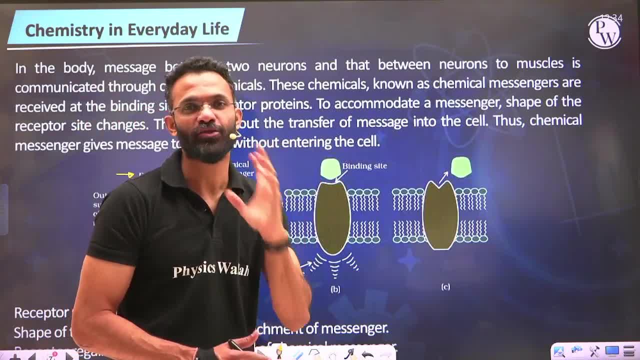 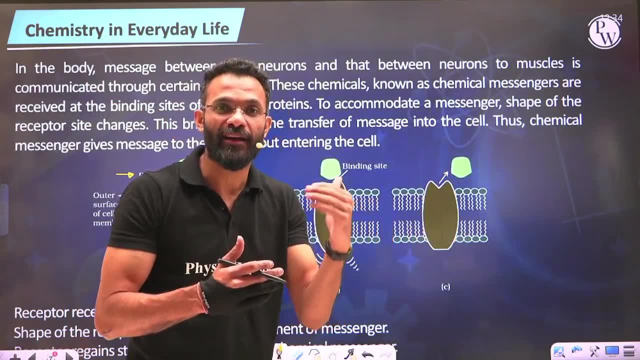 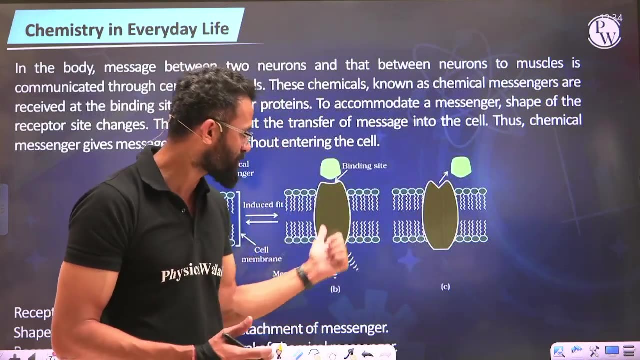 messenger has a specificity to attach to particular receptor. that's why the difference, different kind of signals which are given to our brain are conveyed by the different type of chemical messenger which attaches to the different type of chemical messenger, which attaches to the different type of different or the specific type of receptor protein. so that's how the 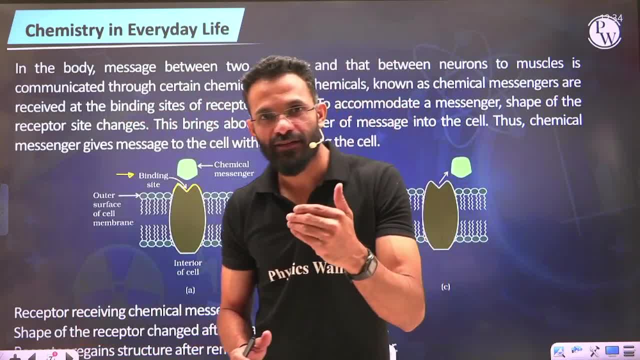 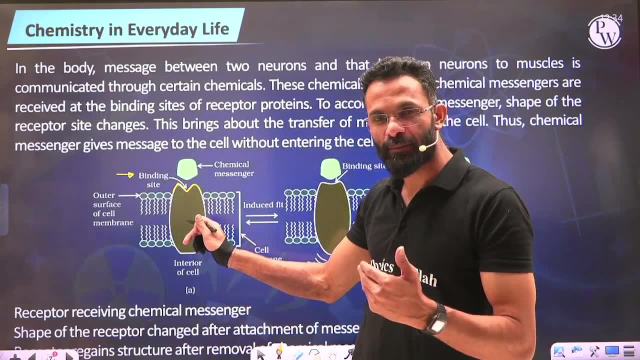 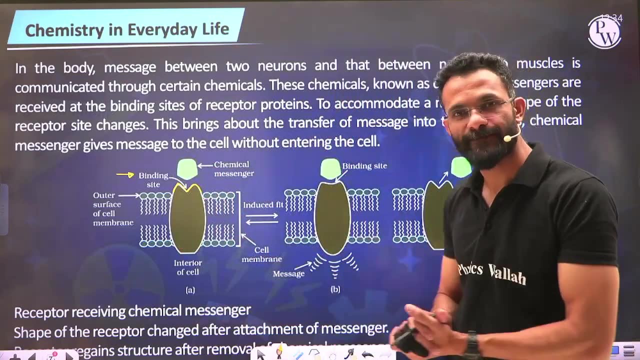 communication or the signals are sent to our brain by the interaction between chemical messenger and the receptor protein, and this is basically, and this is basically taking place because of change in the shape of receptor protein. all right, now we'll have to understand from where does drugs are coming into picture, or how medicines 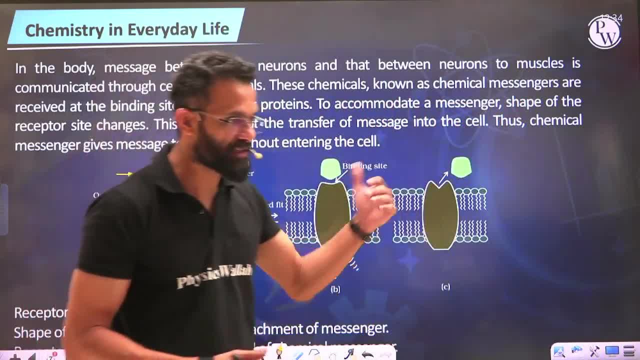 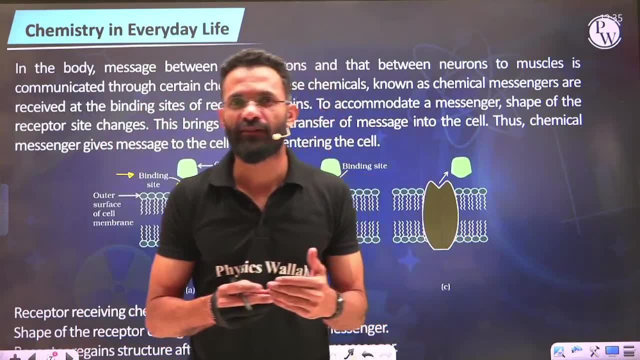 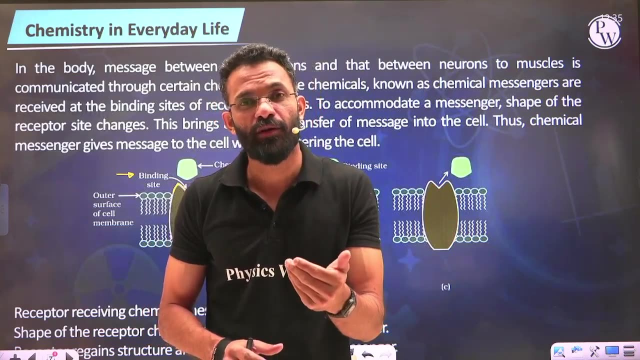 are going to interact with this receptor protein. well, we'll be taking two examples. okay, again, whatever example I'm giving you, this example probably we'll have to consider just for the sake of understanding of concept. biologically it need not be exactly correct one, all right, well guys. 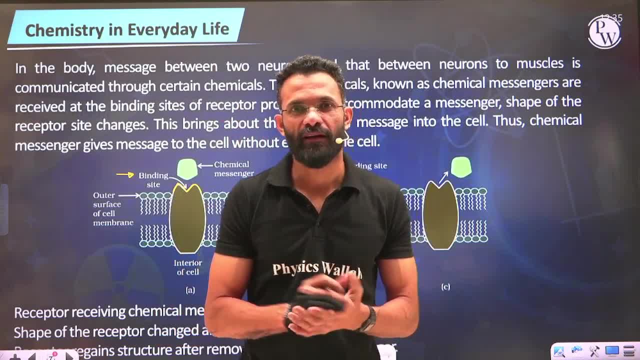 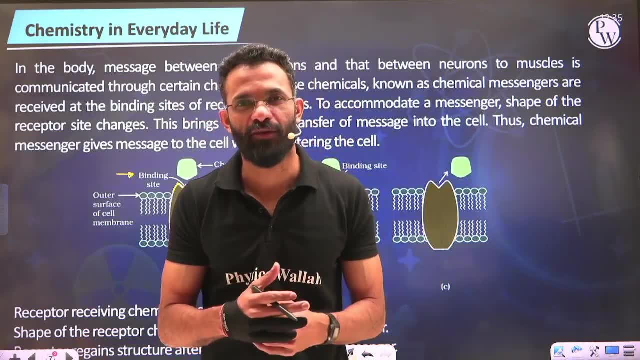 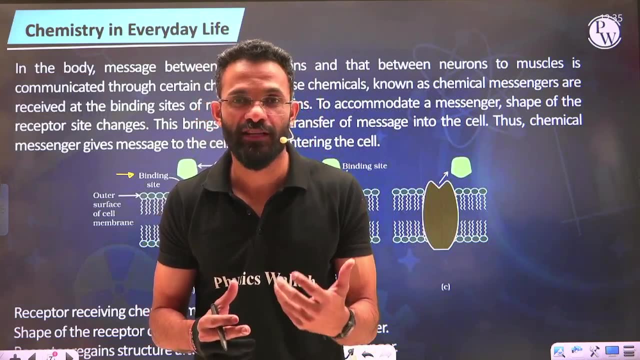 we all are aware that, uh, uh, when we experience or when we feel good for ourself, there is some hormonal play that is taking place in a body. those hormones basically make us feel good, or they give us feeling of well-being, or those are the one which are responsible for keeping our good mood intact. right now let's see. 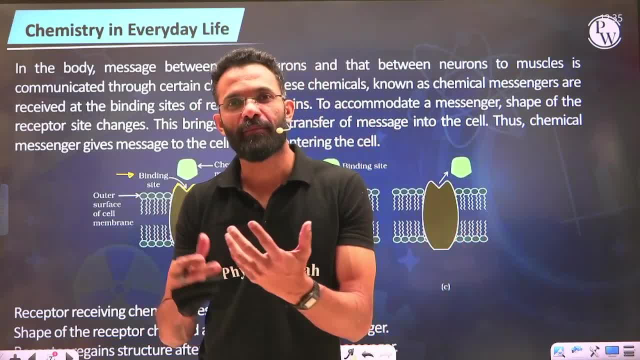 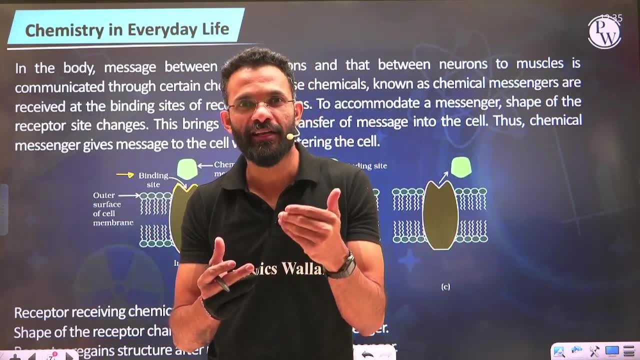 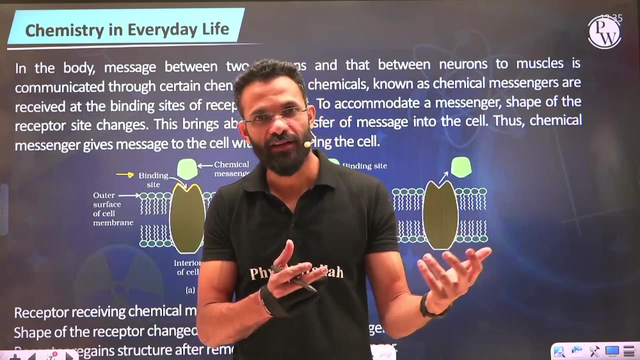 because of some mishappening that is happening in her life. probably that particular person is now no more feeling you know well-being. he started experiencing some stress, some Probably he is undergoing some kind of depression. So he goes to the doctor and doctor prescribes some medicine. 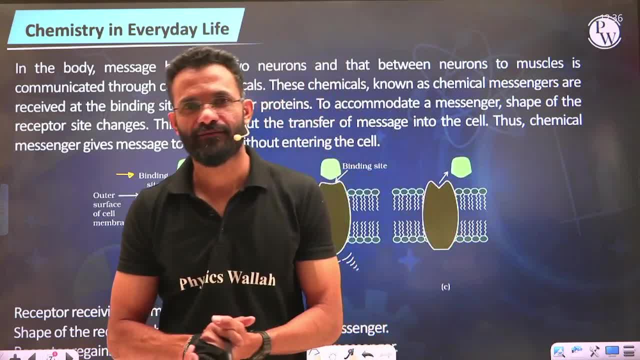 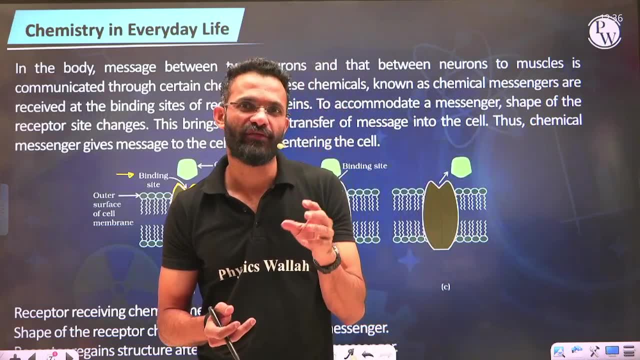 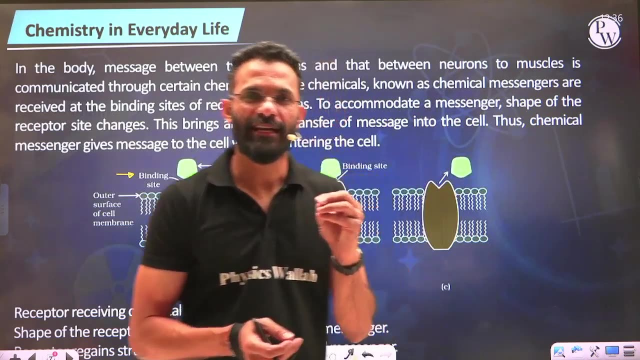 Probably tranquilizer, or probably some anti-depressant drugs or those kind of medicine or stress related medicine. He eats those medicine and he starts feeling better. Now, what exactly is happening here? Look, when our body started experiencing not being well? it is probably because 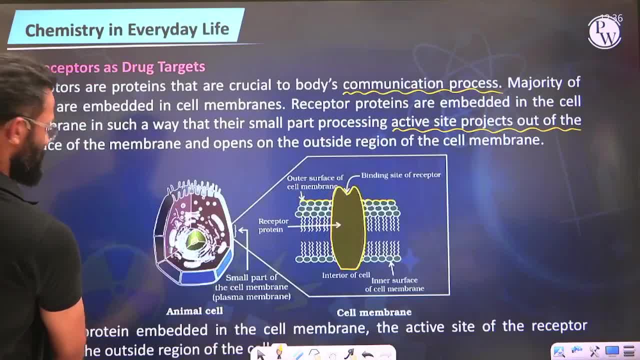 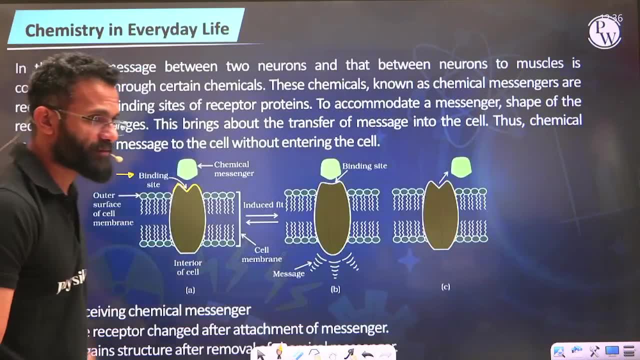 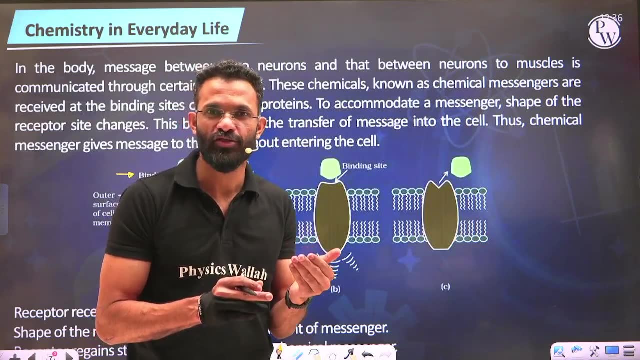 Hold on everyone. Yeah, Guys, hold on All right. So what I said? there are some hormones, basically, which are secreted in the body, and those are the ones which are responsible for making us feel good Right Now. what happens? 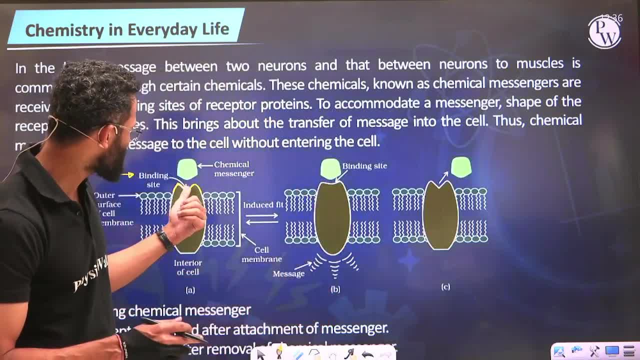 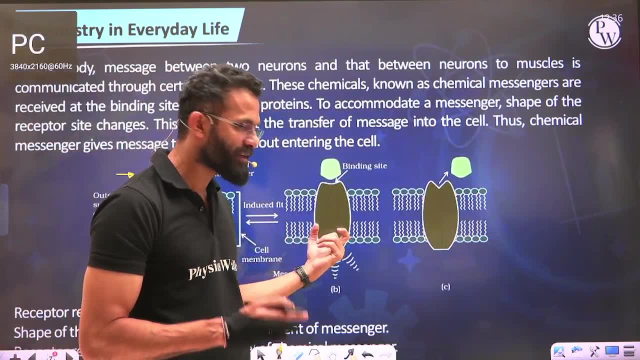 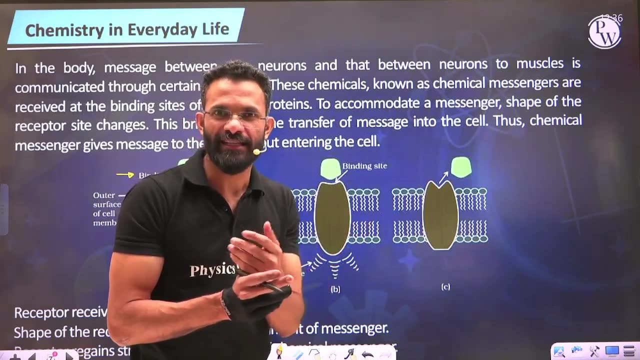 Those hormones or the chemical substances gets deposited at the active site of receptor and then the shape of receptor has been changed and the change in the shape is signaling your body that you are feeling good. So you are in a good mood Right Now. let's say, because of something like I said, you started feeling. 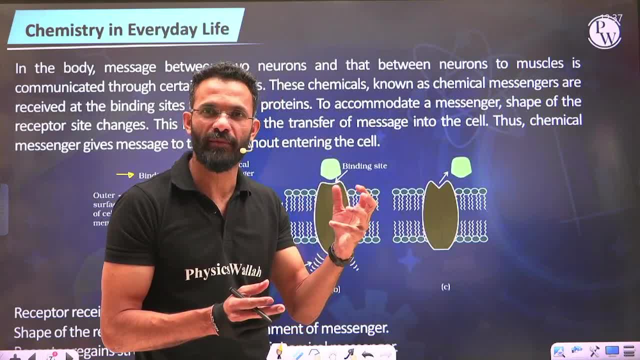 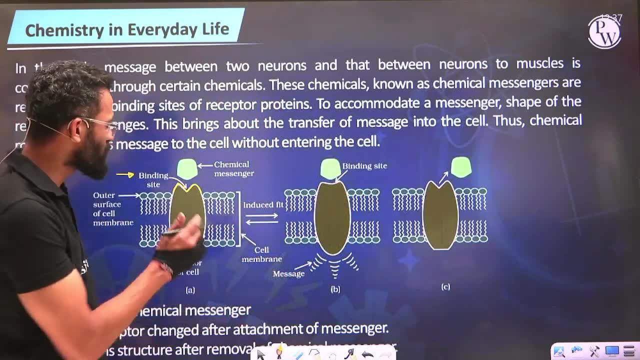 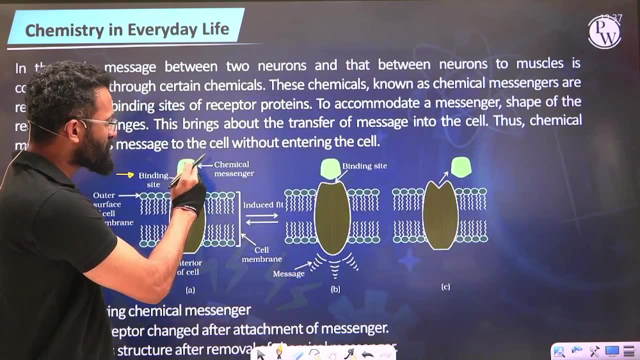 You started experiencing the depression. So doctor gave us some medicine- Now the medicine that is being taken Here everyone- When you started experiencing depression, which means Those chemical messenger or the chemical substances which were getting secreted in the body, those concentration or the secretion amount have been decreased in the body. 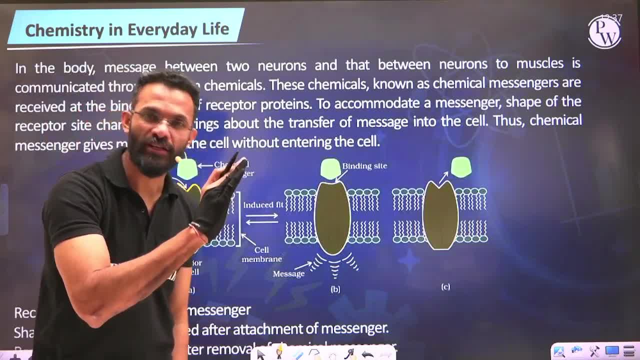 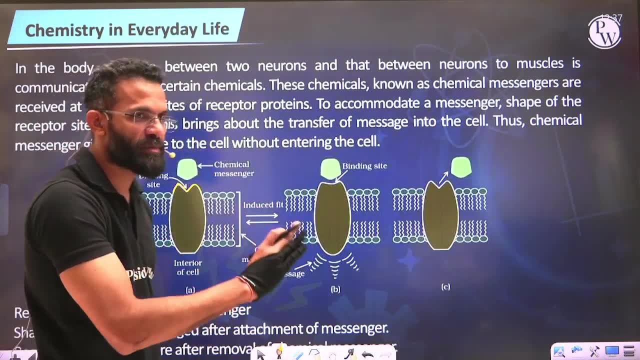 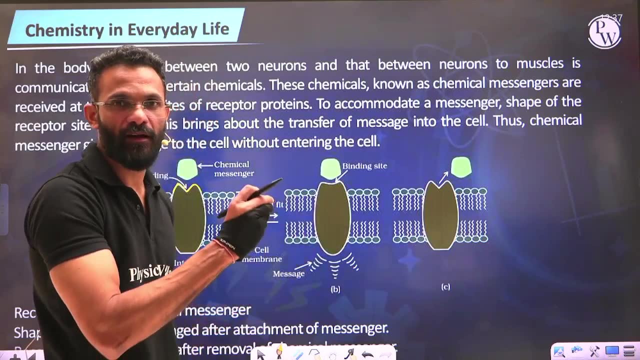 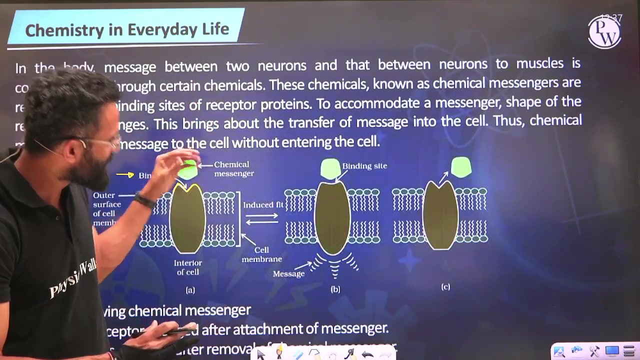 Because of decrease in the concentration of those happy hormones have been decreased, your body is no more experiencing or no more having that feeling of well-being. So the whole reason why you are not experiencing happy is basically because Those chemical substances which were responsible for signaling your body that you are experiencing or you are feeling good have been decreased. 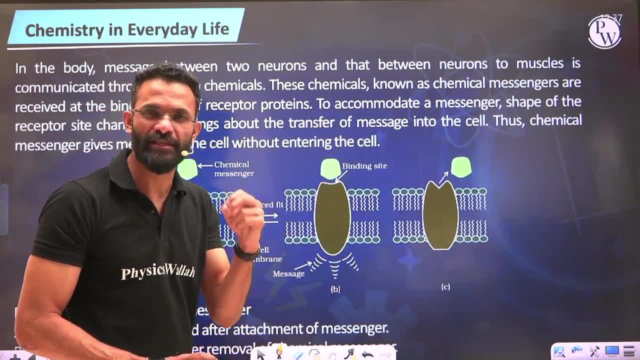 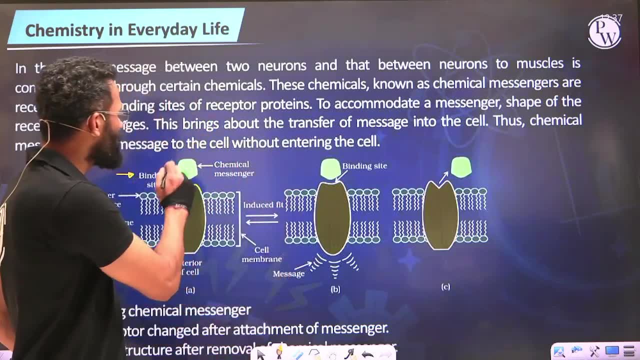 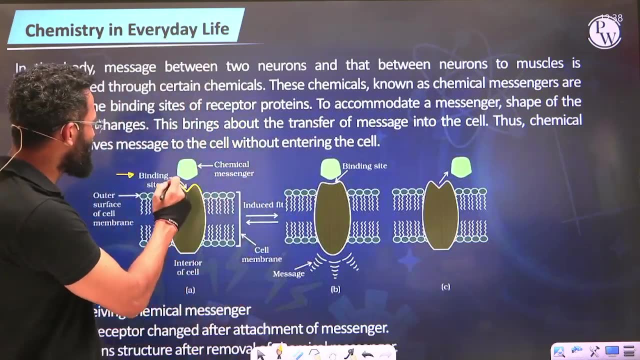 Now, the medicine that we are eating or medicine which are prescribed by the doctor, are those medicine which are going to copy or mimic the same chemical messenger which were responsible for making you feel good. So now those medicine themselves will get attached to the active site of this receptor. 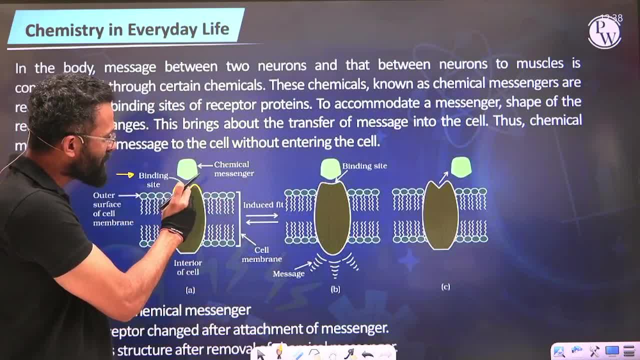 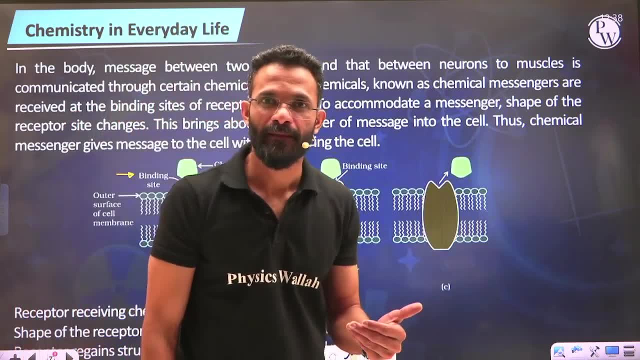 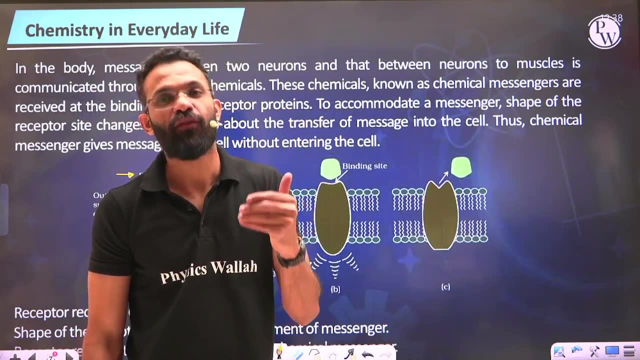 The receptor protein and it will exactly mimic the same role as it was done by the original chemical messenger. So you again start feeling good. So these kind of medicines or the drugs which basically copies the function of those chemical messengers, we call them as agonist. 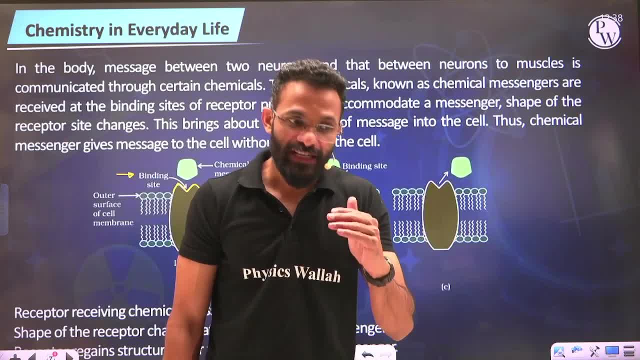 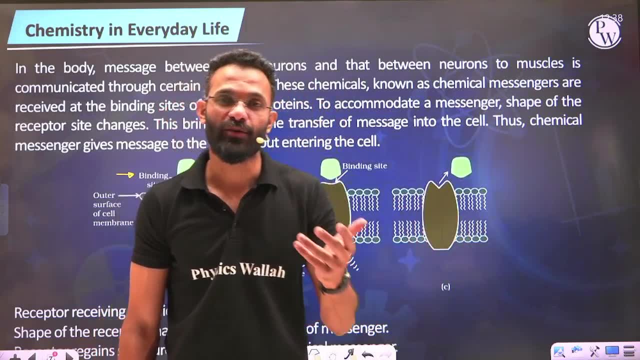 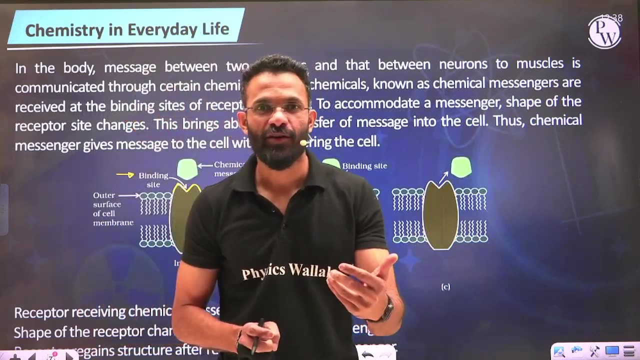 We call them as agonist. Now let's take another type of or take another example Which explains the. This is the type of drug which we call it as antagonist. What are agonist? Agonist are basically those medicines which are going to mimic or copy the function of some chemical messengers. 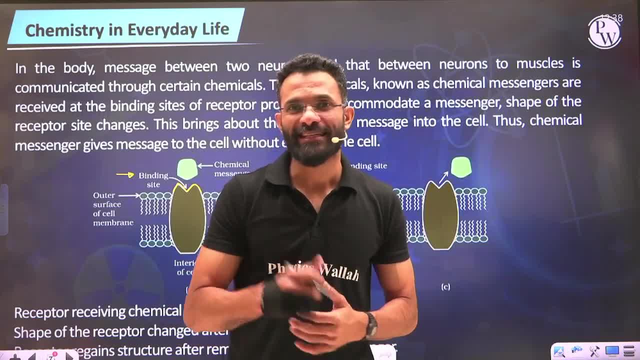 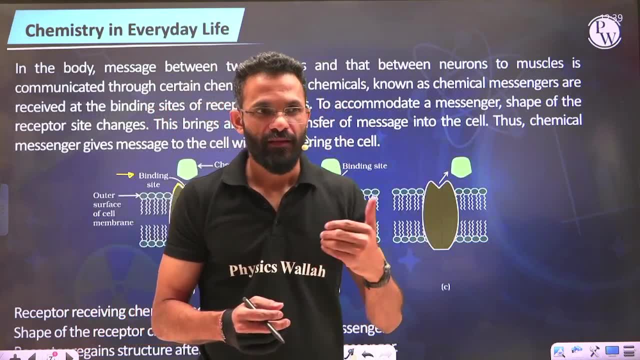 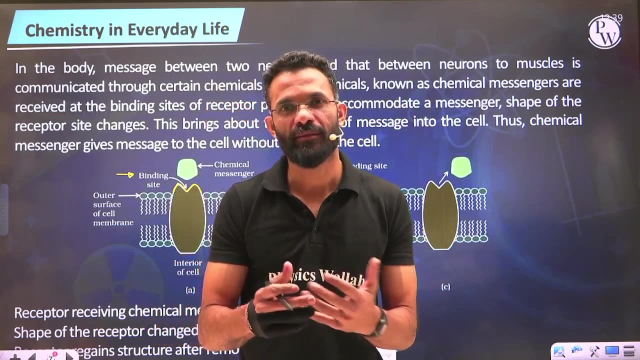 Now let's understand antagonist Well. now, like I said, because of some injury, if person start experiencing unbearable pain, then let's say, if person has met with some accident and he is, he has got some injury. Now that injury can only be treated by operation. let's say: 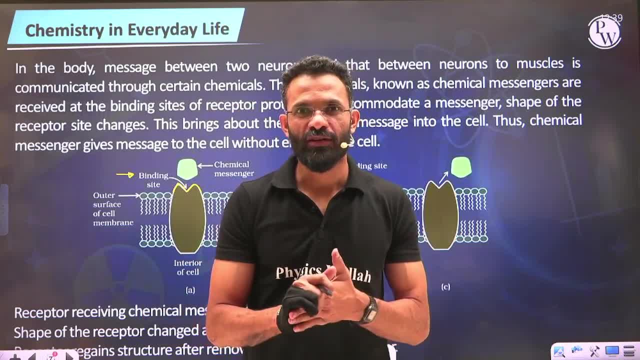 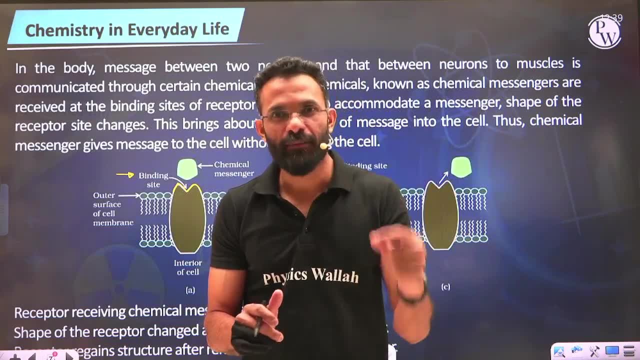 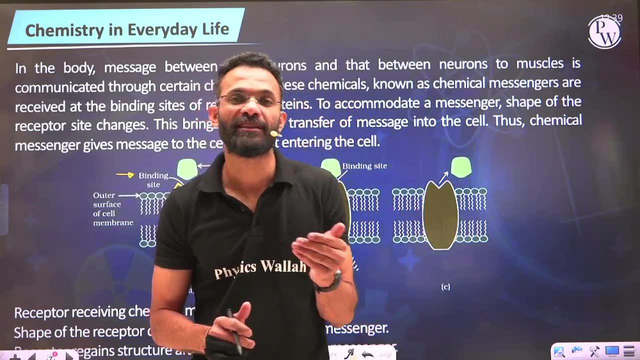 So he goes to the doctor. Now the first thing doctor do is if the pain that person is experiencing is unbearable, doctor first give anesthesia to that part of a body which is to be operated Right. The moment doctor gives anesthesia, that person no more experiences that pain. 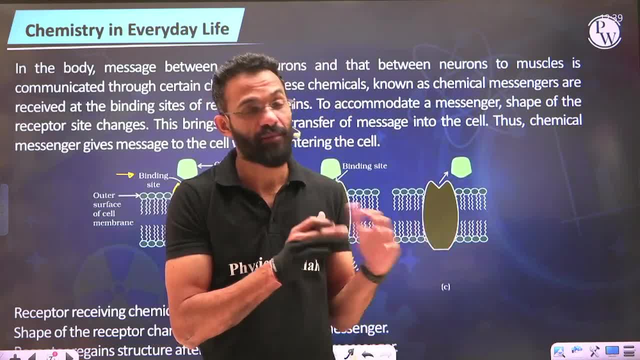 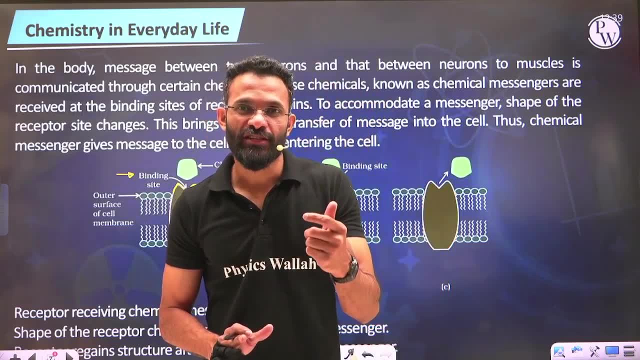 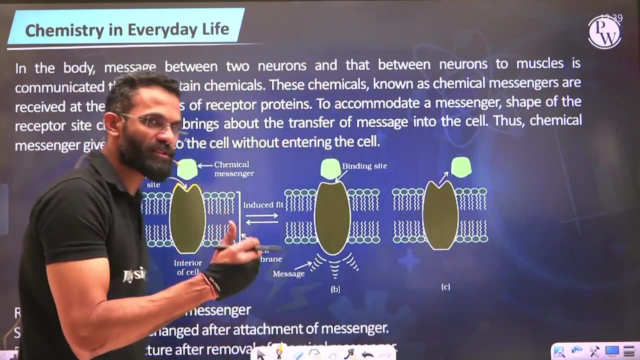 Again the example I am giving you just for the sake of understanding the concept. it need not be biologically absolutely correct. Okay, Now the moment doctor gives anesthesia, that person no more experience that pain. So let's say the pain that person was earlier experiencing was because of some chemical messengers. 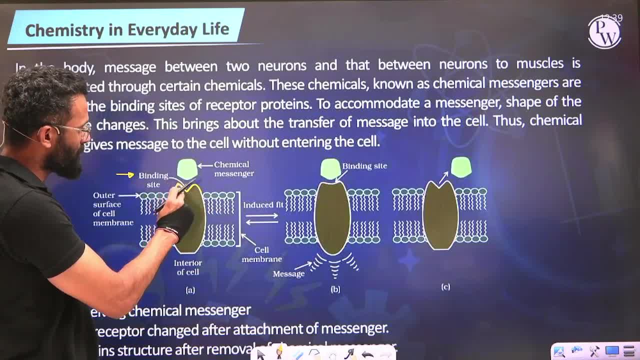 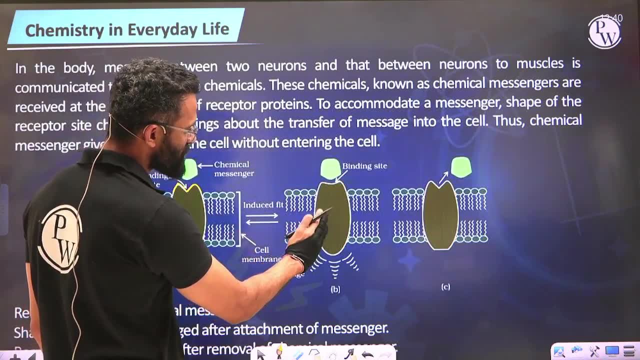 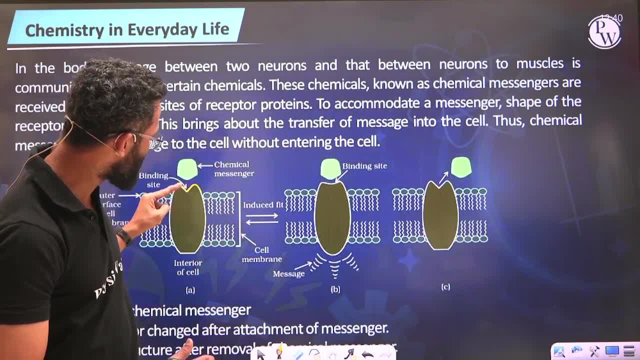 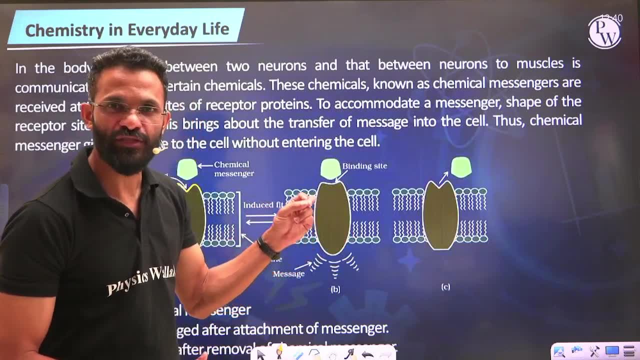 Now, the moment doctor gives anesthesia, that person no more experiences that pain. Now, the moment doctor gives anesthesia, that person no more experiences that pain. chemical messenger: if get attached to this receptor protein, they are going to signal to the body about the pain or the inflammation. so the medicine which was given by the doctor, let's say: 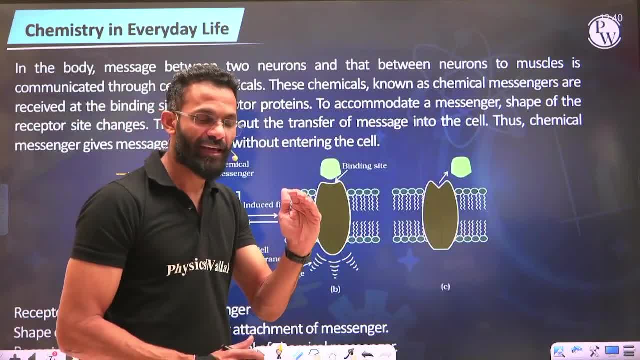 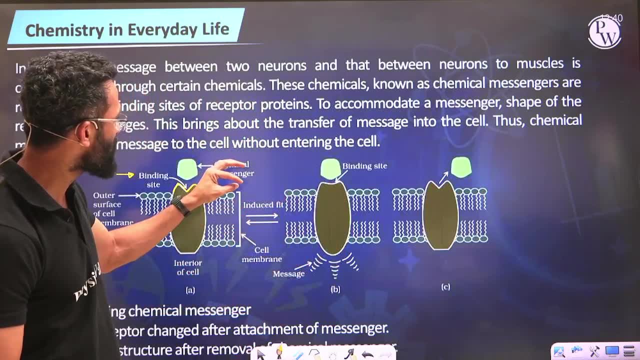 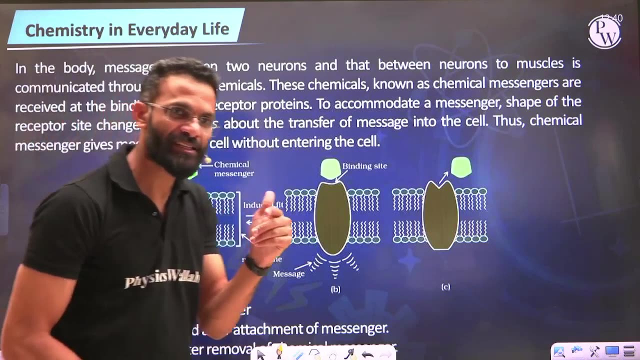 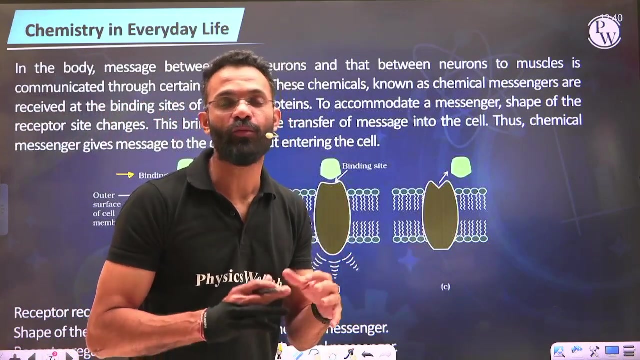 anesthesia. so let's say anesthesia is external chemical messenger that we have injected in the body, so that anesthesia will now compete with the chemical messenger and itself will get attached to this binding site. but because the anesthesia which is given is not communicating a message of inflammation in the body, our body no more experiences that inflammation. so now what? 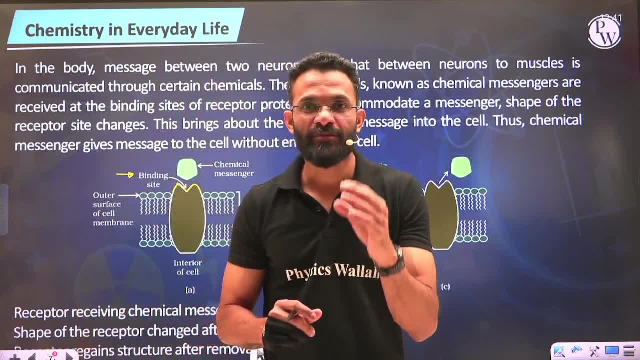 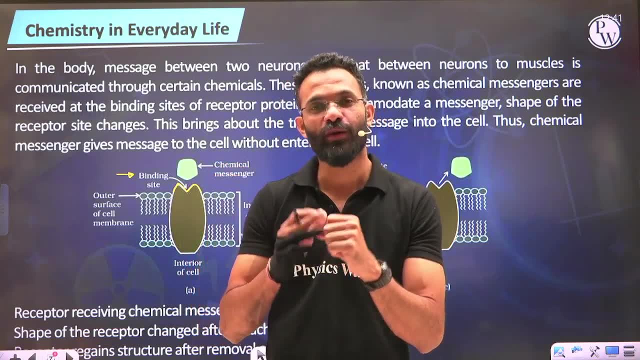 anesthesia has done is: anesthesia has prevented or inhibited the activity of chemical messenger, because of which we are not going to experience that unbearable pain. so such chemical substances, which are not going to be able to be used in the body, are not going to be used in the body. 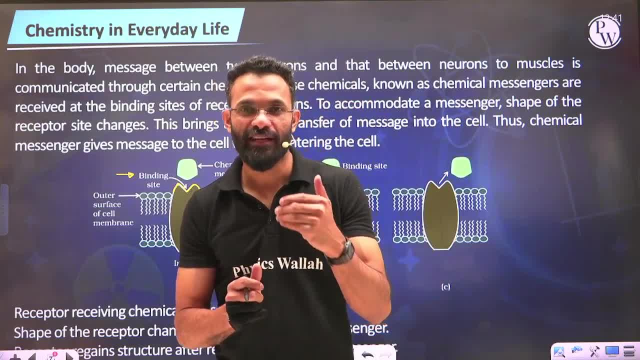 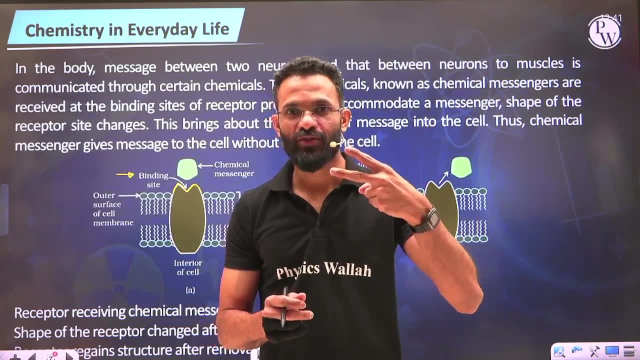 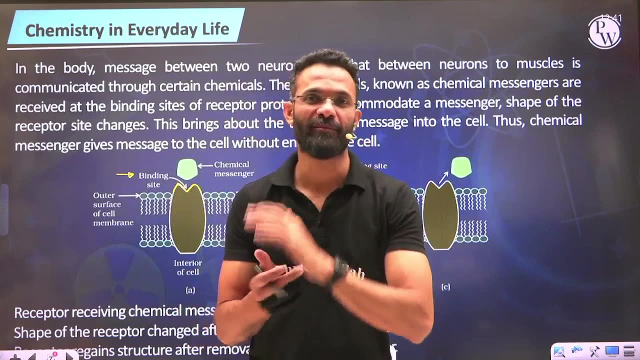 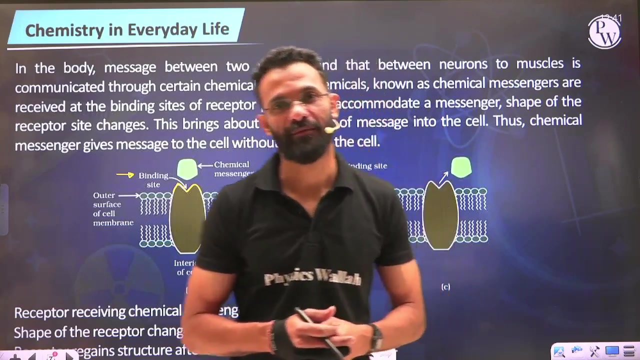 which inhibits the activity, which inhibits the activity of chemical messenger, are what you call it as antagonist. so there are two types of medicines that we studied here: one, agonist, which mimic or copy the action of chemical messenger, and second is antagonist, which basically opposes or inhibits the activity of chemical messenger. we call them as antagonist. 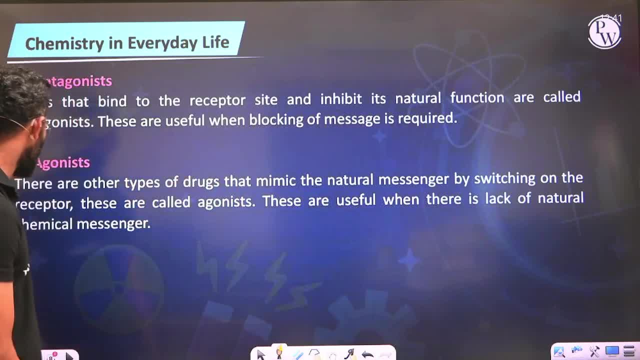 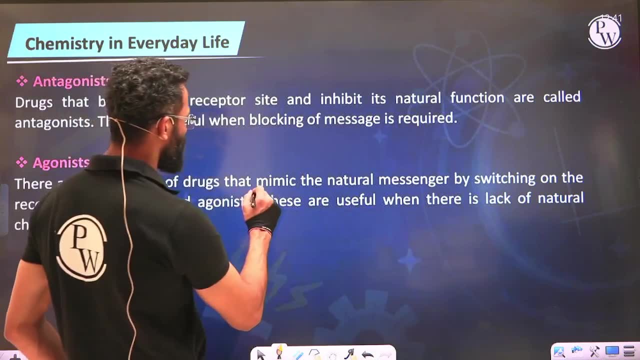 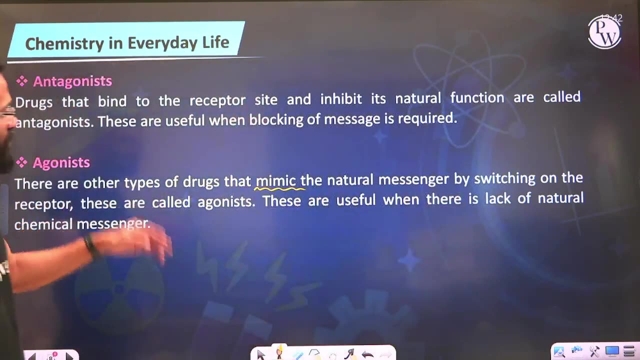 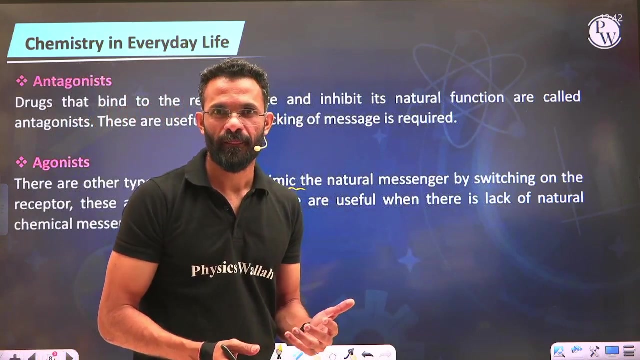 so, dear students, these are the two terms. first, we studied agonist. what are agonist? agonist are those types of drugs or medicines that mimic or copies the natural messenger by switching on the receptor. these are called as agonist, the example which I gave you, you know, when you are undergoing depression, which means there is a 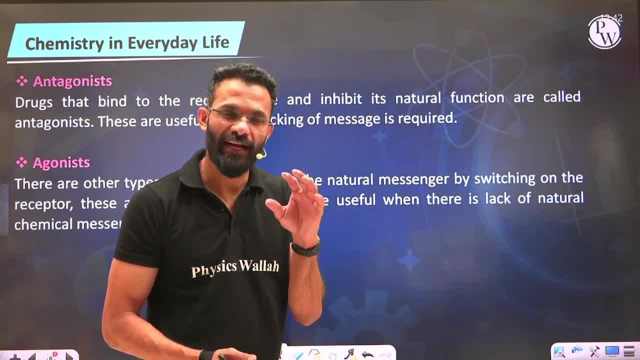 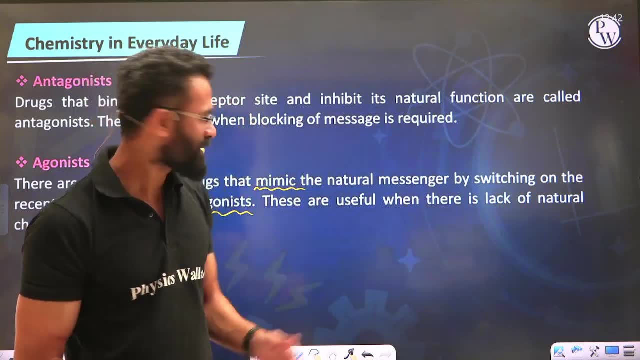 decrease in the concentration level of that chemical substance which was making you feel well-being, of that chemical substance which was making you feel well-being, of that chemical substance which was making you feel well-being of yourself or happy. so basically, this kind of medicine, agonist, are useful when there is a lack of 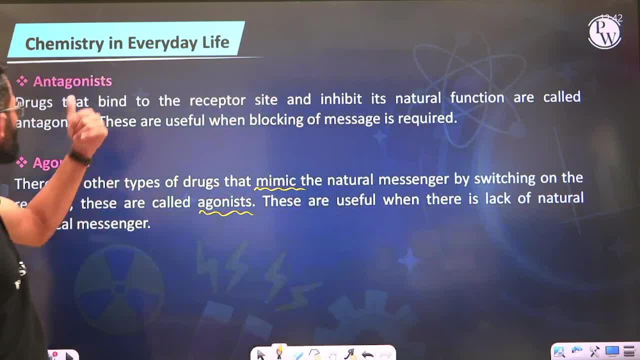 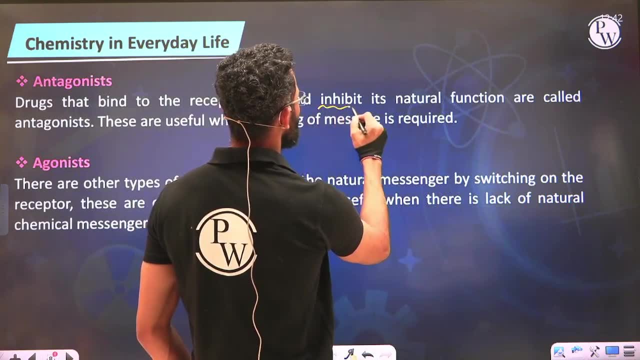 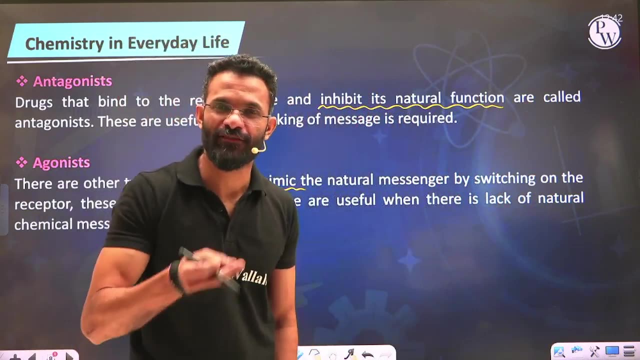 a natural chemical messengers. and what is antagonist? antagonist are those drugs that bind to the receptor site and inhibits the natural function of chemical messenger, like anesthesia. anesthesia itself got attached to the receptor and inhibited the interaction between the natural chemical messenger and the natural chemical messenger and the natural chemical messenger. 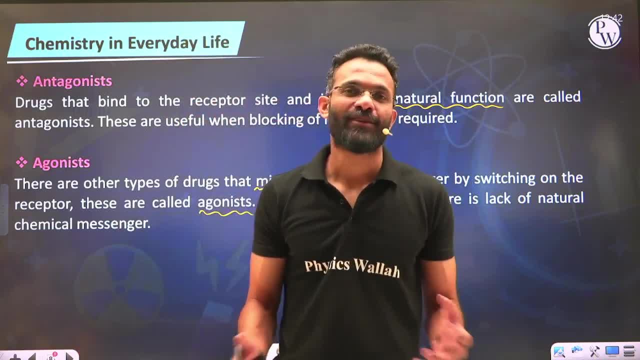 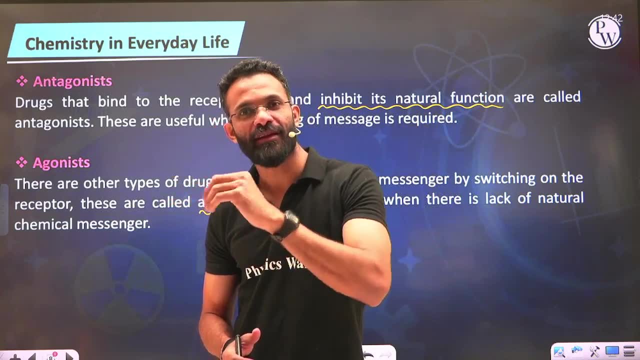 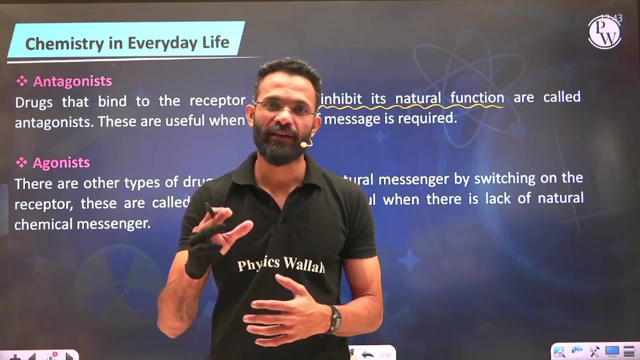 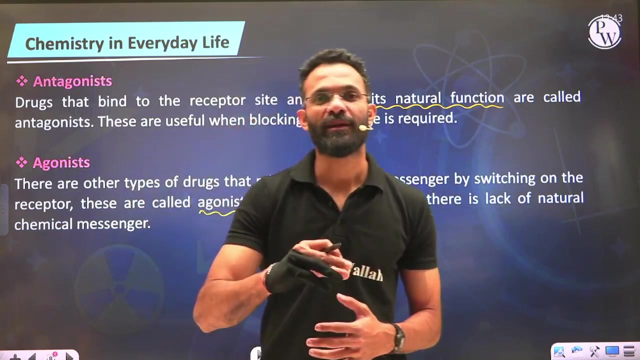 and receptor. so, guys, when we studied interaction of a drug with the target, the first target we studied was enzyme, and with enzyme there are two types of drugs which we studied: competitive inhibitors and non competitive inhibitors. competitive inhibitors: directly compared with the substrate and themselves get attached to the active site. non competitive inhibitor attaches. 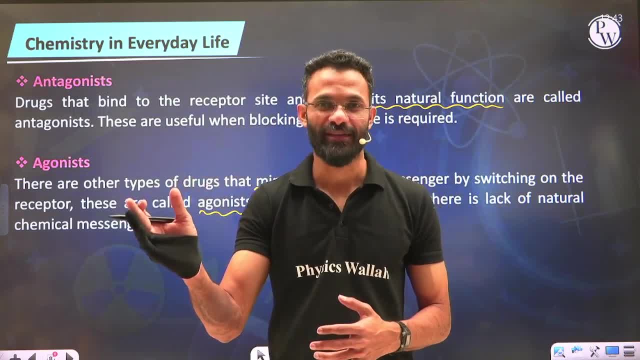 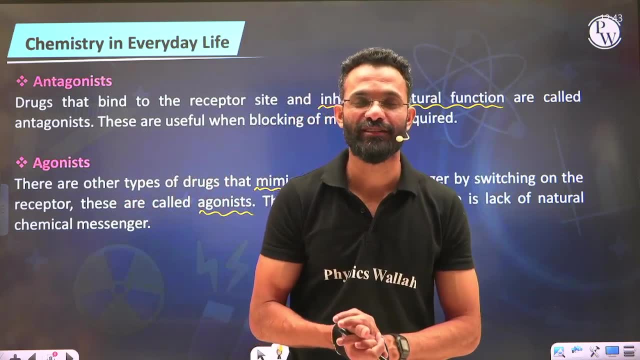 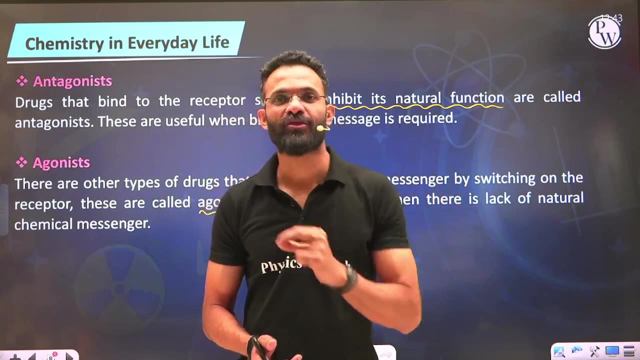 itself to the allosteric site and changes the shape of active site such that that enzyme can no more accommodate the substrate and is no more further interaction with the region can take place, whereas when you talk about drug and receptor interaction, there are two types of drugs which can interact with. 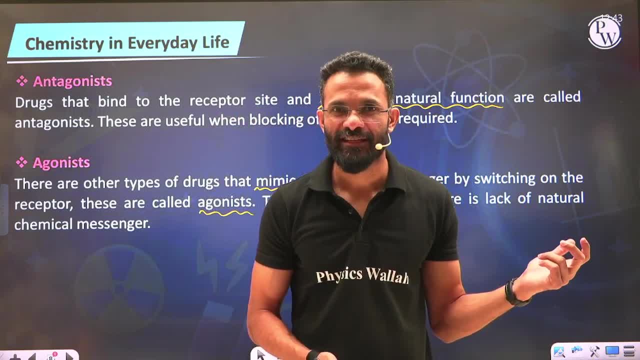 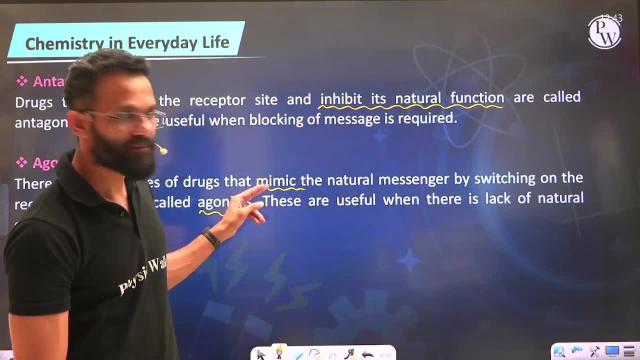 the receptor and produce certain signals. those drugs or the medicines are agonist and antagonist. agonist are the ones which copies or mimics the activity or the function of natural messenger. antagonists are the one which innervates the receptor and acts as a number of workers on the receptor. you can see here the 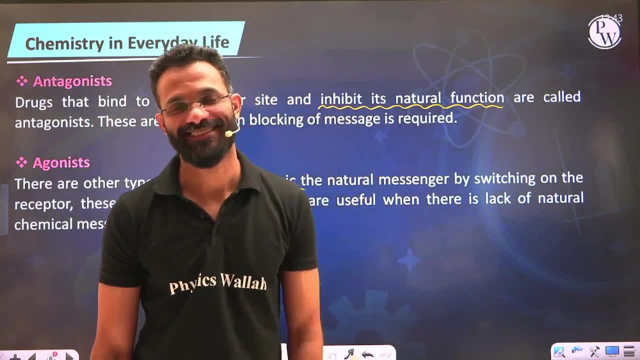 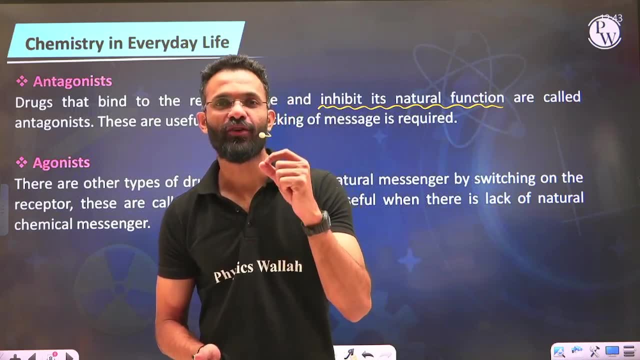 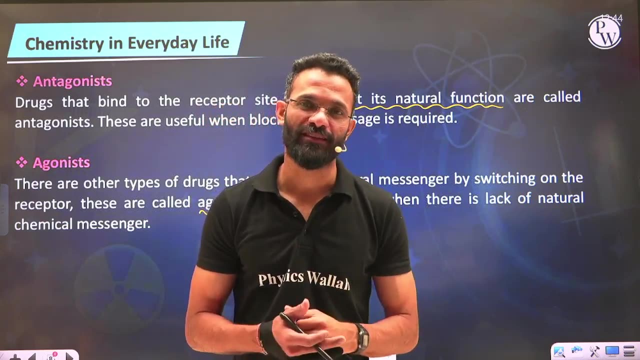 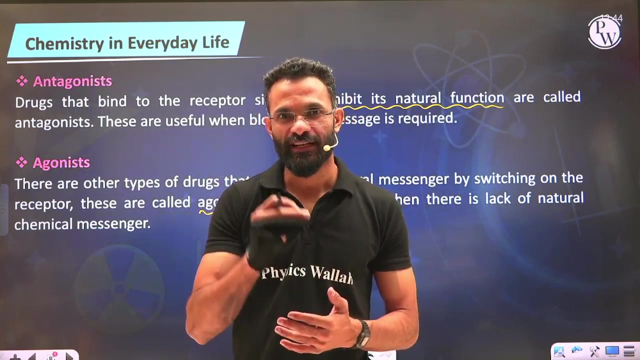 inhibits the function of natural messenger. so, dear students, what we have studied so far? well, we studied three things here. first, we got introduced to a term called as drugs or the medicines. second, we saw how exactly are we supposed to classify the drugs, or how exactly we classify the drugs. and the third one: we studied the drug and target interaction. so we studied. 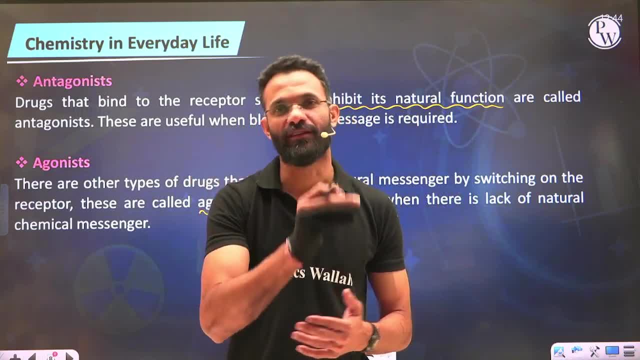 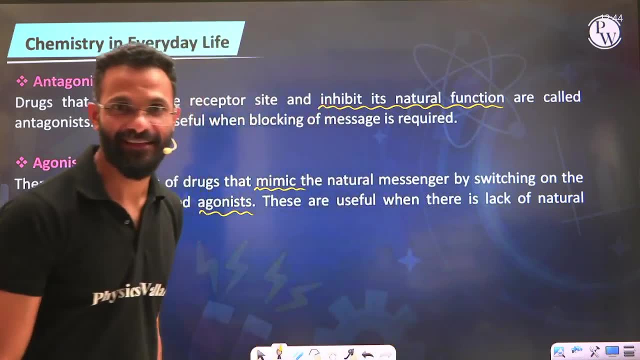 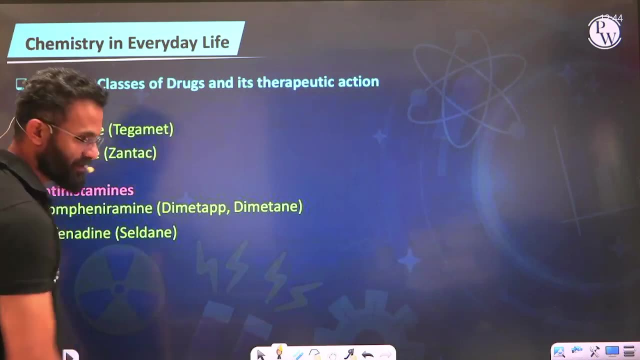 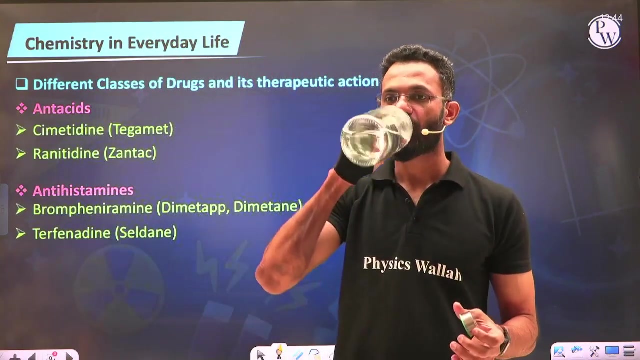 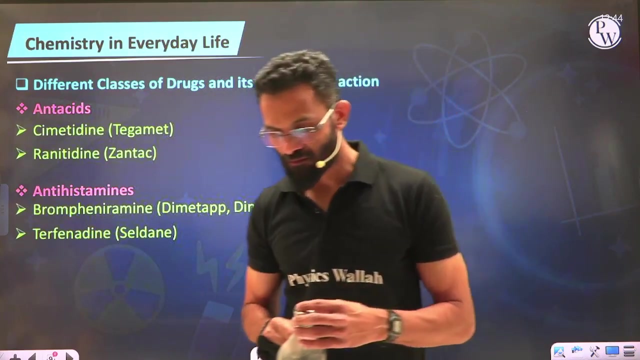 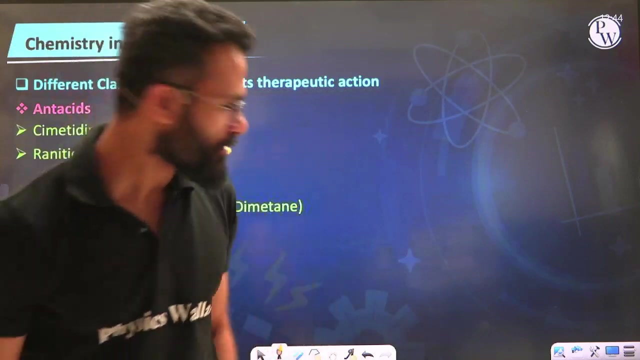 interaction of drug with enzyme and interaction of drugs with receptor protein. now we are entering into the most important part of chapter, that is, different classes of drugs and its therapeutic actions. so, guys, just hold on you, you, okay, everyone. so this is what i was talking about, why we have to learn this chapter. 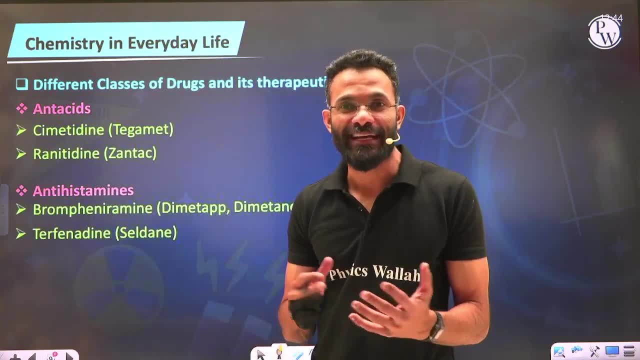 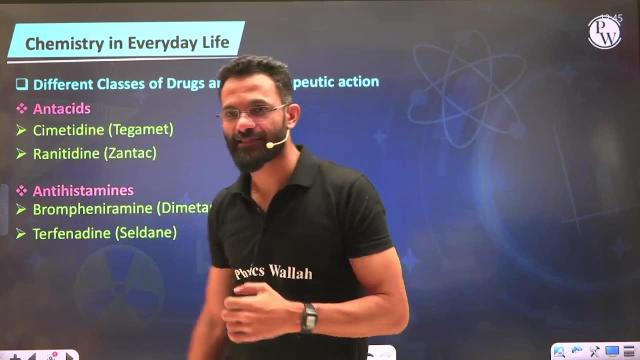 is because there are so many things which we come across in our daily life and we need to have a knowledge of that. so the first important type of drug, or the class of drug that we are learning, is antacids. all right, guys, we all are aware that when we experience that excess of 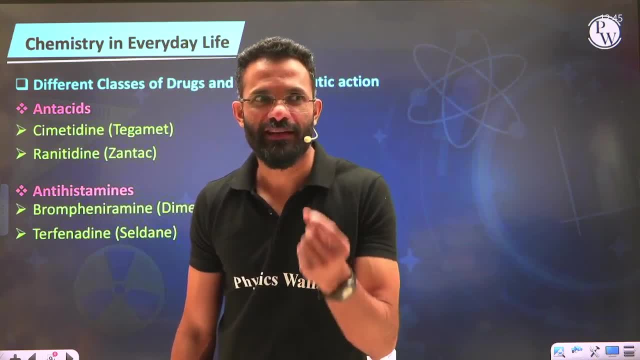 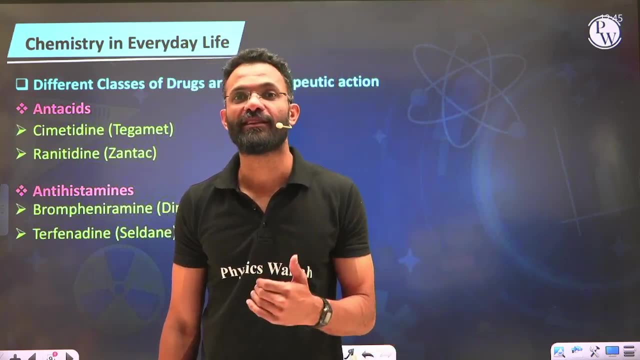 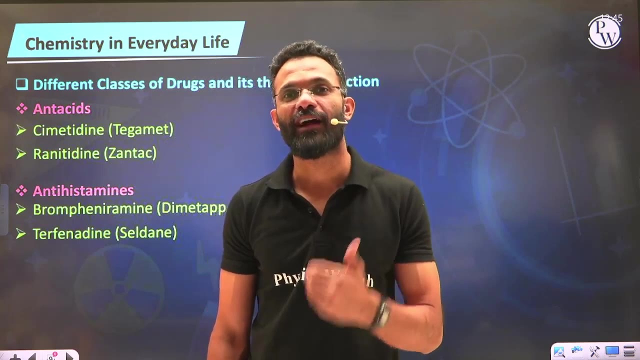 acidity. we eat eno, or we eat a tablet called gelasil right, or omaze is another tablet that we eat before eating the food. now, these all medicines are basically what they are: the one which neutralizes the excess of acidity that we have in our stomach, so those medicines which are used to 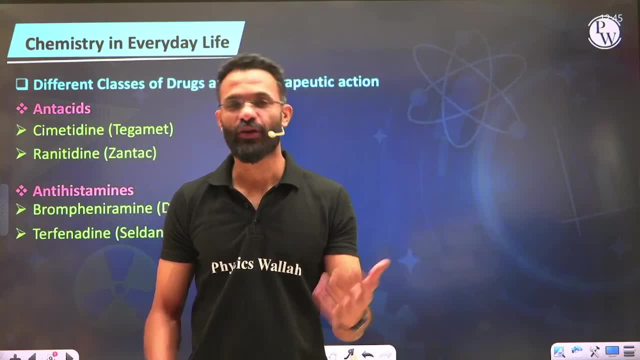 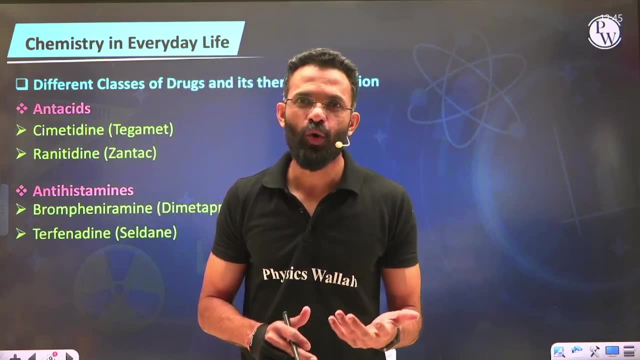 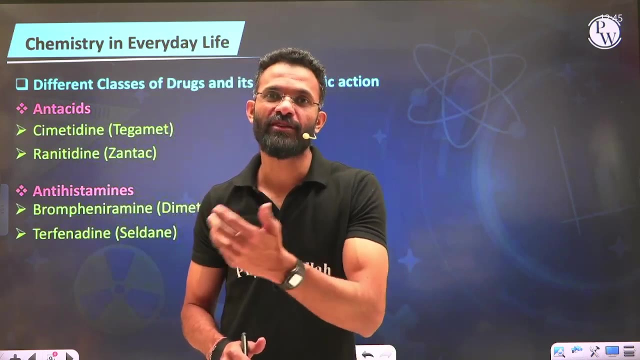 act against the excess of acid is what you call it as antacids. so if you talk about the historical development of antacids, in old days we commonly used to eat antacids such as bicarbonates or metal hydroxides such as mg oh twice or al oh twice, that is, aluminum hydroxide, magnesium hydroxide. 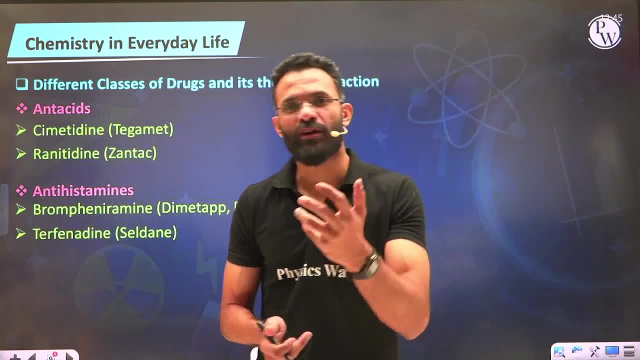 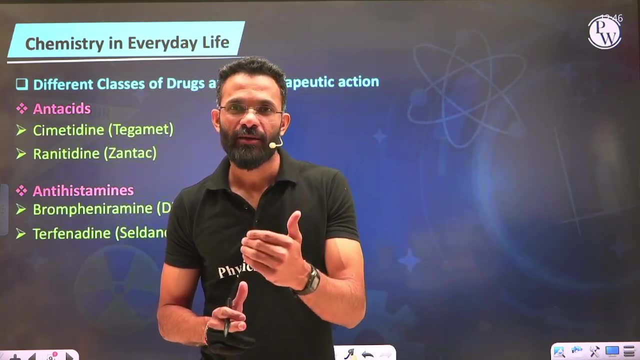 and bicarbonates, out of which, if we talk about the bicarbonates, bicarbonates are not the best of antacids which are considered why? because these bicarbonates are found to be soluble in the body and they are not soluble in the body, so they are not soluble in the body. so 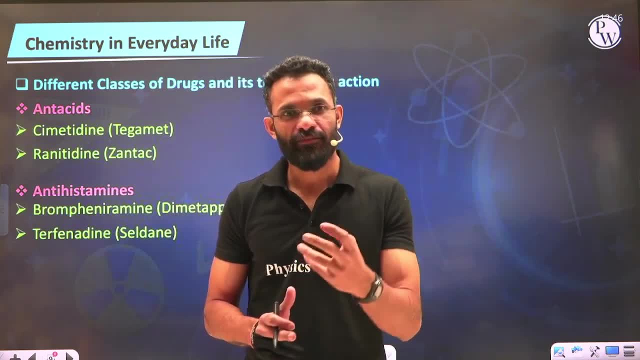 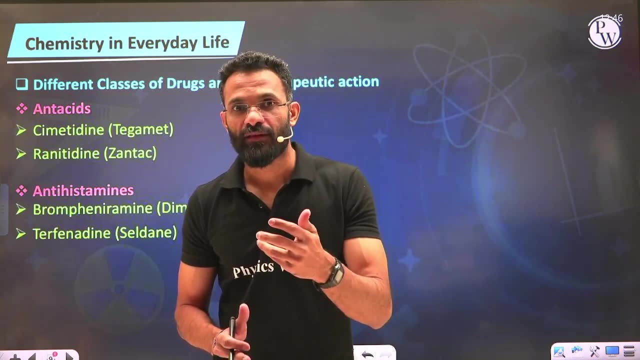 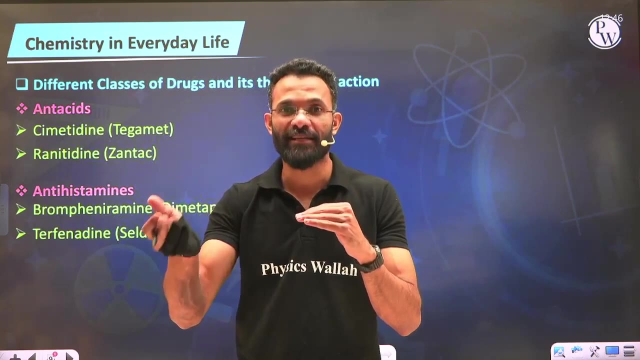 they are not soluble in water. and because they're water soluble, let's say if person is experiencing an acidity, so a person ate that bicarbonates in excess. so whatever acidity that person was experiencing, let's say that acidity got neutralized by the base, that is, bicarbonate. 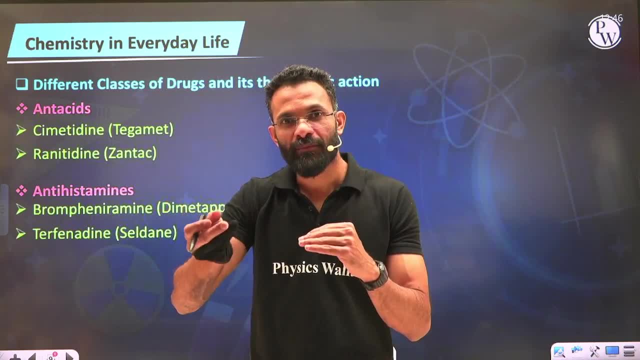 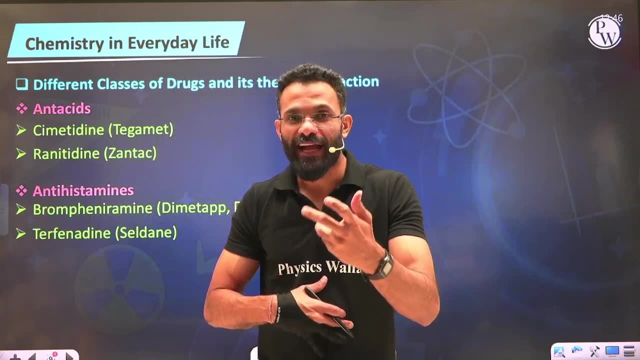 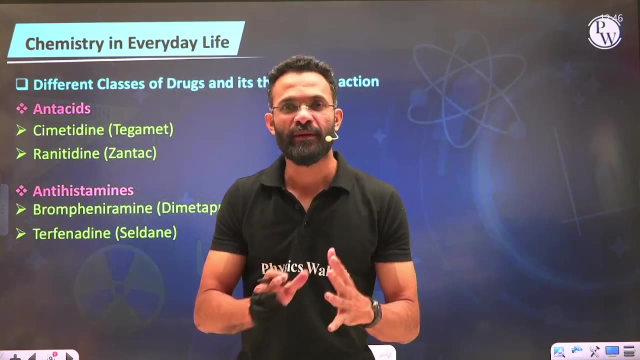 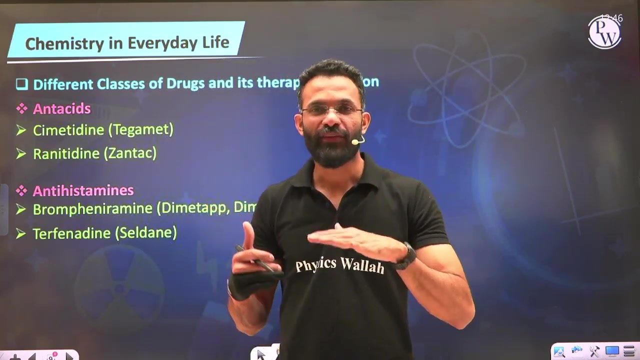 eaten by that person, but because the bicarbonate that person has consumed is in excess, the excess amount of bicarbonate which is present in the stomach. that will cause secretion of more acid to neutralize this bicarbonate. i repeat: if person is experiencing an acidity and let's say that person has eaten the bicarbonate as an antacid, so as much of acidity. 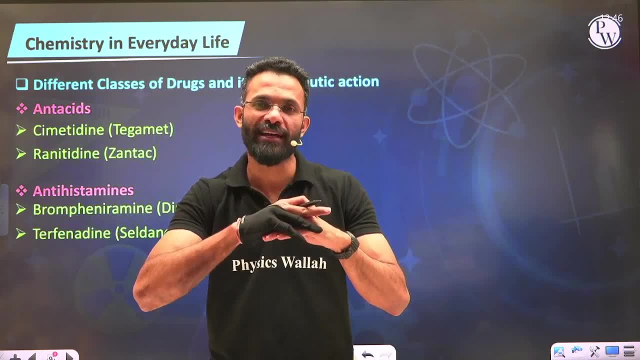 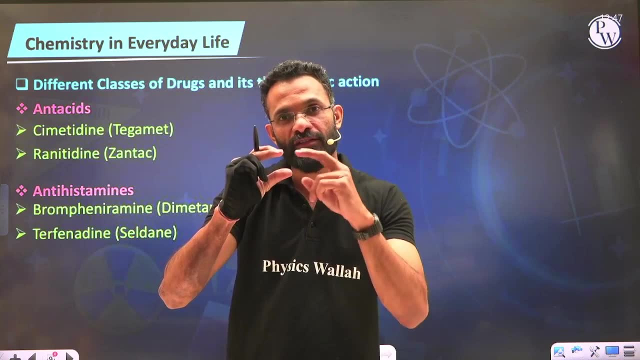 that person is experiencing. let's say, the whole acidity got neutralized by the bicarbonate, but the bicarbonate which that person has consumed is in excess. so the excess amount of bicarbonate which is consumed will now make body to secret even more acid to neutralize the excess of base. 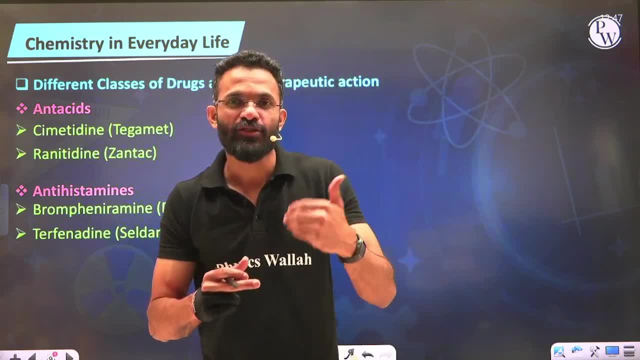 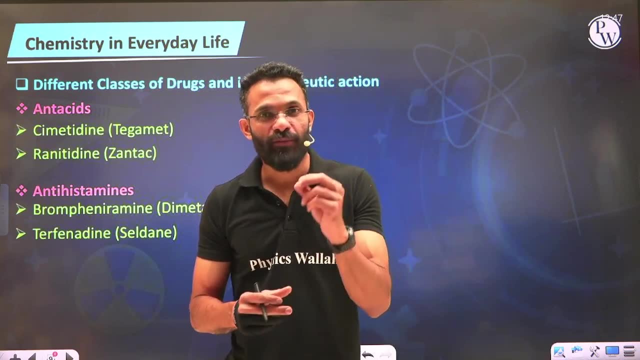 so, in this process, what is happening? there is excess of acid which is getting secreted by the body because bicarbonate is water soluble. hence it was important that you eat precise amount of bicarbonate. by mistake, if you eat excess of bicarbonate, body is going to secret more and 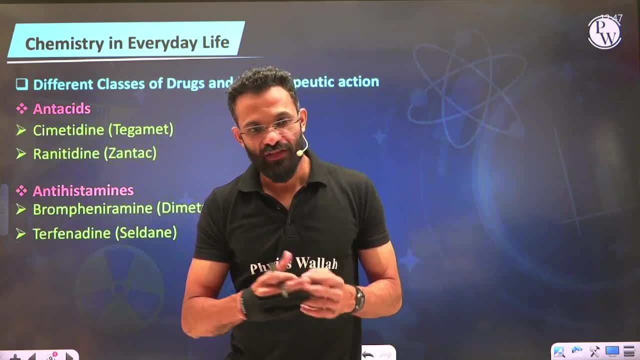 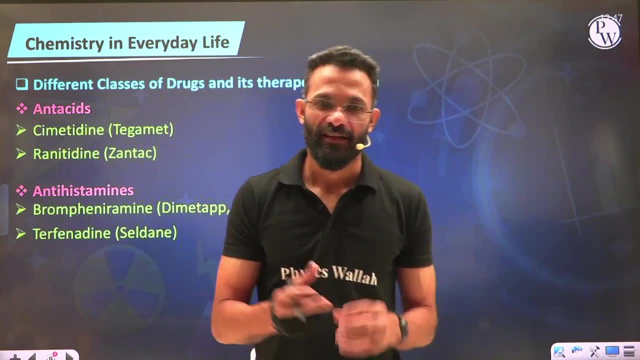 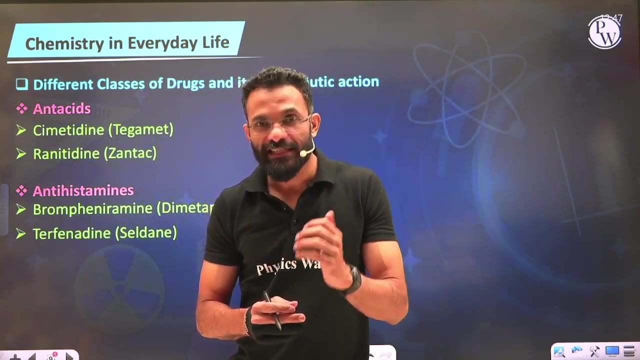 more acid. hence it was not the preferred antacid. so we started eating hydroxides, metal hydroxides such as aluminum hydroxide or magnesium hydroxide. now, these metal hydroxides being water insoluble, it does not cause our body secret more and more acids. hence, those are the 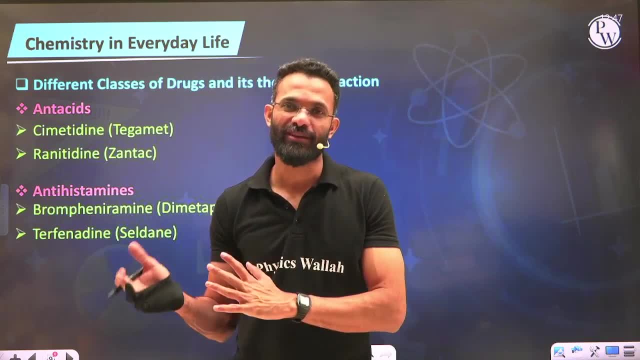 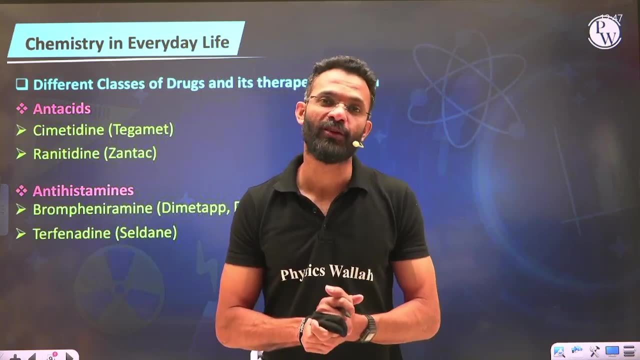 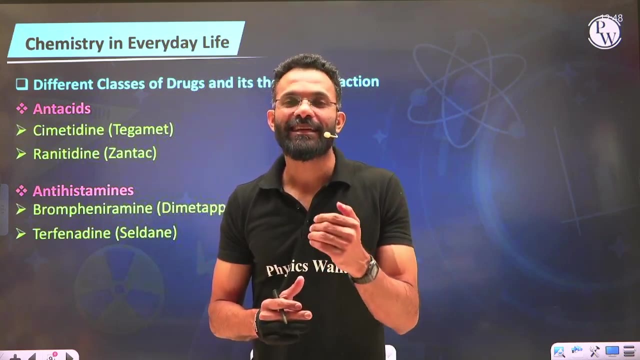 preferred one. so preferred antacids are metal hydroxides, but earlier we also used to eat or consume the bicarbonates. however, let me tell you in our body there exists a chemical substance called as histamine. what that histamine does is this histamine secrets a substance called as. 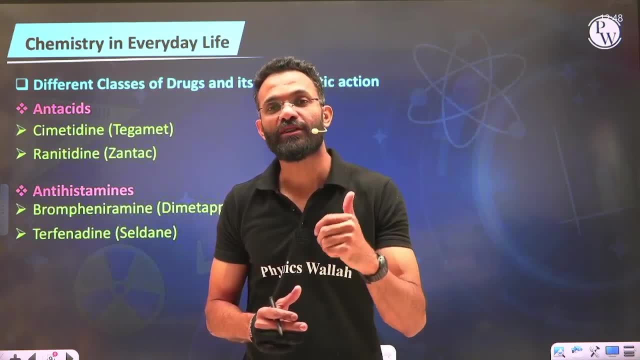 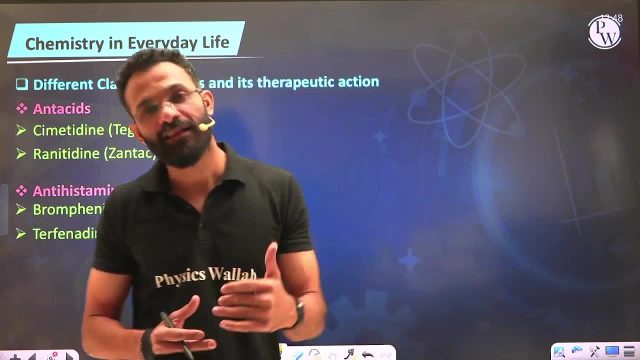 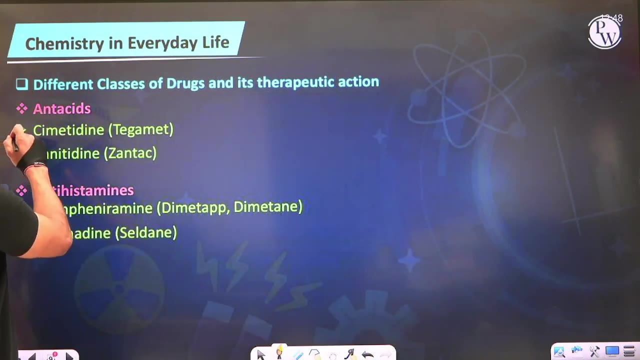 pepsine and hydroxychloroquine, hydrochloric acid which causes inflammation or which causes excess of acidity. so to neutralize this acidity, some other antacids or chemical substances were discovered which were basically cimetidine, also known as tagamet. so cimetidine was one of the most commonly used antacid, which 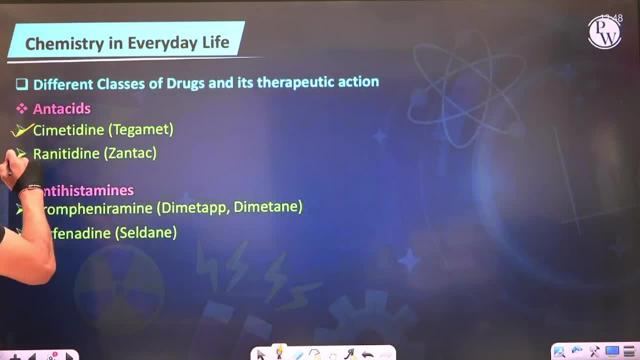 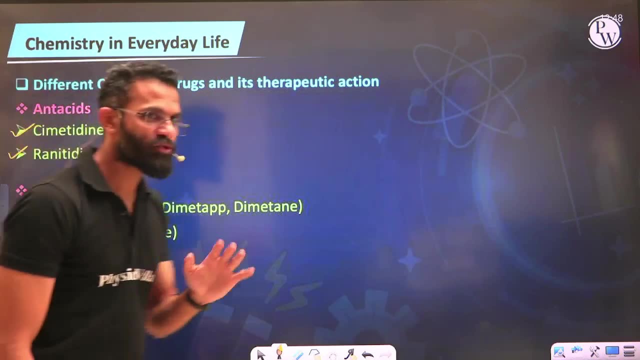 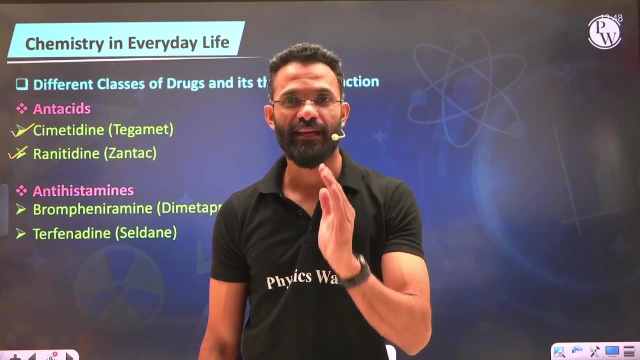 was used in earlier days until the next chemical substance which was derived, called as rinitidine, also known as zantac. so, guys, you will have to remember the names of antacid, first of all, bicarbonate and metal hydroxide. aloh, twice, mgoh, twice other than that, two more, two more antacids that you will have to remember. 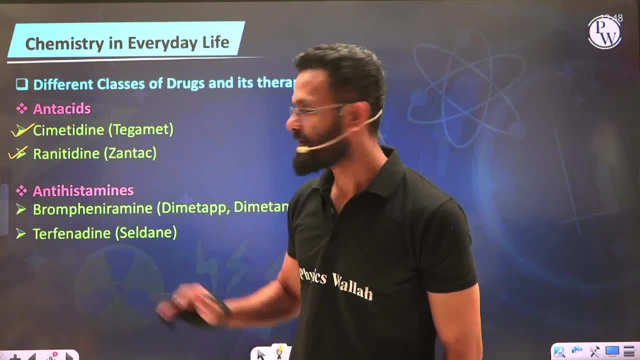 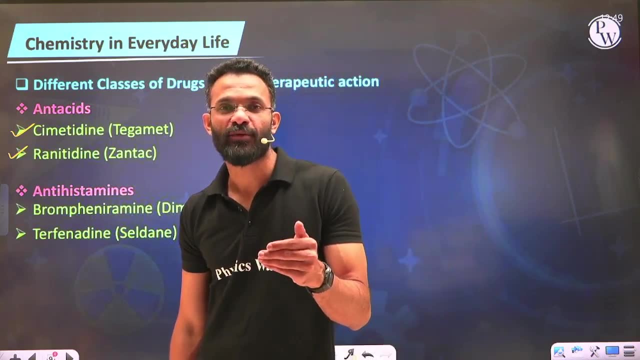 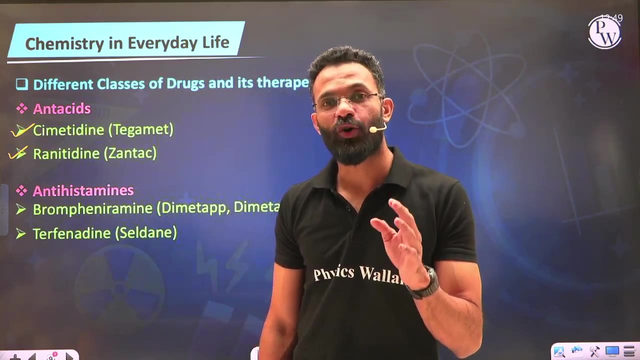 cimetidine and rinitidine. next category of a drug: we call it as antihistamine. well, just now i talked about histamine being responsible for creating acidity by secreting pepsine and hydrochloric acid. other than that, histamines also are the ones which are responsible for allergic interaction, so nasal congestion. 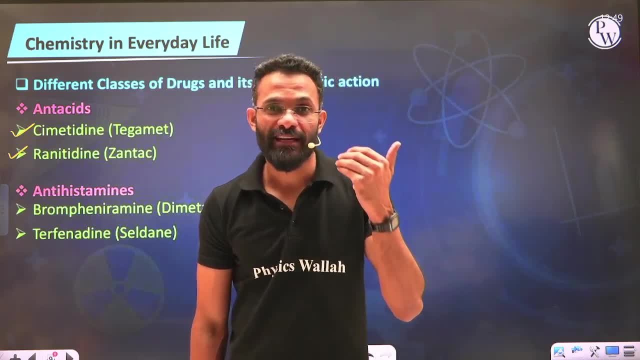 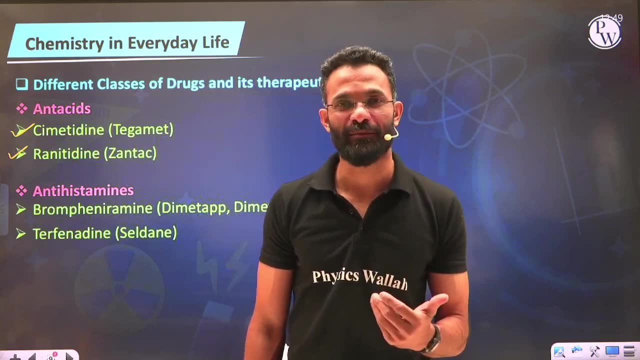 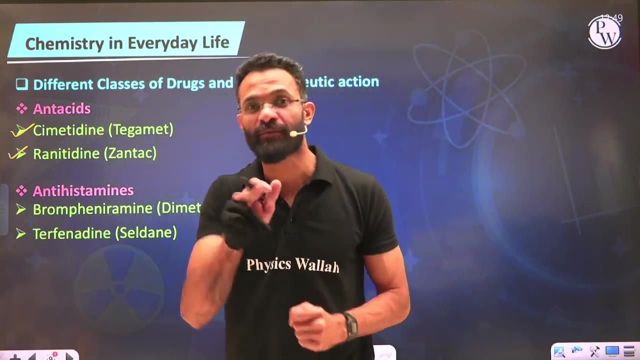 or running eyes, watery eyes, running nose- all these are the allergic responses which are caused due to histamine as a chemical substance. so those medicines are the drugs which are used to inhibit the action of this histamine which causes the allergic responses in our body. 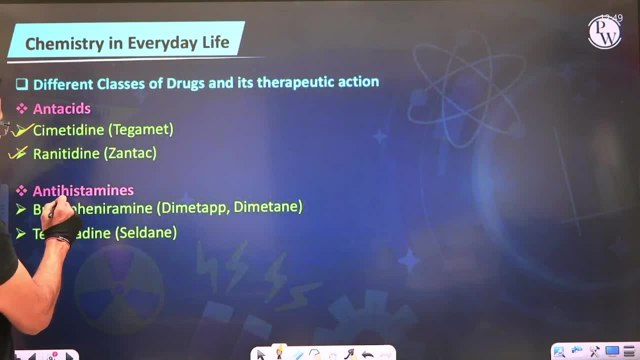 those chemical substances are called as antihistamine, as the name suggests. those medicines which will function against the histamine action are called as antihistamine. so which antihistamine will have to learn first? one is bromphenamine, brompheniramine, which is also. 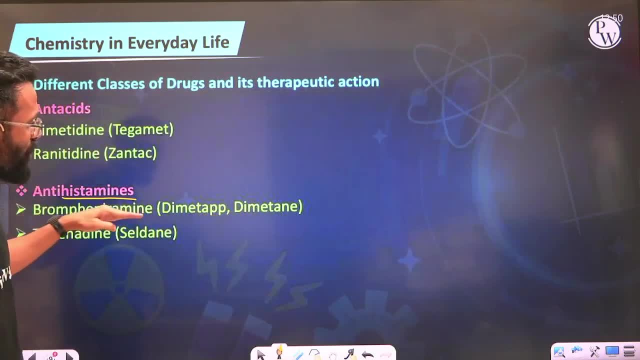 known as dimetap or dimetane. see, we are taking all the possible names here because in exam the question can be asked with respect to any of this name. so remember, the first antistamines is brompheniramine, also known as dimetap or dimetane, and second one is terfenidine, also known as. 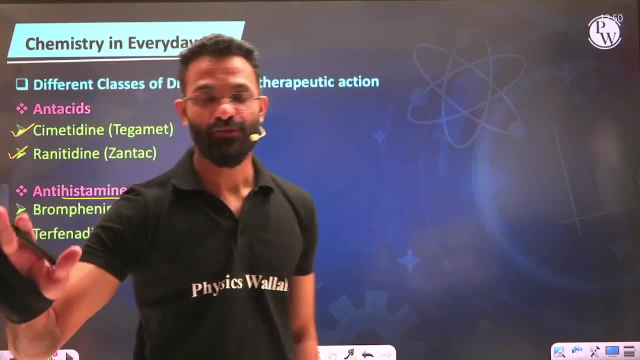 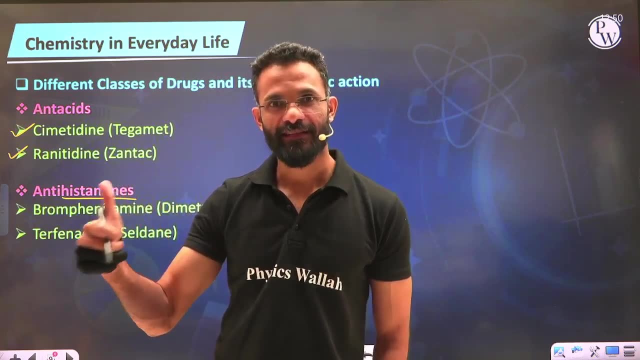 silden. so antacids, which antacids we came across so far? first one bicarbonate, then metal hydroxide, then, other than that, ranitidine and cimetidine. antihistamine are the one which inhibits the function of antihistamine, and this is what we will see here in the next video. so all right. so 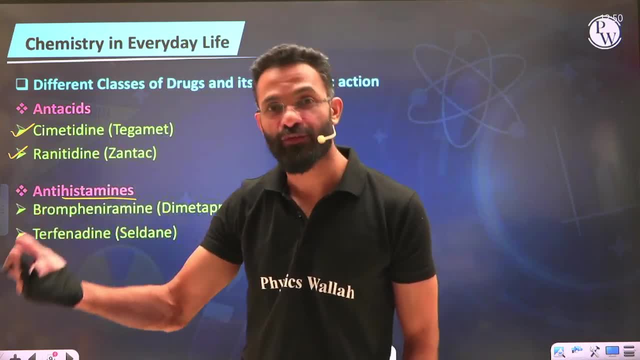 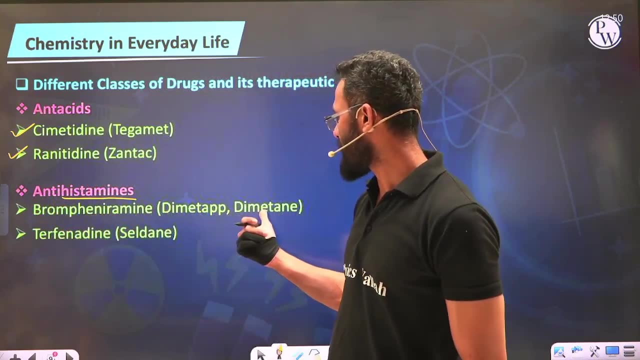 of histamine. histamine is the one which causes allergic reaction in the body. so which are the example of antihistamine? chrome fenyramine, also known as dimetab or dimetan, and then terfenidine, also known as silden. guys, I would highly. 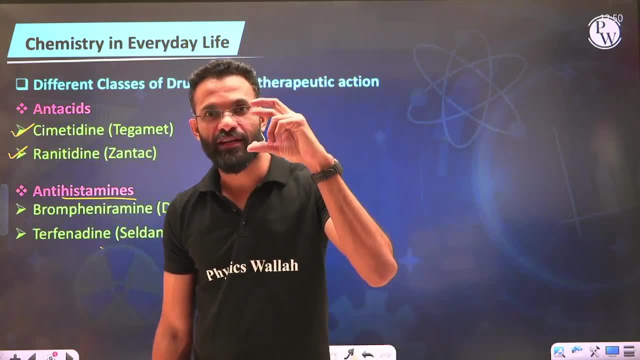 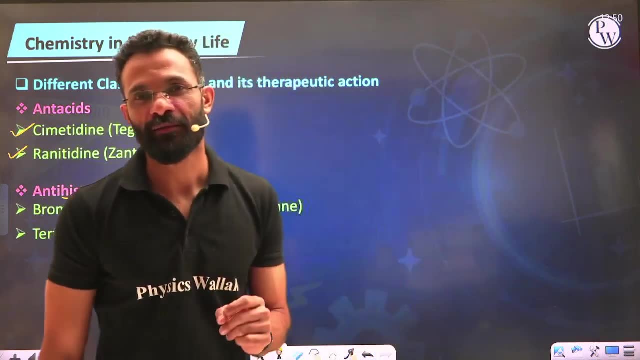 recommend you all that you take a particular category and write down the names of drugs related to that category at least four to five times, so that you will be able to remember it, because you will find maximum questions will be related to the names of drugs only. well, after this, the next category of a drug. 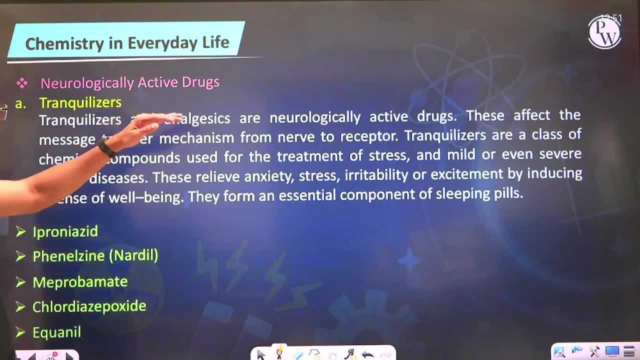 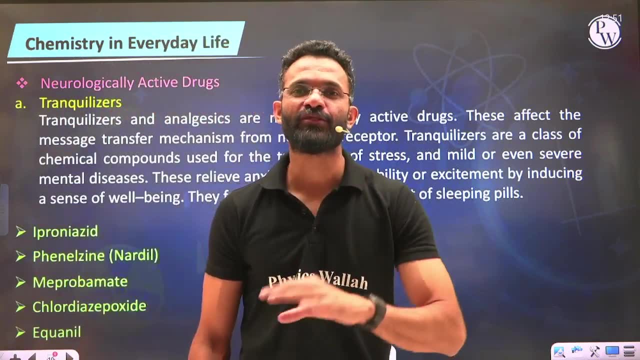 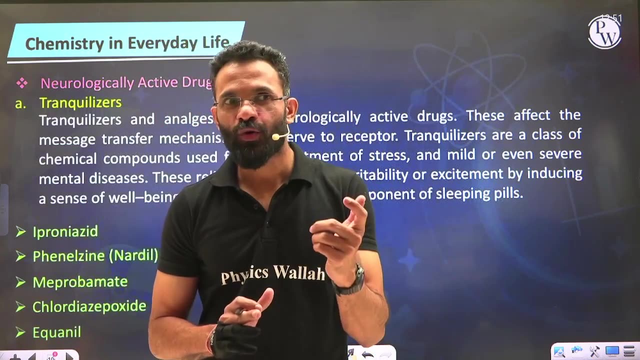 is what you call it as neurologically active drugs. so there are two types of drugs: tranquilizers and analgesics. first, let us get introduced to what exactly a tranquilizer? well, what is the meaning of tranquil? tranquil is the term which is related to calmness or peace of mind. so any 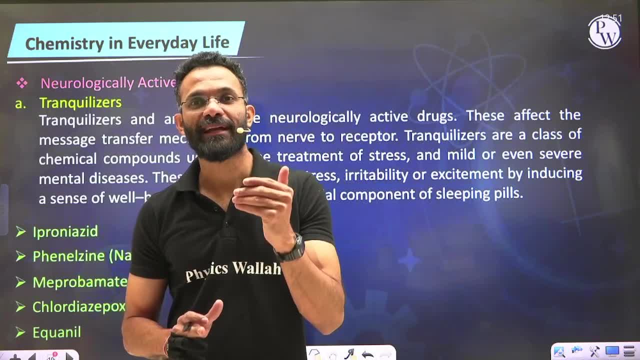 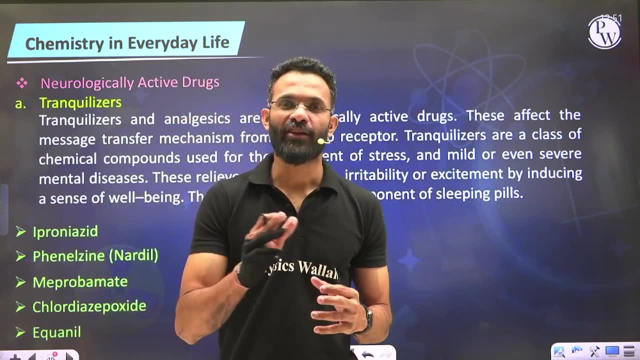 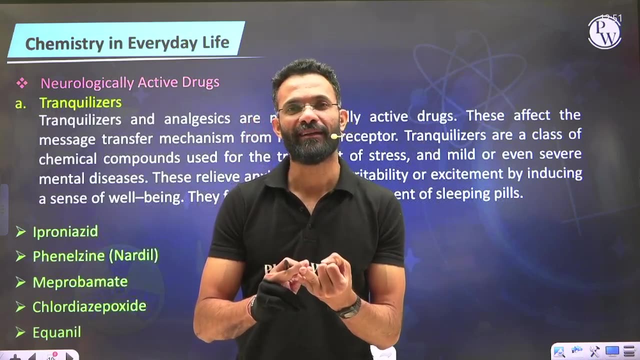 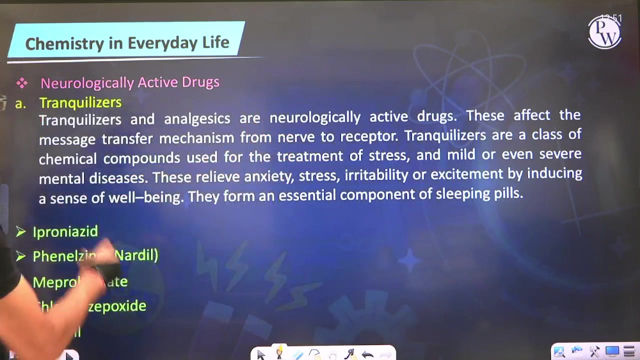 medicine which is used to bring that calmness is what you call it as tranquilizer. so tranquilizer is that category of a drug which is basically used to treat against the stress or any kind of mental illnesses. so hence we say tranquilizers and analgesics are neurologically active drugs. this affect the message transfer. 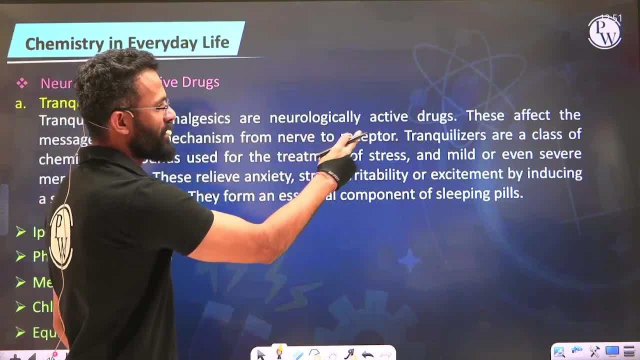 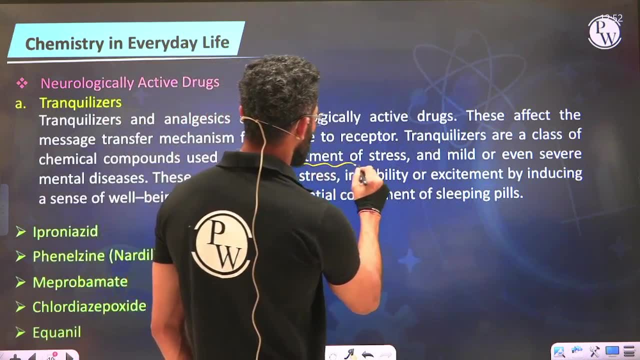 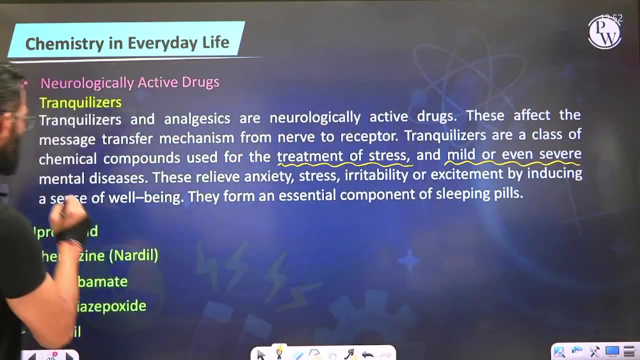 mechanism from nerve to receptor. and tranquilizers are the mass of chemical compound which are used to treat or which are used for the treatment of stress or mild or severe type of mental diseases. all right, so here are some example of tranquilizers and which we'll have to learn a pronia. 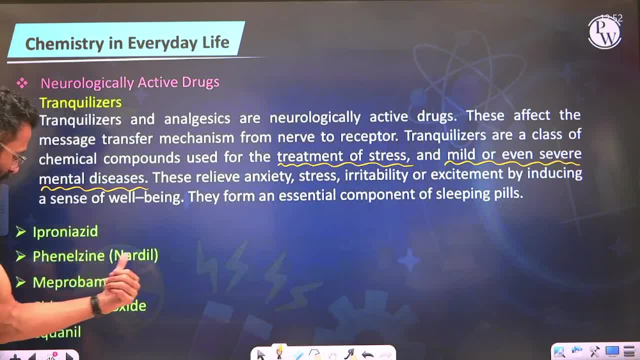 zied when I'll see, which is also known as by the name Nadel, mephrobumate chlordia. as a box side and in the middle of the body, we have a group called the oxide and equanil, and along with this you can also add to the list called equanil and valium. 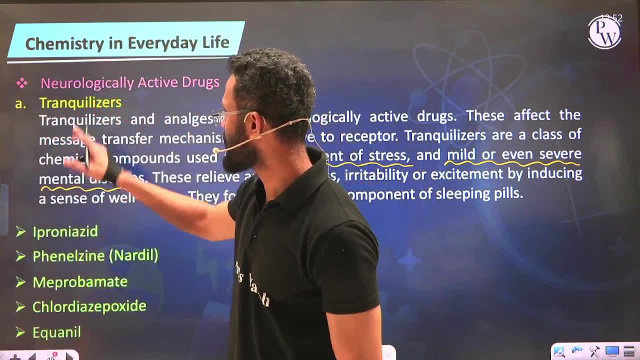 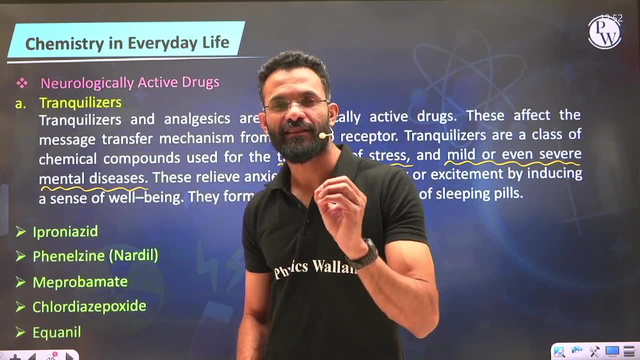 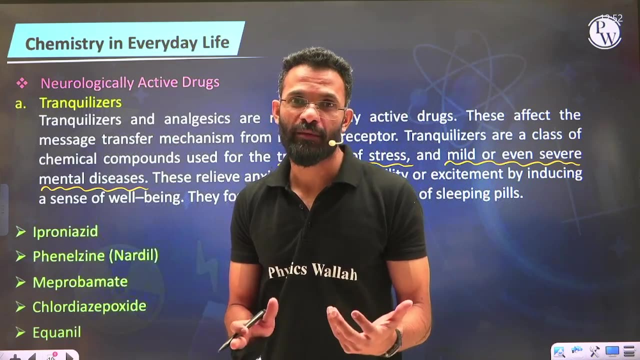 so, guys, these all are the example which belongs to the category of tranquilizers. again, tranquilizers are those medicines which are used to treat against the mental illnesses or any mental disease or stress, or, in fact, in the sleeping pills we use some of the chemical substance, which also belongs to the category of tranquilizers only, and the example that we'll 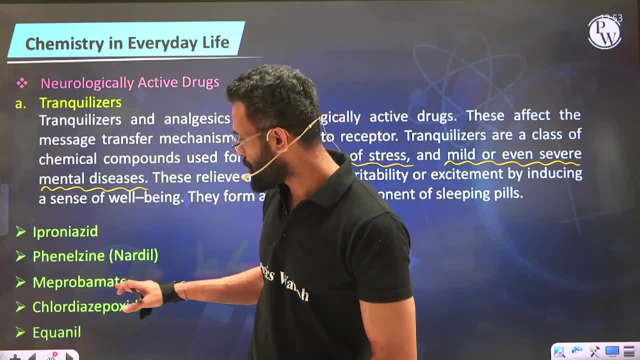 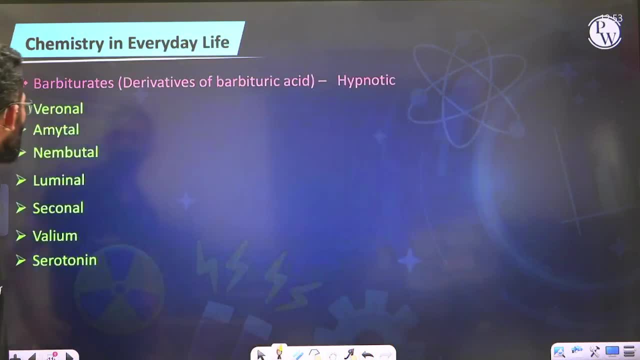 have to remember aproniazide, phenolzene, meprobamide, chlordiazepoxide, equanil and valium. other than this, there are some more which are basically considered to be a derivative of barbutyric acid. so since these all are the derivative of barbutyric acid, we call them as. 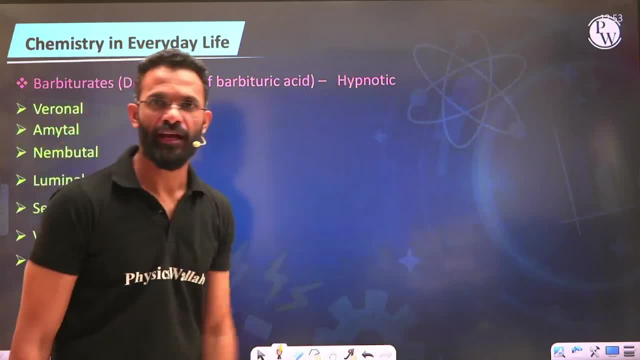 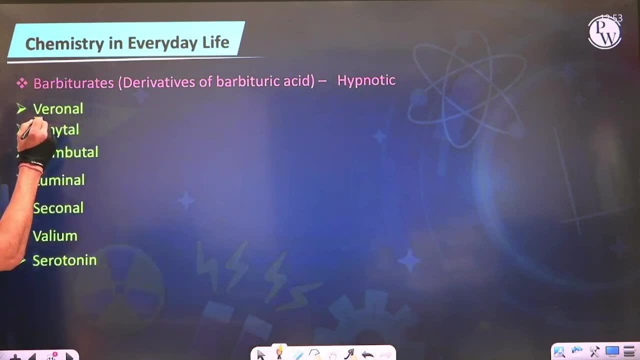 barbutyrates, or you also call them as hypnotic drugs. so to remember this, simply remember word valium, vanillas, vanillas, v stand for veronal, a stand for amytal, n for nebutyl, l for luminal and s for sequenil. so i simply remember this as vanillas v-a-n-l-s veronal, amytal, nebutyl, luminal and. 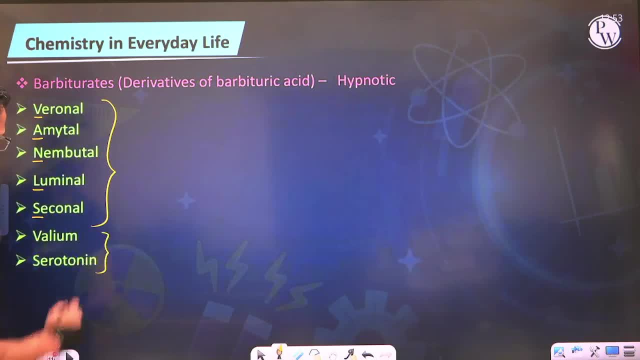 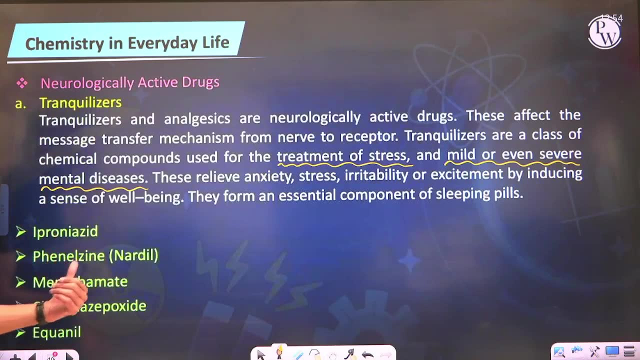 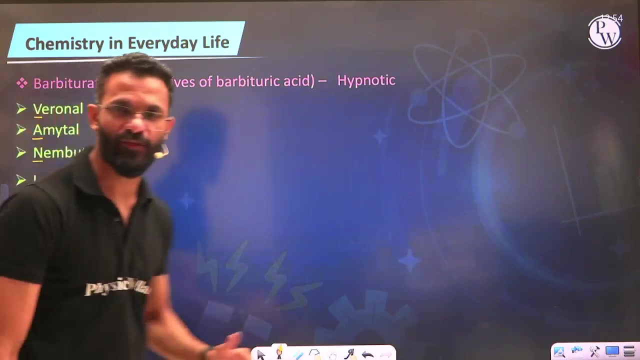 sequenil. other than this, two other than this. there are two more, called valium and serotonin. well, aproniazide, phenolzene, meprobamide, chlordiazepoxide, equanil, valium and serotonin, you remember them, them also together, and then simply add vanillas, veronal, amytal, nebutyl, luminal and sequenil, all. 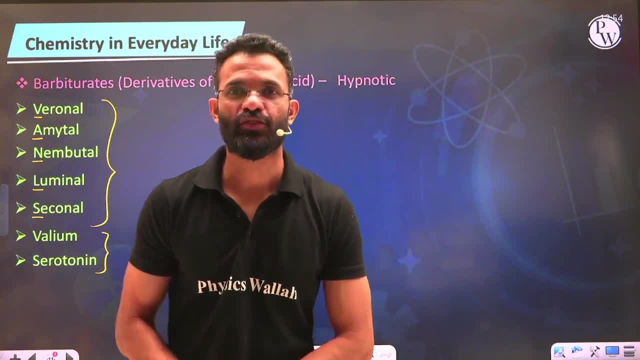 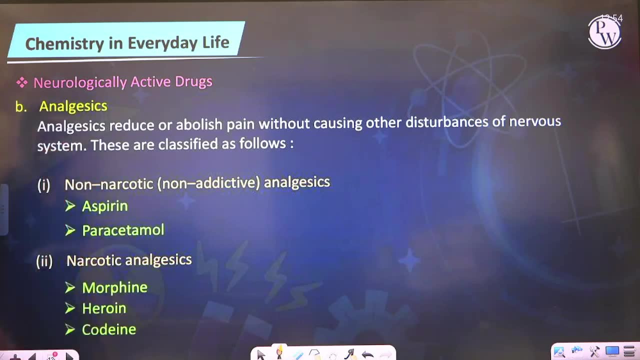 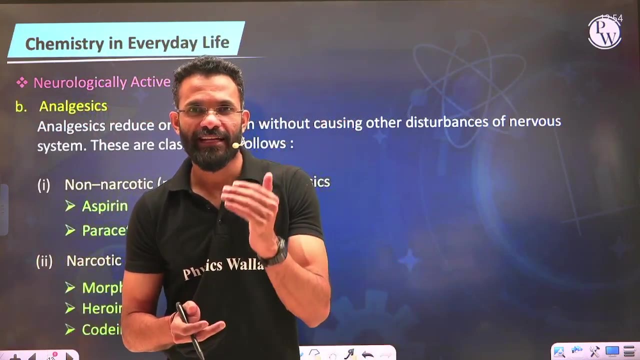 right. so this category of a drug is what you call it as tranquilizers. well, other than tranquilizer, the next category that we said is basically analgesic. analgesic, in simple term, you can also call it as painkillers. all right now, this analgesic we further classify into two categories. 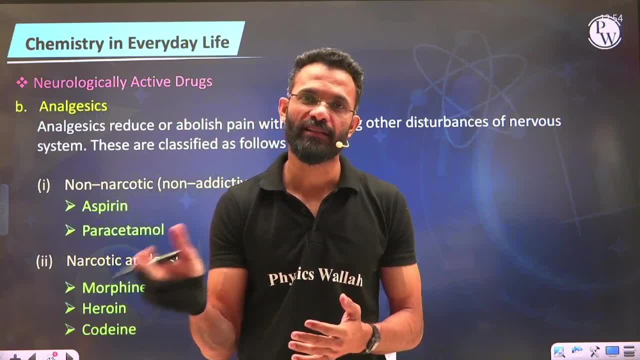 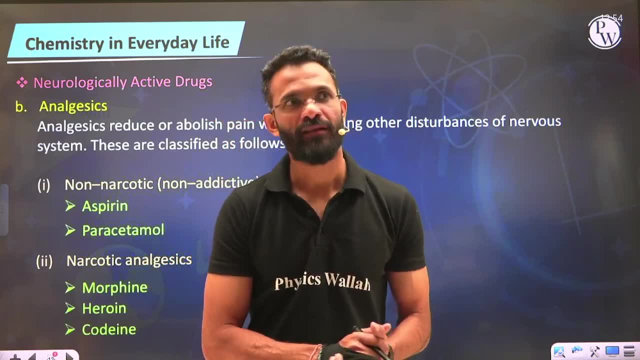 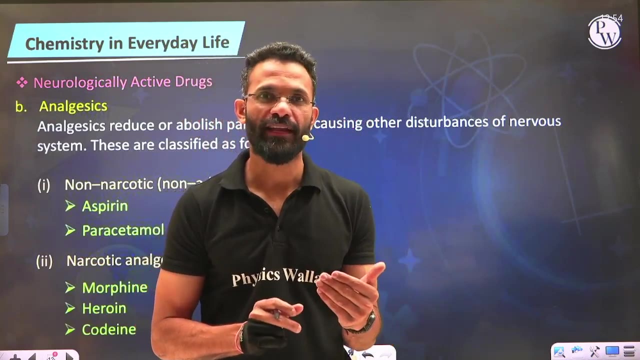 and those two categories are narcotics and non-narcotics. narcotic and non-narcotics: well, there is a term called as narcosis. narcosis is, you can say, a feeling of being in a deep sleep, is what you call it as narcosis, so you will see some kind of pain. 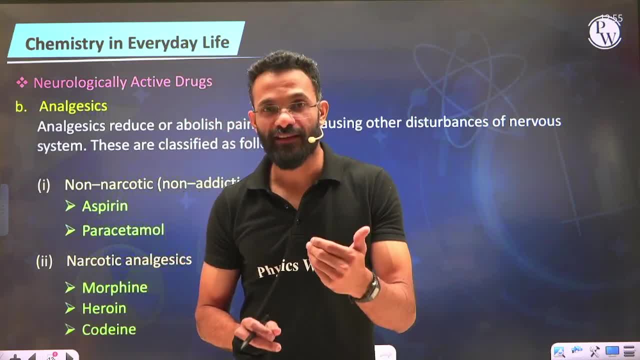 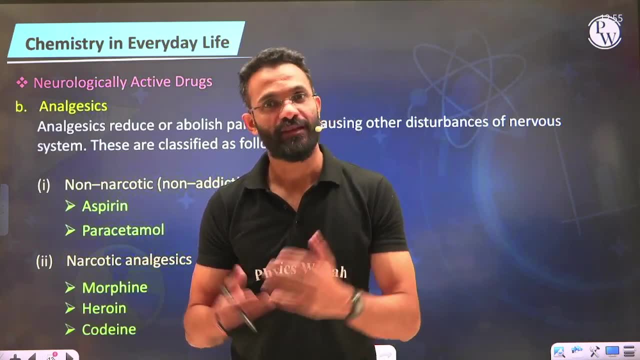 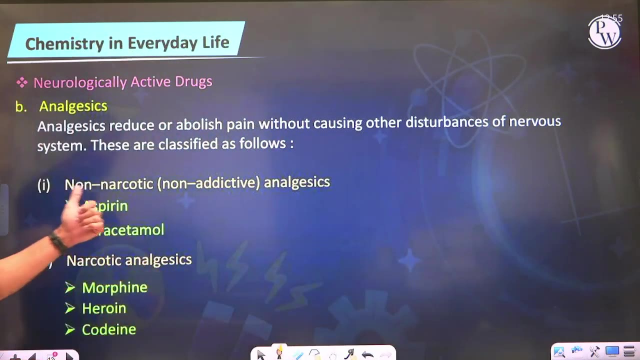 killers that we eat makes us feel like we are in a deep sleep and hence those kind of painkillers could be addictive as well. so when you say there are two types of painkillers or analgesic, which are called as narcotic analgesic and non-narcotic analgesic, so narcotic analgesic, like i said, the 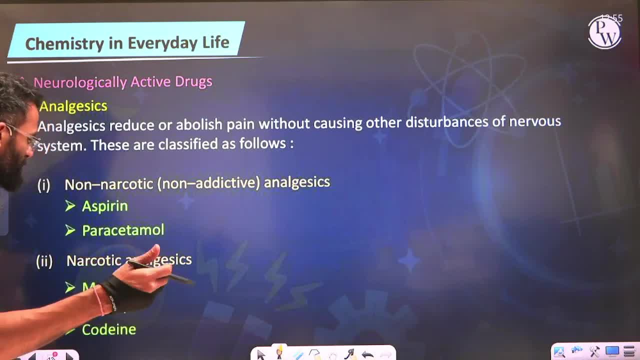 term narcosis meaning feeling of being in deep sleep, so those analgesic or painkiller which are in a deep sleep. if consumed in excess amount or on a regular basis, those could be addictive as well. hence narcotic analgesics are called as addictive painkillers, and the example of those 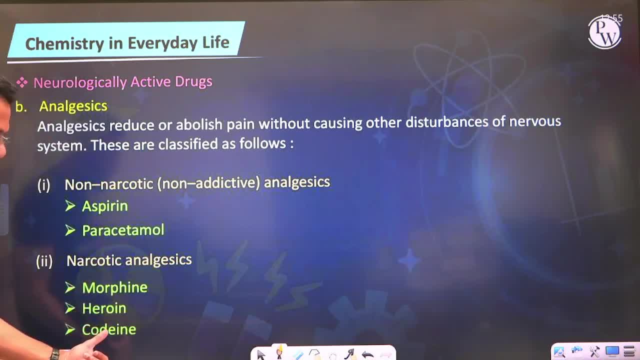 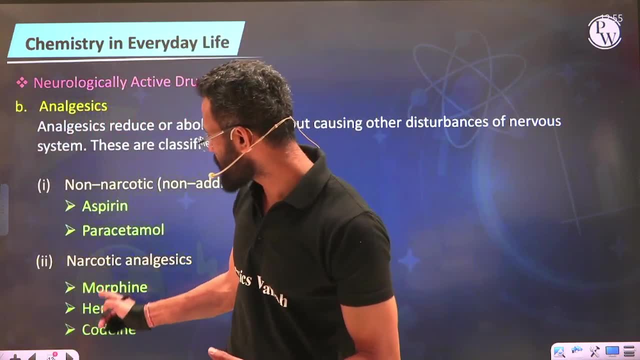 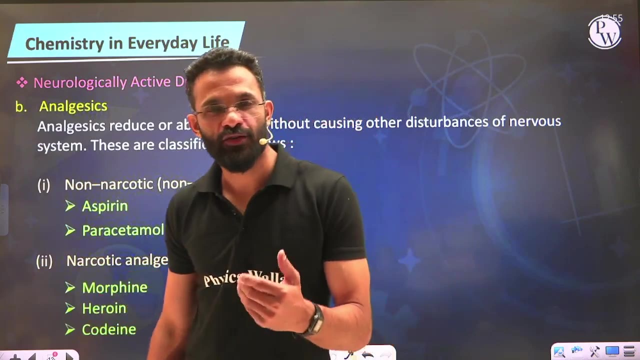 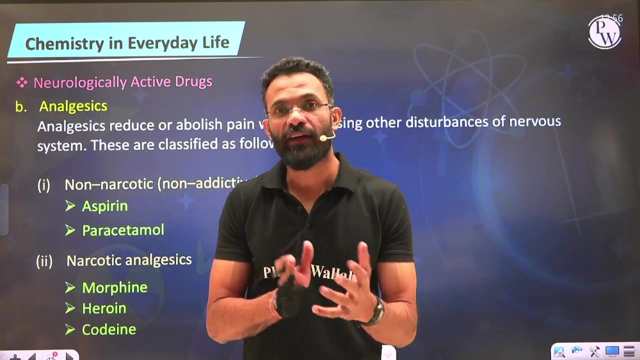 are morphine, heroin and codine. morphine, heroin and codine: well guys, these are high potency analgesics, or painkiller you can call, and hence these are used for. these are used for treating the kind of- you can say- pain a person experiences when they have. 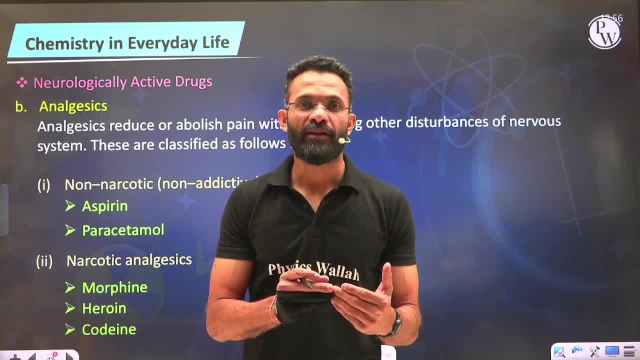 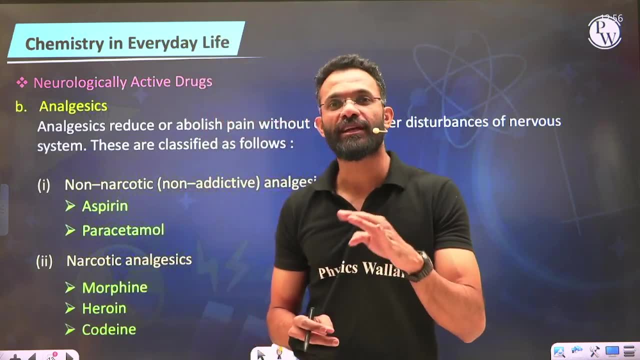 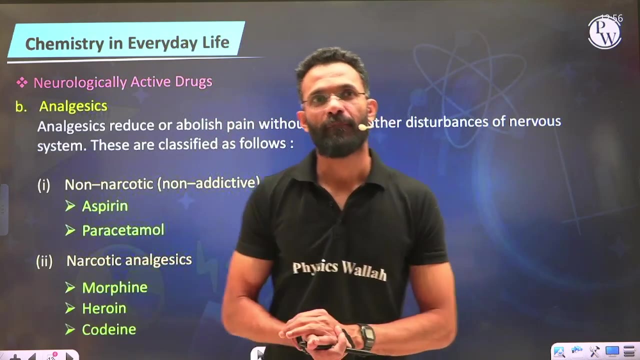 undergone surgery. so when a particular person have undergone surgery, after surgery, the pain that person experiences is enormous. so to subside those kind of pain, the medicines which are given are of this category, called as narcotic analgesic, or a person which is, let's say, 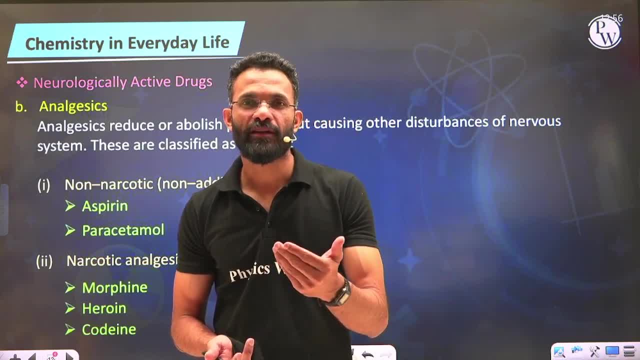 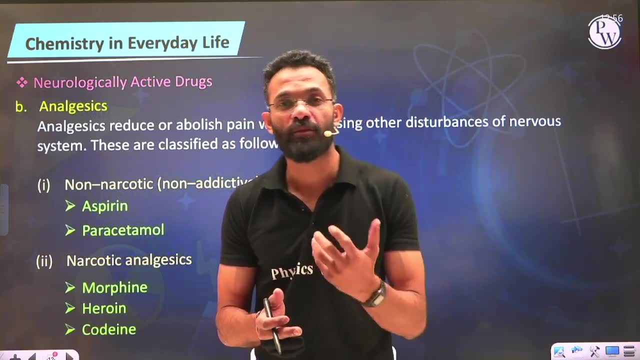 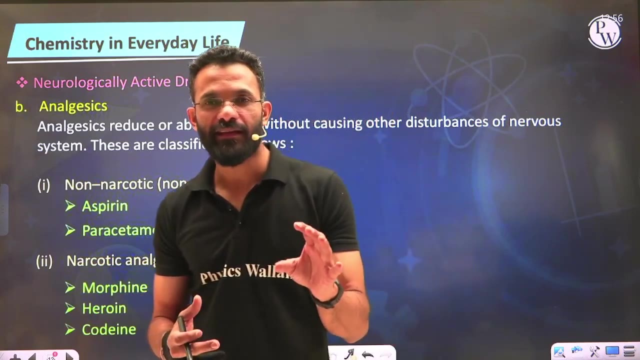 if a particular person has treated for the cancer, let's say so after cancer also. the body when experiences enormous pain, then to subside those kind of pain again we give this kind of medicine. so whenever any pain which is unbearable, then to treat those kind of pain we need high potency. 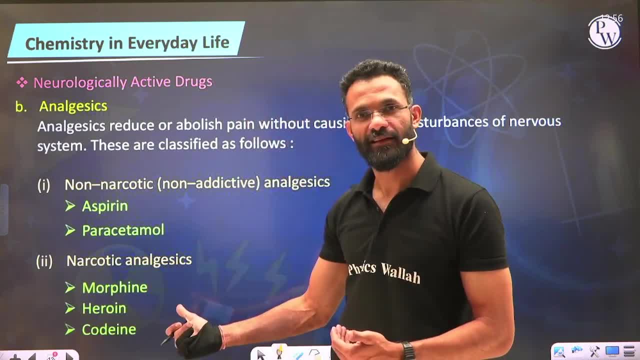 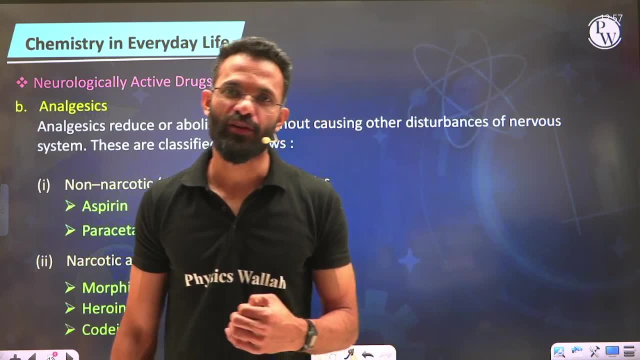 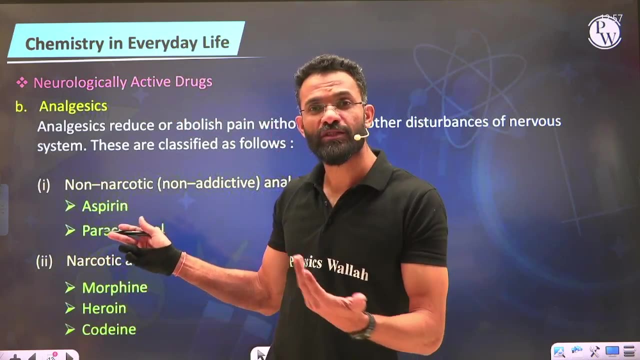 painkillers which are called as narcotic analgesics, whereas aspirin, paracetamol, paracetamol, crocin are very general painkillers that we use in our daily life as well. right, so if you are experiencing, let's say, headache, so what we do? we eat aspirin, we eat, we eat crocin, or if 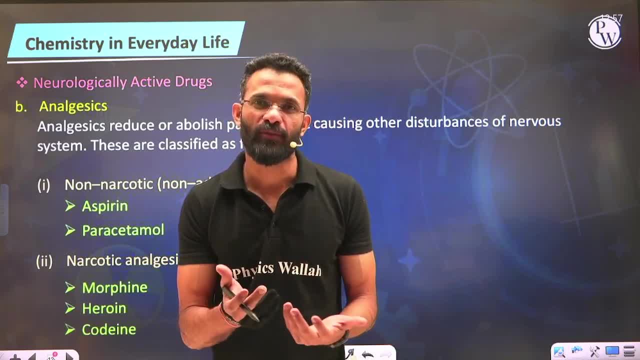 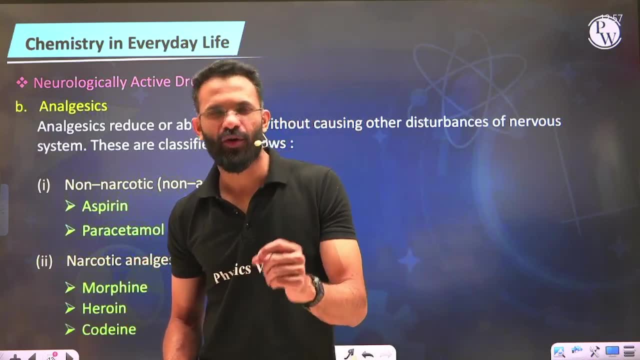 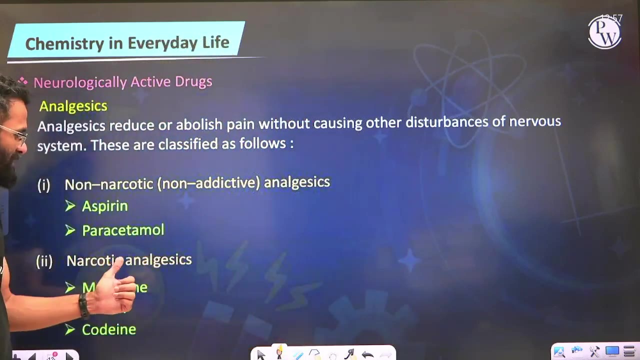 you are experiencing some minor muscular pain. what do we do? we eat myospas or we eat paracetamol. so these kind of medicines are used to treat minor or, you can say, a moderate pain, and they are non-addictive, so narcotic analgesics. 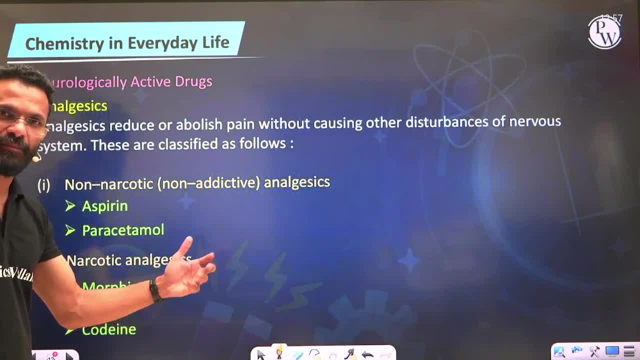 are addictive, which are used to treat against unbearable pains such as post-operative pains or a person who has undergone treatment of cancer. they are also, they also experience those kind of pain, so we give them this kind of medicine, whereas for the general, general pain, or to stop or kill that general pain, we basically give them a substances called, or medicine called, aspirin. 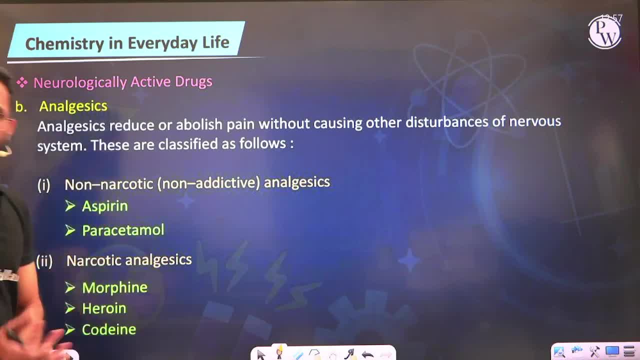 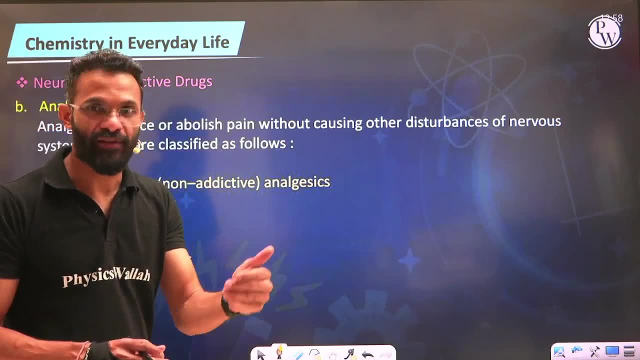 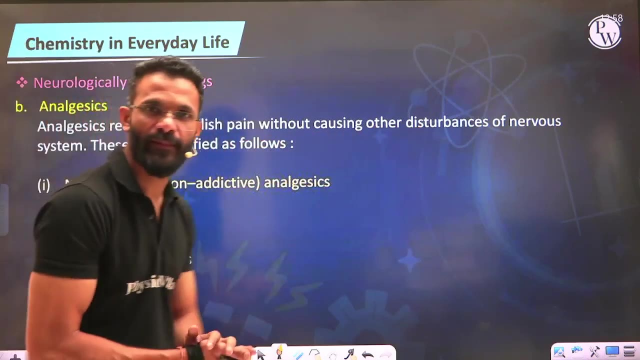 and paracetamol. so, in general, analgesics are painkillers which abolishes the pain without any side reaction. without any side reaction as in, without causing any other disturbances to the nervous system. guys, the categories of a drug which we have studied so far, let me just revise once again. we first started. 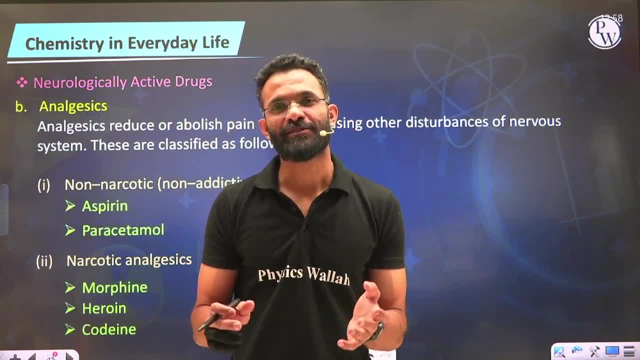 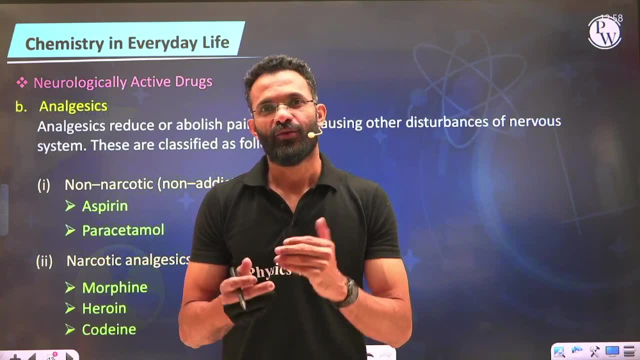 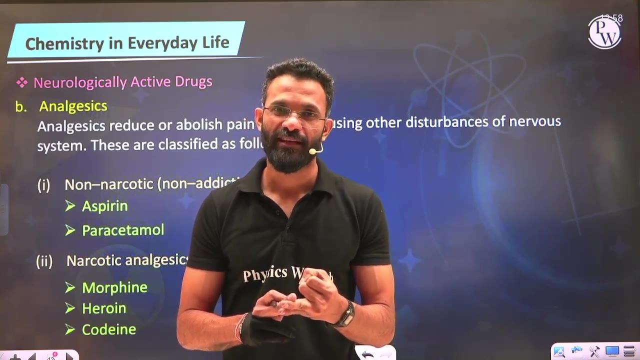 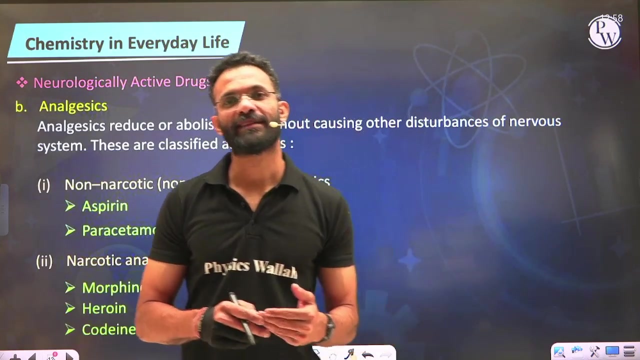 with antacids. so antacids basically are used to neutralize the excess of acidity, to example, which we saw. i repeat again, we discussed about bicarbonates, metal hydroxide, that is, mg, oh twice, aloh twice, and other than that we also studied ranitidine and simetidine. after that we came across uh medicines called as: 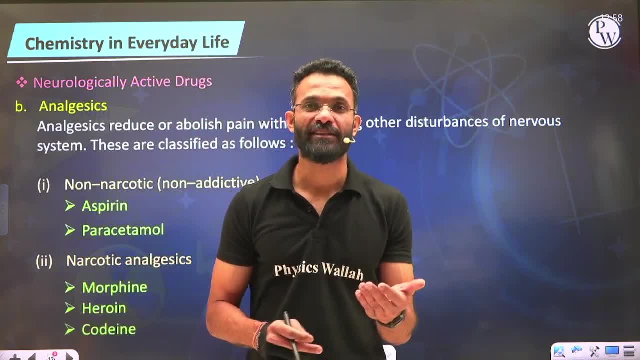 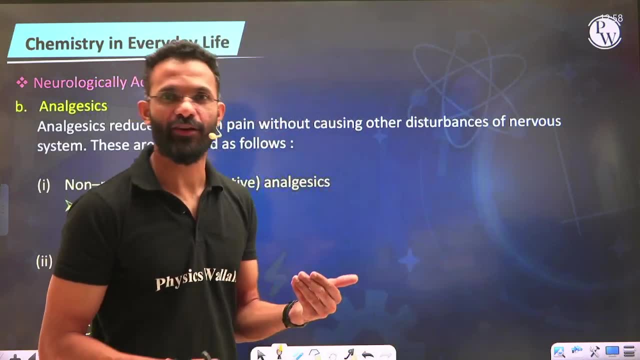 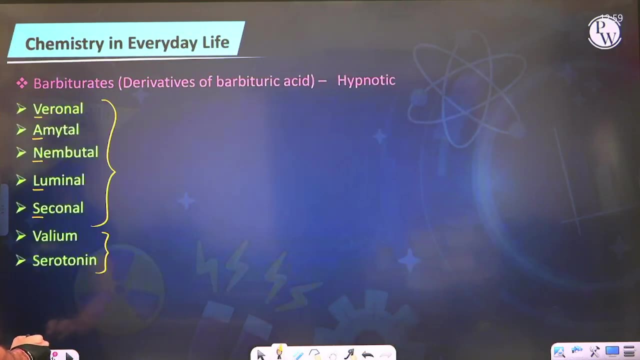 antihistamine. examples of antihistamine we came across were bromphenolamine- right, everyone. and then we studied another category of medicines, or a drug which is basically analgesics, before which we studied, yes, tranquilizers. these all are the example which come under category of 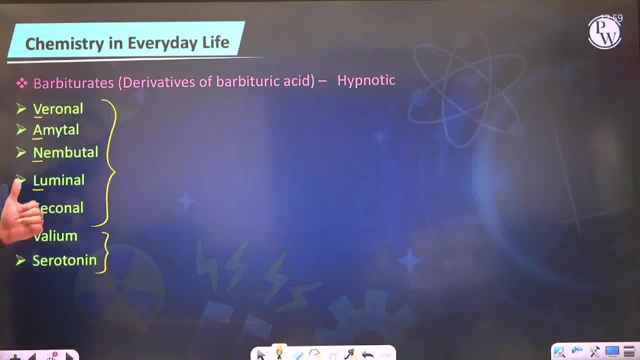 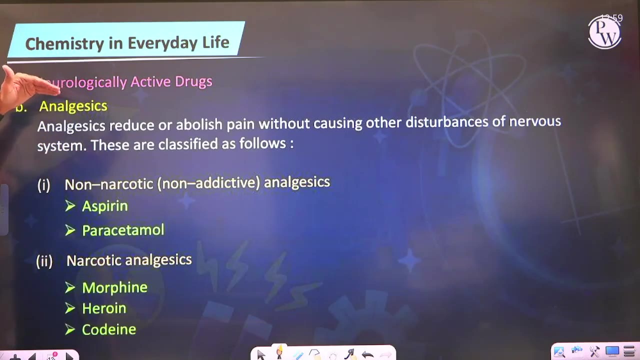 tranquilizer, then under the tranquilizer, we also studied the subtype that is called hypnotic or also called as barbuterase. we'll have to remember all these examples- followed by neurologically active drugs. the second category is analgesic. after tranquilizer, we are learning analgesic. 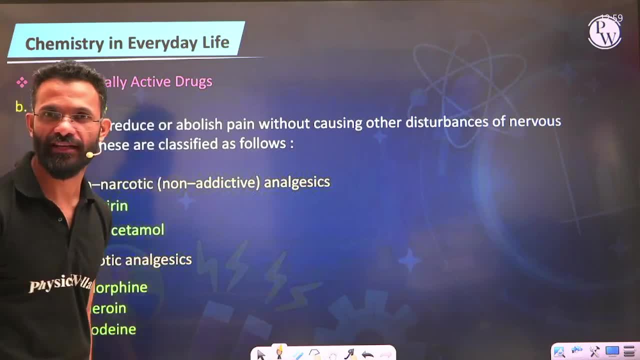 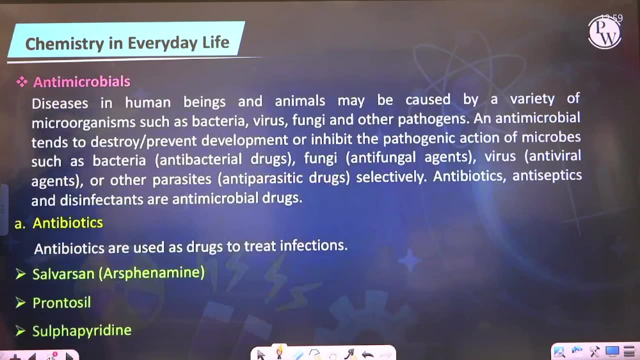 which are of two type: narcotic and non-narcotic analgesics. well guys, like i said right in the beginning, this is an informative chapter, so you'll have to remember lot many names of the drugs. the next category of a drug that we are learning is called: 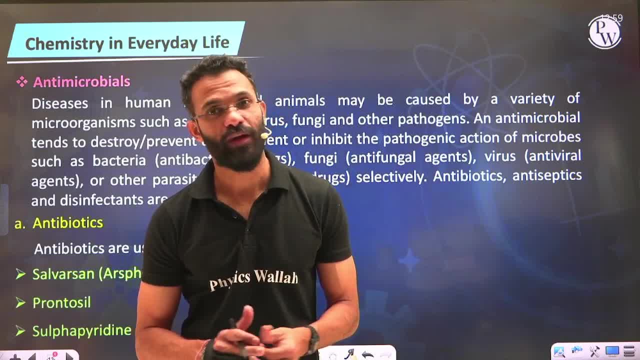 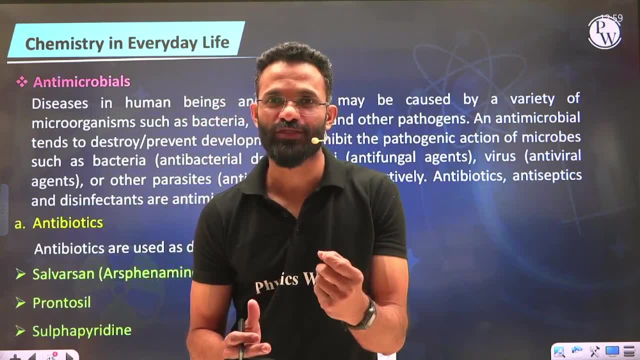 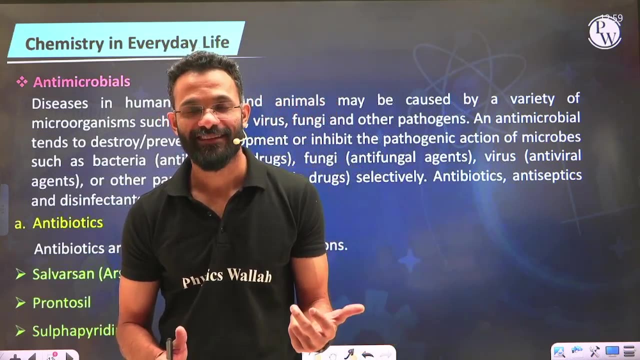 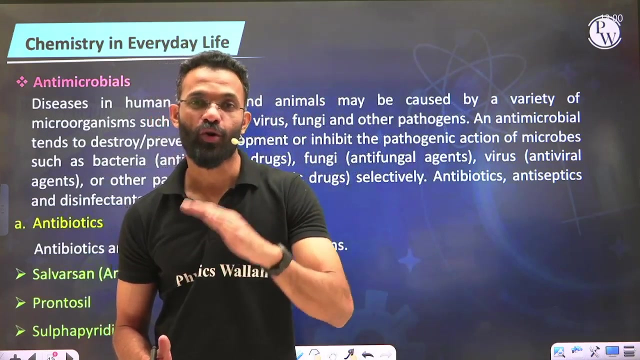 as antimicrobial agents. well, since we have recently come out of covid coronavirus, we know that how this pathogen, such as viruses, then uh, bacterias, can affect our body adversely. hence we need some medicines to treat them, either to stop the growth of such microbes or to kill such kind of microbes. 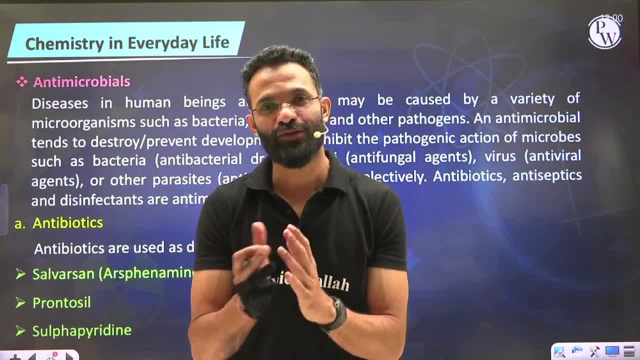 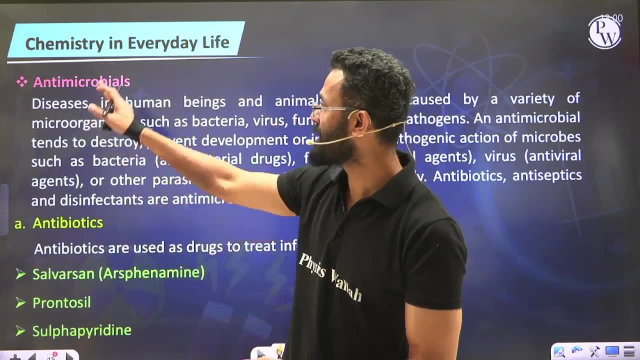 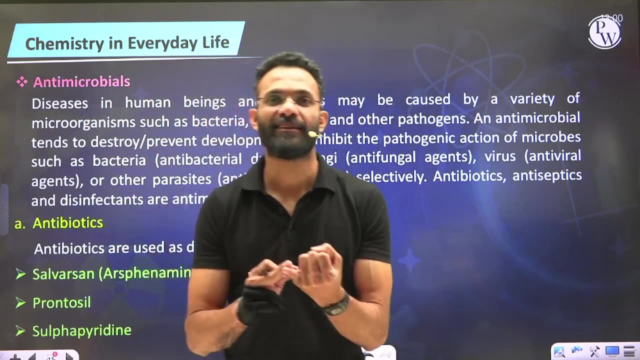 we need some medicines, those all medicines which are used to prevent the growth or kill those kind of microorganisms, is what you call it as antimicrobial. so antimicrobial are further of three category: one is antibiotic, second is antiseptic and third one is anti and antiseptic. 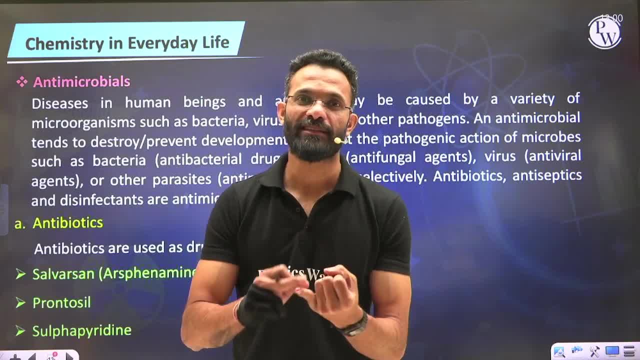 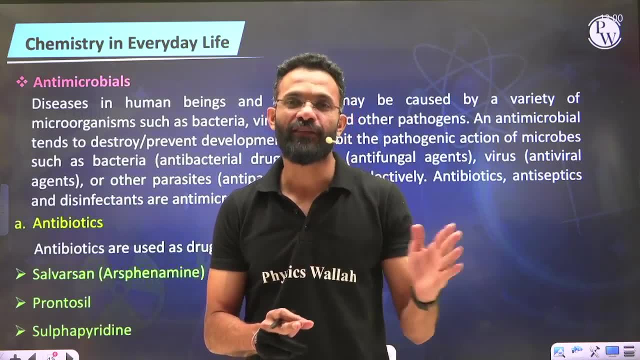 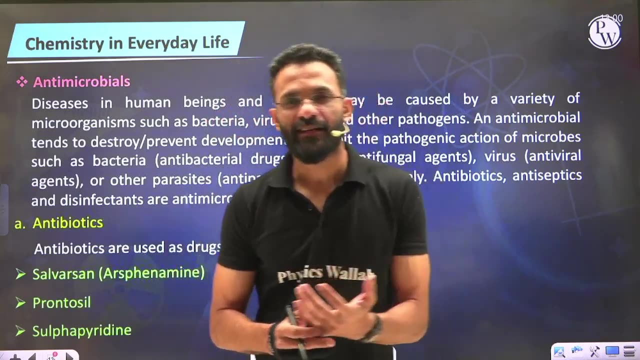 i'm sorry. uh, the first one is antibiotic, then antiseptic, and third one is disinfectant. now how does this three differs from each other? well, let's first talk about the antibiotic. just to give you an example, let's say we are experiencing a throat infection. 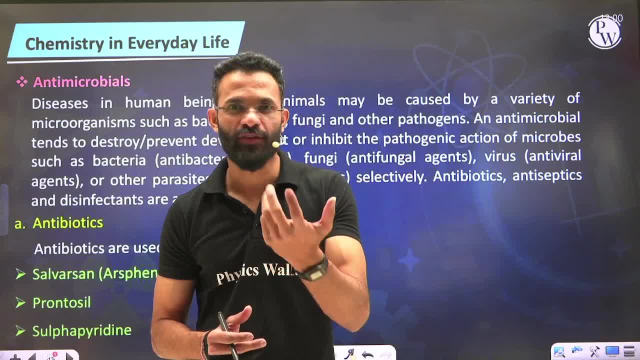 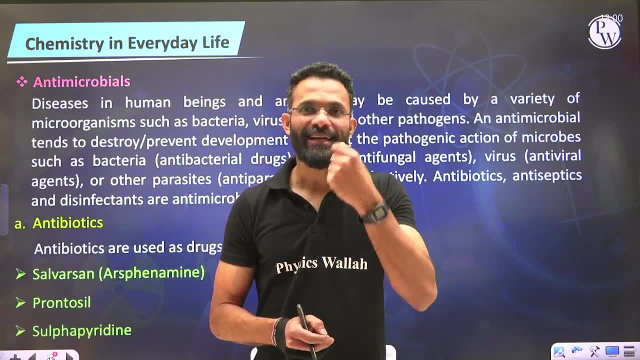 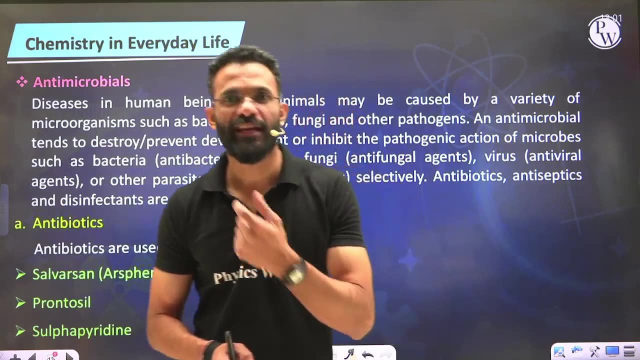 so we go to the doctor and doctor prescribes medicine. one of the common medicine doctor prescribed is erythromycin or azithromycin, right, so we have to eat that tablets. so after eating that, active pharmaceutical ingredients act upon the infection or the bacteria which are causing that infection, and then we start feeling better. 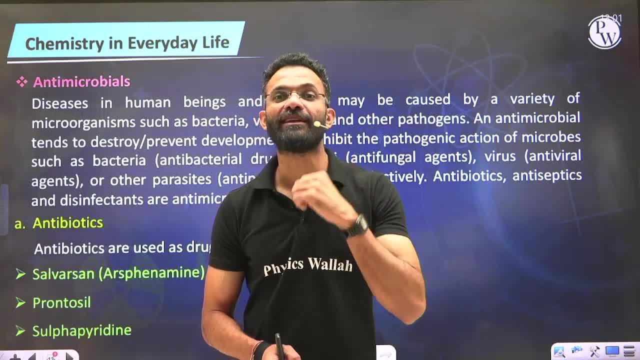 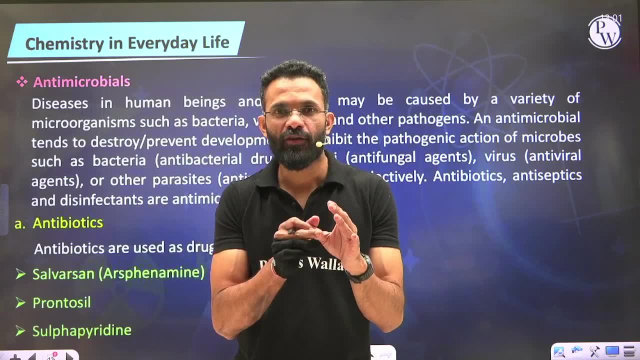 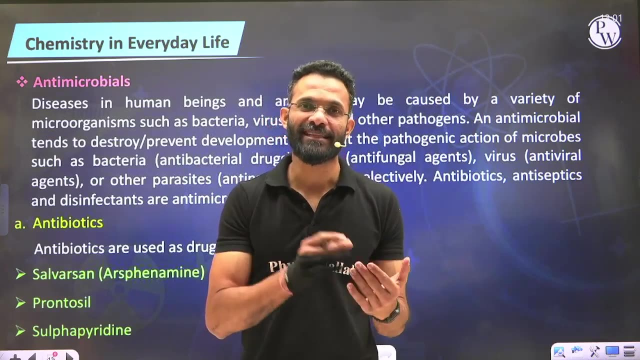 so, basically, antibiotics are the medicine which we eat. again, a particular type of antibiotic that we eat need not be applicable for all the infections that we are experiencing, so there is a type of antibiotic that we eat. let's understand what are the different types of antibiotics. one type of antibiotics are the one 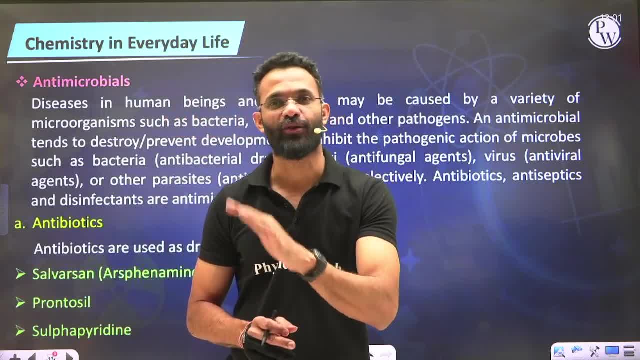 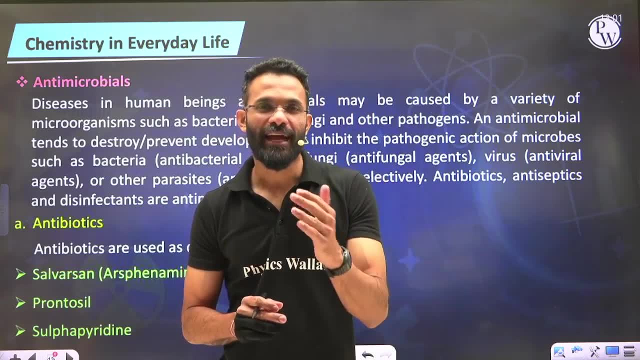 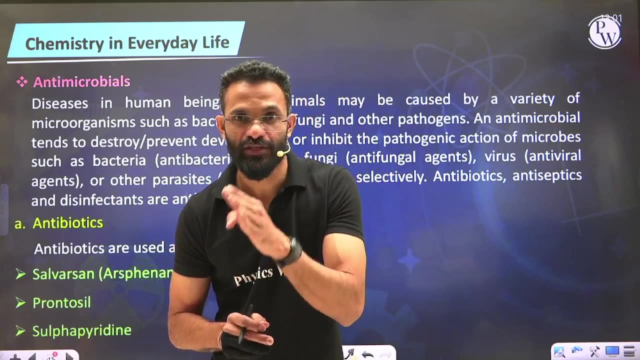 which basically stops the growth of microorganism, whereas second types of antibiotics are the one which kills the microorganism. so those antibiotic which stops the growth of microorganism- we call them as bacteriostatic- which stops the growth of bacterias, and the second type, which kills the 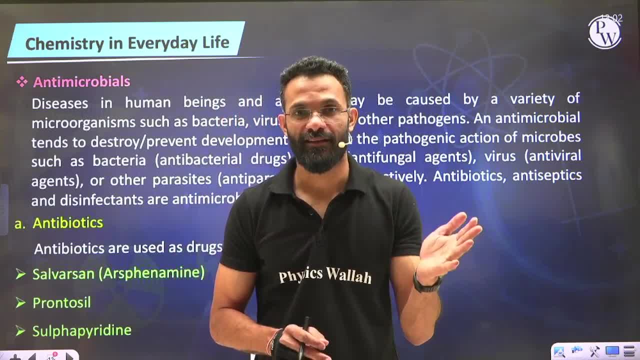 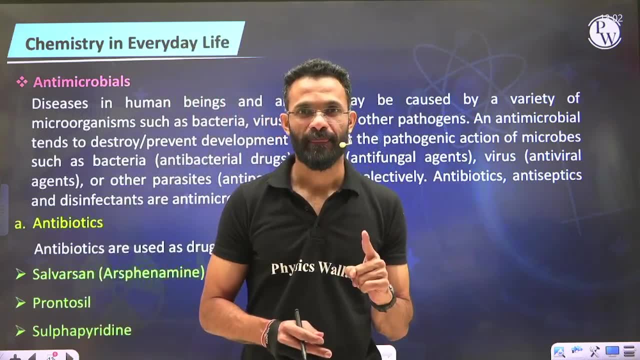 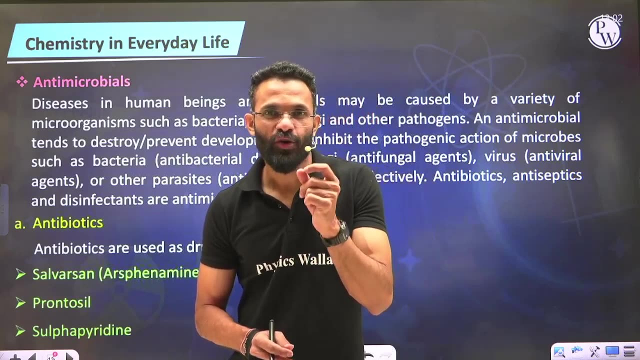 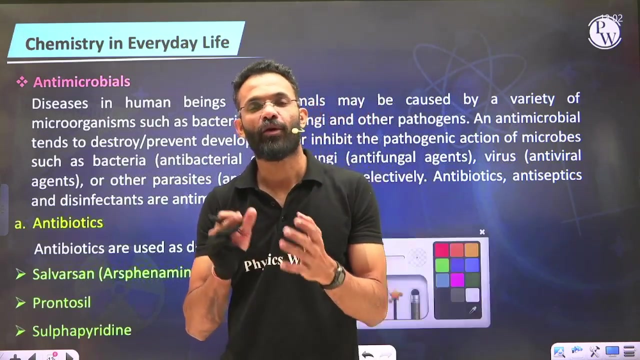 bacterias is called as bactericidal. bactericidal means those are the medicine which are going to kill the bacterias. this is the first classification. then the second classification of antibiotic is based on which particular type of bacterias that particular medicine can treat. so we classify them as broad spectrum antibiotic and narrow spectrum antibiotic. 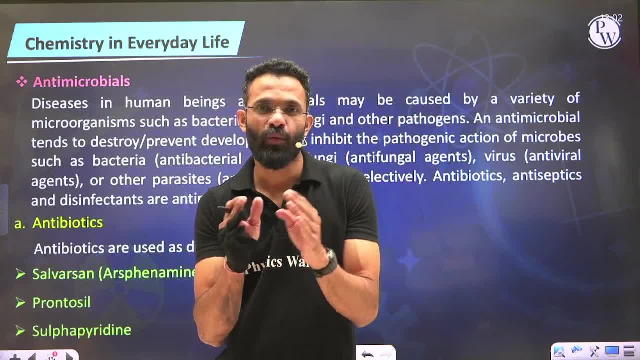 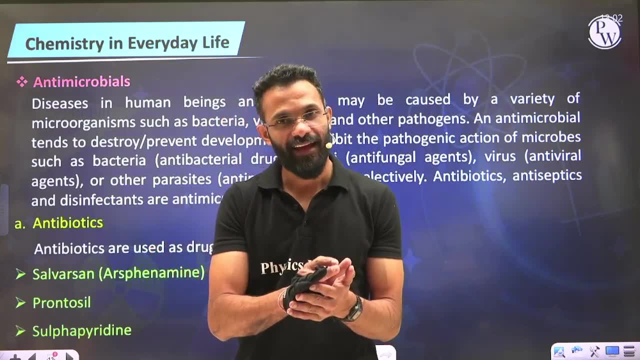 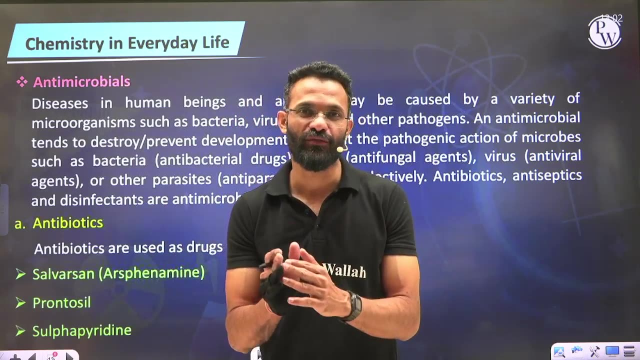 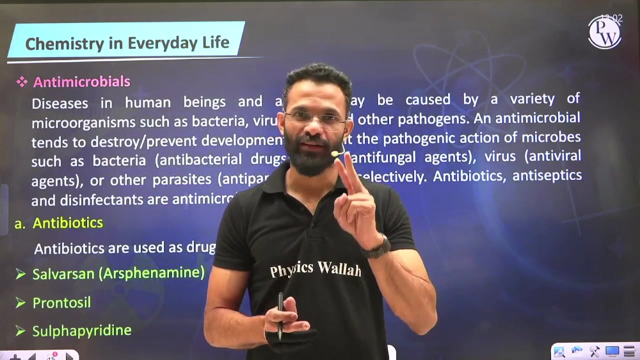 so broad spectrum antibiotics are the one which are used to treat against gram positive as well as gram negative bacterias, and the narrow spectrum antibiotics are the one which are used to treat against either gram positive or gram negative bacterias. so, guys, antibiotic can be classified in two categories. number one: bacteriostatic, bactericidal. number two, broad spectrum. 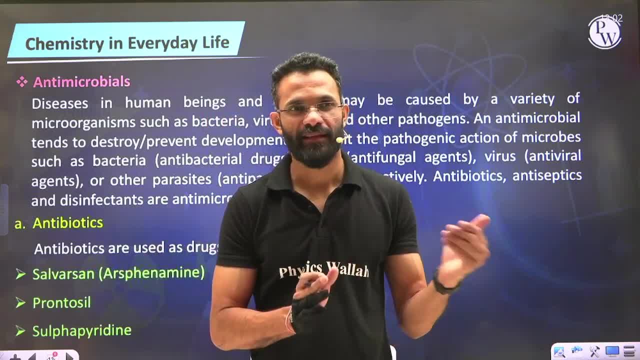 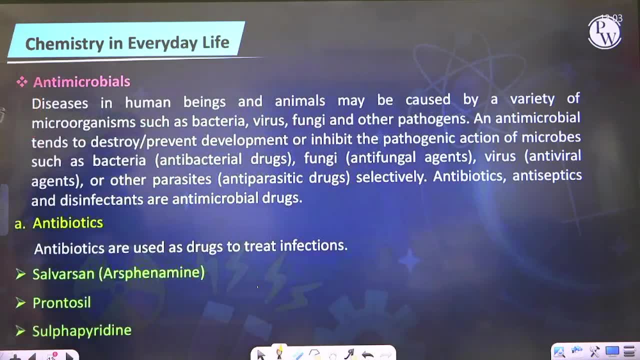 antibiotic- narrow spectrum antibiotic- and there are some specific spectrum antibiotic as well, but we need not look into it as of now. so yes, disease in the human beings and animals may be caused by varieties of microorganisms such as bacterias, virus, fungi and other pathogens. an antimicrobial 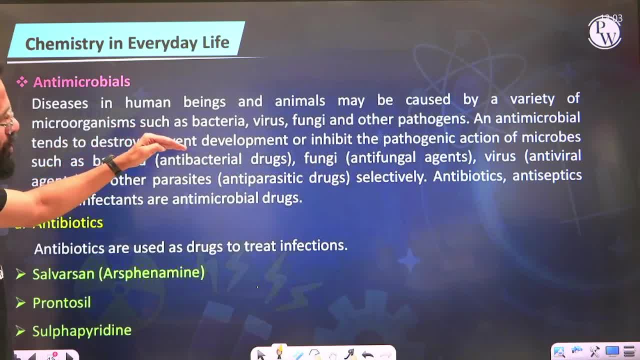 tends to destroy or prevent the growth or inhibit the pathogenic action of microbes, such as for treatment of bacteria. we use antibacterial agents to treat fungus. we use antifungal agents to treat virus, use anti viral agent and for other parasites selectively so. based on that, we classify this into 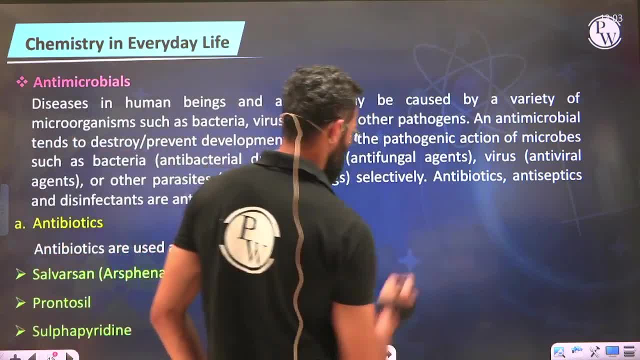 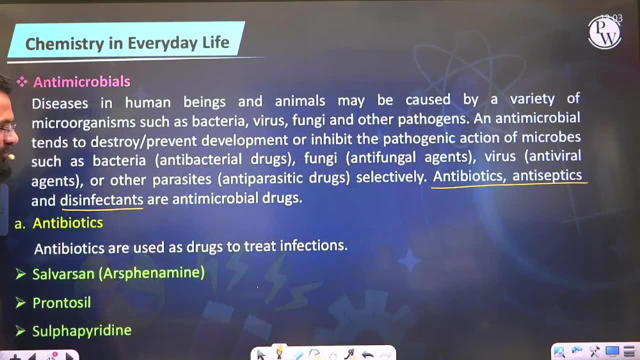 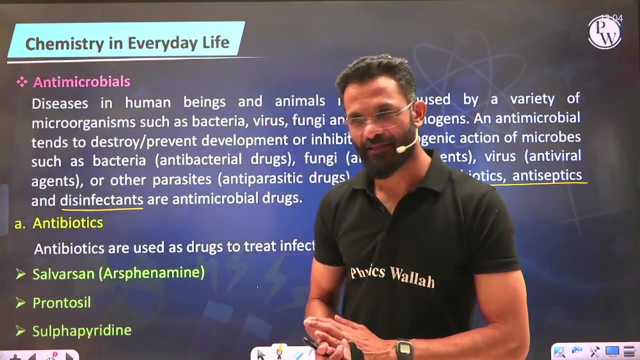 three categories- antibiotic, antiseptic and the third one is disinfector- are the three major categories of antimicrobial drugs. so first we're talking about antibiotic. well, so antibiotics are the drugs which are used to treat against the infection or which are used to treat the infections. well guys, if you just go back to the history of this, 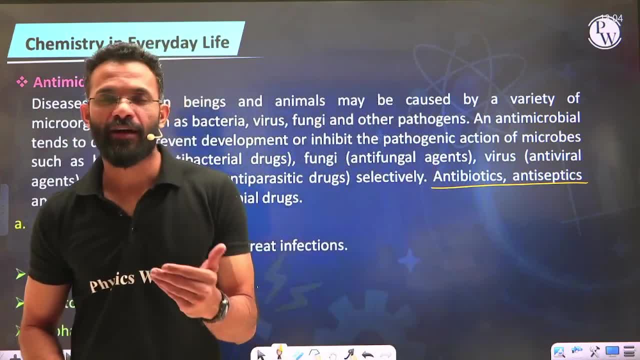 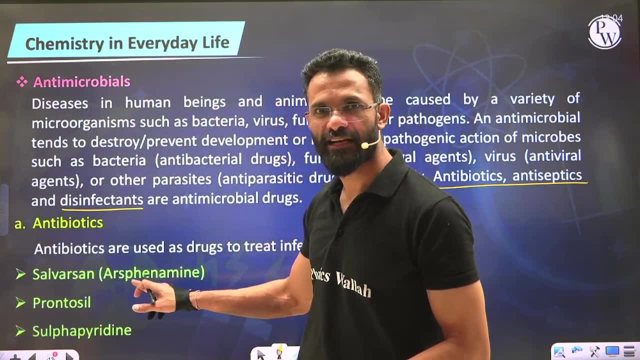 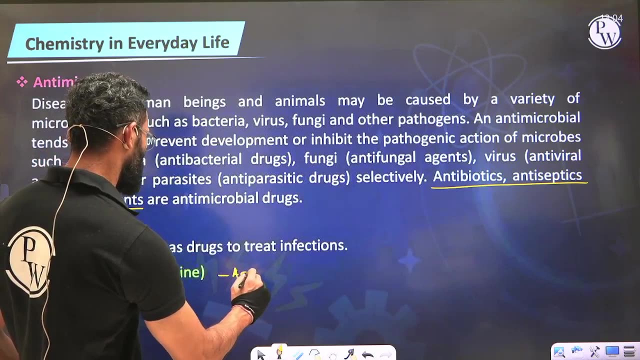 in earlier days when the antibiotic was developed. the first antibiotic which was developed was salverson, which is basically a compound which was containing arsenic, arsenic double bond. well, so arsenic is a nitrogen family member. so that drug was found to be containing arsenic, arsenic. 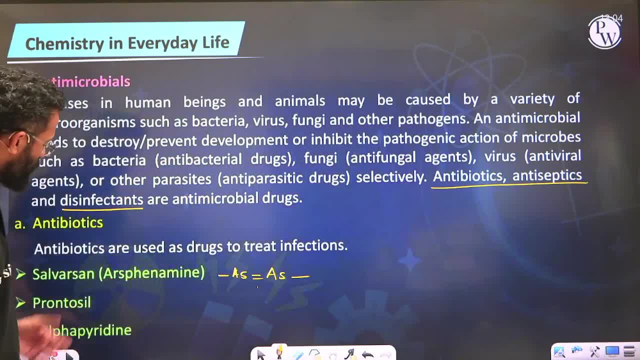 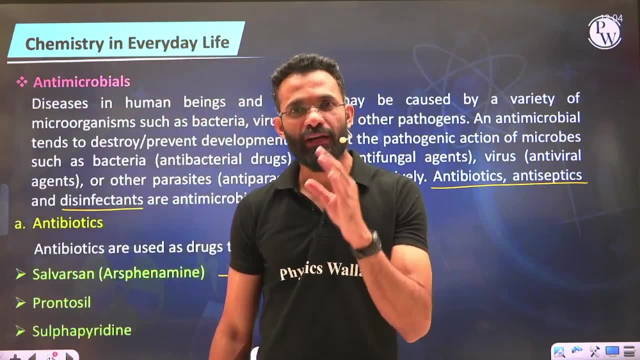 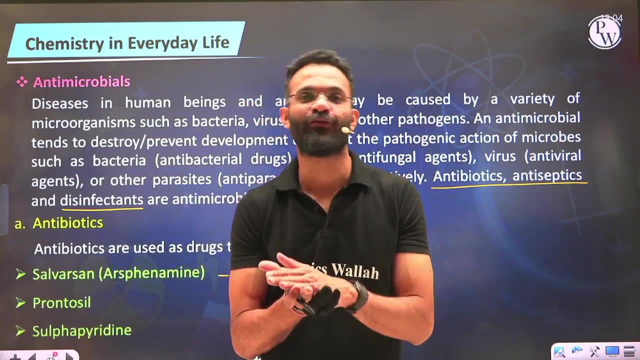 double bond, so you call it as arsphenamine, whereas it is essential that the antibiotic that we are consuming should only stop or kill the bacteria which is present on the host cell, but it should not have any harmful effect on the host cell or host tissue, for example. 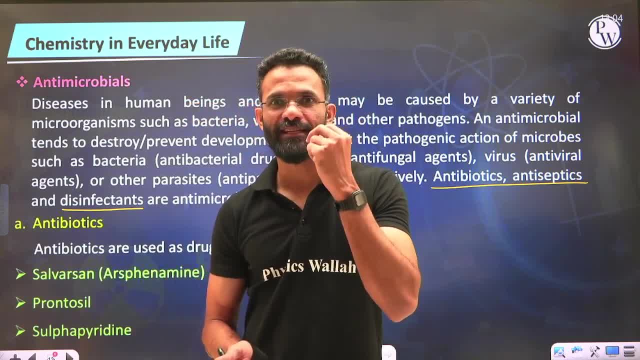 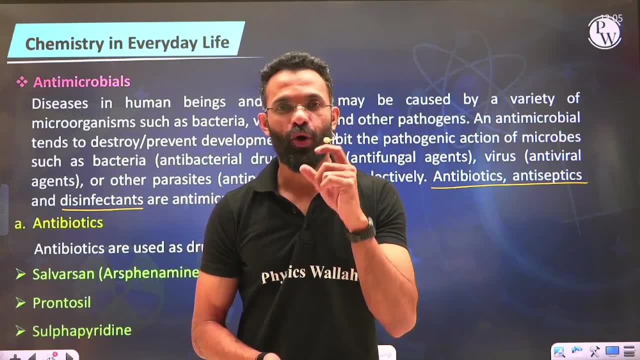 you If you are experiencing the throat infection and if you eat, let's say, erythromycin. that erythromycin should only kill the bacterias but should not have any harmful effect on the host tissue on which that bacterias have grown. 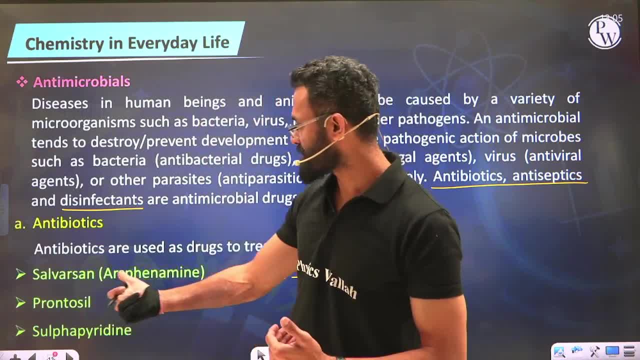 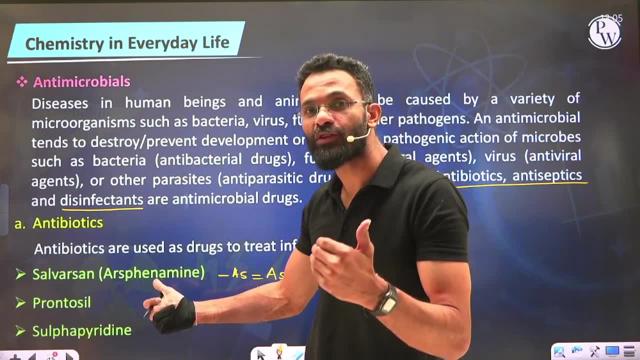 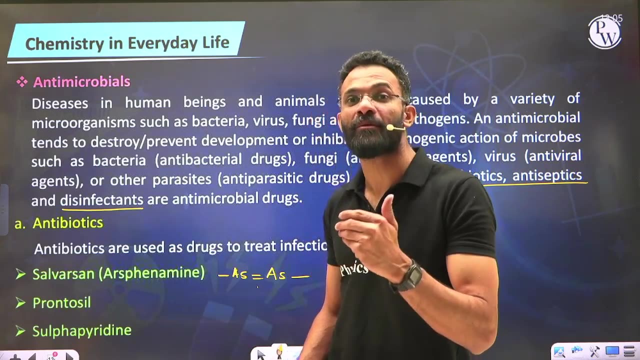 So in the old days, medicines such as salivarsan, which was discovered by the scientists, was effective against the bacteria, but it was also harmful to the human. But of course, the harmfulness to the human was relatively to a lesser extent as compared to its impact on the bacterias, and that's why it was continued. 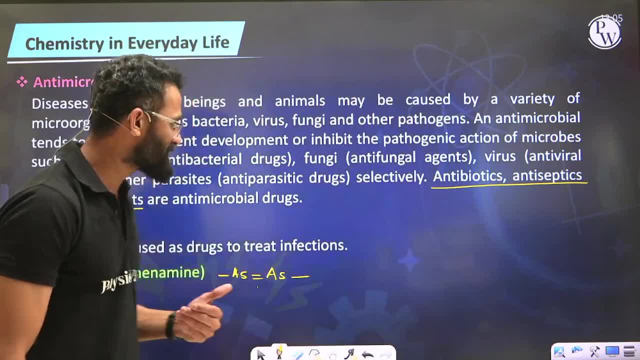 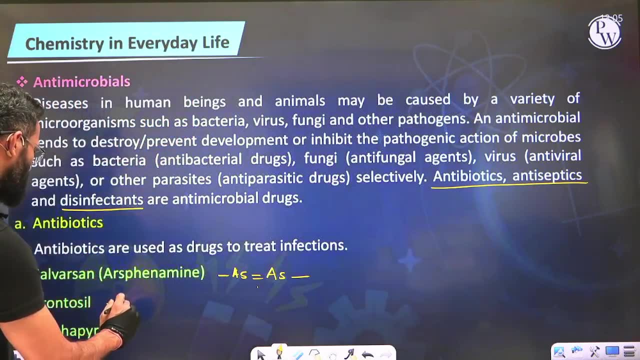 However, as the research went on, we realized that there is another medicine called prontosil, which is basically an azodi which contains nitrogen-nitrogen double bond, which was found to be as effective as salivarsan and found to be having less. 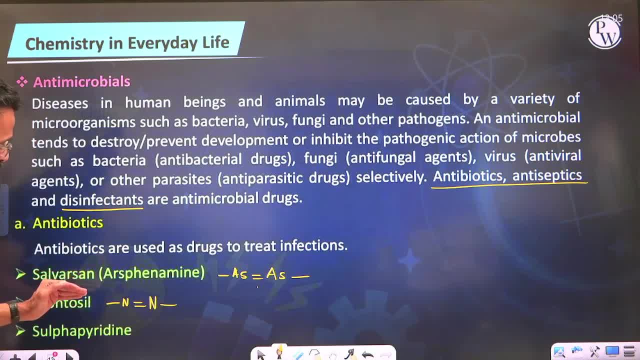 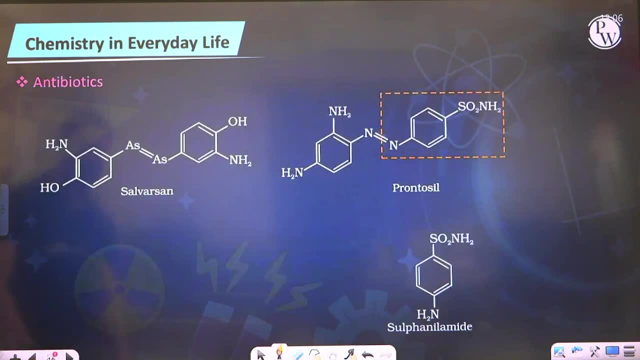 The effect or harmful effect on the living tissues was relatively lesser, so we started using the next medicine, that is, prontosil. Other than that, there is another drug which is used as antibiotic, called as sulfapyridin. Let me show you the structures of salivarsan and prontosil. 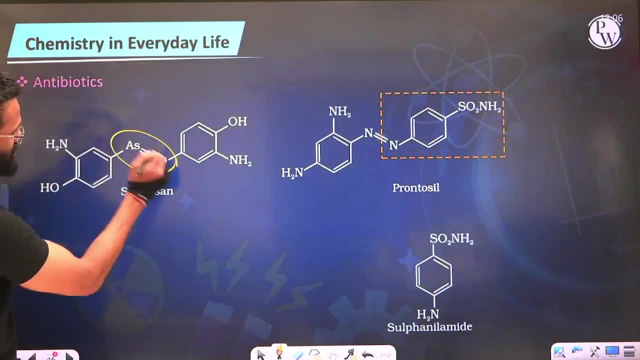 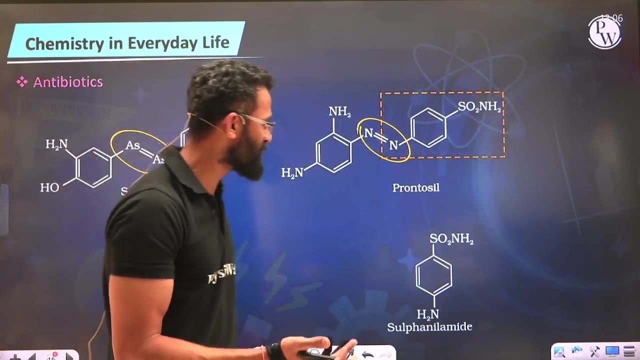 If you see here, this is salivarsan carrying arsenic-arsenic double bond. You are not supposed to remember the structure, but at least you need to know the data. This was the first antibiotic And similar to that, the other one which was discovered, which was even more effective, with the lesser side effects, was prontosil. 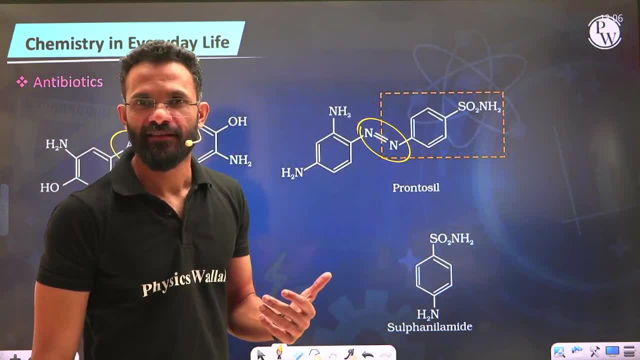 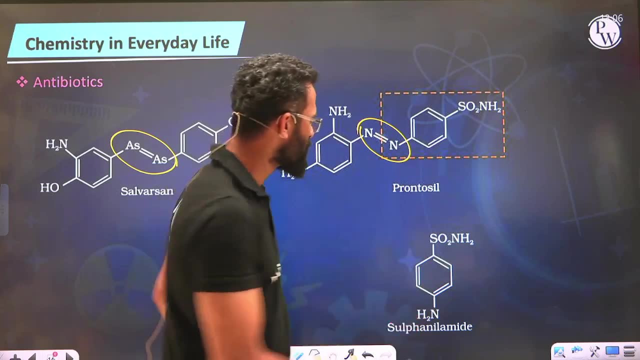 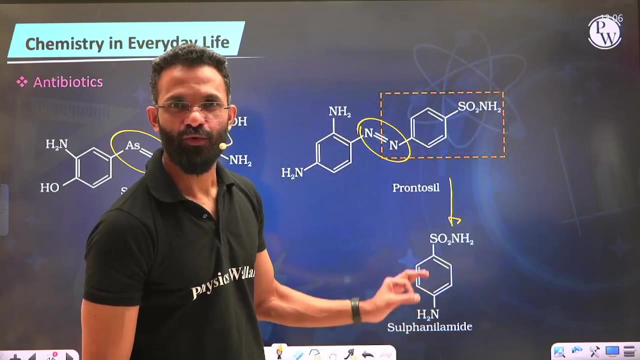 Well, there is one common question that they generally ask: When you actually eat prontosil in our biological system, it basically breaks down and releases the substance that is called as sulfanilamide- So the actual chemical substances, which acts like an antibiotic and functions against the bacterias. 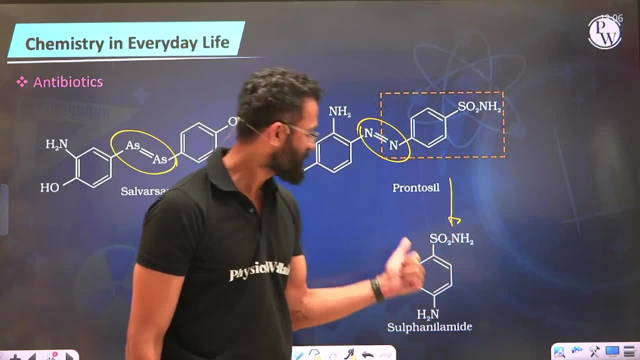 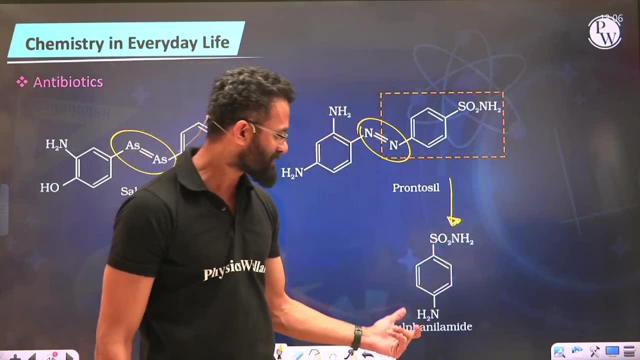 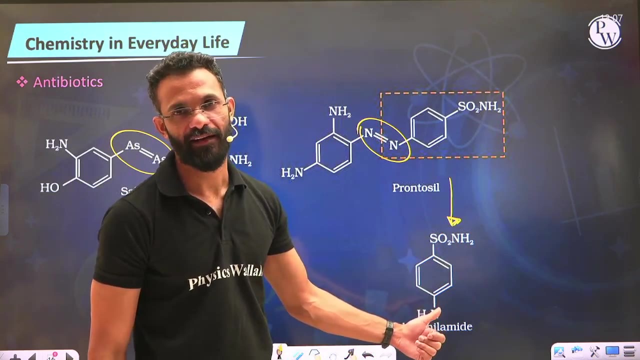 is your sulfanilamide. So remember, when prontosil is consumed it basically releases the chemical substances. which is actually effective against the bacterias is called sulfanilamide. So those were some of the examples of antibiotic. 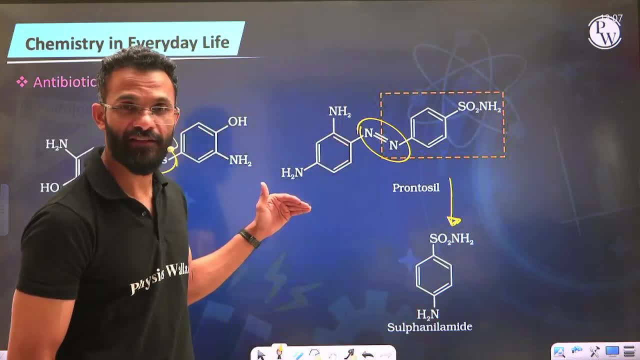 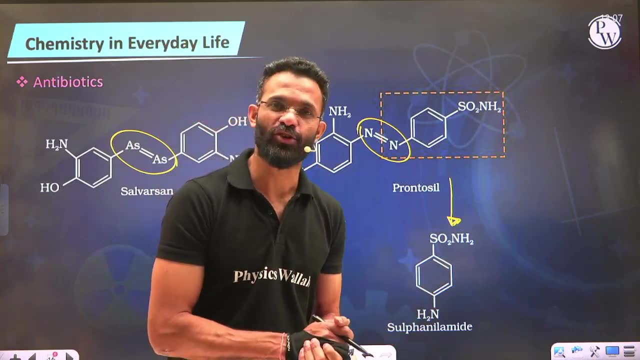 However, after this, after salivarsan and prontosil, so many synthetic antibiotic were developed. So let me show you. So let me show you the list of commonly used antibiotic and their categories. Guys, here is the list. 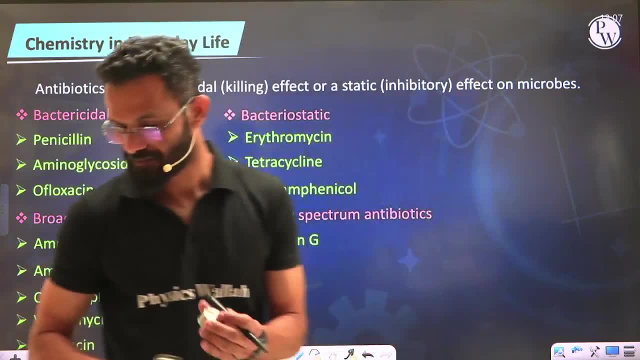 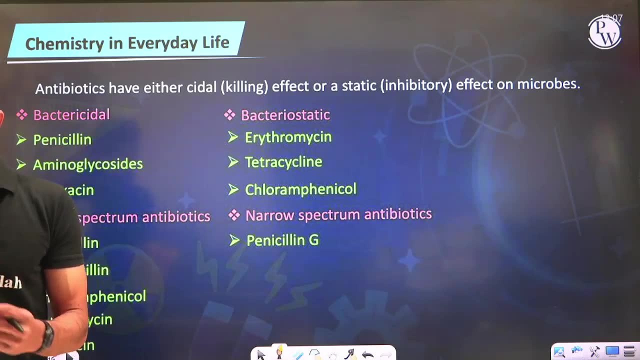 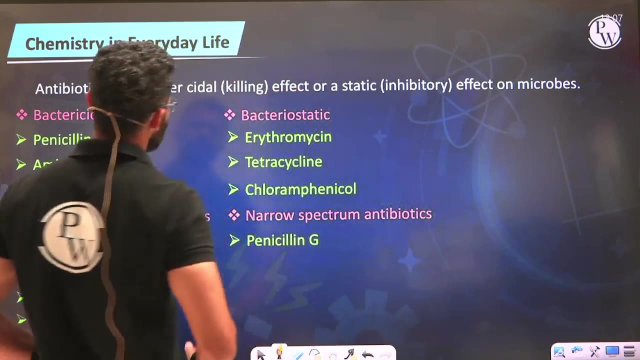 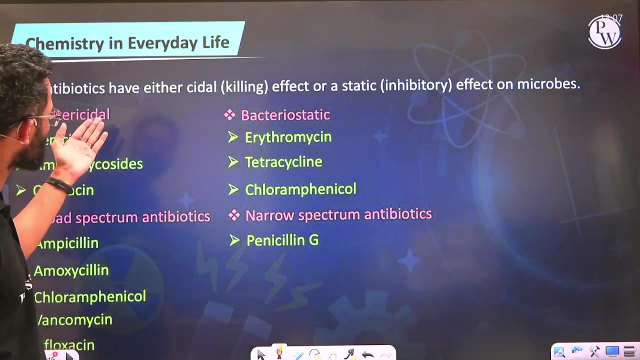 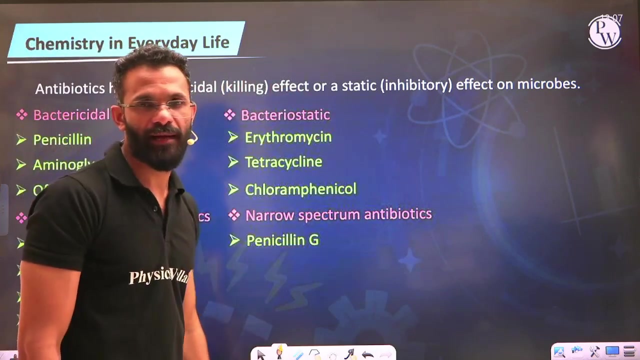 Hold on for a while. everyone, All right guys. So, like we said, antibiotics we classify in two ways. First way of classifying is bactericidal, which has the ability to kill the bacterias, and bacteriostatic, which basically stops the growth of the bacterias. 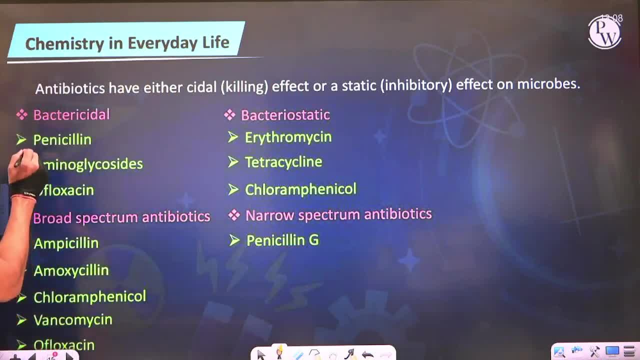 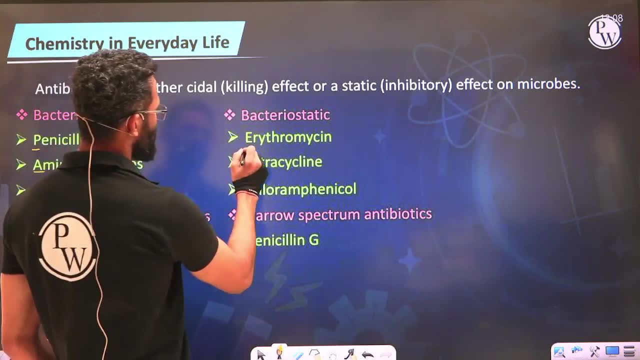 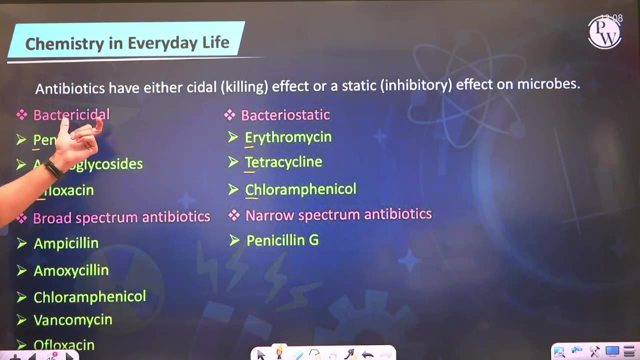 Some examples of bactericidal are penicillin, aminoglycoside and ofloxacin, whereas bacteriostatic are erythromycin, tetracycline and chloramphenicol. I repeat: bactericidal are the one which kills the bacterias. 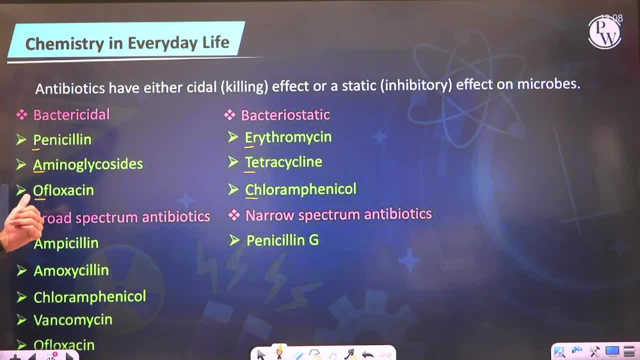 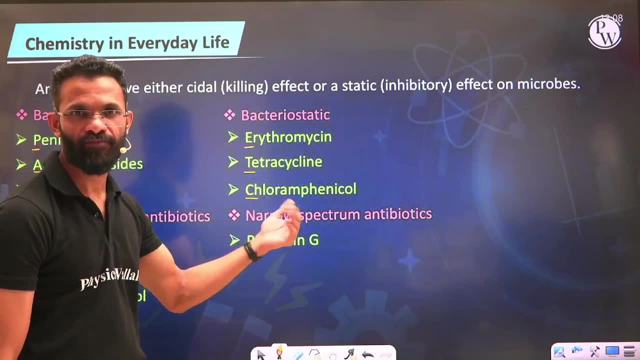 Examples are penicillin, aminoglycosides and ofloxacin, whereas bacteriostatic are erythromycin, tetracycline and chloramphenicol. Second way of classifying these medicines, or the antibiotic, are broad-spectrum antibiotic. 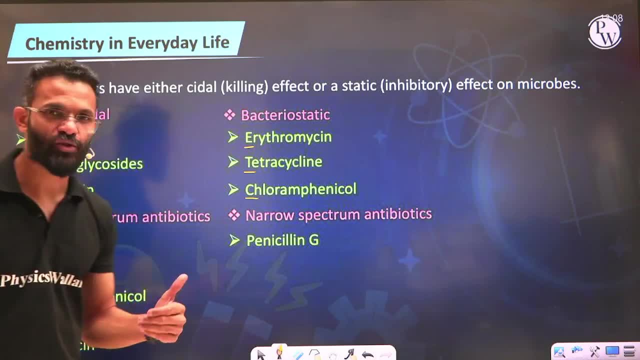 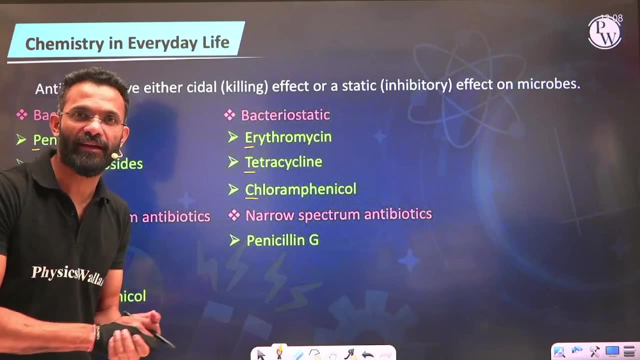 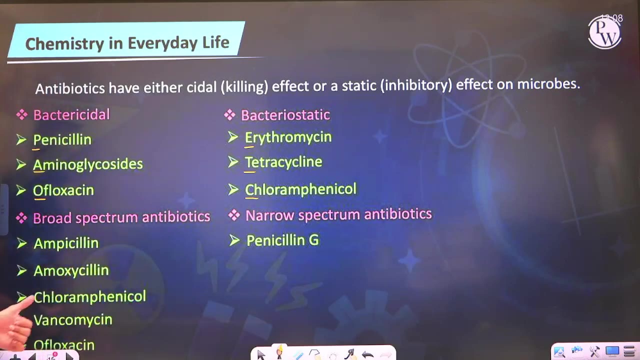 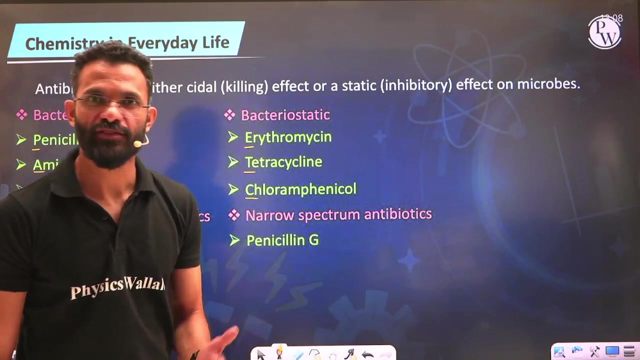 Like I said, broad-spectrum antibiotic are those antibiotic which functions against gram-positive as well as gram-negative bacterias, And the examples are ampicillin, amoxicillin, chloramphenicol, vancomycin and ofloxacin, Whereas narrow-spectrum antibiotics are the one which works. 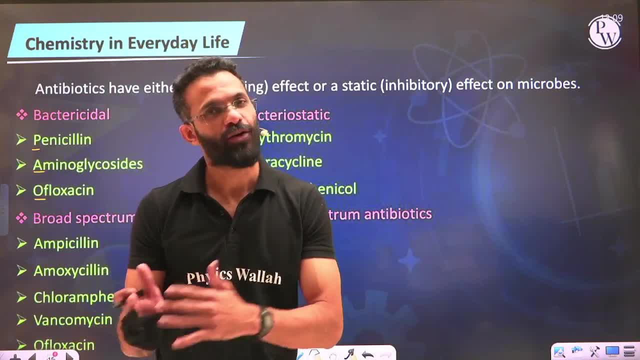 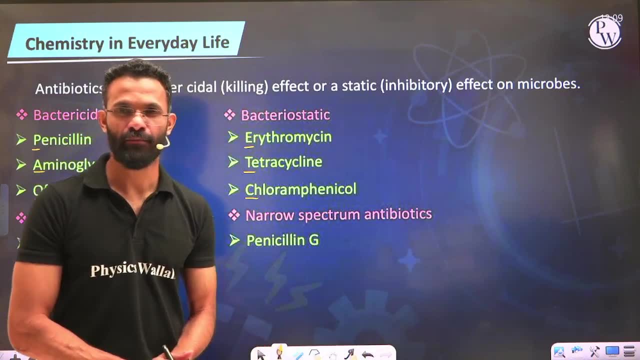 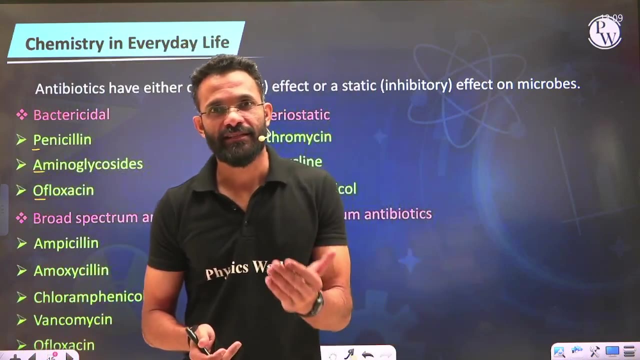 or which are effective against either gram-positive or gram-negative, And the example is penicillin G. That was all about antibiotic. Second category is what we call it as antiseptic. Well, as the name suggests, antiseptic, meaning again, it is going to function against the infection. 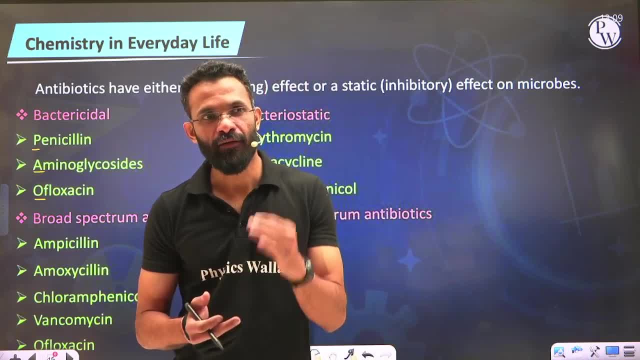 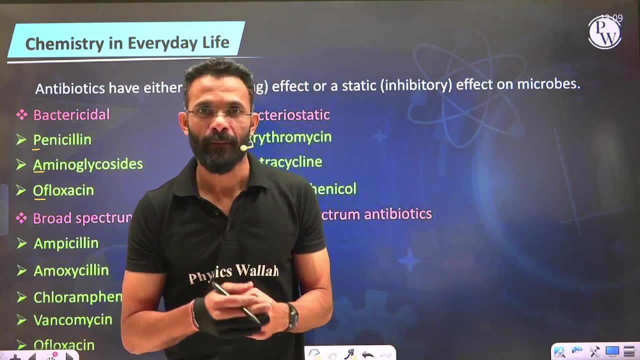 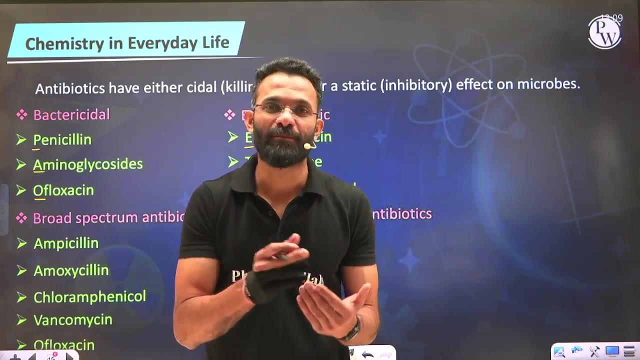 poison septic right. However, these are the medicine which we apply externally on the living tissues. For example, if we have got some wound, we put detol over it. So what is detol? Detol is antiseptic. 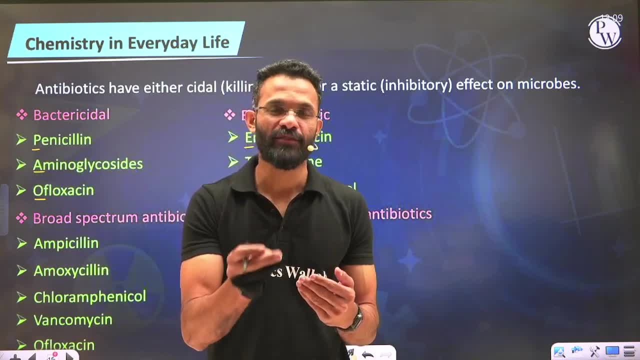 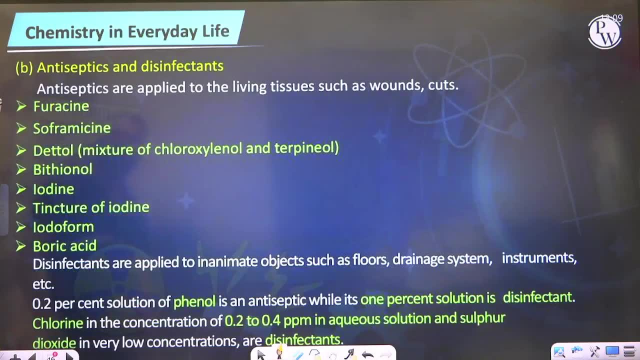 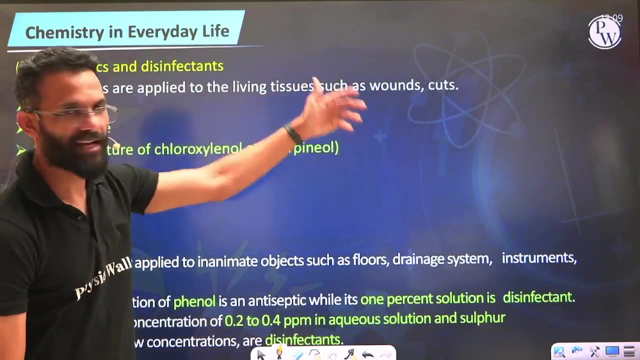 So detol is that chemical substance which we apply externally on the living tissues. So the second type of antimicrobial is antiseptic, And then the third one is disinfectant. So antiseptics are the ones which are applied to the living tissues, such as wounds and cuts. 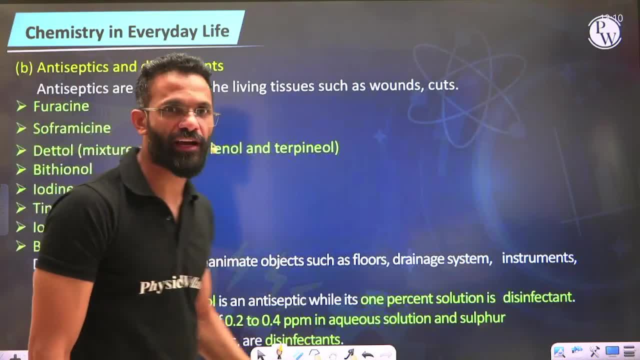 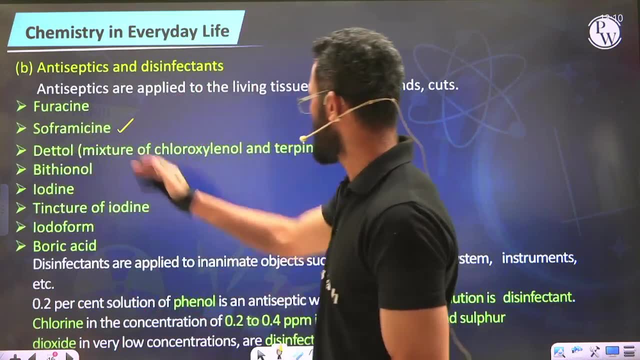 Examples. so many of these guys we have seen in our daily life as well. Puracin soframycin is one of the very common antiseptic Detol. Of course. with the structure of components of detol, it is mixture of chloroxylenol and terpineol. 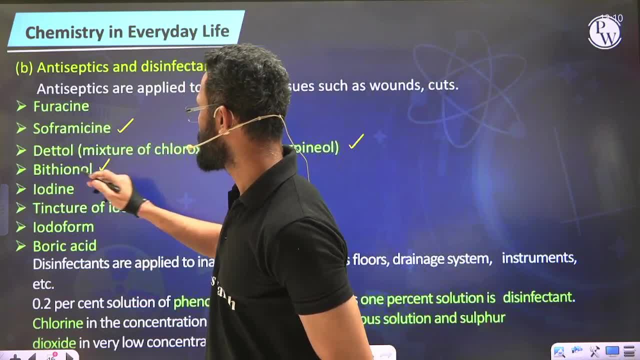 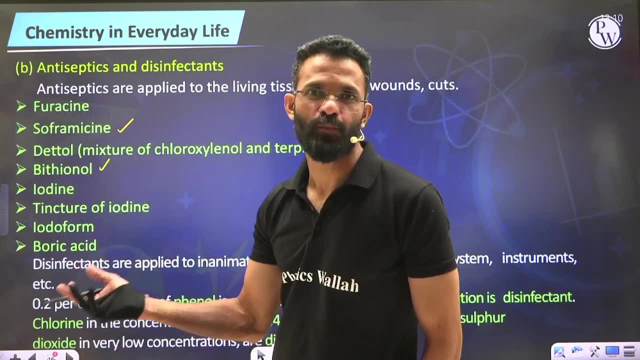 Then we have got bethionol. Well, bethionol or bethionol you can call it. This is that chemical substance or antiseptic which we generally found in soaps. Then we have got iodine, Then there is tincture, iodine and iodoform. 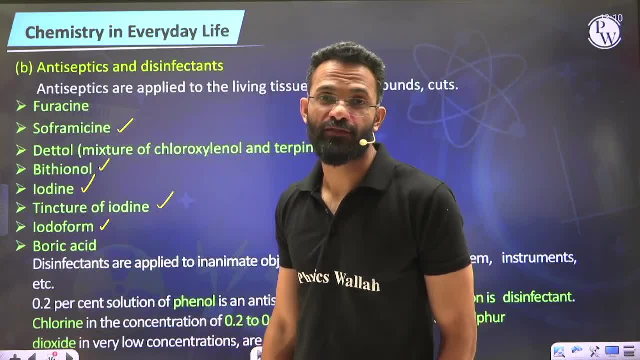 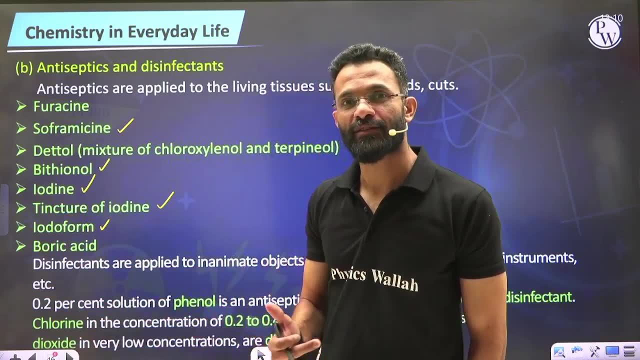 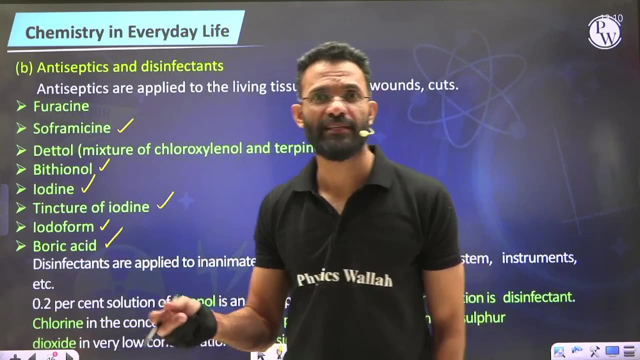 These three are the antiseptic because of the antiseptic ability of iodine And generally in the schools, you see, the antiseptic which is used is either of this. Then we have got boric acid. Boric acid is used as antiseptic very commonly in the eye drops. 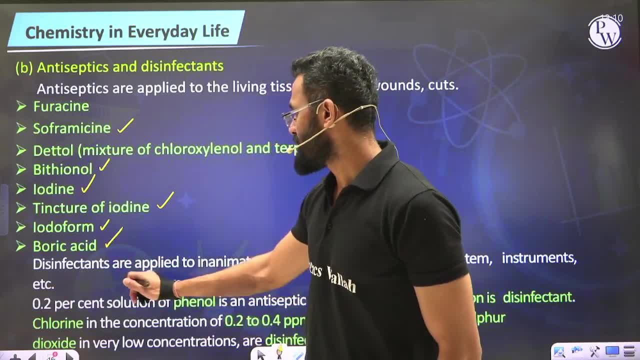 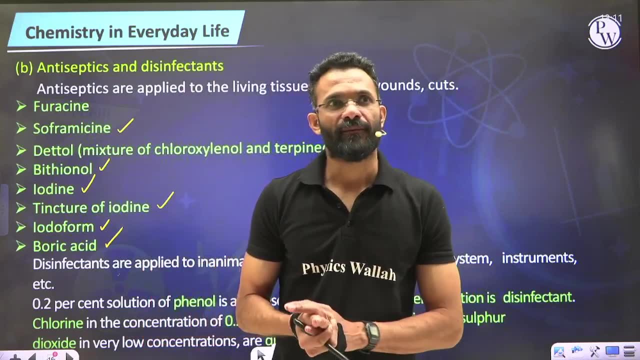 So that's boric acid. Disinfectant is the third category After antiseptic disinfectant. Well, guys, just to give you an example, In our house also, we use disinfectant, For example, whenever we have to clean the floors. 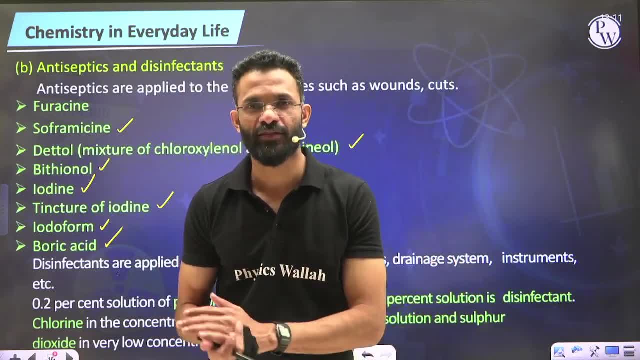 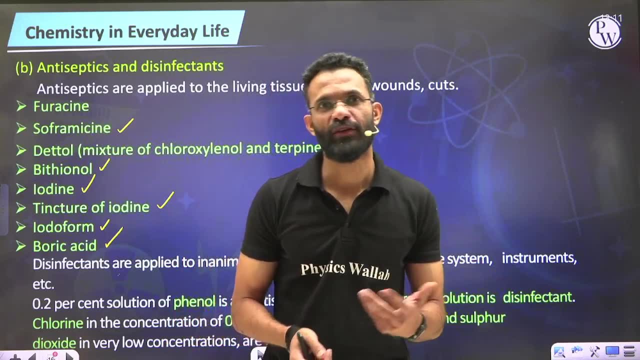 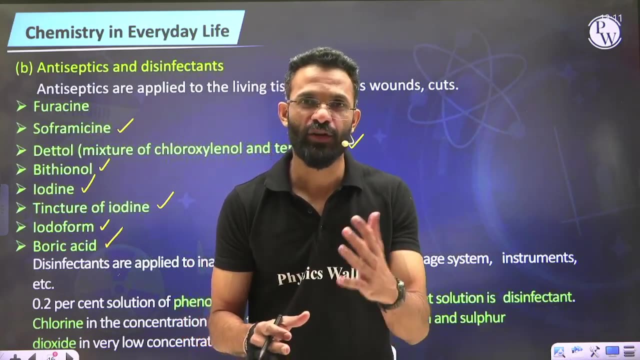 Or the surfaces of other tools such as table or whatever. So we use some cleaners. For example, we use, let's say, Lysol. Lysol is used as a floor cleaner- That is what we call it as disinfectant, which basically kills the microorganism. 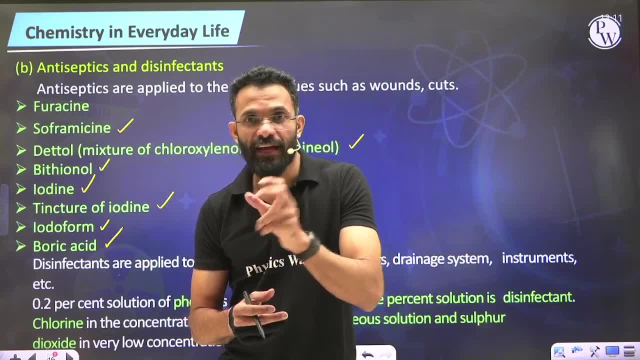 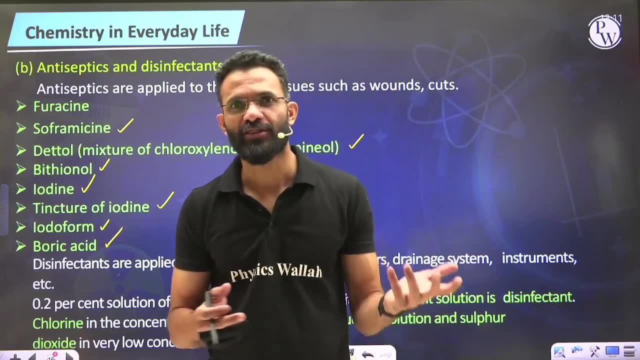 But understand the difference in antiseptic and disinfectant. Just to give an example, Let's say One fine day we are out of Lysol. We don't have a Lysol at home But we have got a Dettol. 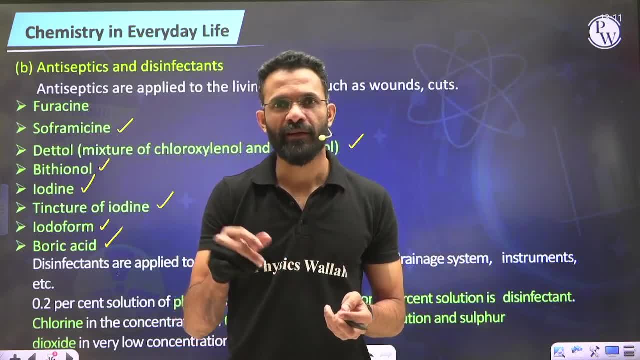 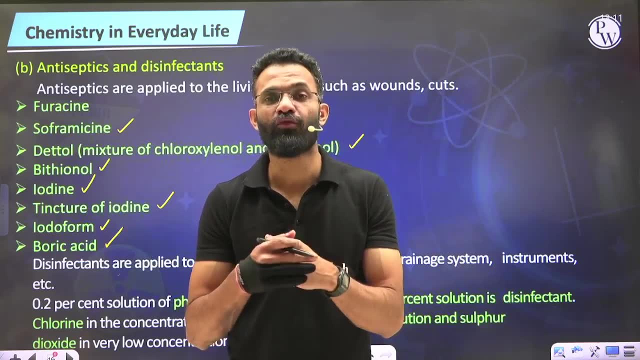 So what we do? We take a Dettol, We put it in a water, We make a solution And we clean the floor, Correct. The same Dettol is used for cleaning the wounds as well, So Dettol is used as an antiseptic. 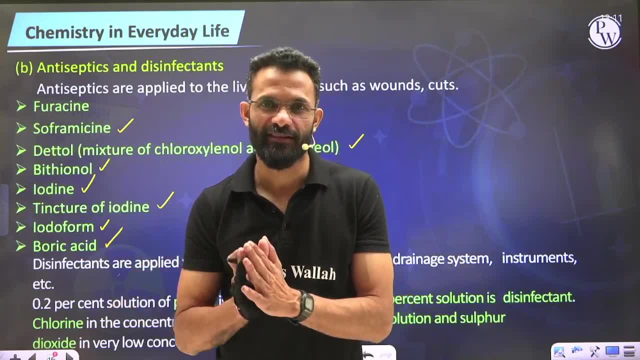 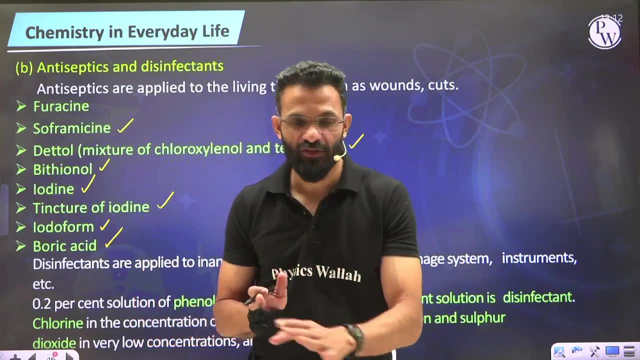 And at times we also use it as a disinfectant. Now see, Imagine one fine day we don't have Dettol, But we have got Lysol- The same Lysol which we use for cleaning the floors, Correct? 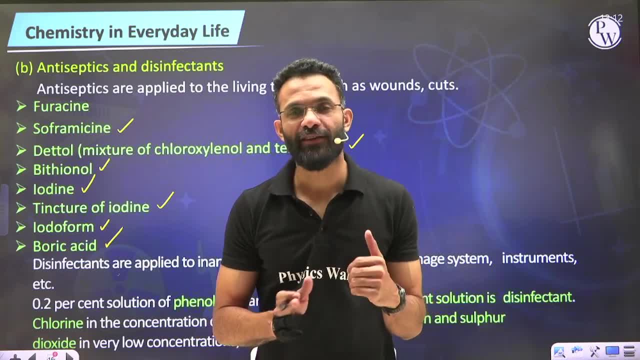 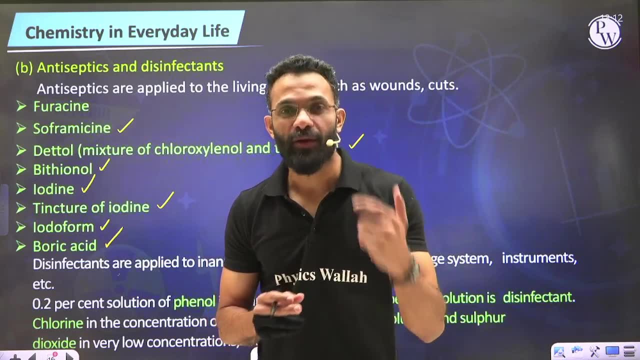 Tell me one fine day, if we have got some wound, Will we be able to apply Lysol over there? We cannot Why? Because Lysol, which is disinfectant. It is harmful to the living tissues, So we cannot use it. 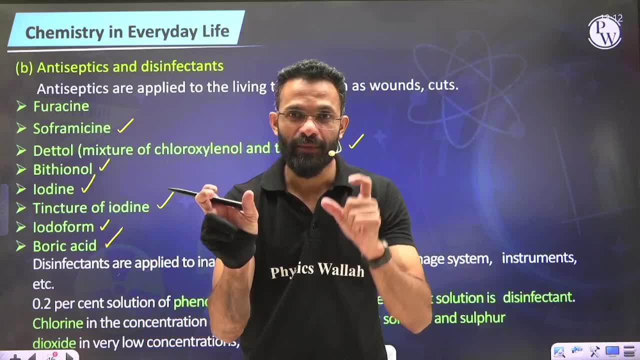 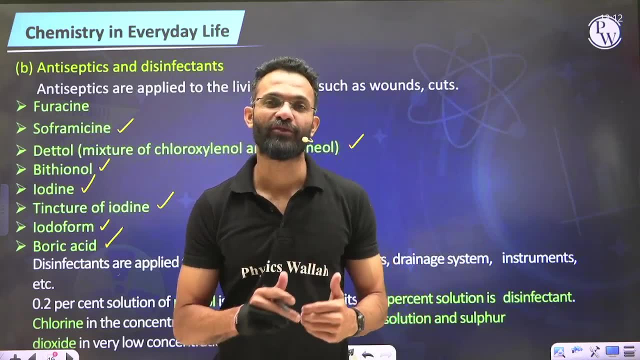 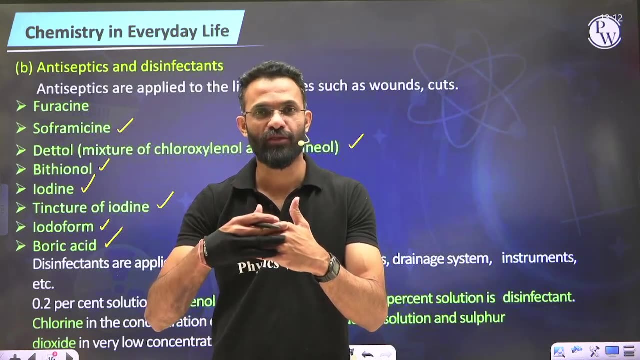 So the difference in antiseptic and disinfectant lies on, first of all, the concentration And the second, whether or not it is harmful to the living tissues. So antiseptic and disinfectant, Antiseptic, are applied on the living tissues over the cuts or the wounds, because they are not harmful to the living tissues. 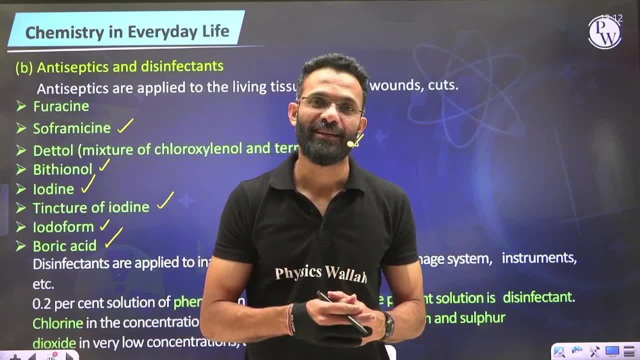 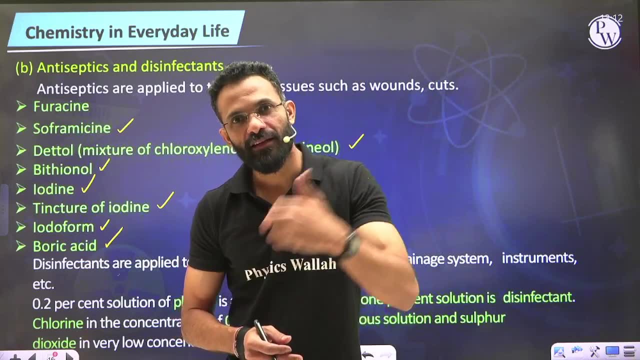 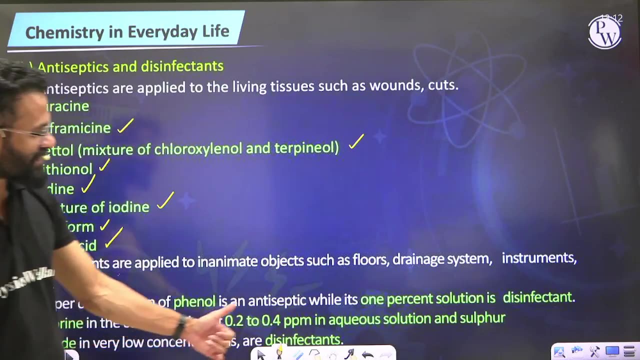 Whereas disinfectant are harmful to the living tissues. So several times you will find some of the compounds in a lower concentration are used as antiseptic. In higher concentration they are used as disinfectant, Such as phenol. 0.2% solution of phenol is antiseptic. 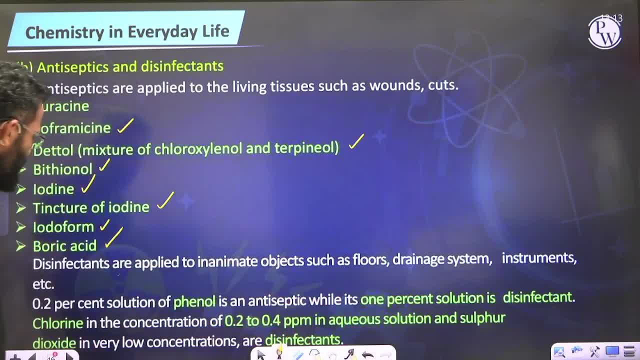 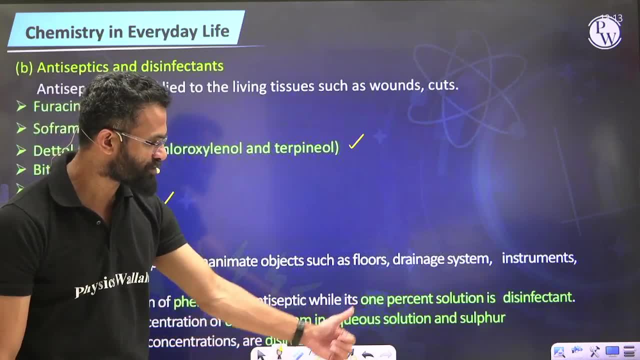 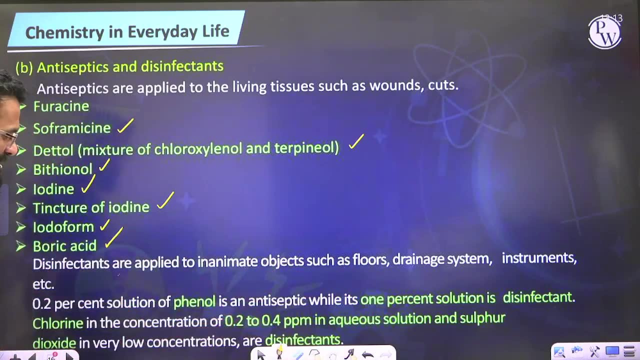 Whereas 1% solution of phenol is disinfectant. Similarly, chlorine in the concentration of 0.2 to 0.4 ppm in aqueous solution and also sulphur dioxide in a very low concentration are used as disinfectant. So you can remember this example. 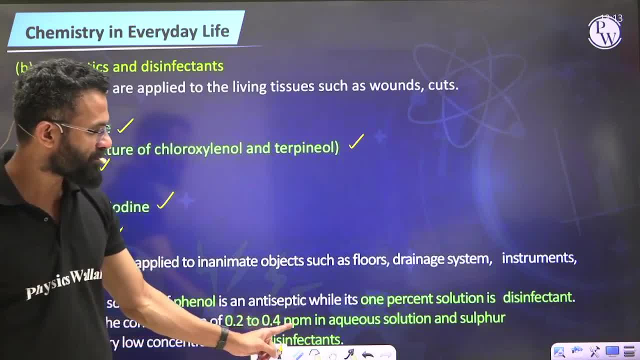 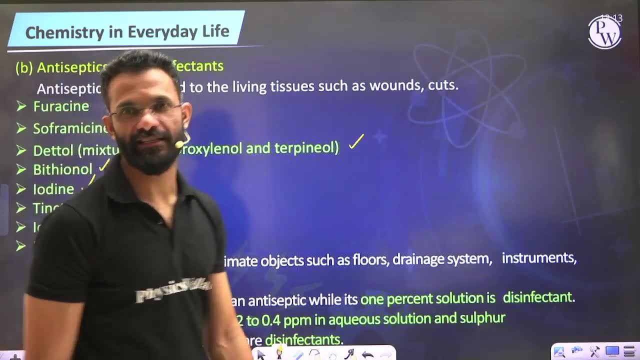 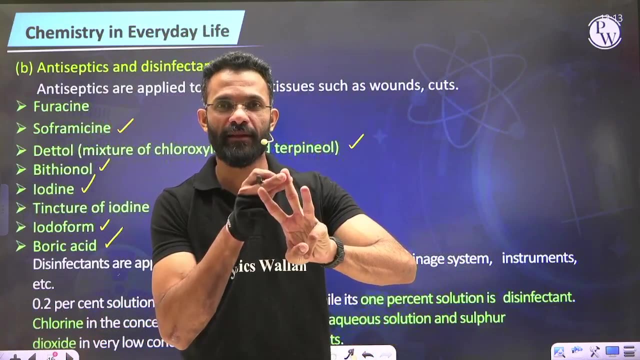 Phenol 1%, 0.2 to 0.4 ppm of a solution of chlorine and sulphur dioxide in lower concentration will be acting as a disinfectant. So, guys, antimicrobials. we studied three antimicrobials: Antibiotic, antiseptic and disinfectant. 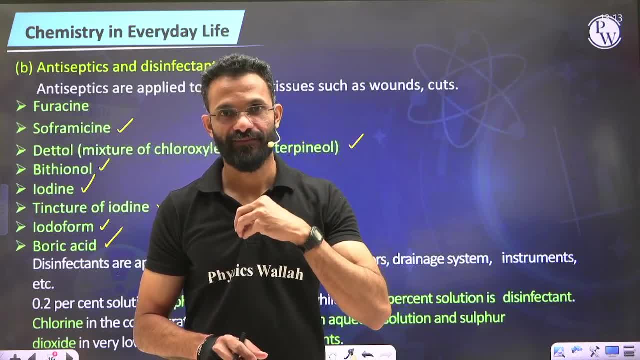 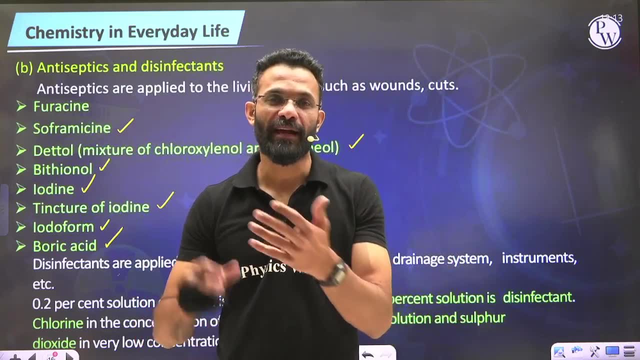 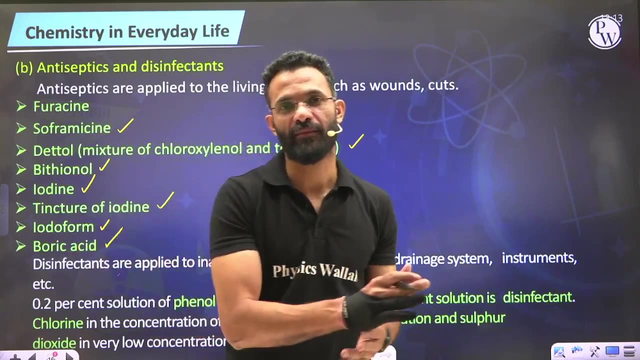 Antibiotic which we consume and internally they helps to get rid of those bacterias. Those antibiotic could be bacteriostatic or bactericidal, And they can also be classified as broad spectrum and narrow spectrum antibiotic, Whereas antiseptics are the one which we apply on the living tissues over cuts or the wounds. 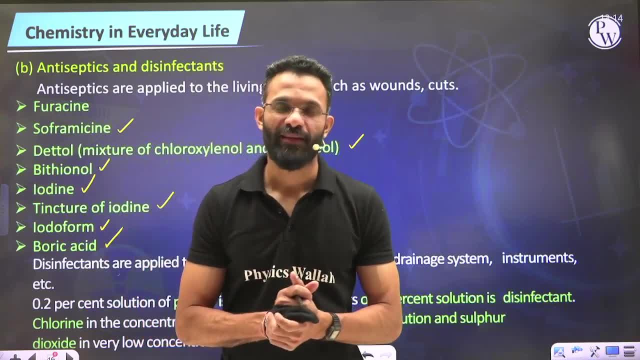 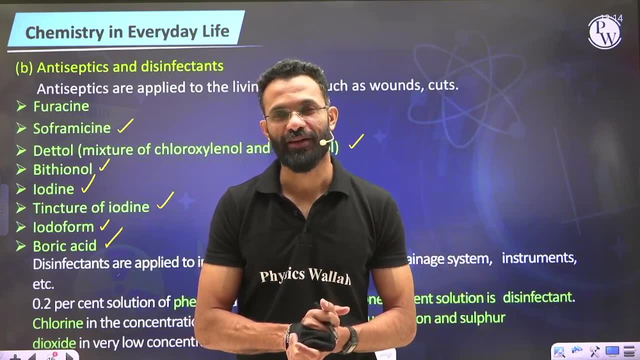 That kills the growth of microorganism, Whereas disinfectants are the one which we generally use to clean the surfaces, basically, And they also kills the growth of microorganism. So that was about the antimicrobials. So, guys, what all category of medicine that we have come across. 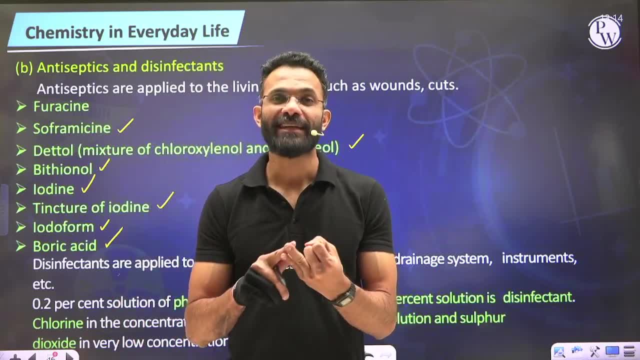 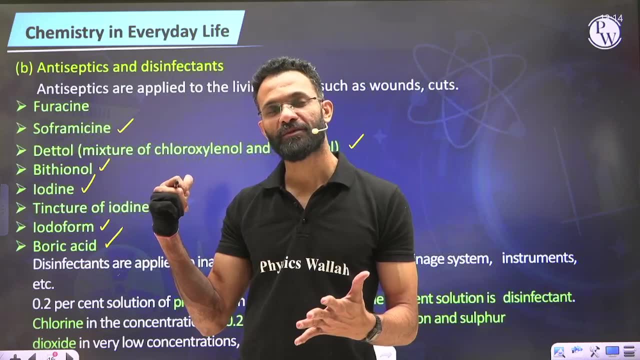 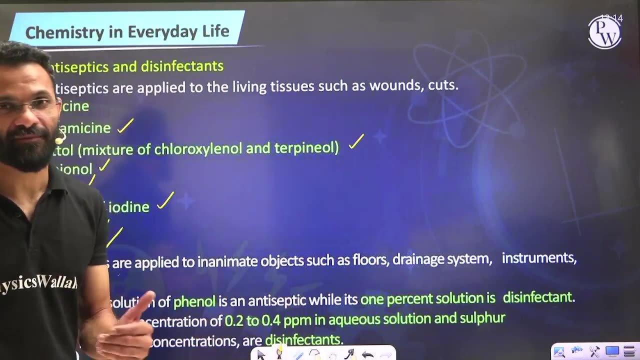 We studied antacid, We studied antihistamine, We studied tranquilizer, We studied analgesics. We talked about antimicrobials, that is, antibiotic, Antiseptic, Antiseptic and disinfectant. You guys will have to write down all these examples several times to remember the names and their respective category. 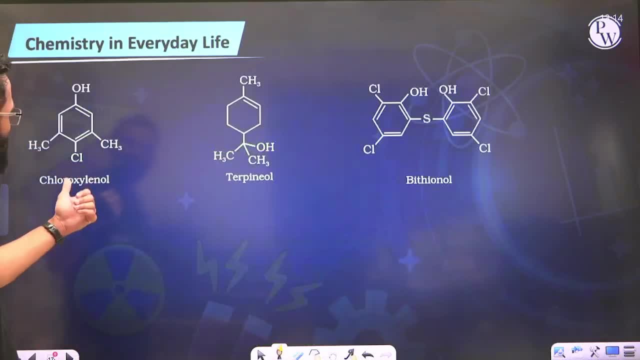 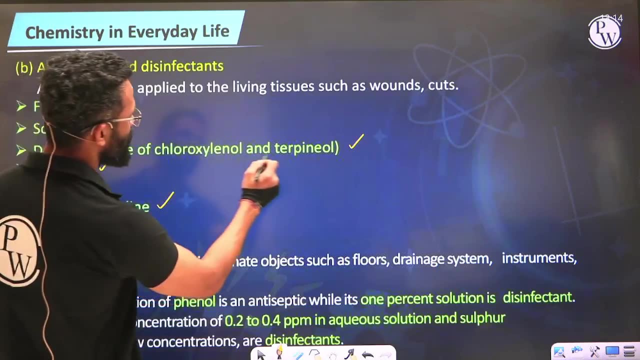 So you will see, chloro xylenol and terpeneol are the constituents of detol. Detol is a mixture of chloro, xylenol and terpeneol. So these two are the structure. Probably these two structure you can remember. 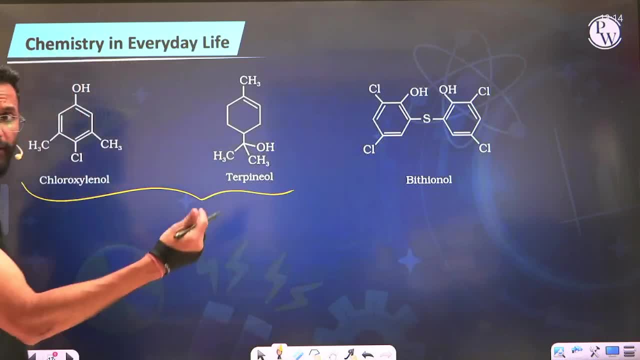 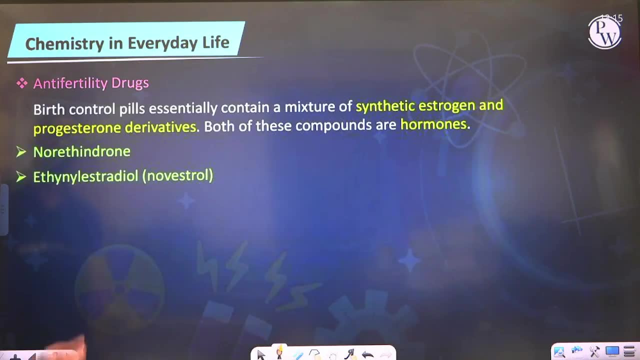 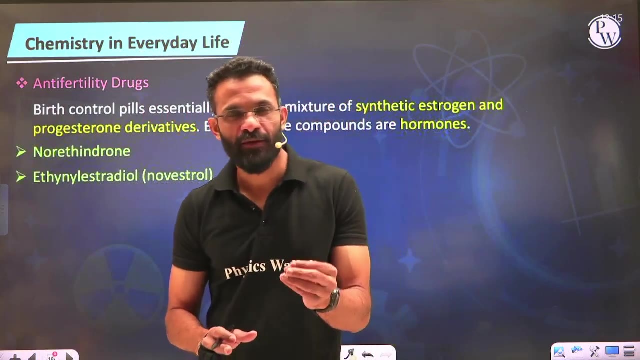 And here is the structure of bethional, The one which I said commonly used in the soap, Because our system한�t of drug is darkest drug And we do call it as oxytocin and penetrate as it is, Alright. Well, the next category of a drug that one will have to learn is anti-fertility drugs. 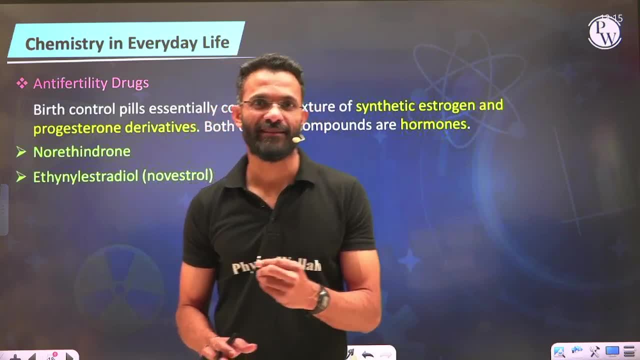 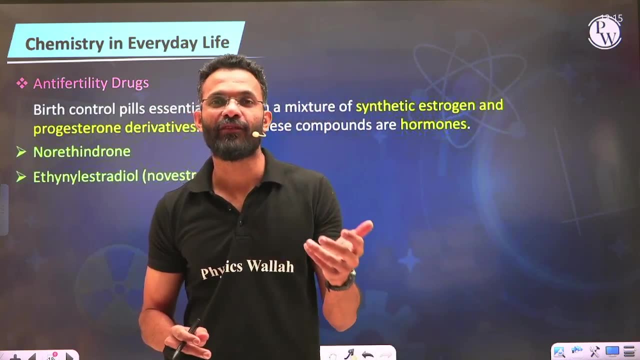 Well, anti-fertility drugs. in simple words, they are nothing but the birth control pills, Right So to stop or prevent pregnancy. the medicines that a person eat is basically anti-fertility drugs. You'll find these anti-fertility drugs are nothing but derivative of the hormones. 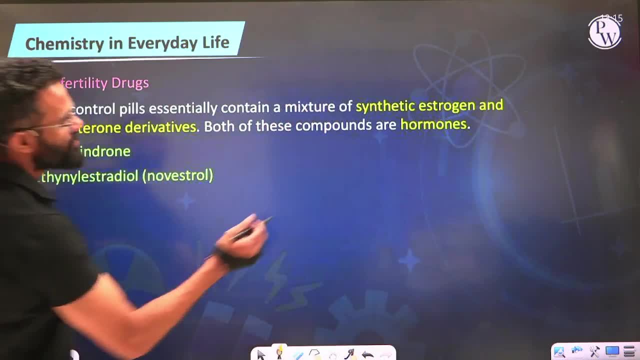 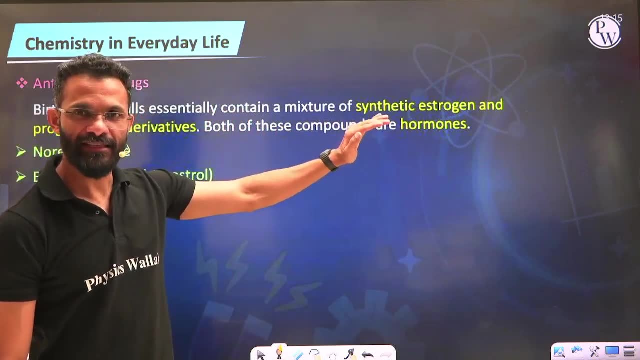 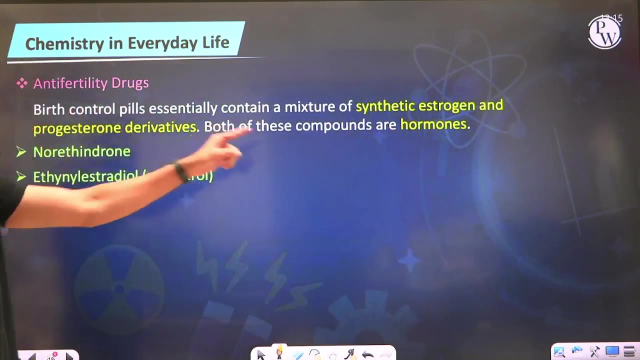 estrogen and progesterone. so estrogen and progesterone basically are the hormones and the medicines which are used to treat against those hormones are the one which are derived from this estrogen and progesterone. so synthetic estrogen and progesterone which are used for the birth control pills is what you call it as anti-fertility drugs. so two example you all can. 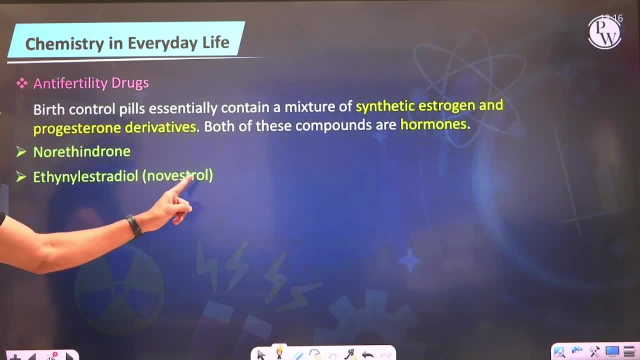 remember norethindrone and novastrol. norethindrone and novastrol- novastrol is just a name of ethinyl estradiol. ethinyl estradiol is what you call it as novastrol, so remember these two names. 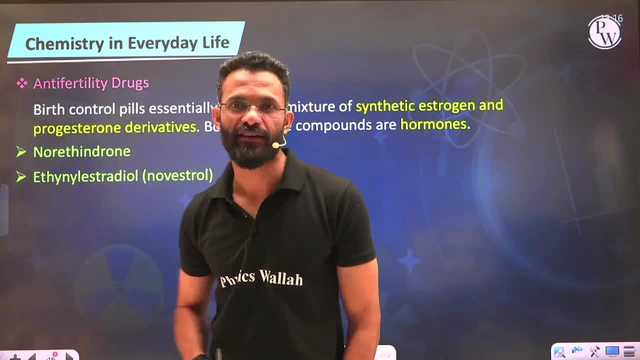 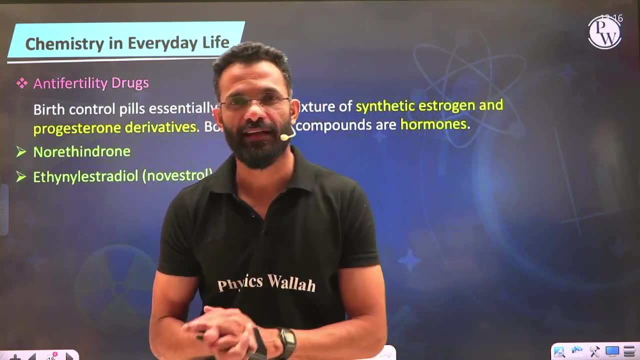 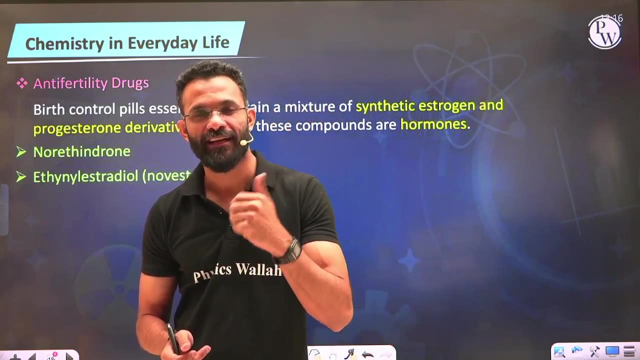 norethindrone and novastrol, which are anti-fertility drugs. so, guys, that was all about the classification of the drugs and its therapeutic action. i'm again telling you, guys, we'll have to write down the names, at least four to five times, of each category and try to remember them, because most of the 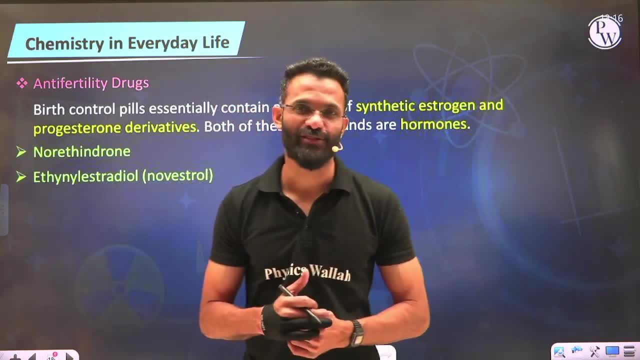 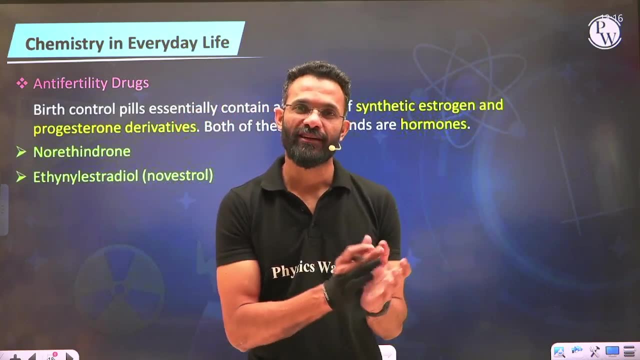 question you'll see always coming up from the names of drugs itself. so let me summarize what we have seen so far. right in the beginning, we discussed about what are called as drugs and how do we classify them. the second subtopic: we saw how drugs interact with the molecular target. 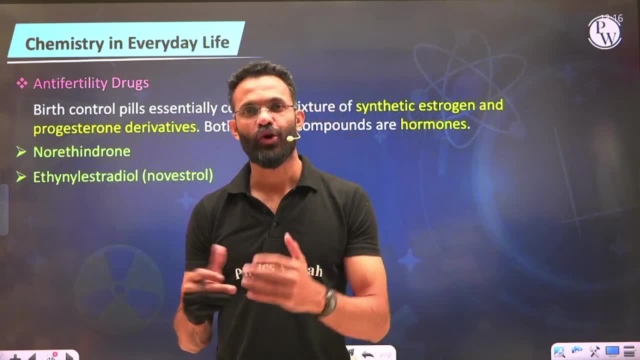 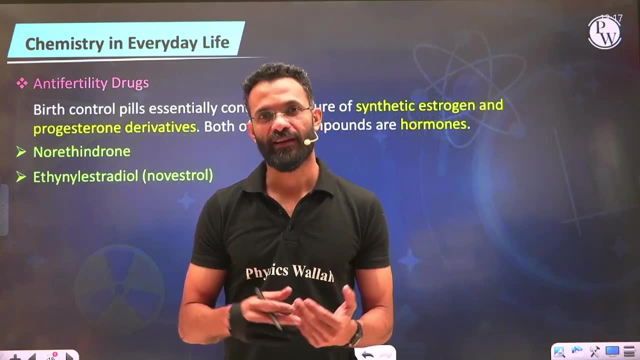 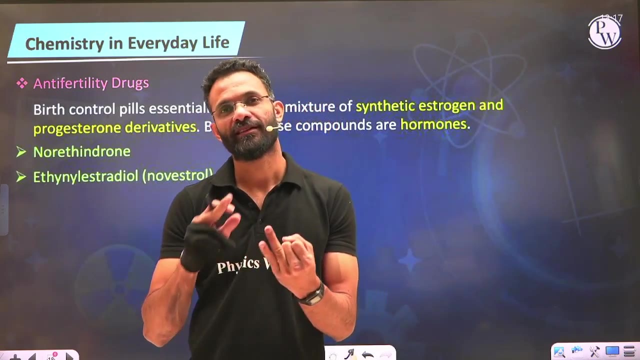 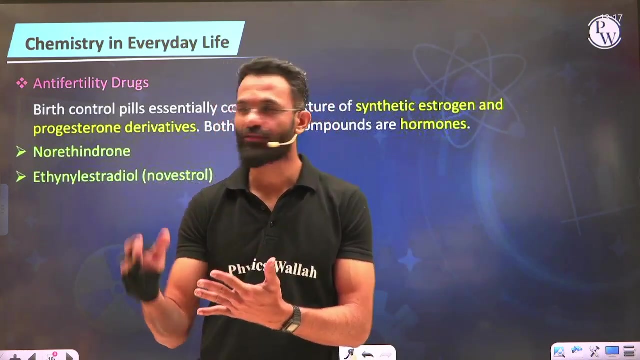 such as enzymes and receptor, and the third, which we saw, a classification of drug. the important type is this: the classification of drug and its therapeutic action, in which we included several types of drugs such as antacid, antihistamine. then we also studied tranquilizer, analgesics. we also discussed about antibiotic, antiseptic, disinfectant. 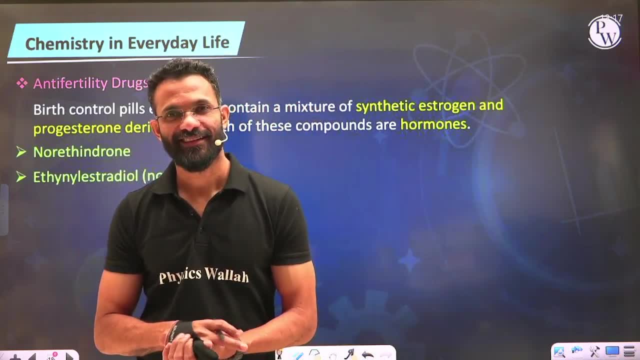 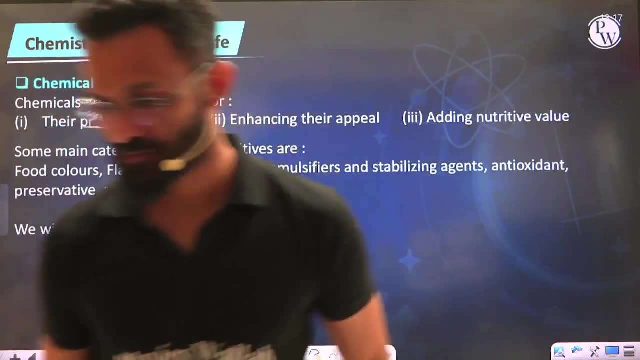 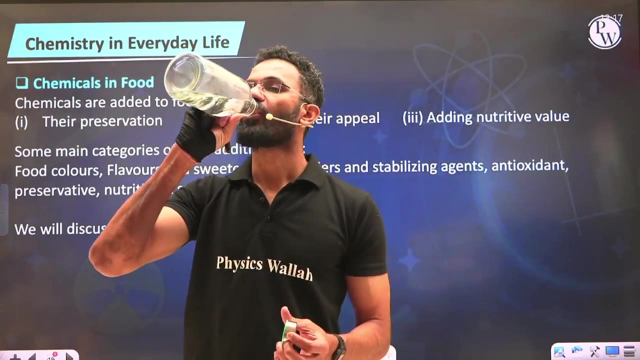 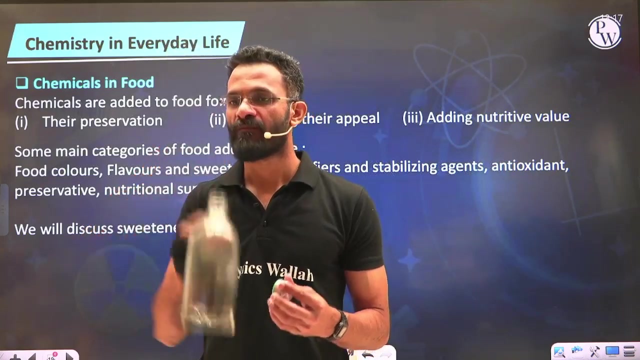 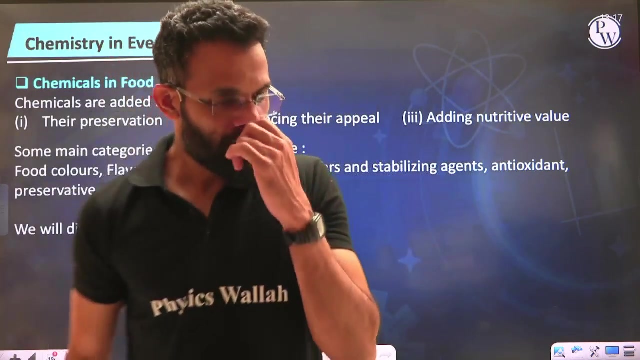 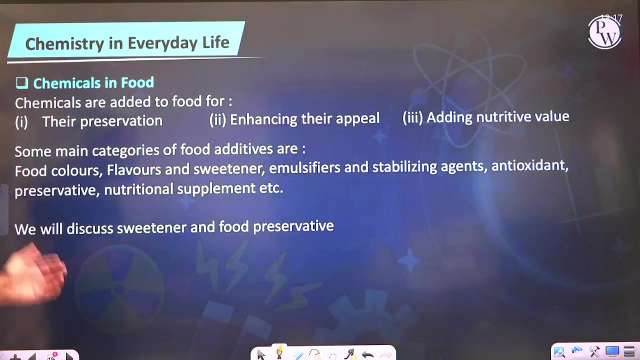 and anti-fertility drugs. now the last part of the chapter is chemicals in food. well, hold on, everyone, live while the subtitles are annoying. Habib Aliqrahi, All right guys. chemicals in food. Why we have to learn chemicals in food? because we have seen that these days we are so used to use stored eats 여기에. 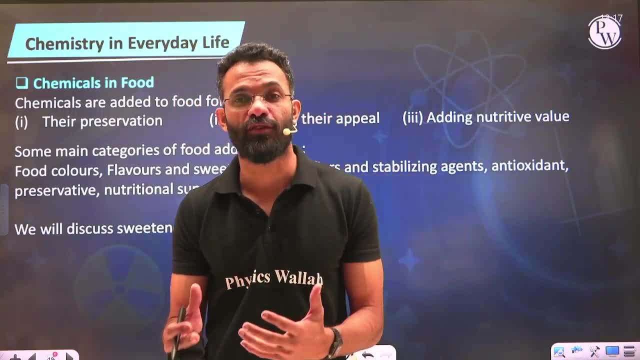 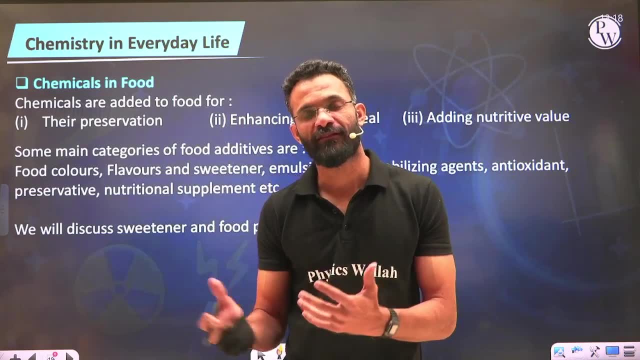 We have seen that these days we are so used use stored eats 여기에 to eat stored food right in our busy life. you have seen that in many of the cases when both husband and wife are working, they don't really get time to prepare food, so they opt for a substitute. 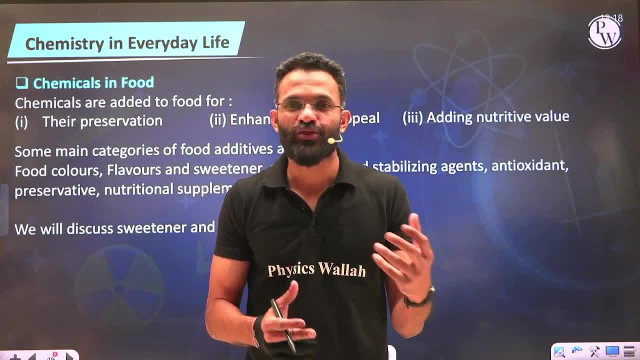 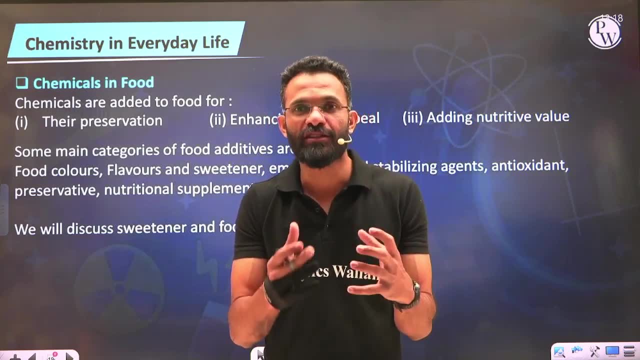 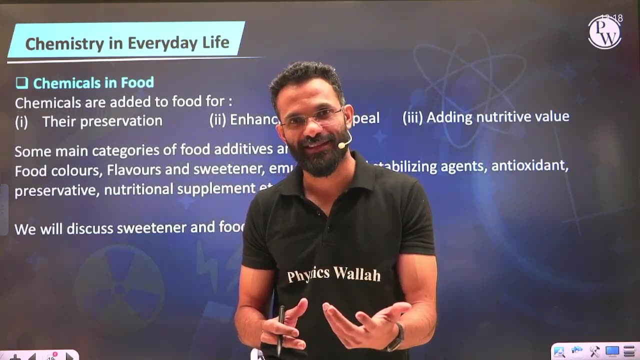 food, which is basically a stored food. so the stored food and the fresh food of course has a difference in its nutritional value. however, to keep the nutritional value intact, we further use some of the process which is called as food preservation techniques or food preservation process. so when you talk about increasing the shelf life of that particular food, that shelf 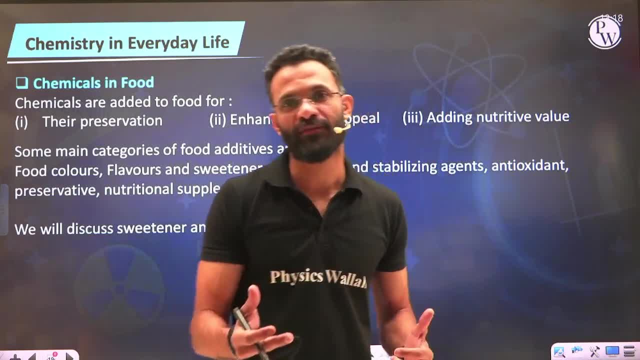 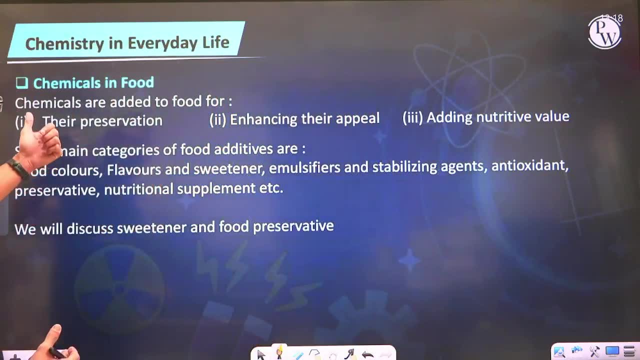 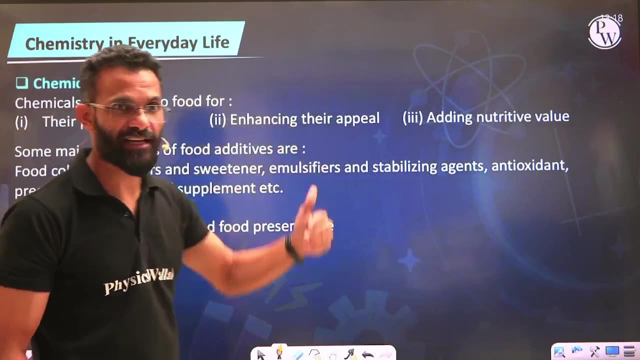 life of a food can be increased by addition of some of the chemical substances. so one of the reason why we have to add chemicals in the food, of course the chemicals that are added to food are for their preservation, like i said, or enhancing their appeal. that is how exactly. 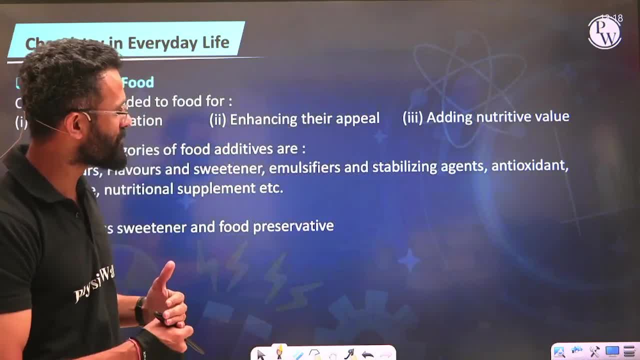 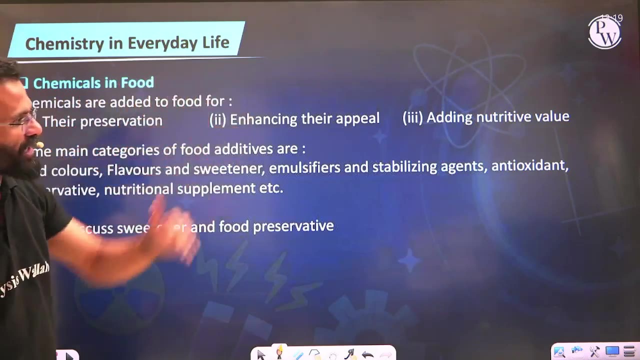 they look like, or how exactly uh, the color has to be used for that particular food, or they're also used for adding the nutritional value. so, guys, how exactly do we, how do we exactly uh maintain this, that is, preservation or enhancing the appeal or addition of nutrition value, are we can do that by adding. 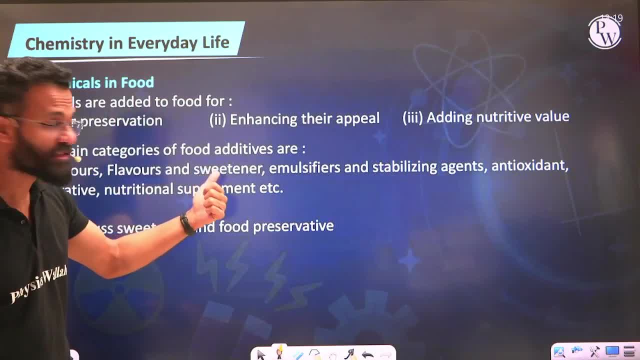 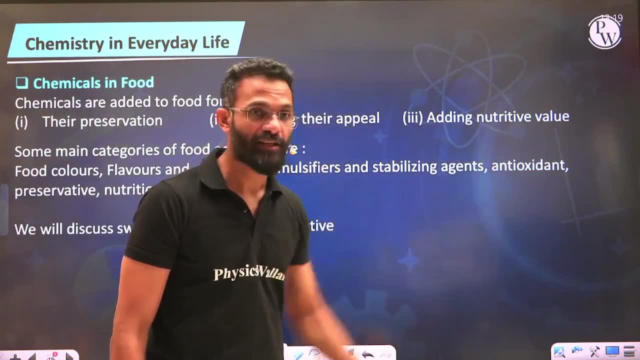 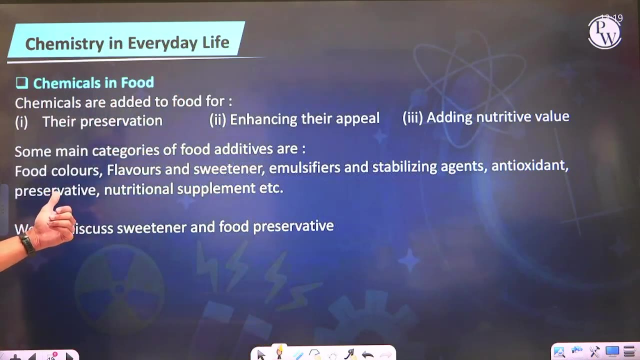 food colors or flavors or the sweeteners. we do it by adding emulsifiers, we add some stabilizing agents, we add some antioxidant which basically stop the oxidative spoilage of food. right, that is what you call it as antioxidant. we we also use some nutritional supplements, so basically, 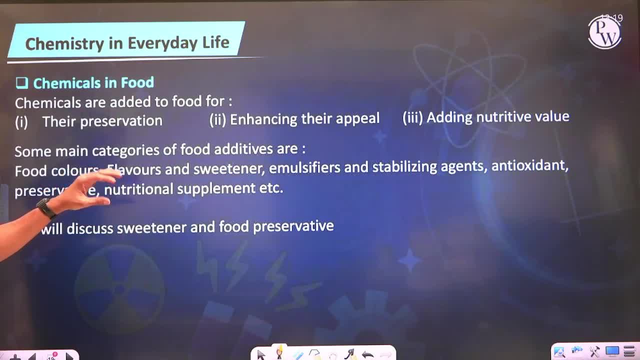 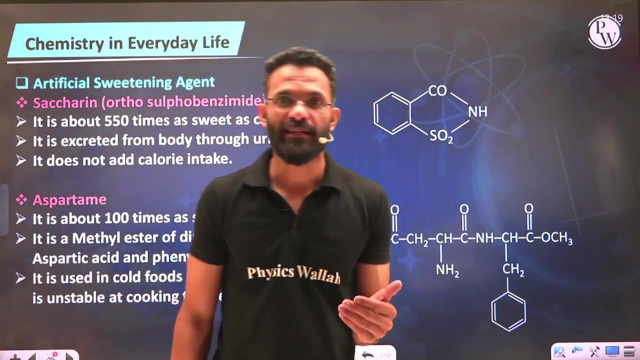 these all are the main categories which we add to a particular food in order to achieve these things. however, as far as our syllabus is concerned, we are only going to discuss about artificial sweetening agent and food preservations. you L when we talk about artificial sweetener. we have seen commonly diabetic people eating this kind. 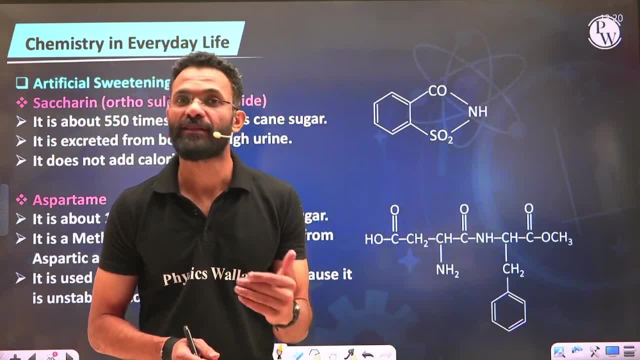 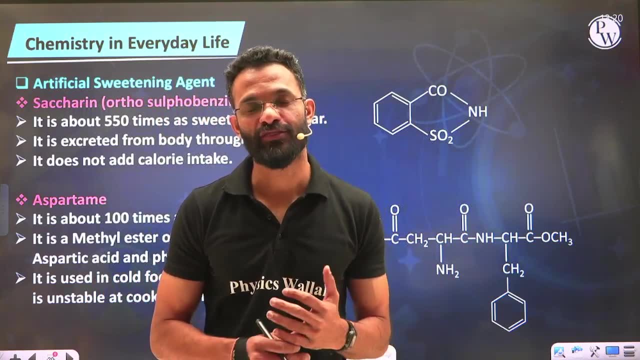 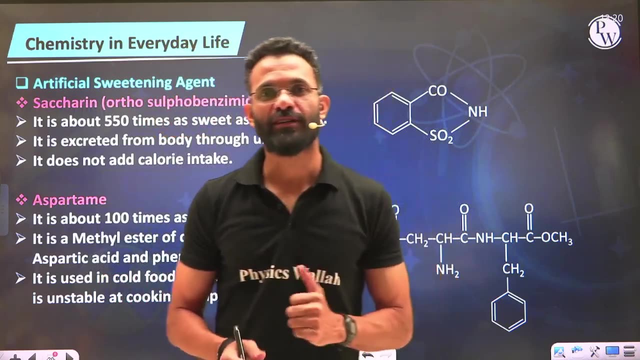 of artificial sweeteners also. we have seen the some of the health conscious people also, as an alternative to sugar, eat this artificial sweetener. so what exactly this artificial sweetener? do look, when we talk about a natural sugar such as cane sugar, we know that cane sugar 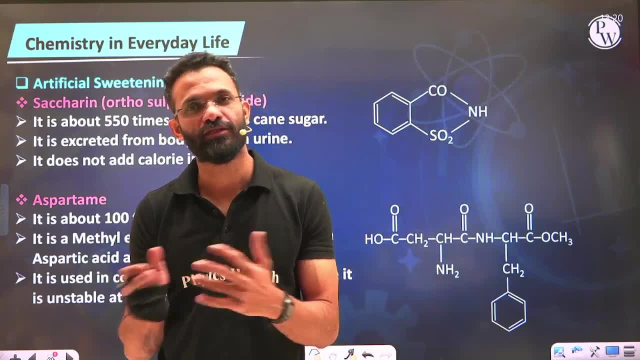 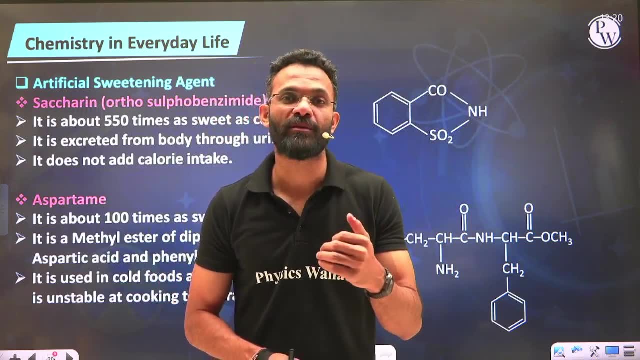 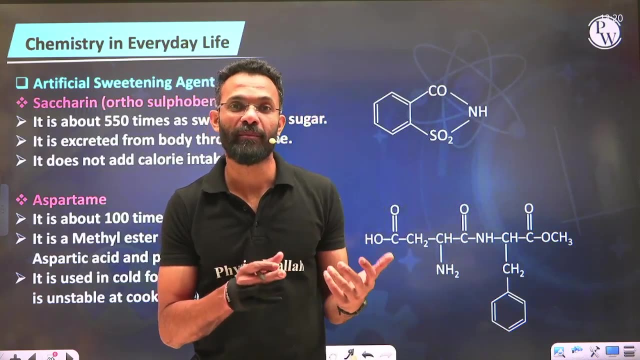 sugar- that is, sucrose- is basically a disacker of glucose and fructose. so when you eat it, other than giving us a sweet taste, it also add up to some calories, and that's why you must have seen that the health conscious people, or to lose weight people, stop eating sugar, because eating sugar also adds some calories. hence, alternatively, what we do is we eat those kind of substances which will give that sweetness which a natural sugar gives, but won't add up to the calories. now, why won't it add up to the calories is because this kind of artificial sweetening agents are never 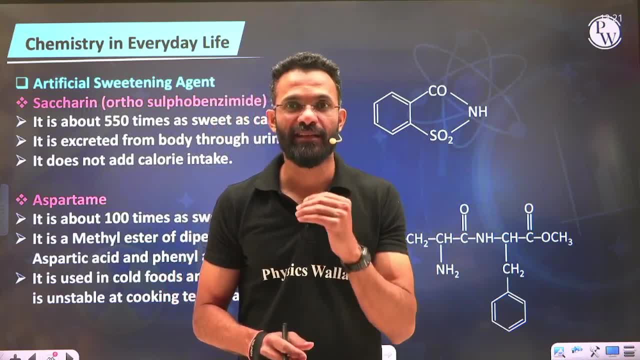 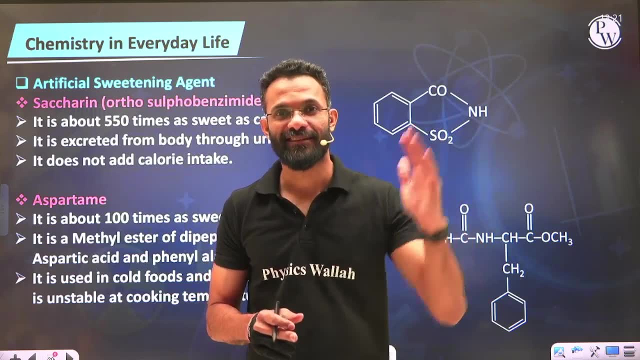 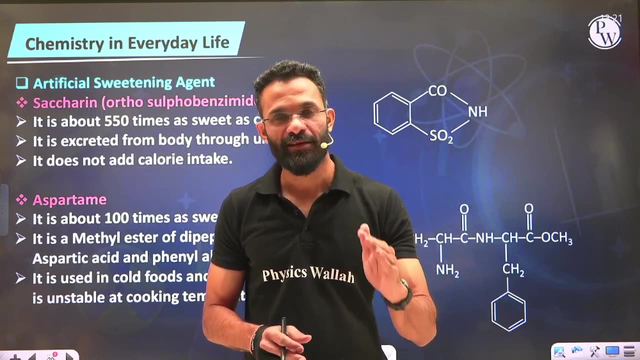 absorbed or consumed in the body. so when you eat it they will give you that sweetness. but because they are never digested in the body, our kidney has to secret it. so artificial sweeteners will add up to the, will give the sweet, sweet taste, but it won't add up to any calories. so the several type of example which we study in the artificial 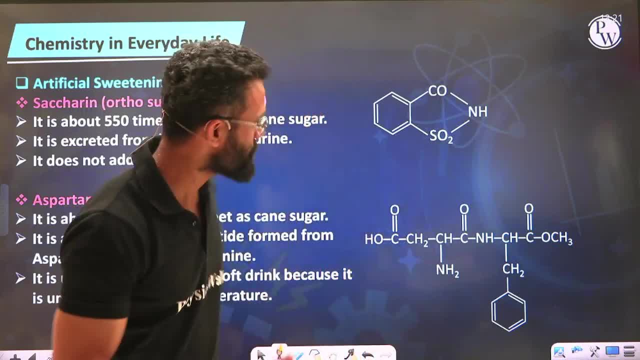 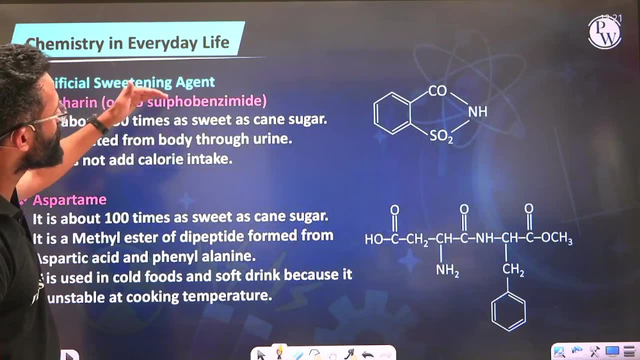 sweetener which are very commonly used by the diabetic people, one of which is saccharin. i'm sure everyone is aware of this. saccharin is nothing but ortho sulfo benzimide. here is the structure. you can see. you can remember. this structure is pretty simple. now, this saccharin: 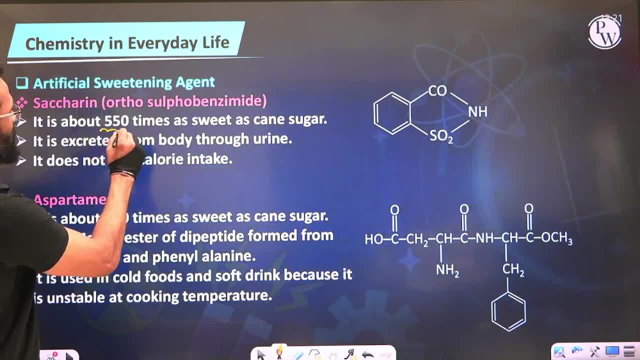 is found to be about 550 times sweeter than the artificial sweetener. so this is the structure you can see in the physical form of an artificial sweetener: these two elements of alopecia and that of cane sugar and, like i said, since it is never digested in the body, it has to be excreted. 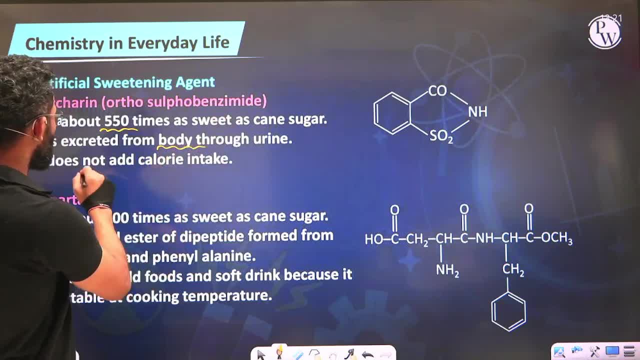 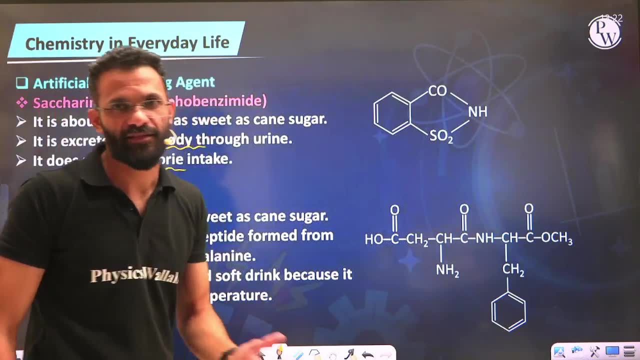 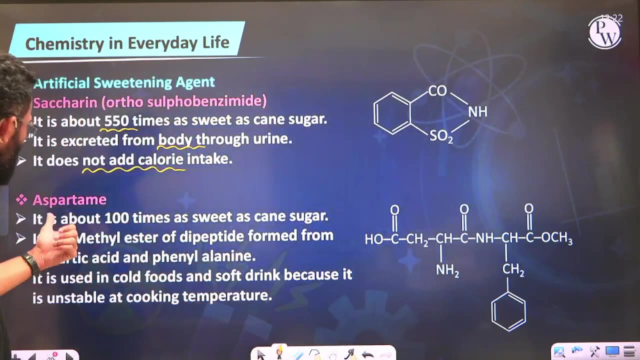 from body through urine and it does not add any calorie to our body because of course it is never absorbed or digested. so that was all about saccharin, very commonly used artificial sweetening agent. just like that, we study three more. second one is called as aspartame- aspartame. 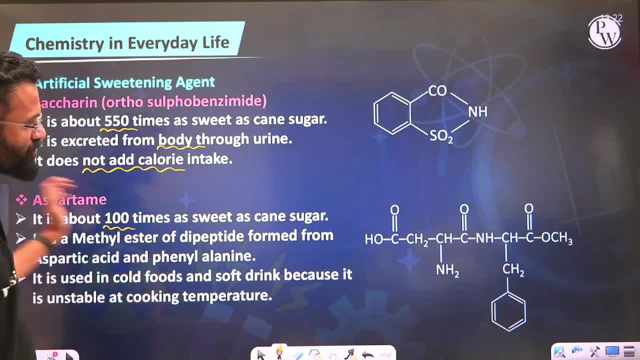 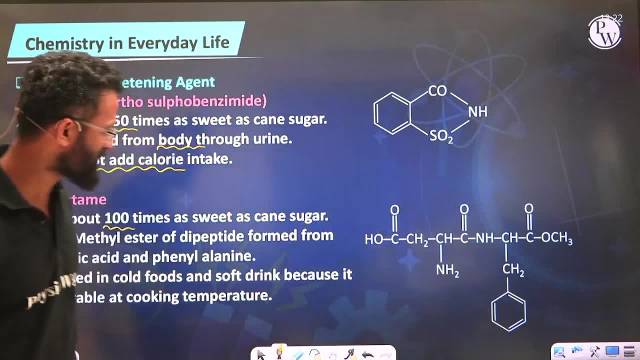 is about 100 times as sweet as cane sugar. you can see the structure right here. you are not expected to remember the structure, but yes, this is how it looks like. it is basically methyl ester of dipeptide formed from aspartic acid and phenylalanine. so you will see there are two. 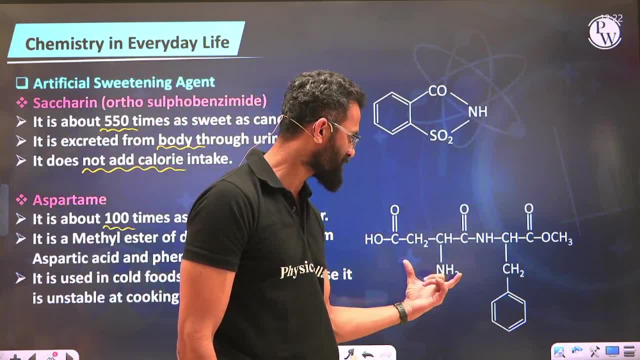 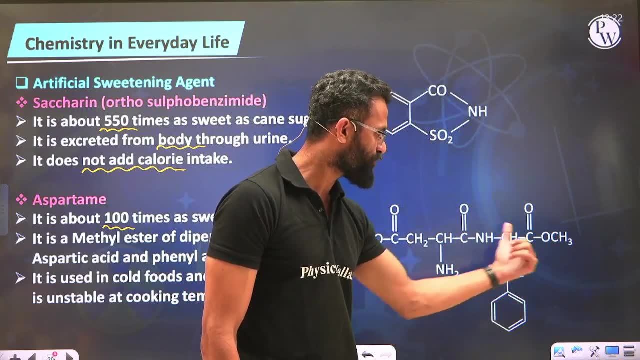 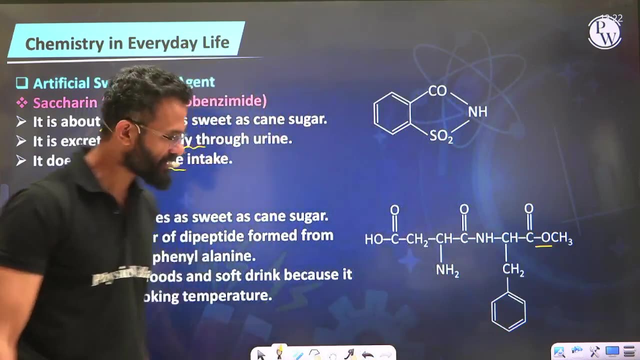 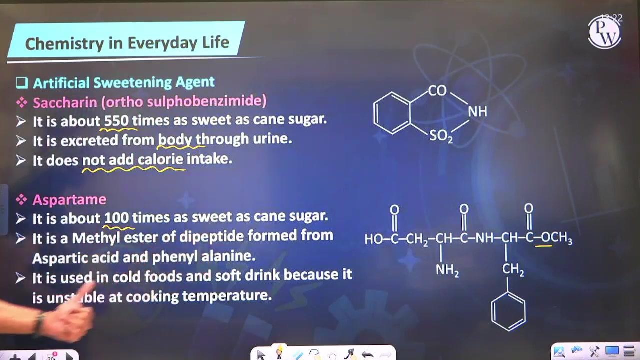 parts here, this first part in the structure basically corresponding to aspartic acid, that is, acetic alpha amino acid, and there is another alpha amino acid that is called as phenylalanine, and this is the ester of those alpha amino acids. so it is a methyl ester of dipeptide formed from aspartic acid and phenylalanine. and where do we? 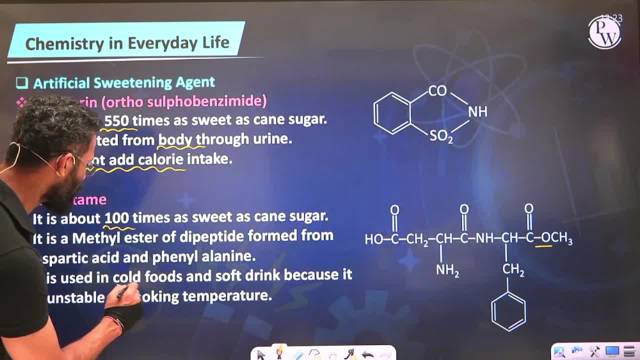 use it. commonly, it is used in cold foods and the soft drinks. and why so? remember this is important data, because aspartic acid is formed from aspartic acid and phenylalanine. and where do we use it? aspartic acid is unstable at cooking temperature. 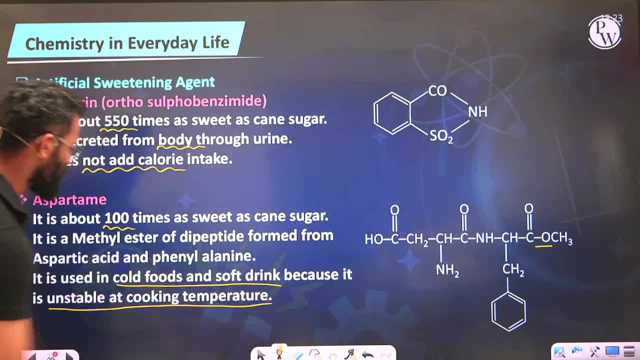 because aspartic acid is unstable at the cooking temperature, we use it only in those foods which are preserved at a lower temperature. all right, so saccharine 550 times sweeter, aspartic acid 100 times sweeter. next is alletame. alletame- you can see structure here, just for the information. 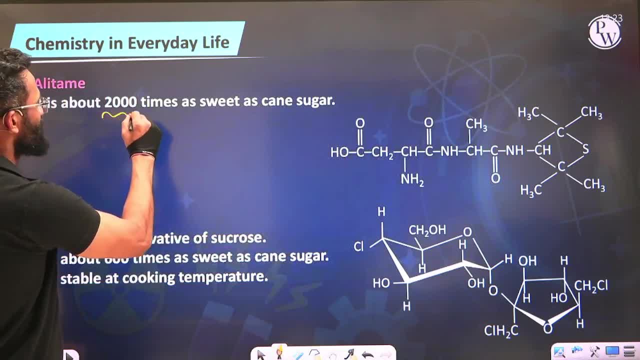 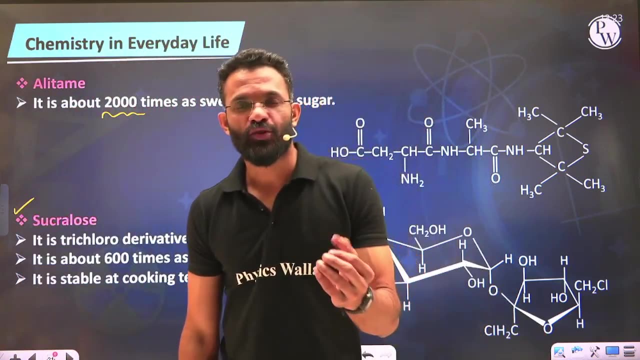 and it is 2000 times as sweet as cane sugar and it is found to be even more stable than the aspartame. the fourth one is sucralose. well guys, if you just check some of those supplementary food, you will find to increase the shelf life. 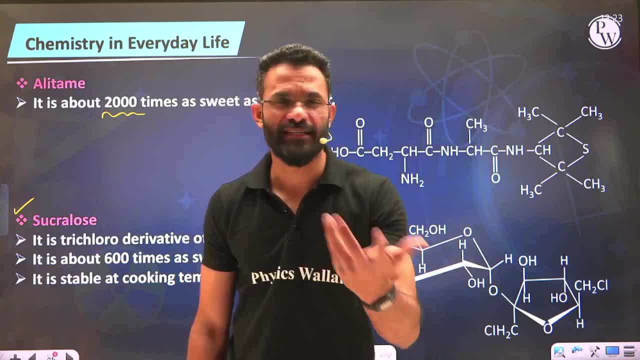 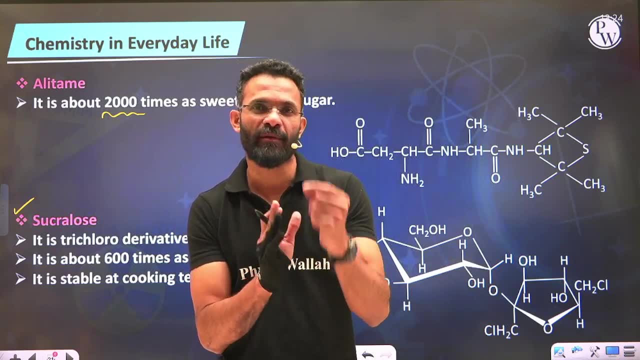 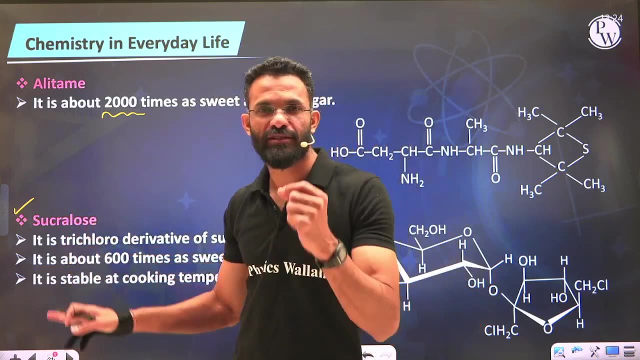 of the supplementary food such as, let's say, protein supplement. if you ever see, if you ever see, uh, if you ever see the protein supplement, read its ingredient. you will find the sugar that they use in protein supplement, generally sucralose, because natural sugar has a very lesser shelf life. to increase the shelf life, 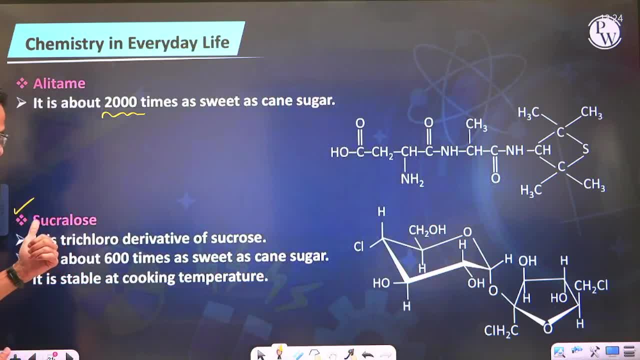 of that product, we use a sugar that is called as sucralose, and this is how the sucralose looks like. this sucralose is nothing but trichloro derivative of sucrose itself, and it is about 600 times as sweet as cane sugar, and this can be used at a cooking temperature as well, because it is stable. 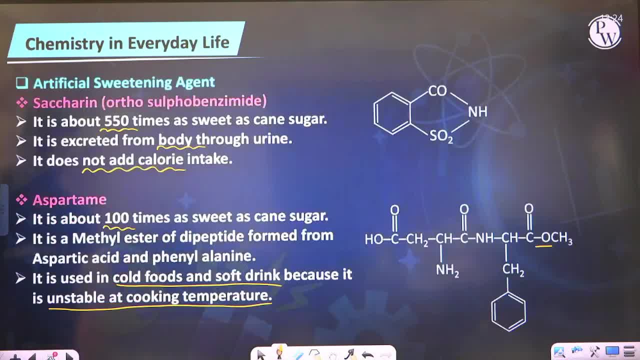 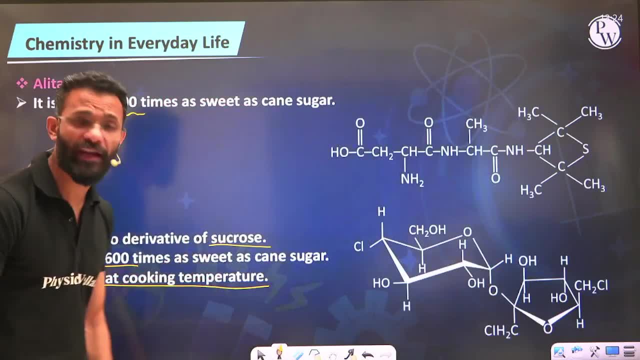 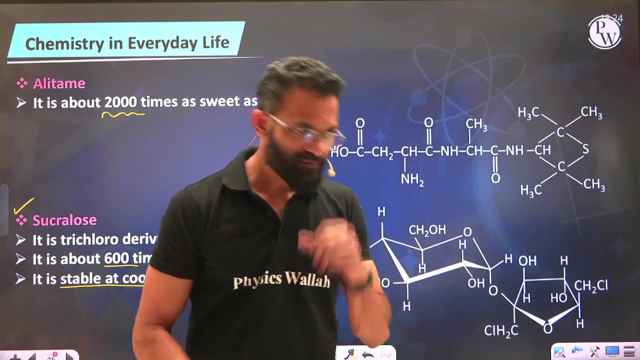 at cooking temperature. so remember, aspartame is unstable at the cooking temperature, whereas sucralose is stable at the cooking temperature. you may have question on this particular data. so that was all about artificial sweetening agent and, like we said, other than this artificial sweetening. 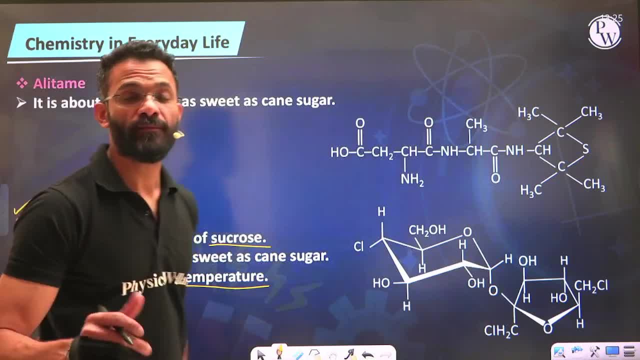 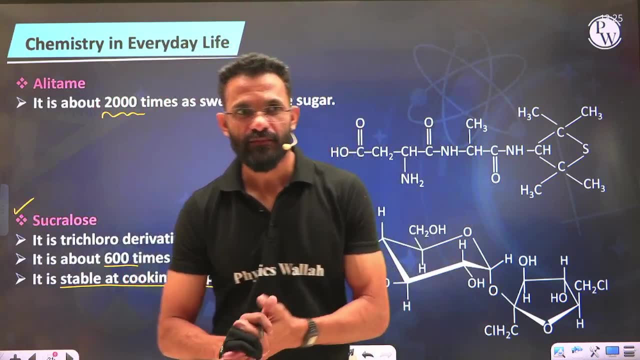 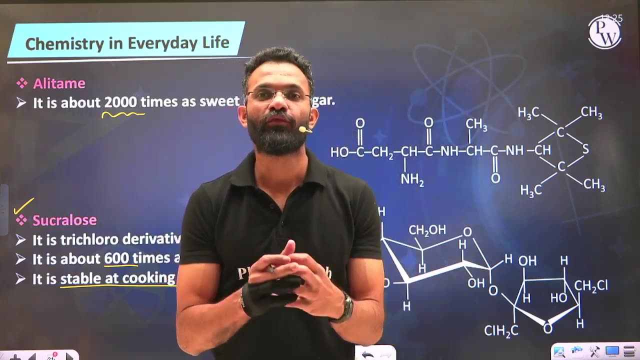 agent. we also talk about artificial food preservatives. now, why do we not? why do we need artificial food preservatives? is basically because, like we said, these days we depend, we are dependent on lot- upon the food which is readily available to us, and that's why we need some of the techniques or 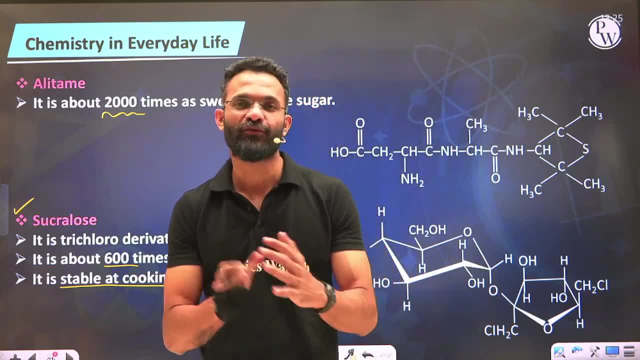 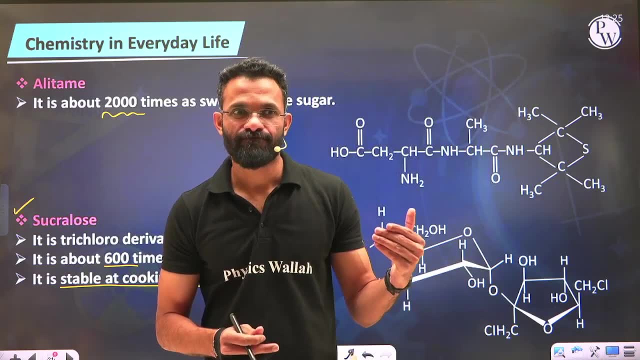 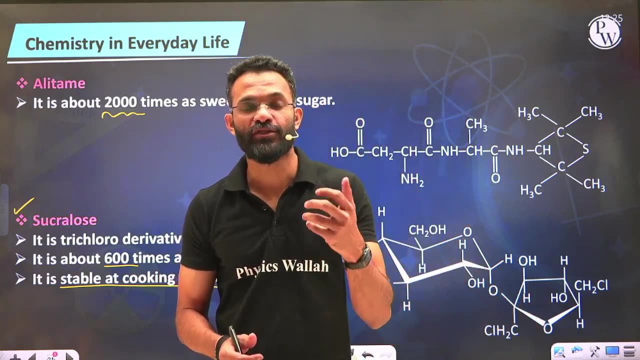 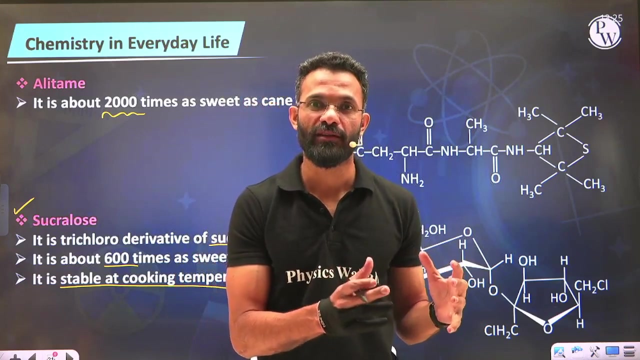 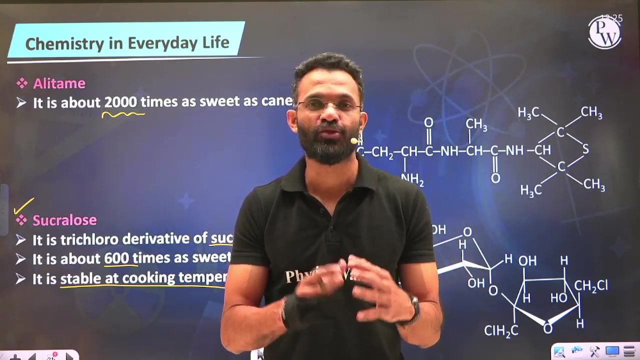 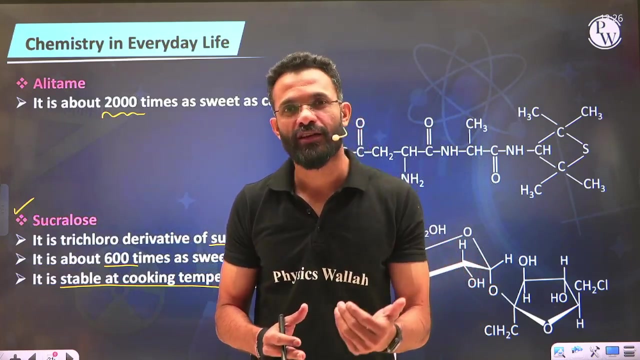 the processes which can help to preserve the food for a very long time. so, everyone, if you just talk about all the uh, you know the traditional methods that we used to use in old days. like uh, you can say Trojan. any Chinese acrylic Father said the method which used to be made from. Fourier skateboard is from: associate of social science. like blowing ball power, applies this to the food by leaving some healthy mineral resources but decreasing healthy or refreshing fuel and matter of earn, while preserving food tastes, actually removing, pull nutrition from the food with these processes. these placements are slow, producing acidic cooking substances. 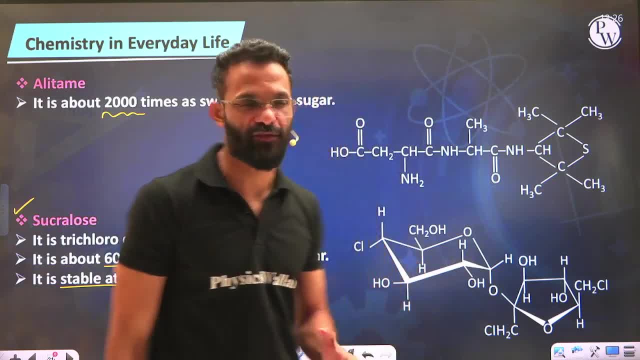 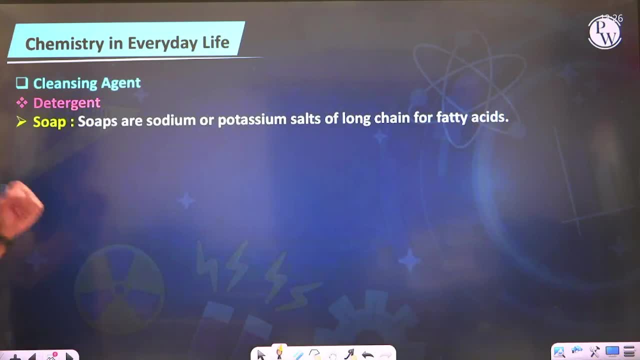 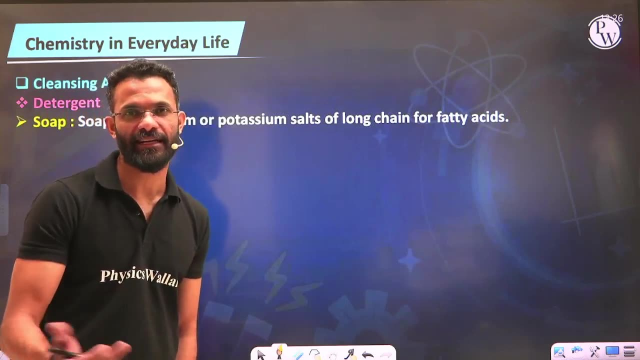 sodium benzoate is very commonly used food preservative guys. after this, the last part that we'll have to learn is about the cleansing and the cleansing agent. so there are two types of cleansing agent that we learn. one is soap and other is synthetic detergents. all right, let us understand first what 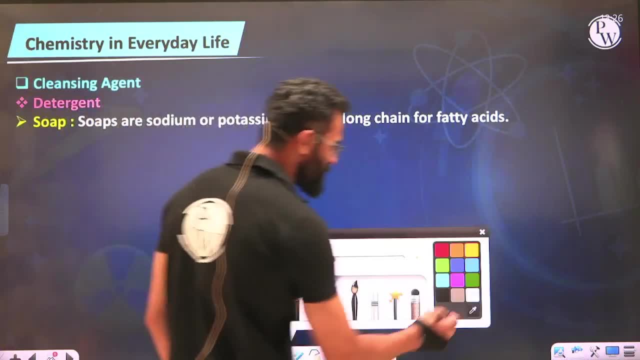 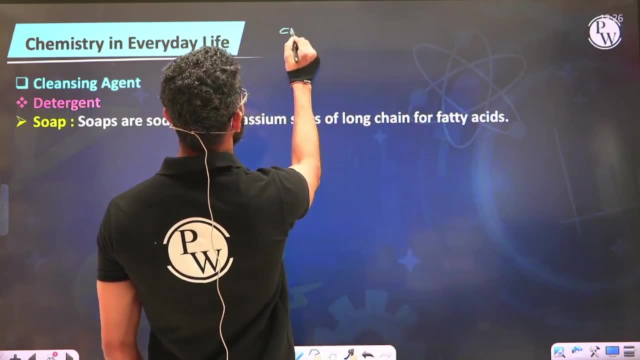 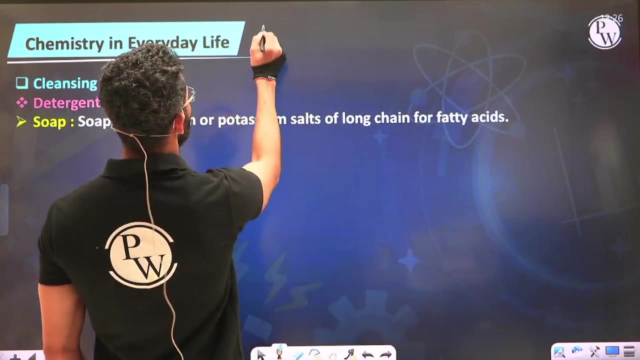 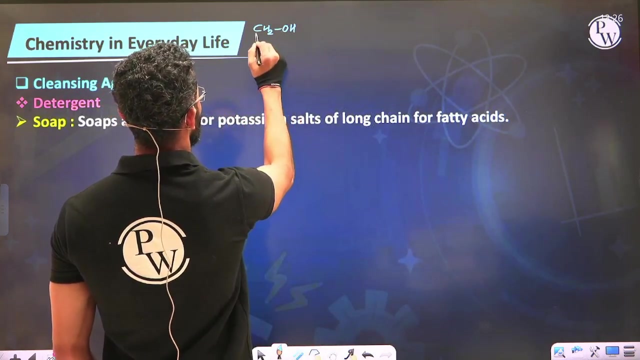 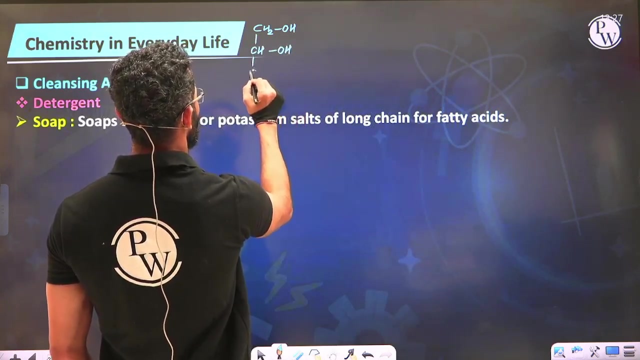 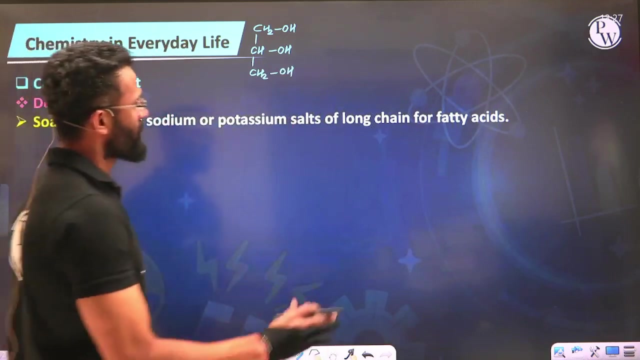 is soup. well, as let's see one general reaction here, suppose if I say I have glycerol, okay, so let's say we have glycerol, glycerol is propane, one, two, three, try, all okay. and let's say, if I treat this with some long-chain fatty acids such as oleic, 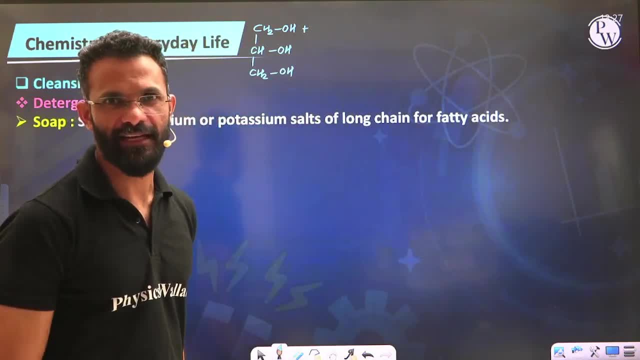 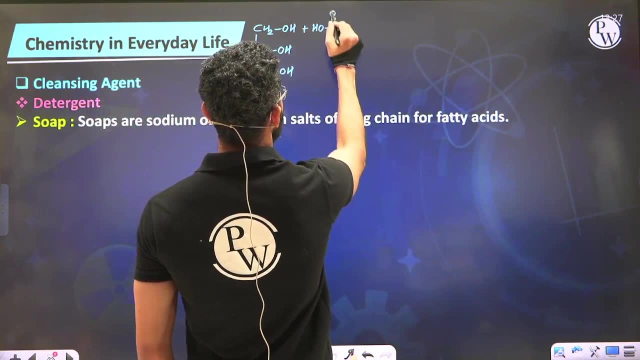 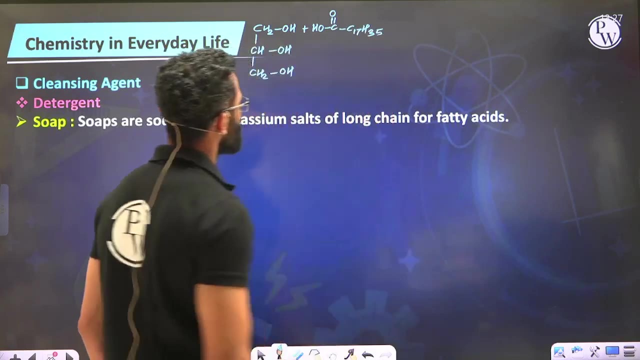 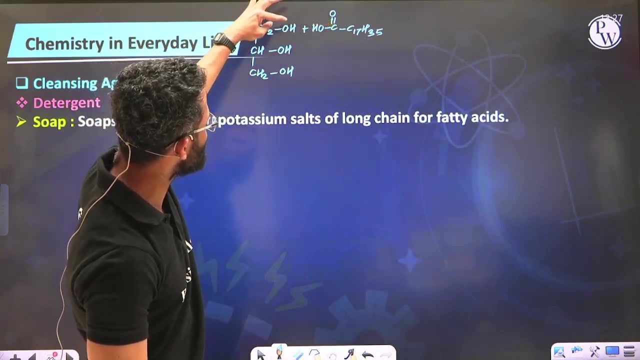 acid, linoleic acid, stearic acid, palmitic acid, anything. okay, let's say I'm taking stearic acid, see 17h 35. okay, you can see here. this is alkali function. this is carboxylic acid. when carboxylic acid and alcohol are treated. 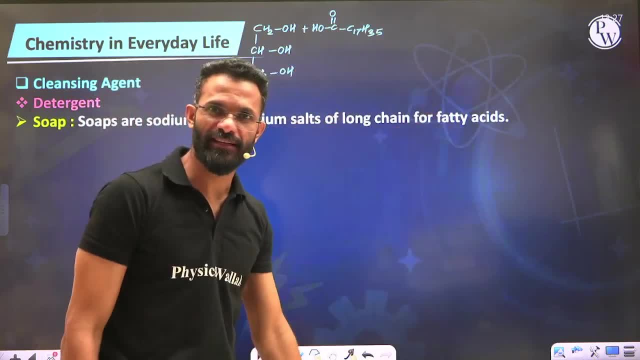 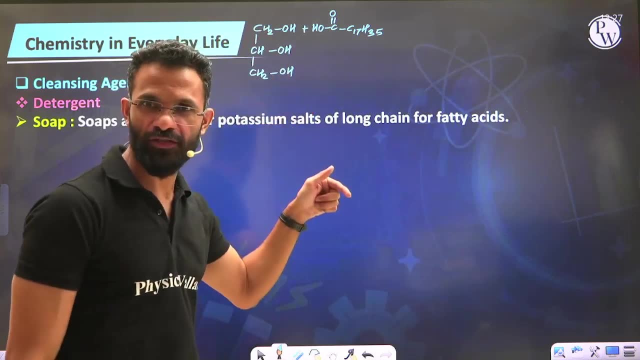 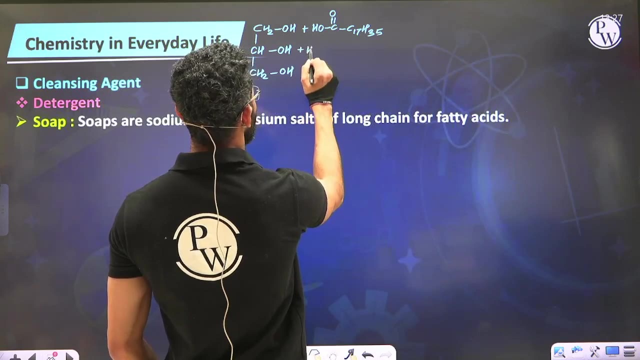 they undergo condensation reaction to produce an ester right. so if I remove OH from acid and H from alcohol, we are gonna get ester functional. since I've got three such alcoholic OH group, let's say I'm taking three equivalents of this stearic acid, so this is second equivalent. 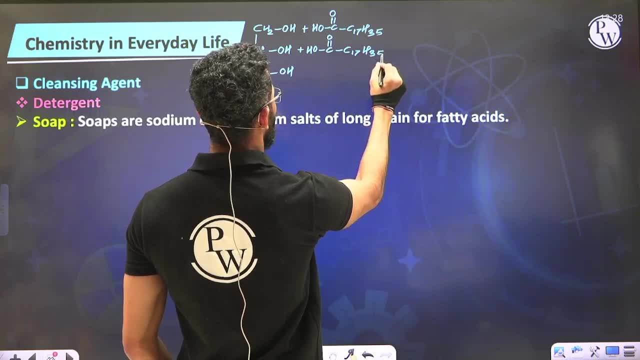 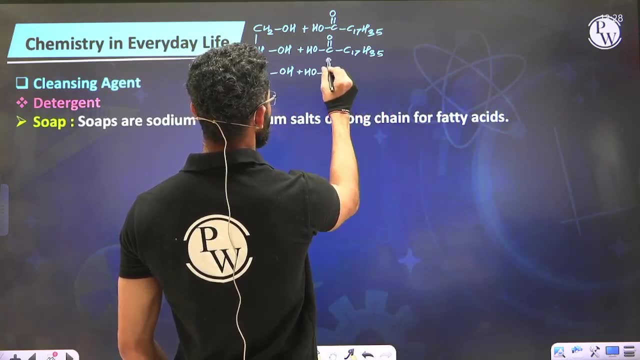 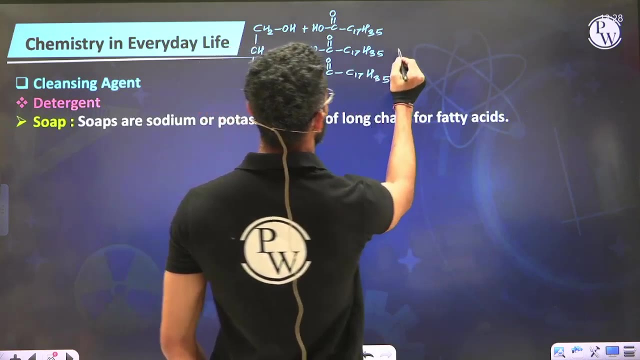 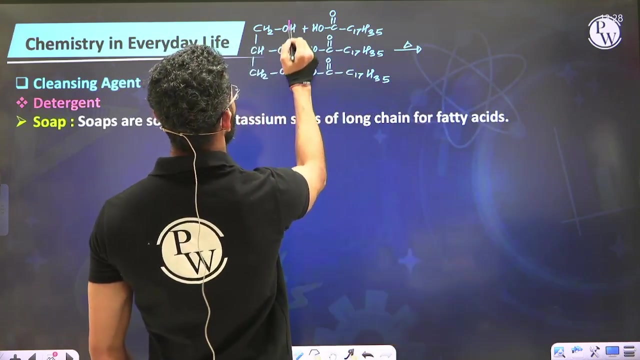 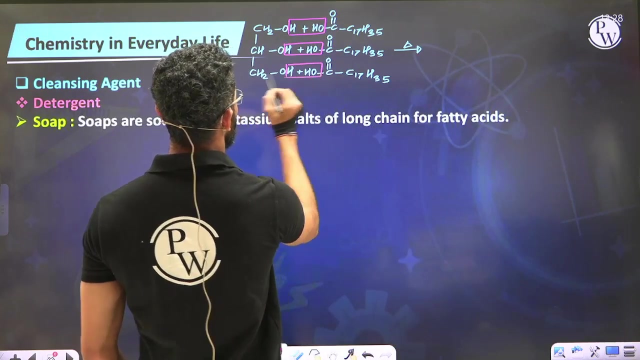 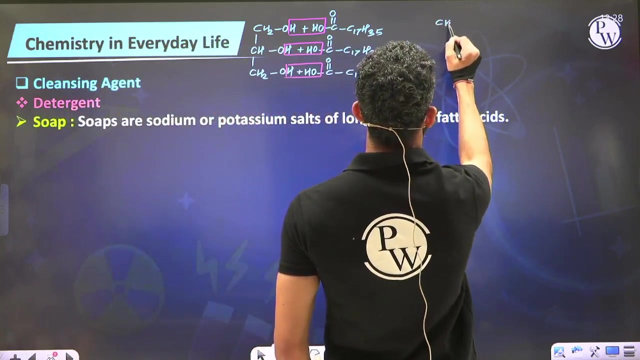 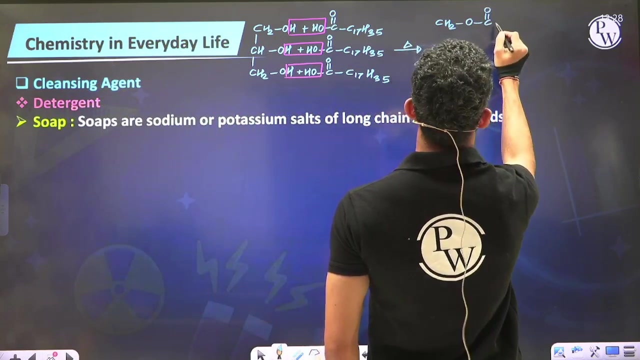 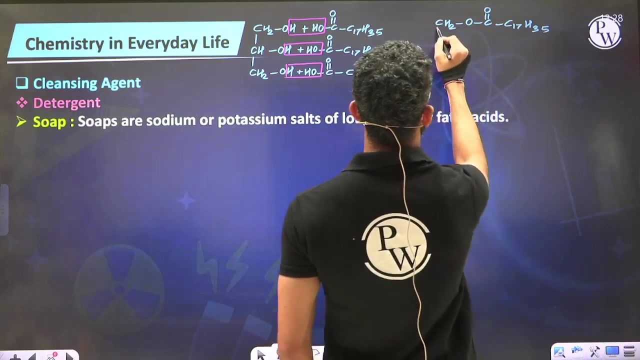 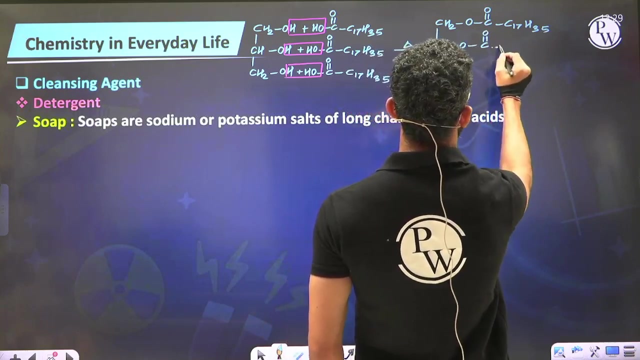 you, and here is the third. okay, and if you condense it, let's say the product that we are getting is CH2OCOOC17H35.. CHOCOOC17H35.. CHOCOOC17H35.. CHOCOOC17H35. 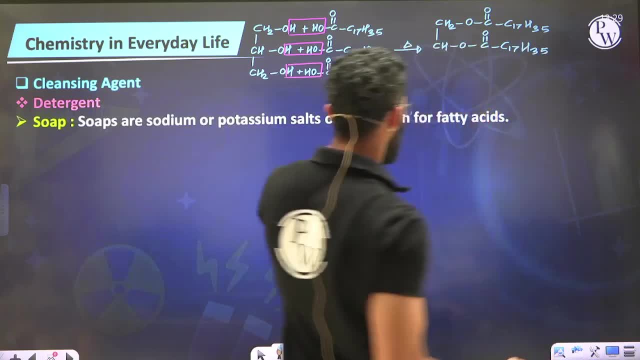 CHOCOOC17H35.. CHOCOOC17H35.. CHOCOOC17H35.. CHOCOOC17H35.. Again here, CHOCOOC17H35.. CHOCOOC17H35.. CHOCOOC17H35.. 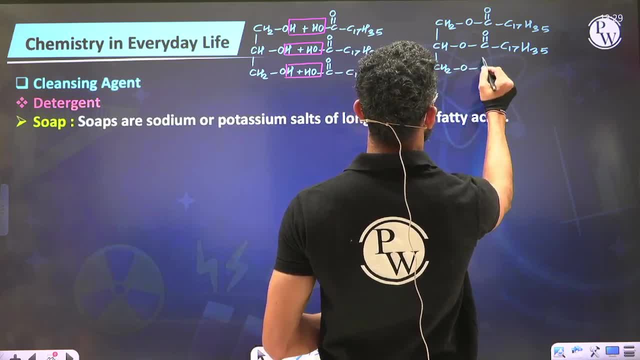 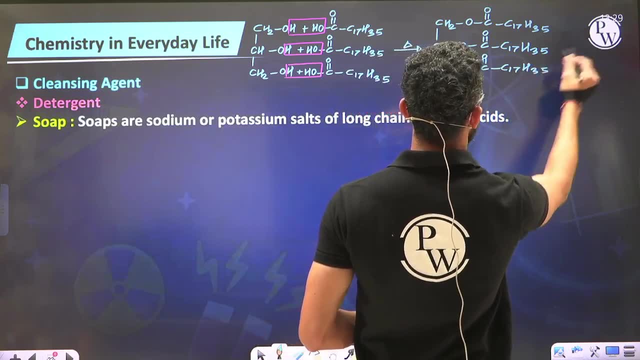 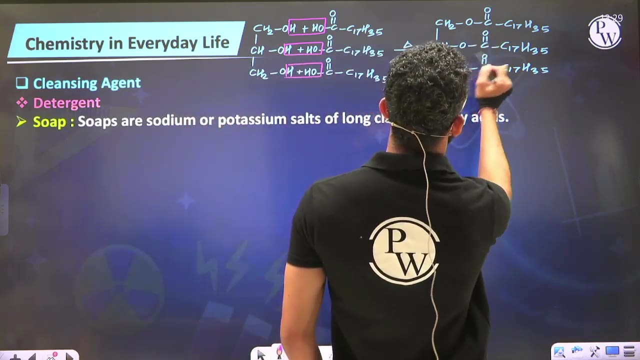 C17H35.. Chocobo-N, C17H35., C17H35.. And, of course, through equivalent of water molecule. Now see the product which is obtained here. contain 3 ester group 1, 2 and 3.. 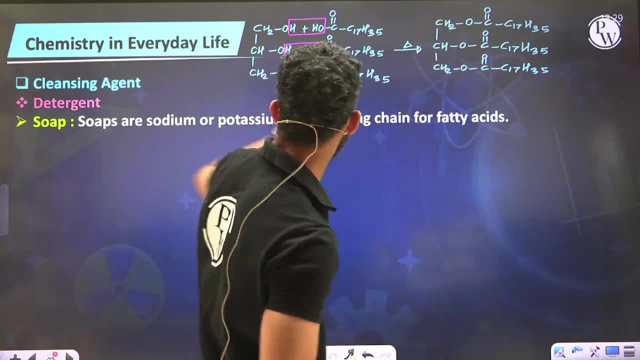 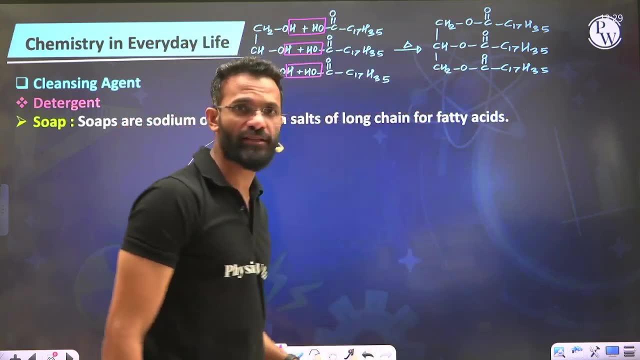 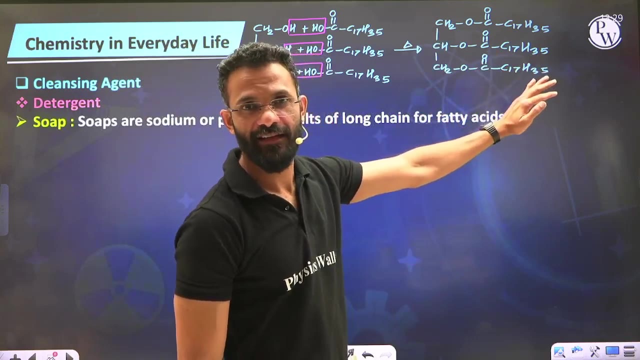 I'll call this as triester of glycerases and fatty acid. triester of glycerol and fatty acid, fatty acid is your stearic acid, so this is called as triester of glycerol and stearic acid. now, this triester is sometime also referred as 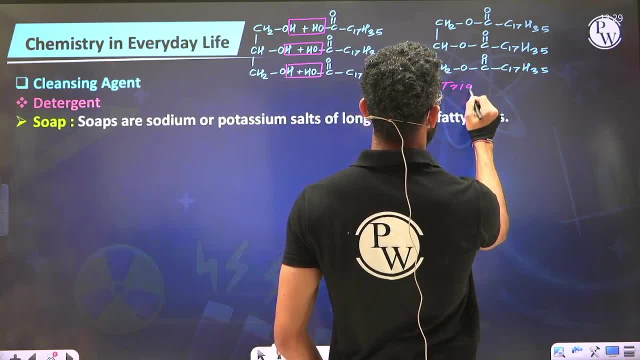 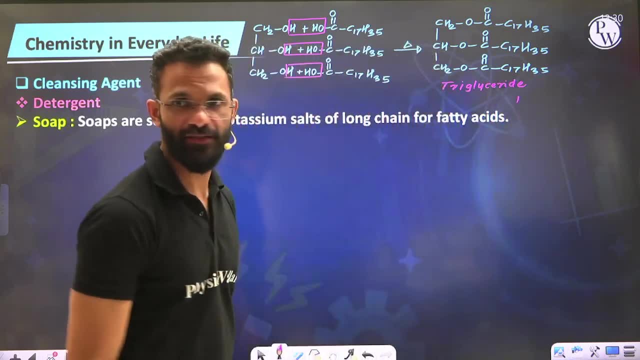 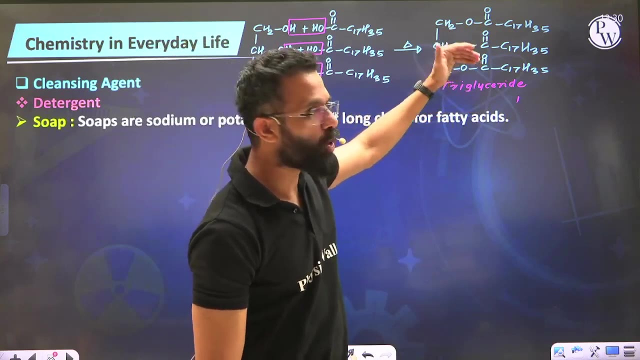 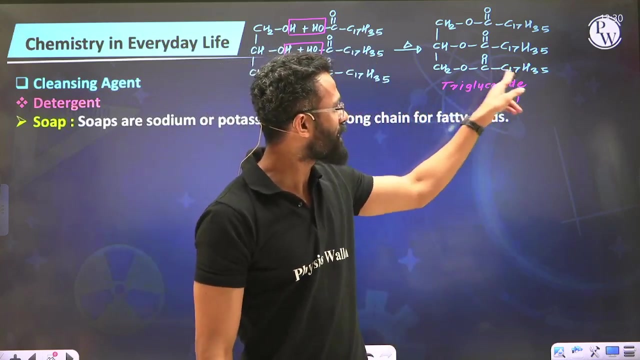 triglyceride, triglycerides- alright, now let us say this triglyceride we have taken over here. now this triglyceride could be oil or could be a fat, depending upon the nature of hydrocarbon part present here. so let us say if this carbon chain or the hydrocarbon part is having some 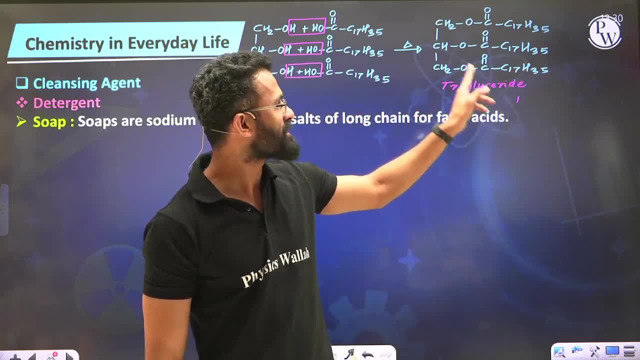 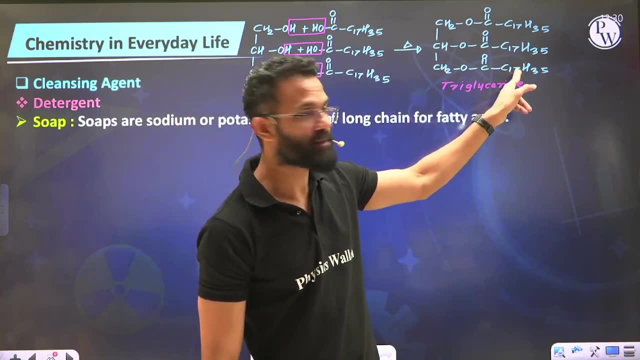 unsaturation, having double bond, let's say. then i will say this is the tri triglycerides. now let us say this triglyceride could be oil or could be a fat, depending upon, of glycerol with unsaturated fatty acids. if there is unsaturation present here, imagine, then i would 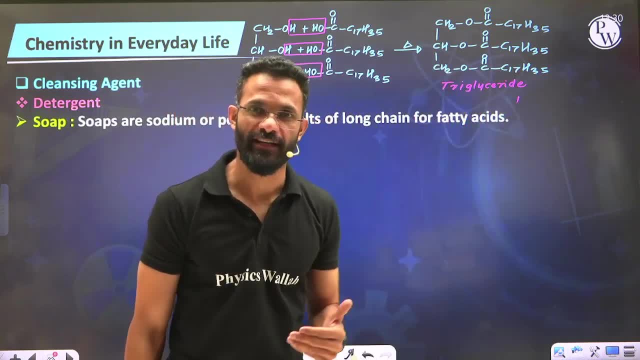 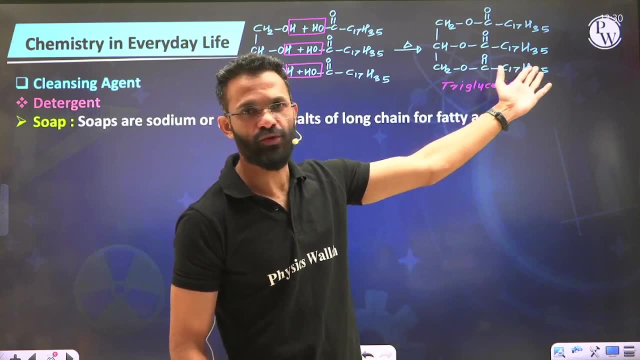 say this is a triester of glycerol with unsaturated fatty acid. that triester of glycerol with unsaturated fatty acid is what you call it as oil and, like like here, it is a saturated one. so i will say this is triester of glycerol and saturated fatty acid, which you call it as fat. 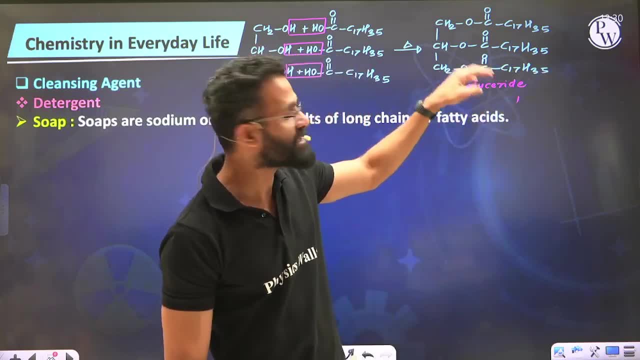 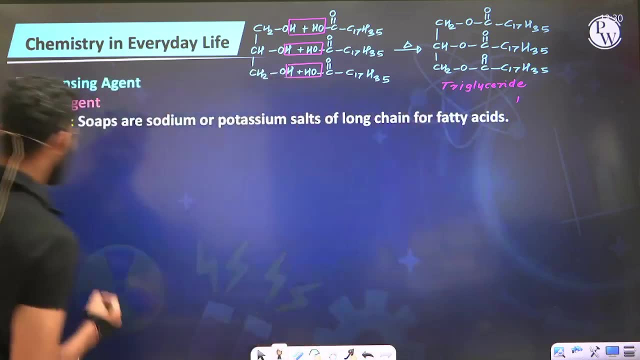 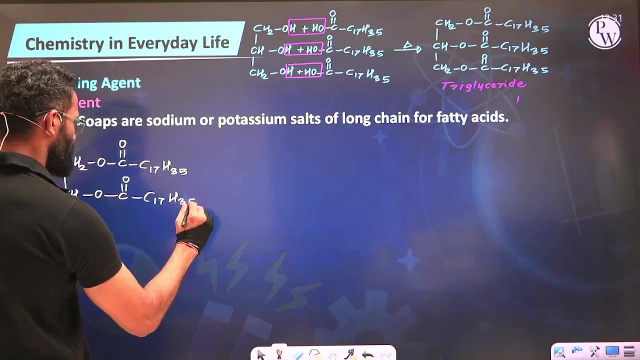 so this triglyceride is basically a fat. if i take this fat here, i'm taking that fat ch four c double bond, oh c 17 h 35. weather connected to ch2 oh c double bond, oh e17 h35. okay, so this is what a fat, which is basically triester. 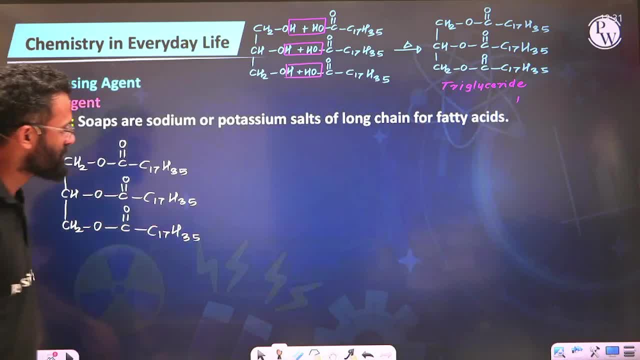 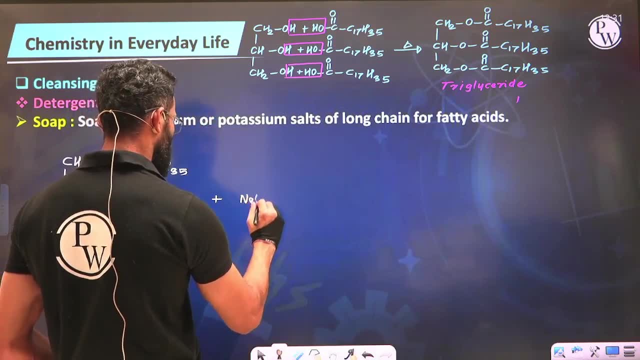 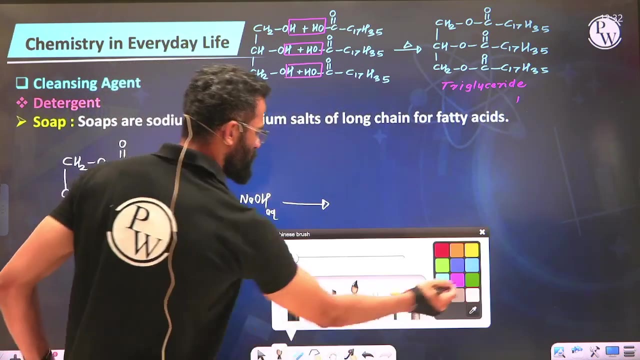 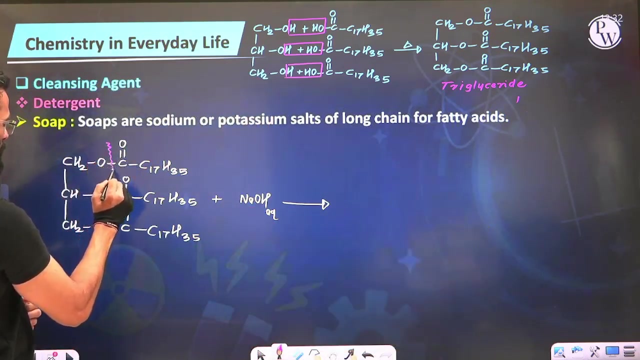 of glycerol, glycerol with stearic acid suppose, if i allow this, the process of alkaline hydrolysis. if we subject this to the process of hydrolysis, hydrolysis is breakage using water. so let's say breakage using water. if we carried hydrolysis, so everywhere ester linkage will be broken. 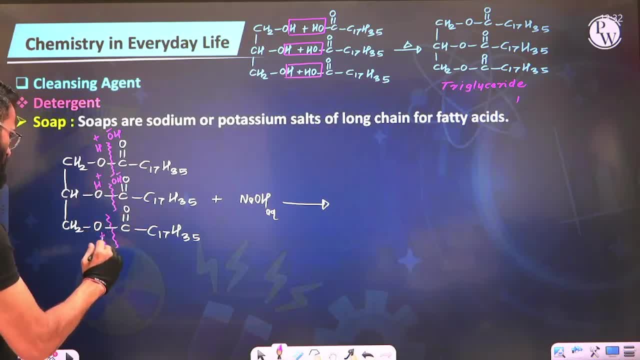 here as well. you'll see, the left hand side part is forming CH3, 2 OH, CH 2 H and CH 2 H, meaning we'll be getting glycerol back, and the right hand side part is forming C, 17 H, 35 COOH, that is, steric acid. so since we have got triacyl, let's say, if I multiply, 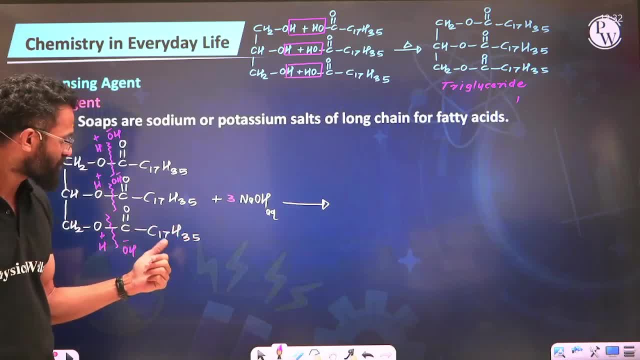 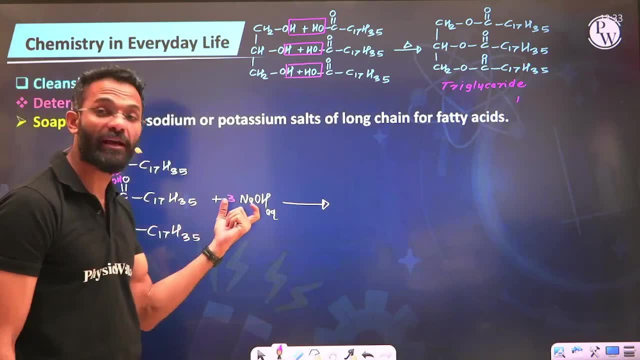 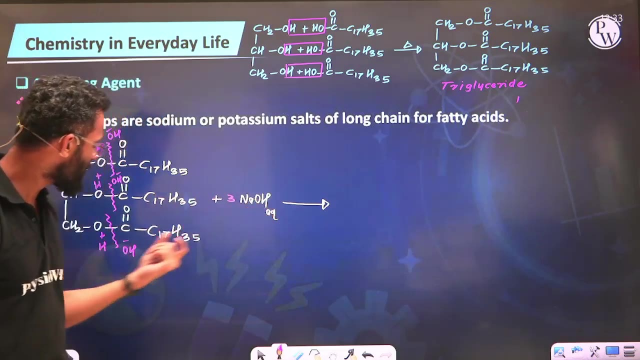 here by 3, so I'll be getting 3 equivalent of C 17 H 35 COOH, which is steric acid. but as soon as this acid will be formed, because conditions being alkaline, this base will react with an acid to form a salt. that salt would be OH, will take away H plus from here, so you will get C 17 H 35 COOH. 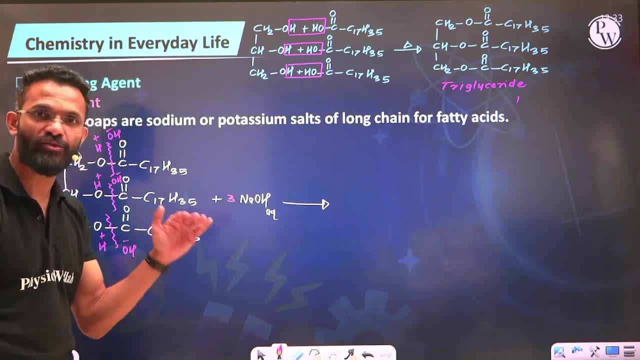 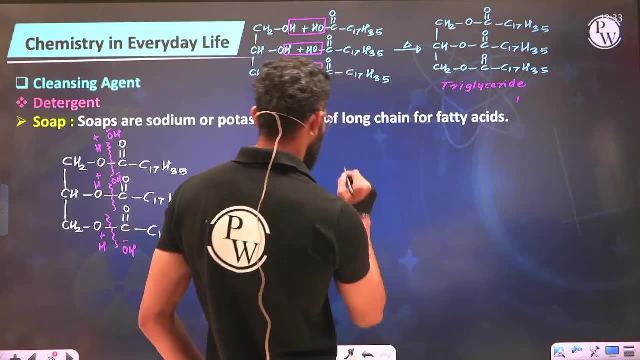 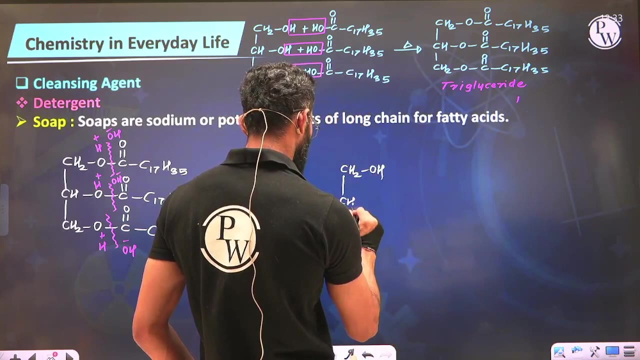 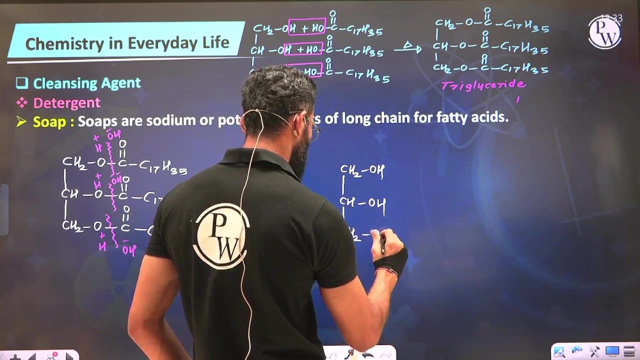 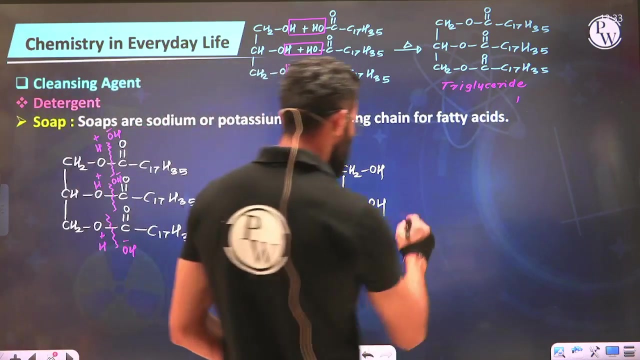 minus Na, plus, meaning it is going to be a sodium salt of steric acid. we can call it as sodium stearate. let us write down the structure first. we have got glycerol, and along with that we got C, 17, H, 35, COOH, na. 3. 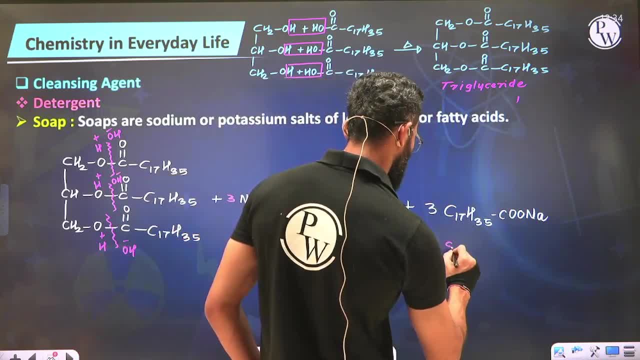 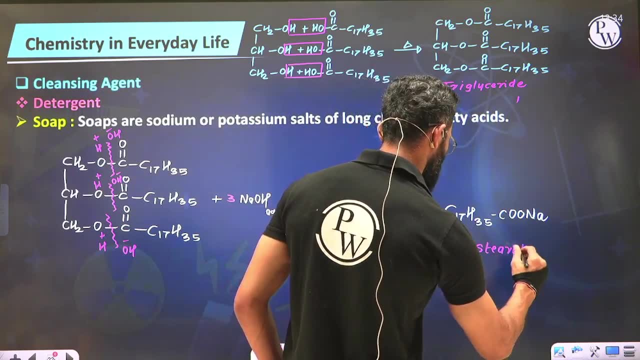 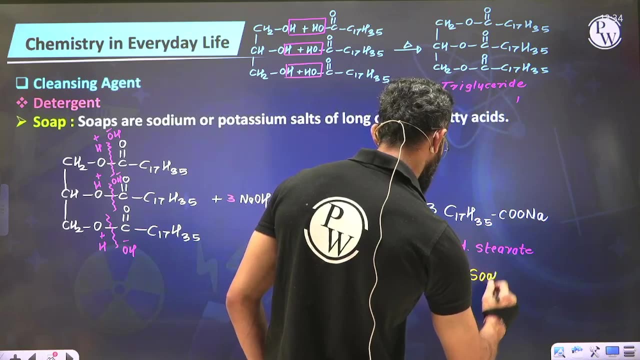 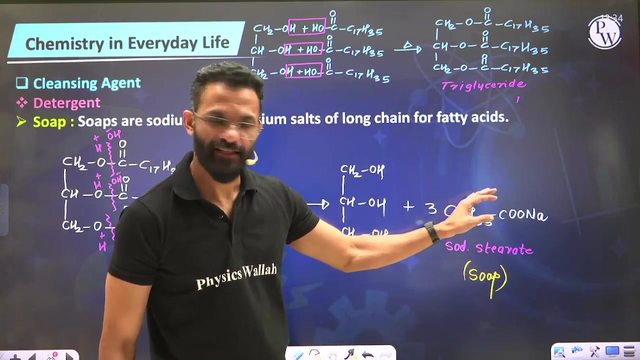 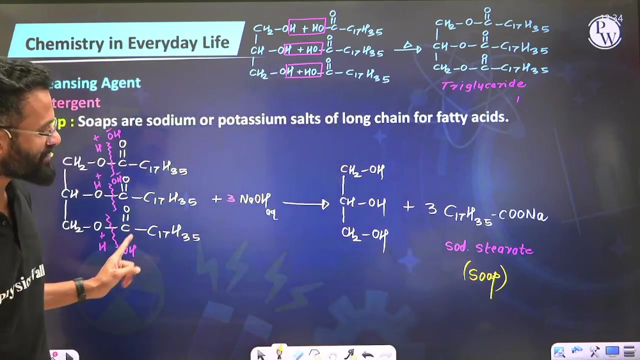 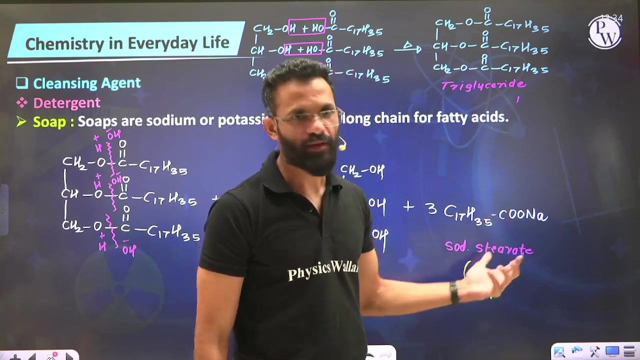 now this is what we are calling it as sodium, salt of steric acid, meaning sodium stearate. and your student? this sodium stearate is nothing but or soob. so can we find a Gladbetter? salt of fatty acid is what you call it as soap, so this soap is very commonly used as a cleansing. 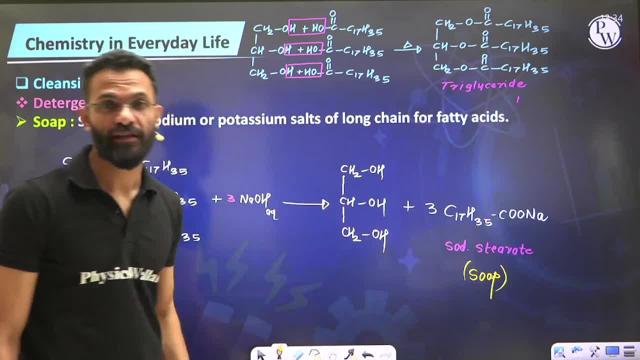 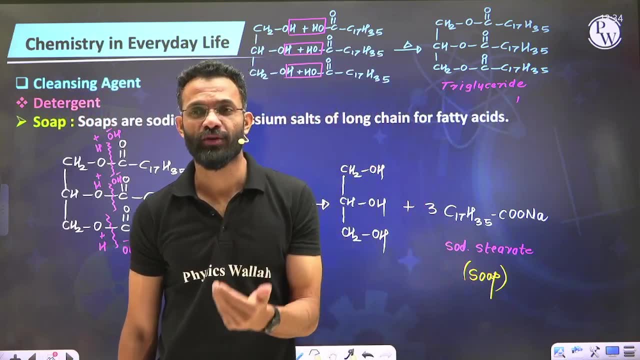 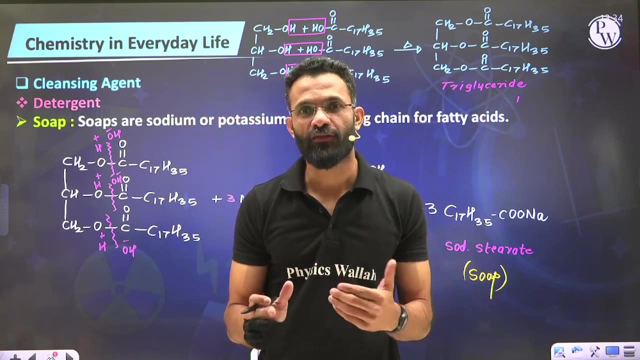 agent. as we know, in our daily life we come across soaps. however, there are limitation to the soup. well, in the chapter such as hydrogen, i'm sure you guys have come across something called as soft water and hard water. so if your water is hard, generally soap does not function that effectively. 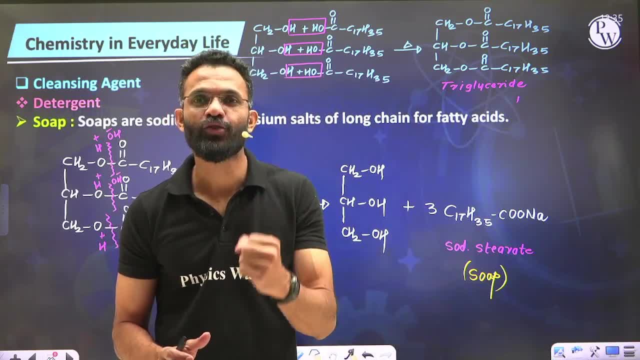 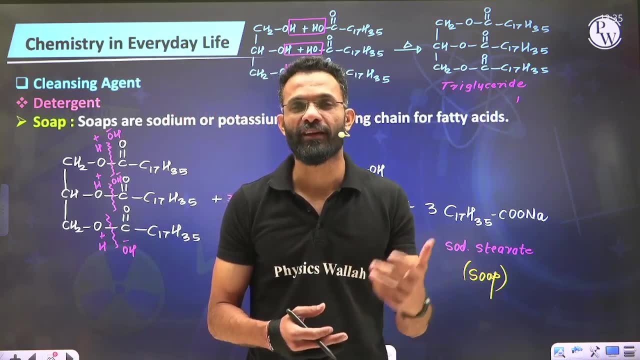 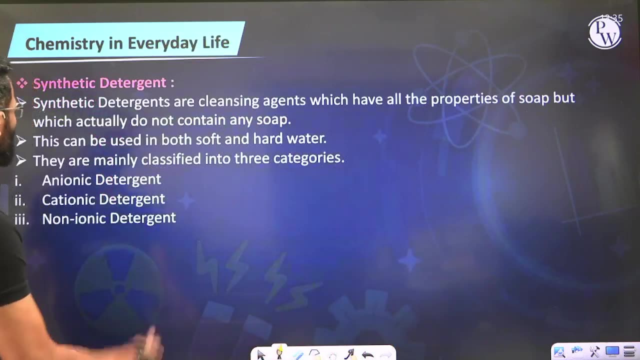 in hard water, because most of the soap gets consumed by the metal ions present in that hard water, and that's why the limitation of soap is that it is not that commonly effective in hard water. so, alternatively, what we do is we use a synthetic detergent. so what are synthetic detergent? 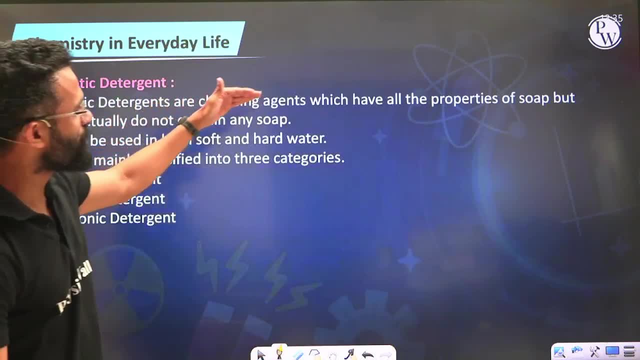 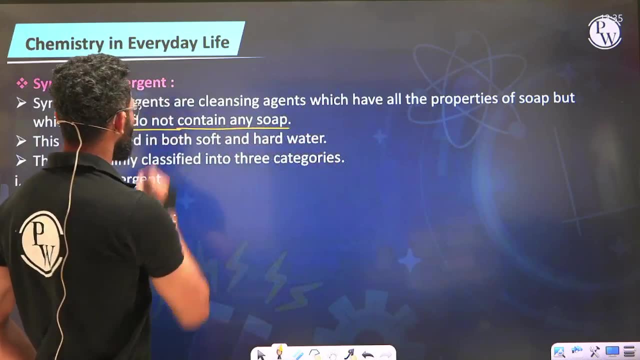 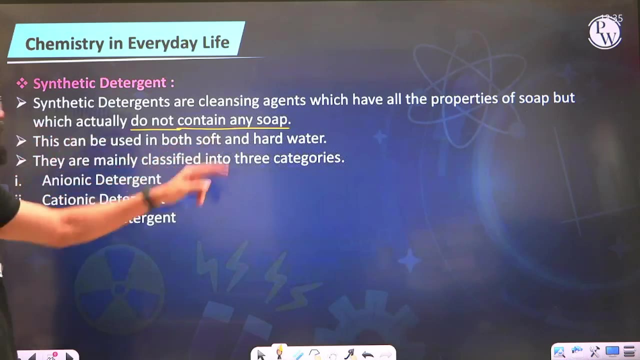 synthetic detergents are the cleansing agents which have all the properties of soap but do not contains any soap in it do not contain any soap but it has all the properties of soap. and the advantage is that synthetic detergent can be used in both soft and can be used 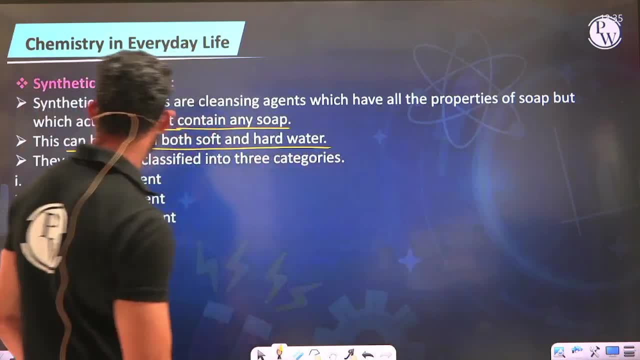 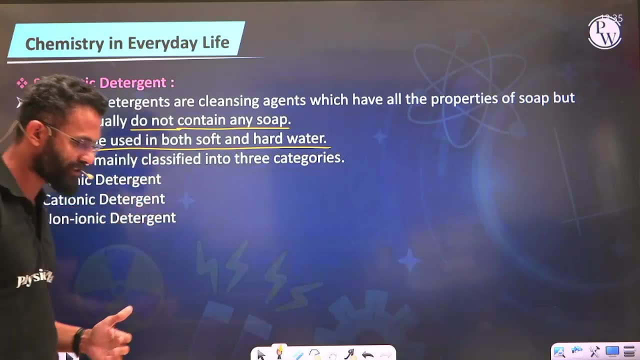 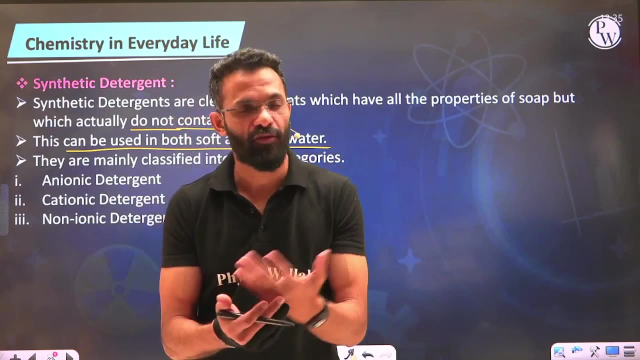 in both soft and hard water. we classify this detergent into three categories: cationic, anionic and non-ionic detergent. well, how exactly detergent functions to take away the fats from the fabric or from any other substance is what you have already studied in the chapter of surface chemistry, so we are not going to. 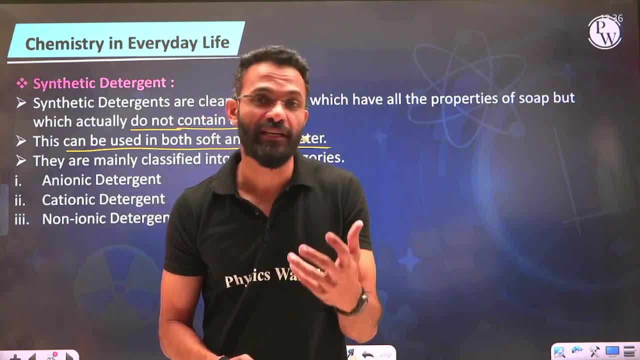 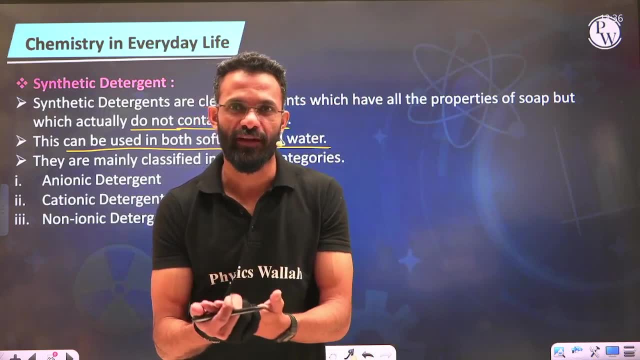 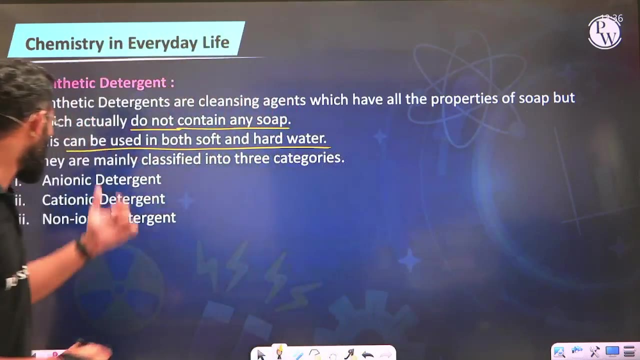 study the detail: ionic micelle formation of the detergent which are useful for the removal of fats or any other dust or any other substance which is attached to the fabric. you all have studied that in surface chemistry. we will be just getting introduced to three types of detergents: anionic- 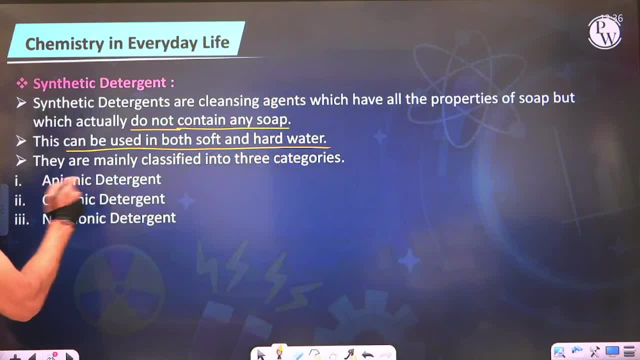 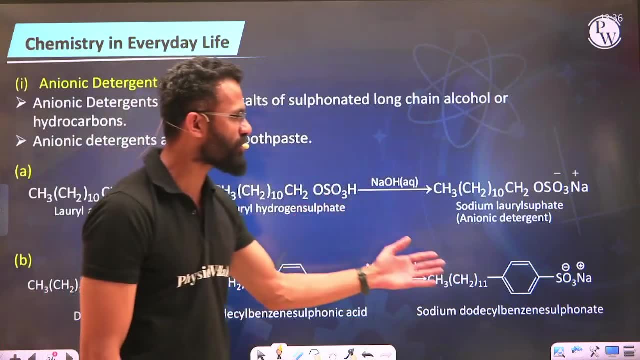 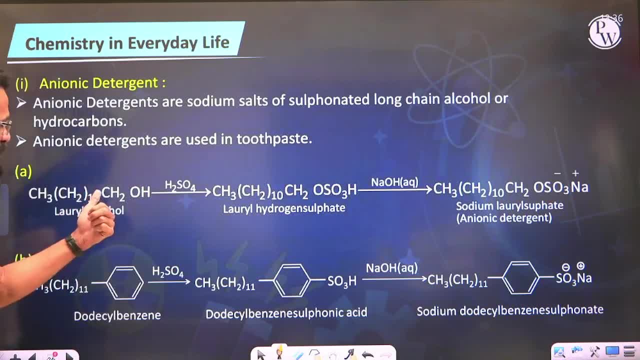 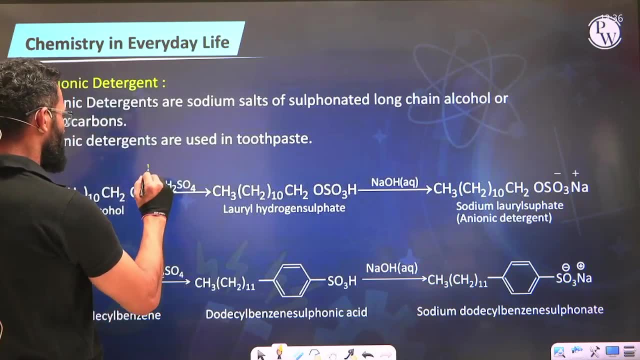 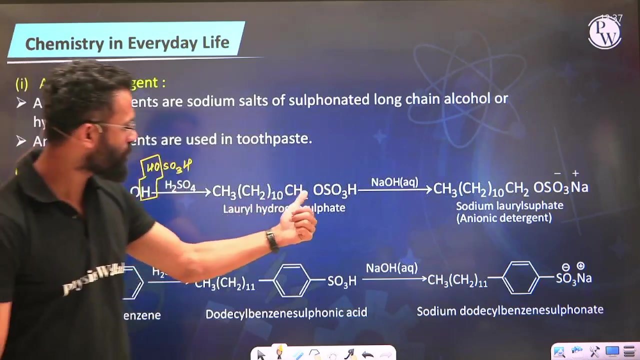 can see here, all together 12 carbon street chain containing function loop as an alcohol. if you allow this to react with sulfuric acid, well, to understand, let's write it this way: this is sulfuric acid and now? so if i remove water from you, what are we going to get? th3, ch2, 10 times ch2, oso3h, right, oso3h. this is what you call it as. 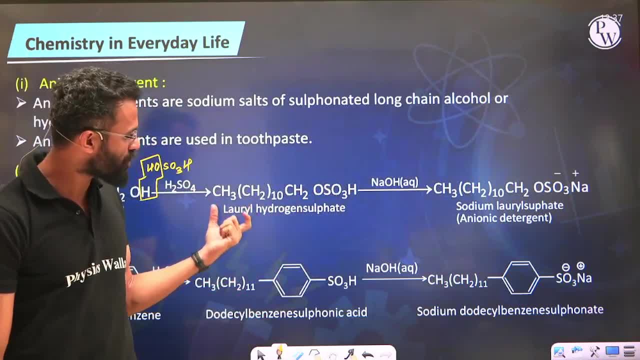 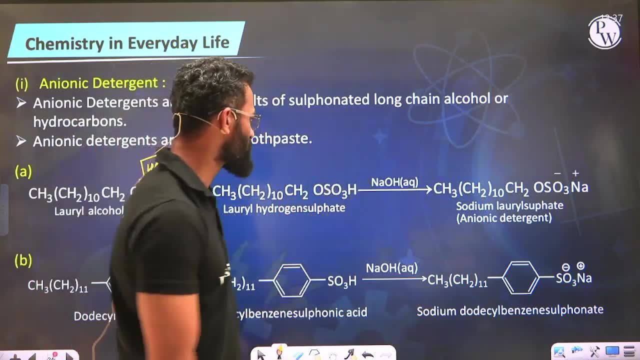 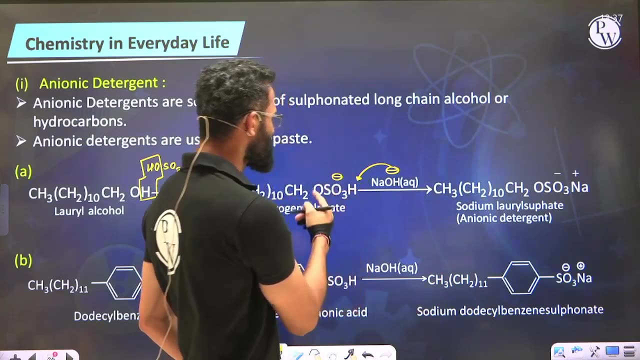 hydrogen sulfate of lauryl alcohol, so you can call it as lauryl hydrogen sulfate. now here at the end we have got sulfonic acid as a group. if i treat this with aqueous naoh naoh being base, it will accept h plus ion to form a conjugate base, that is, oso3 minus. 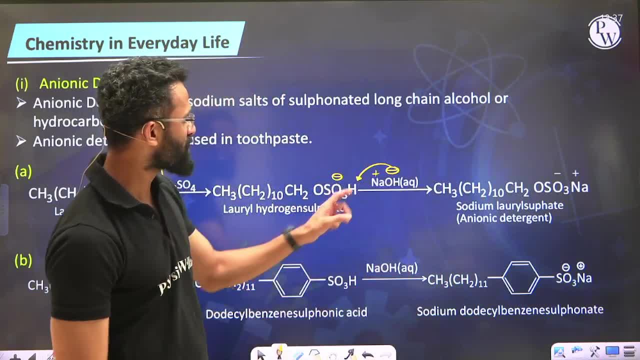 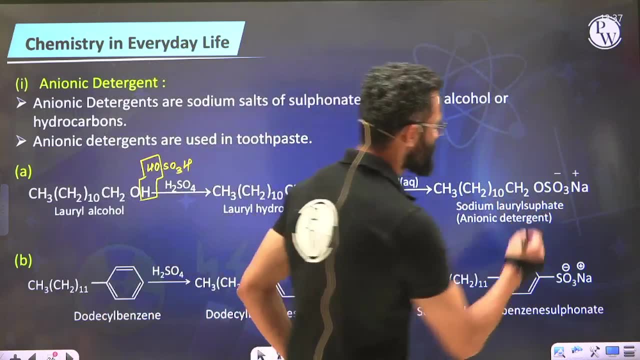 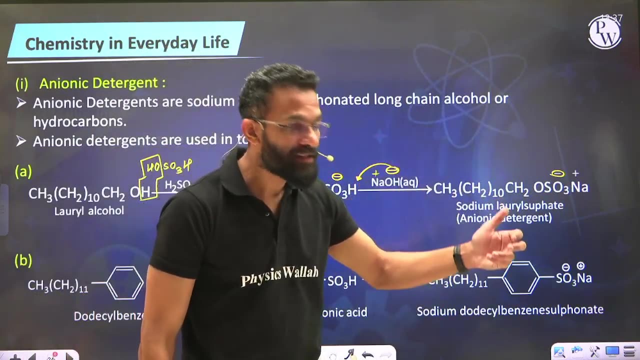 which will be balanced by this na plus. so we are going to get sodium salt of lauryl hydrogen sulfate, so you call it as sodium lauryl sulfate. now, since the end of this compound is anionic, to this anionic end it can bind to that dirt or dust which is supposed to be removed from the 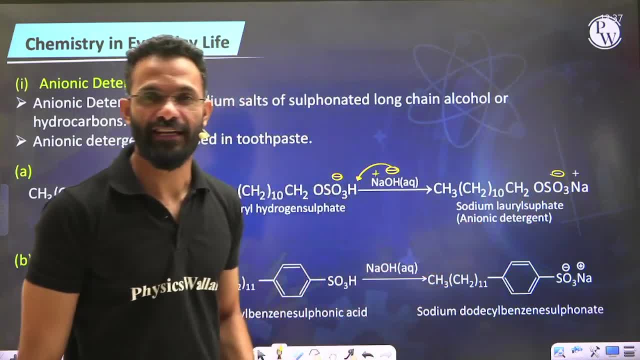 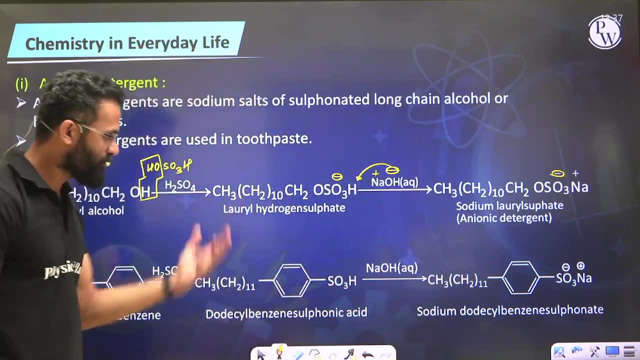 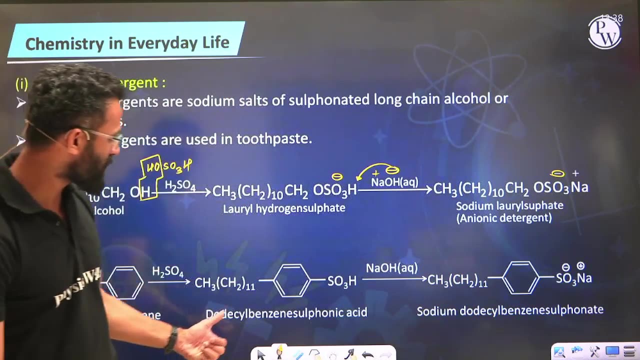 fabric, and that's why such kind of detergents which are helpful for the removal of dirt through its anionic end, we call them as anionic detergent. one more example of anionic detergent: you can see here dodecyl benzene, which is sulfonated first to give you dodecyl benzene, sulfonic acid again when you treat that with the 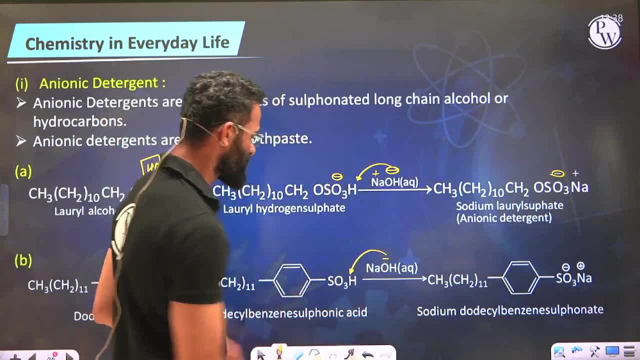 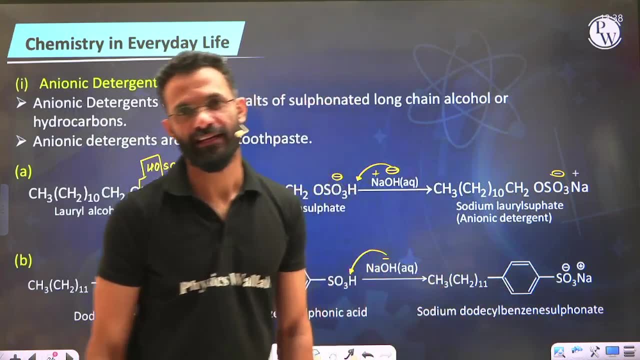 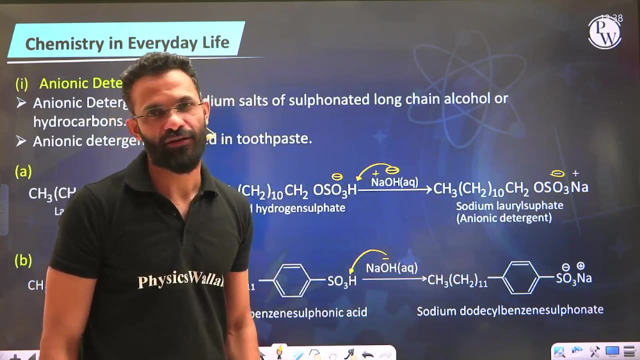 base. base will accept H plus and convert that into a sodium salt. so sodium dodecyl benzene sulfonate is another example of anionic detergent. guys, you will just have to remember the names and once you remember the name, i guess remember the structure is not really that difficult. 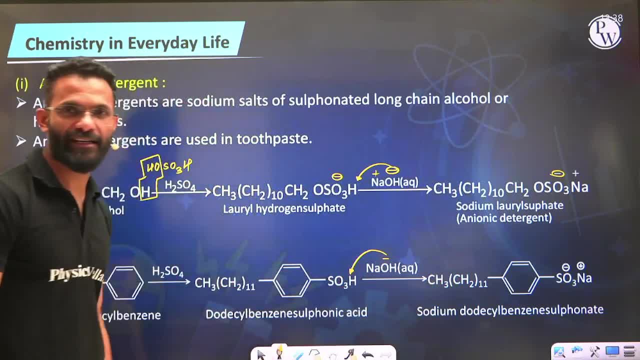 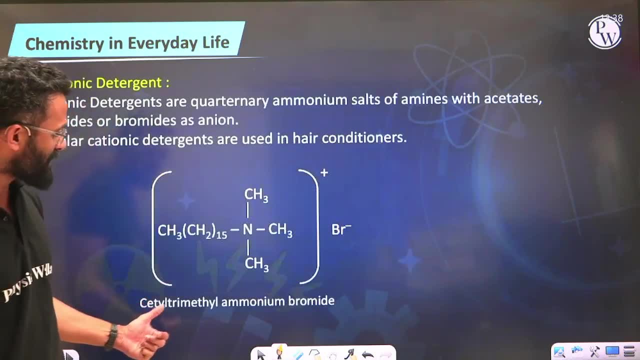 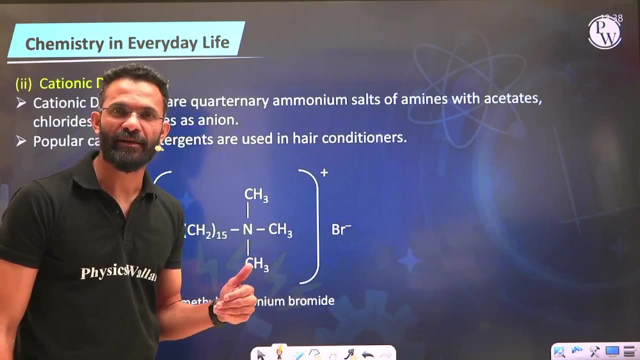 so this two example belong to category of anionic detergent. likewise, there exists cationic detergent. a very famous example of that is cetyltrimethyl ammonium bromide. well, you will find, in general, cationic detergents are basically ammonium salt of acetate or halides. but the common example which 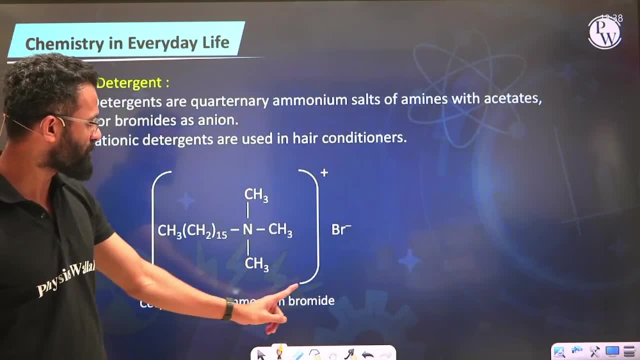 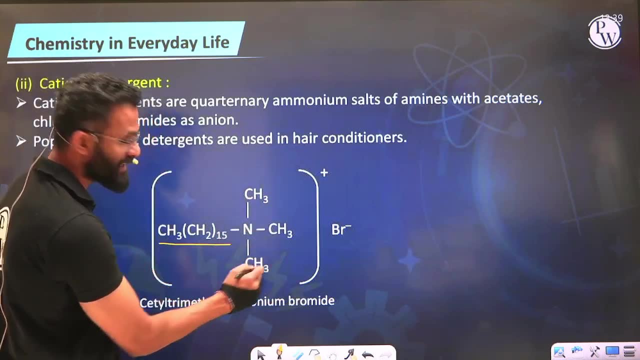 you all will have to remember, is this cetyltrimethyl ammonium bromide. so you can see, there is a long chain of hydrocarbon which is further connected to nitrogen, which is methylated. so this is your cetyltrimethyl ammonium bromide and you will see. 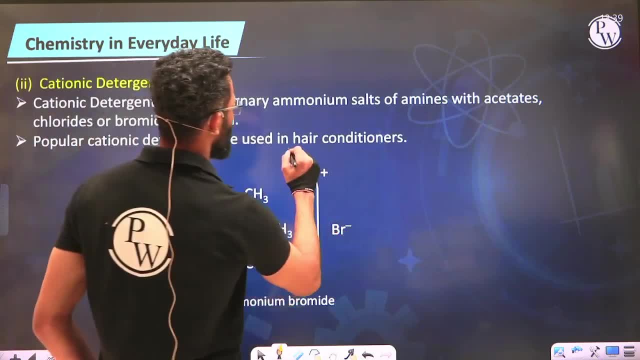 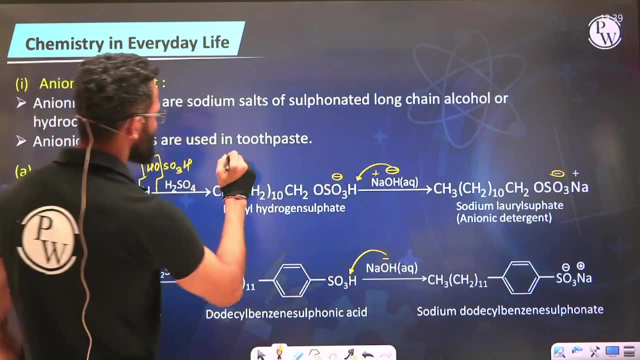 that this cationic detergents are very commonly used in hair conditioners. and when you talk about anionic detergents, these anionic detergents are very commonly used in toothpaste. so, as a usage, you may have to remember that this cationic detergent is very commonly used in toothpaste. 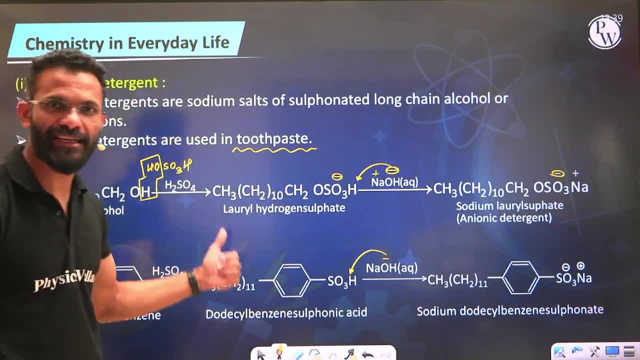 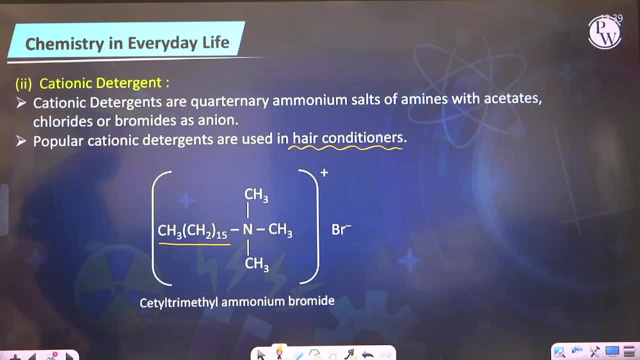 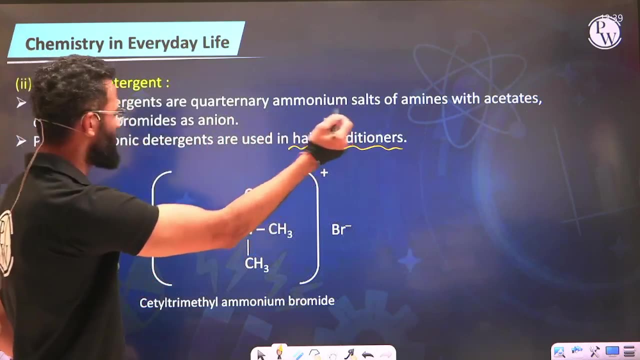 so these two are the example of anionic detergents, and what we saw here, cetyltrimethyl ammonium bromide, is example of cationic detergents. what are cationic detergents? they are generally quaternary ammonium salts of amine with acetate, or in general halides, as anion. and then there exists third. 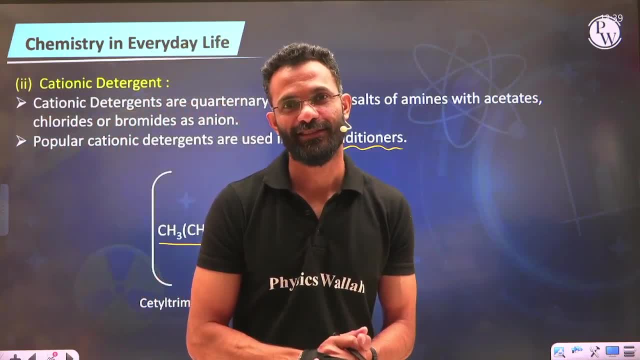 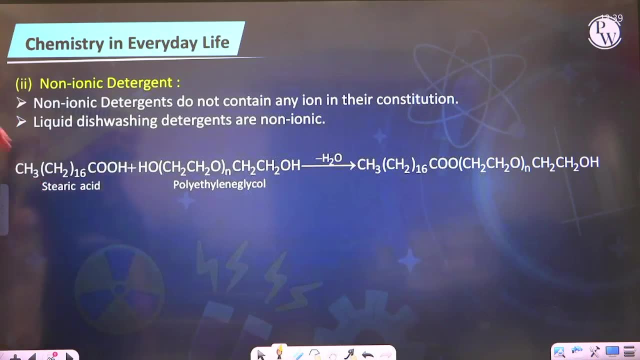 category that is called as non-ionic detergents. so non-ionic detergents example that you all will have to remember is basically, it is an ester of stearic acid and polyethylene glycol. so just now we saw example of stearic acid that is c17h35 coh, which we are treating with polyethylene glycol. now, if we carry, 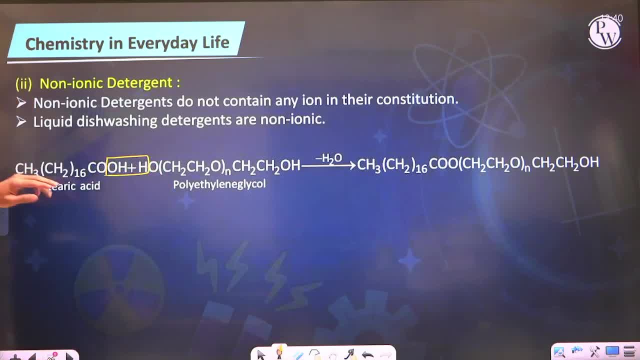 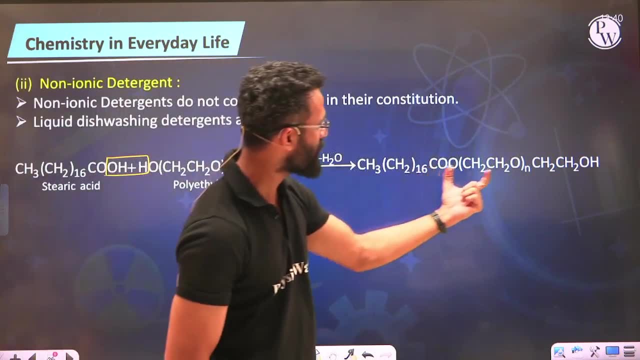 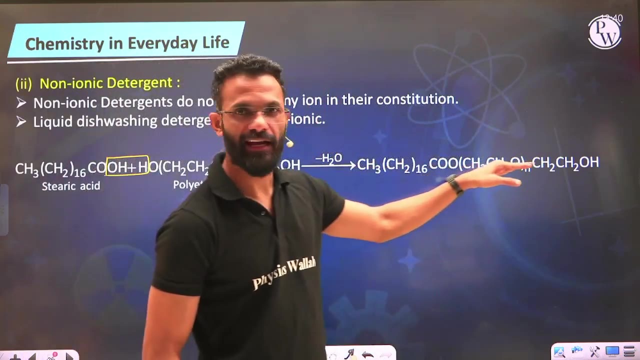 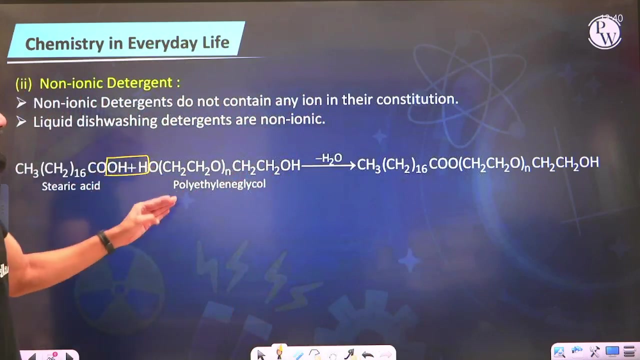 out condensation, you will see stearic acid will be forming an ester linkage here, so coo and further chain. so this is basically a substance which is neither carrying cationic nor anionic in here, so you call it as non-ionic detergents. example is ester of stearic acid and polyethylene glycol glycol.